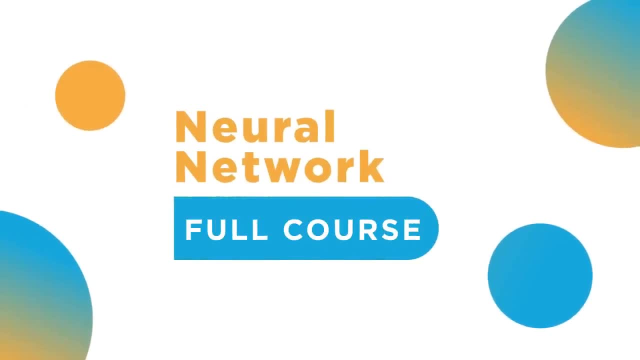 Neural networks, typically used in deep learning, are computing systems inspired by the structure and function of a human brain. It is used to find solutions to those problems for which the algorithmic method is expensive or does not exist. Neural networks learn by example, so we do not need to program it in depth. 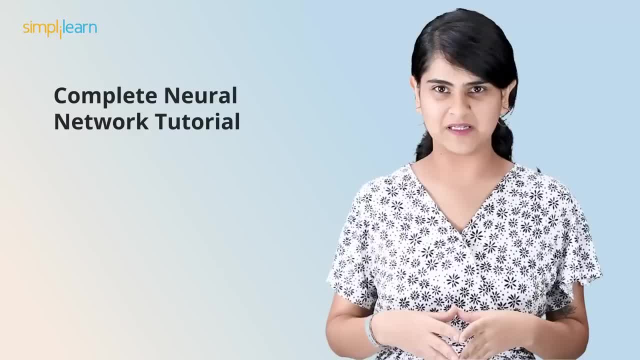 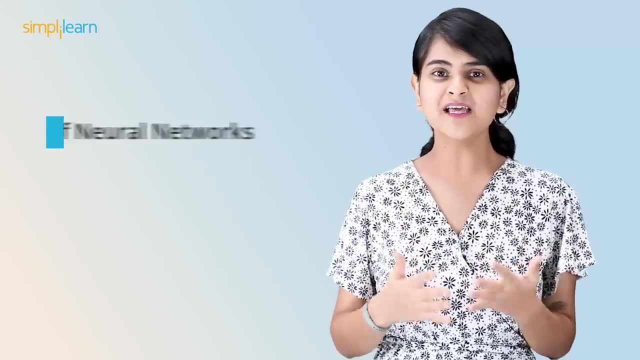 Hi guys, welcome to the complete neural network tutorial by simply learn. But before we begin, make sure to subscribe to our channel and hit the bell icon to never miss an update. First we will understand the basics of neural networks and see its practical implementation. 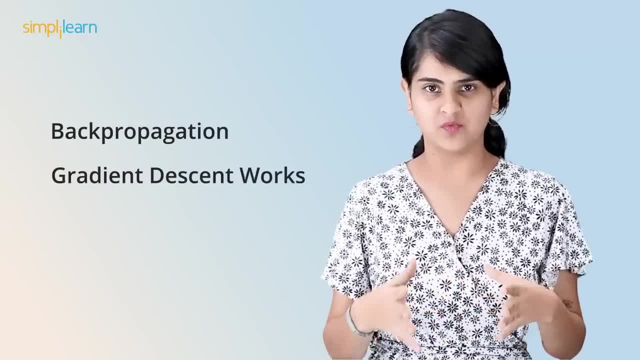 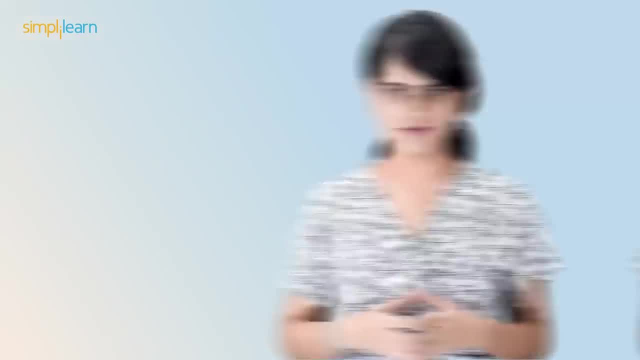 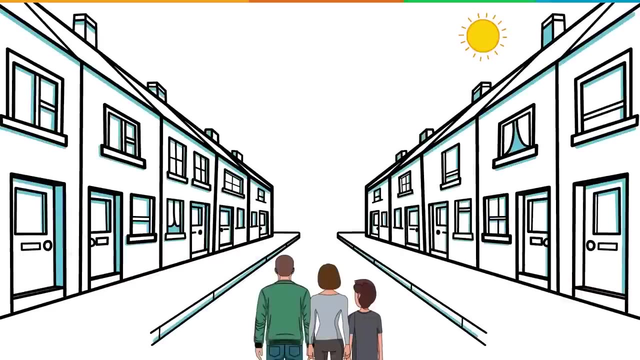 Then we will learn how back propagation and gradient descent works. Finally, we will understand the concepts and practical implementation of convolutional and recurring neural networks. Let's first look at a small animated video to understand neural networks better. Last summer, my family and I visited Russia, Even though none of us could read Russian. 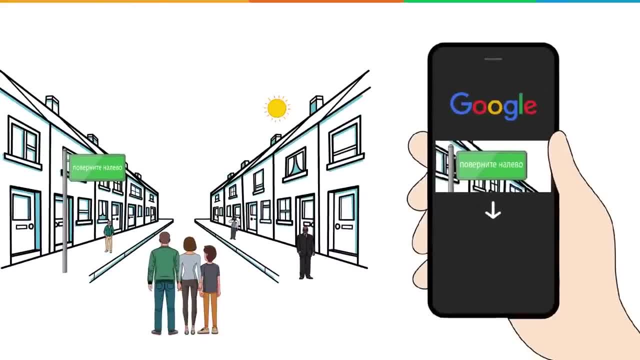 we did not have any trouble, So we decided to learn the basics of neural networks and see its practical implementation. It is very simple and figuring our way out, All thanks to Google's real-time translation of Russian boards into English. This is just one of the several applications of neural 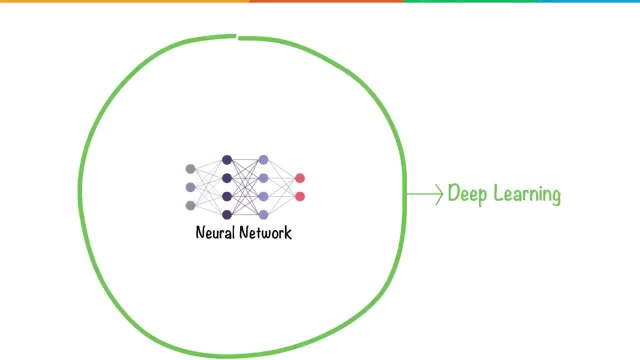 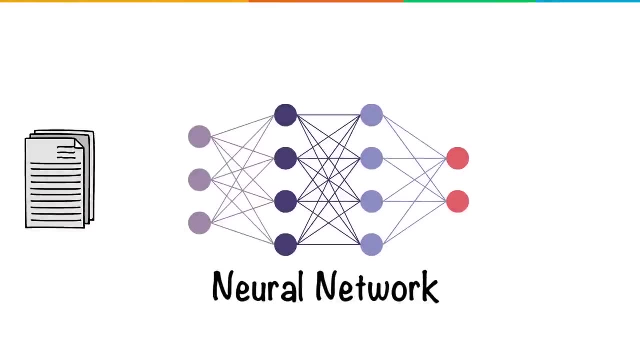 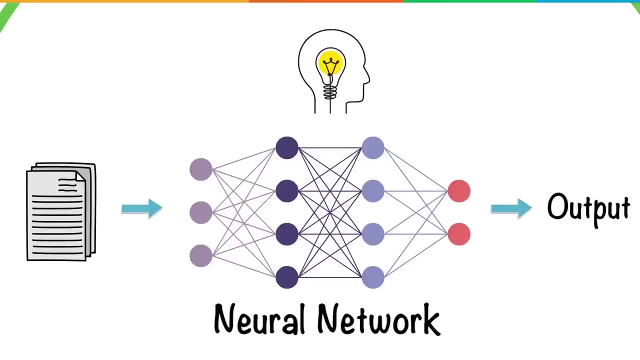 networks. Neural networks form the base of deep learning, a subfield of machine learning where the algorithms are inspired by the structure of the human brain. Neural networks take in data, train themselves to recognize the patterns in this data and then predict the outputs for a new set of similar data. Let's understand how this is. 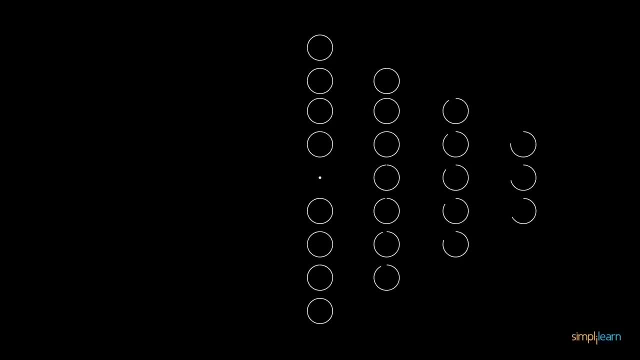 done. Let's construct a neural network that differentiates between a square, circle and triangle. Neural networks are made up of layers of neurons. These neurons are the core processing units of the network. First we have the input layer, which receives the input, The output layer. 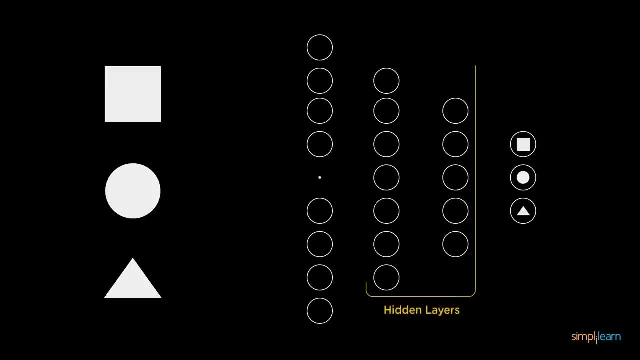 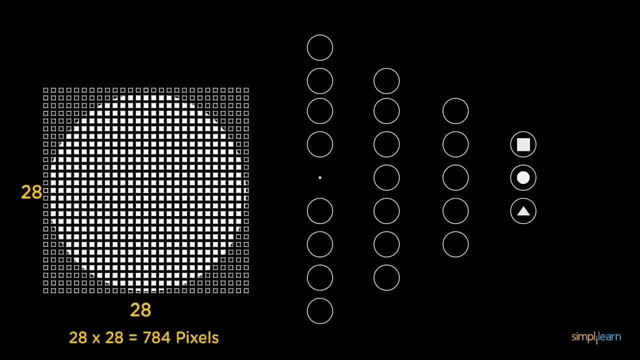 predicts our final output. In between exist the hidden layers which perform most of the computations required by our network. Here's an image of a circle. This image is composed of 28 by 28 pixels, which make up for 784 pixels. Each pixel is fed as input to each. 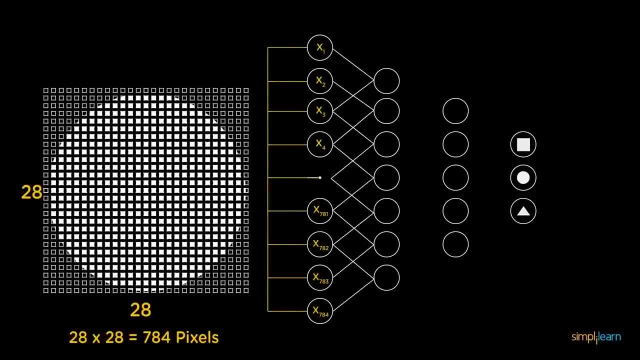 neuron of the first layer. Neurons of one layer are connected to neurons of the next layer through channels. Each of these channels is assigned a numerical value known as weight. The inputs are multiplied to the corresponding weights and their sum is sent as input to. 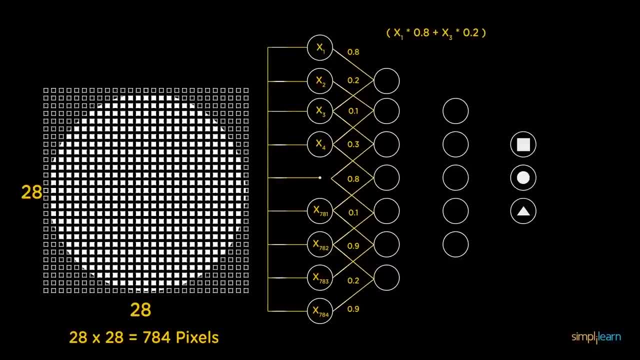 the neurons in the hidden layer. Each of these neurons is associated with a numerical value called the bias, which is then added to the input sum. This value is then passed through a threshold function called the activation function. The result of the activation function determines if the particular neuron will get activated or not. An activated 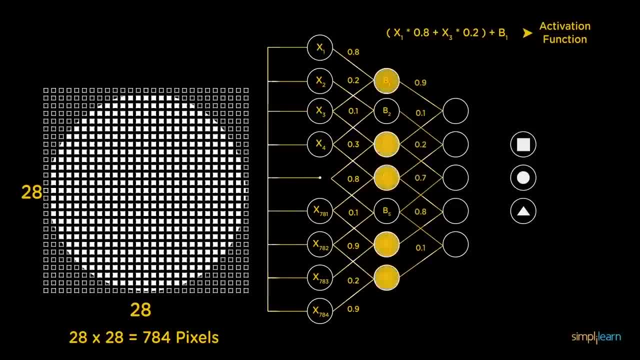 neuron transmits data to the neurons of the next layer over the channels. In this manner, the data is propagated through the network. This is called forward propagation. In the output layer, the neuron with the highest value fires and determines the output. The 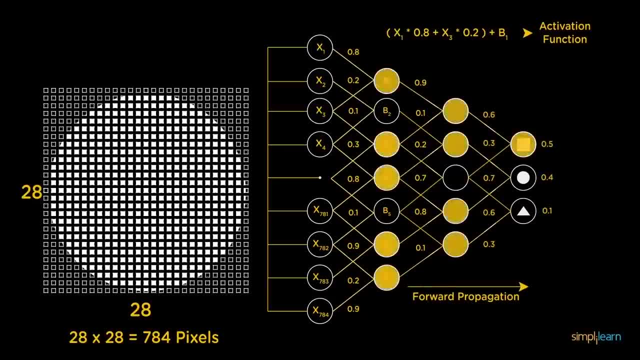 values are basically a probability. For example, here our neuron associated with square has the highest probability. Hence that's the output predicted by the neural network. Of course, just by a look at it we know our neural network has made a wrong prediction. 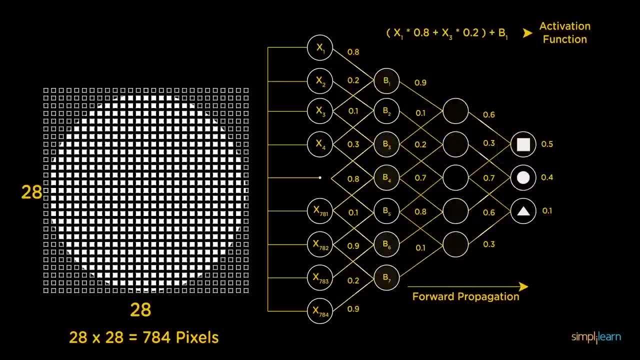 But how does the network figure this out? Note that our network is yet to be trained. During this training process, along with the input, our network also has the output fed to it. The predicted output is compared against the actual output to realize the error in prediction. 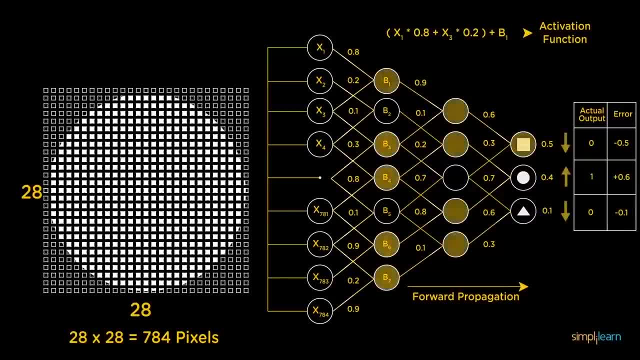 The magnitude of the error indicates how wrong we are, and the sign suggests if our predicted values are higher or lower than expected. The arrows here give an indication of the direction and magnitude of change. to reduce the error, This information is then transferred backward through. 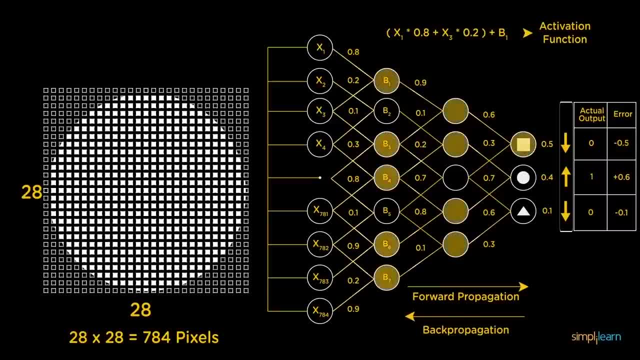 our network. This is known as back propagation. Now, based on this information, the weights are adjusted. This cycle of forward propagation and back propagation is iteratively performed with multiple inputs. This process continues until our weights are assigned such that the network can. 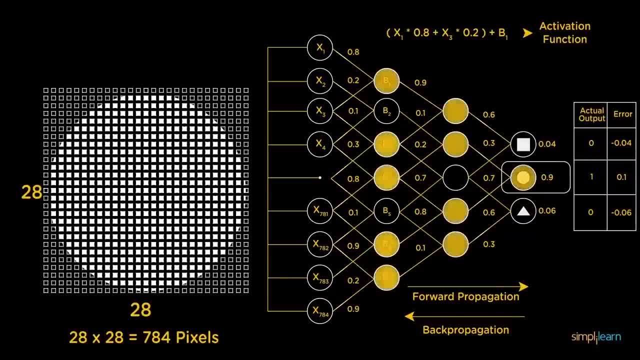 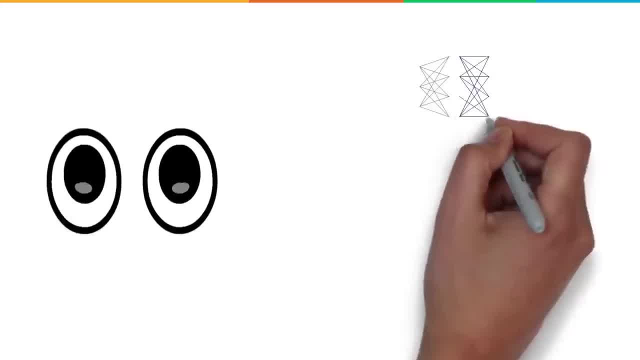 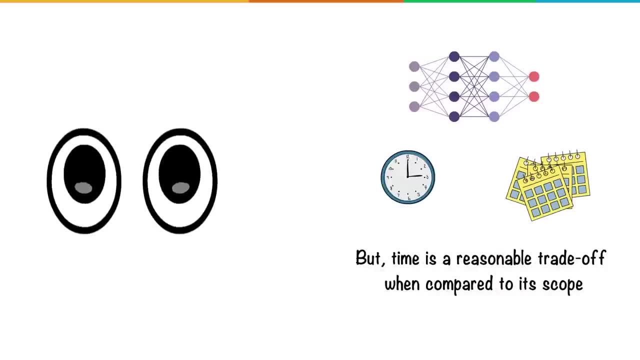 predict the shapes correctly. in most of the cases, This brings our training process to an end. You might wonder how long this training process takes. Honestly, neural networks may take hours or even months to train, But time is a reasonable trade-off when compared to its scope. Let us look at some of the prime applications of neural networks. 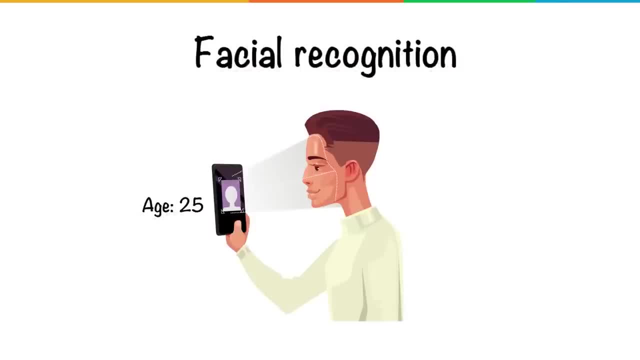 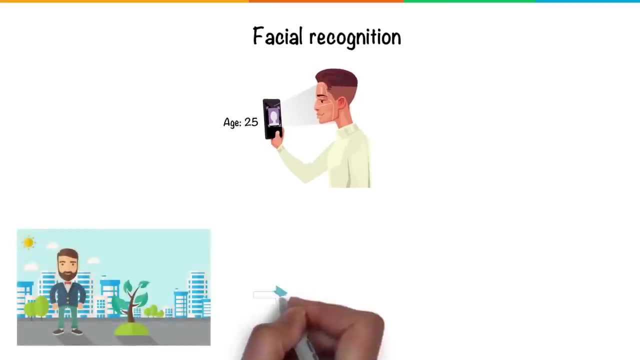 Facial recognition Cameras on smartphones these days can estimate the age of the person based on their facial features. This is neural networks at play, first differentiating the face from the background and then correlating the lines and spots on your face to a possible age. 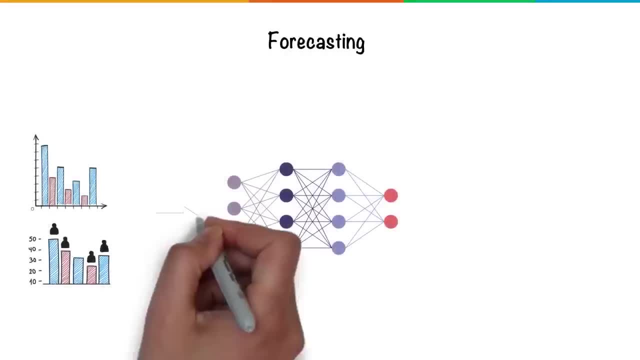 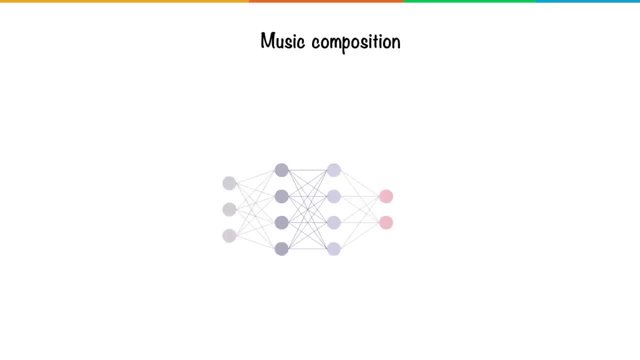 Forecasting. Neural networks are trained to understand the patterns and detect the possibility of rainfall or a rise in stock prices with high accuracy. Music composition: Neural networks can even learn patterns in music and train itself enough to compose a fresh tune. So here's a question for you: Which of the following statements does not hold true? 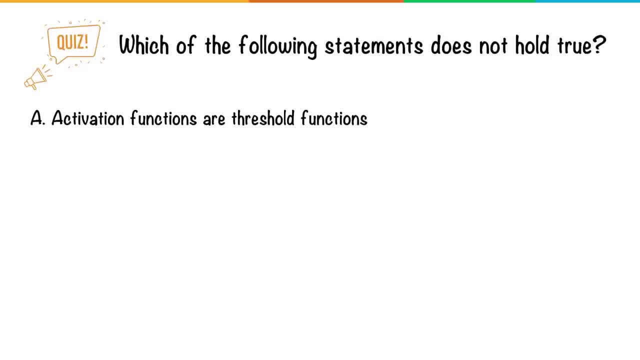 A- Activation functions are threshold functions. B- Error is calculated at each layer of the neural network. C- Both forward and back propagation take place during the training process of a neural network. D- Most of the data processing is carried out in the hidden layers. 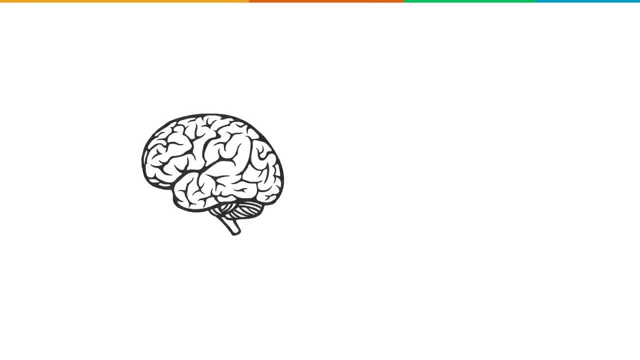 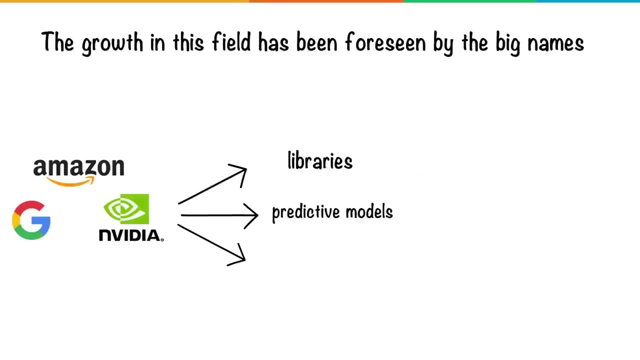 Leave your answers in the comment section below. With deep learning and neural networks, we are still taking baby steps. The growth in this field has been foreseen by the big names. Companies such as Google, Amazon and Nvidia have invested in developing products such as libraries, predictive models and 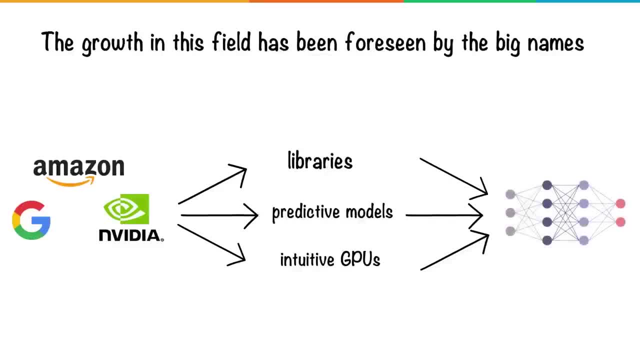 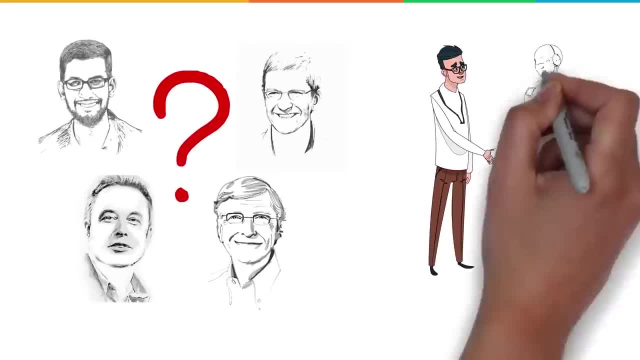 intuitive generalization. This is the first step in the development of neural networks. This is the first step in the development of neural networks. The question dividing the visionaries is on the reach of neural networks. To what extent can we replicate the human brain? We'd have to wait a few more years to give a definite answer. 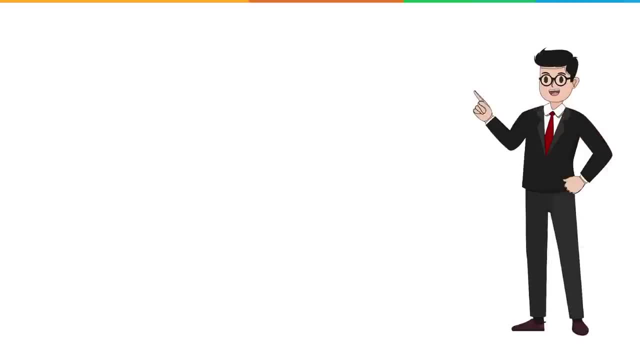 But if you enjoyed this video, it would only take a few seconds to like and share it. Also, if you haven't yet, do subscribe to our channel and hit the bell icon, as we have a lot more exciting videos coming up. Fun learning till then. 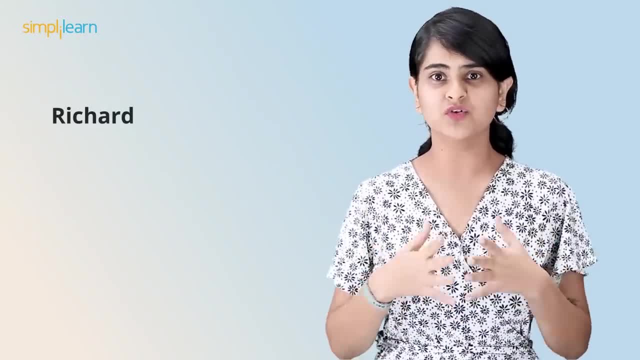 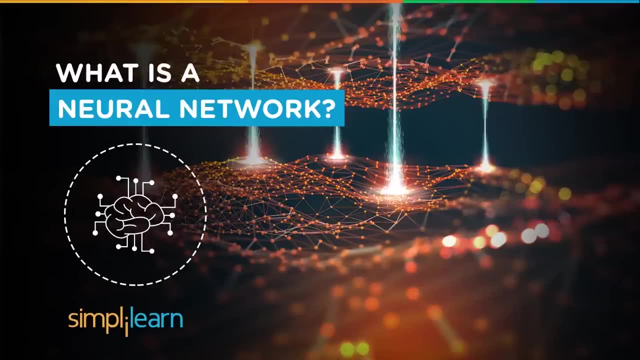 Now we have Richard, who will take you through the remaining part of the course and make you understand neural networks in detail. With that, over to you, Richard. What is a neural network? Welcome to today's lesson. My name is Richard Kirshner. I'm with. 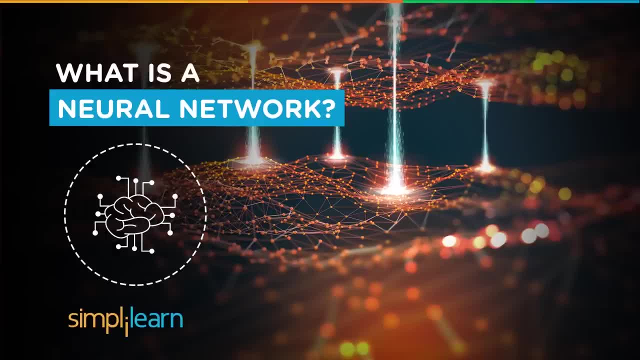 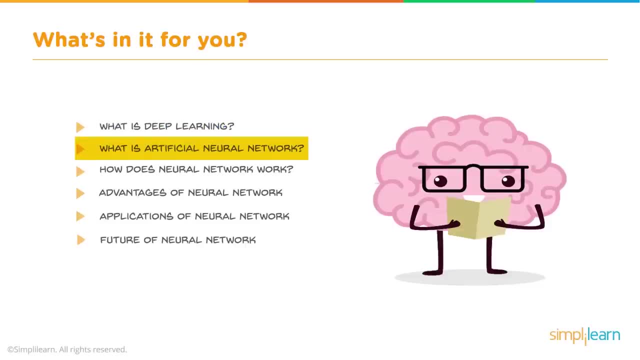 the Simply Learn team. Today we want to discuss the very basics of a neural network and what that is. So what's in it for you today? What is deep learning? What is artificial neural network? How does neural network work? Advantages of a neural network. 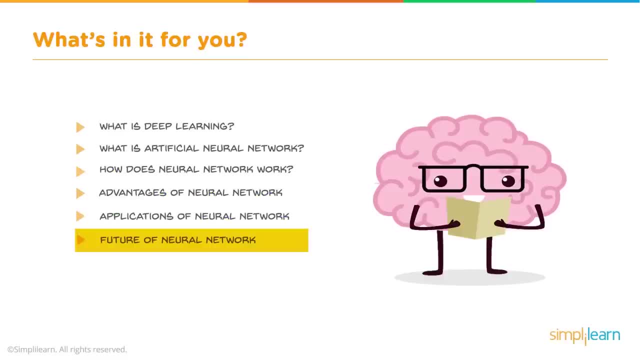 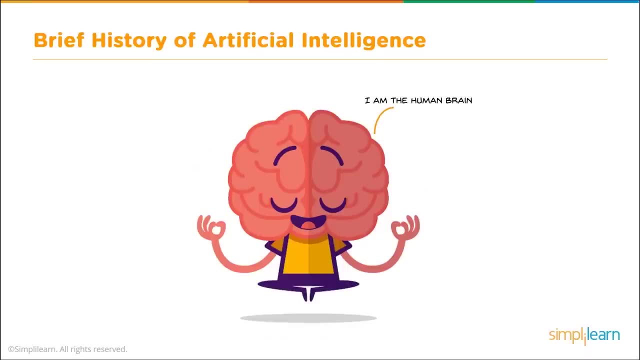 Applications of a neural network And the future of neural networks. Let's start with a brief history of the artificial intelligence. Hello, I am the human brain. This one is seeking enlightenment and has sat and meditated. I am the most complex organ in the human body and I help you to think, understand and make. 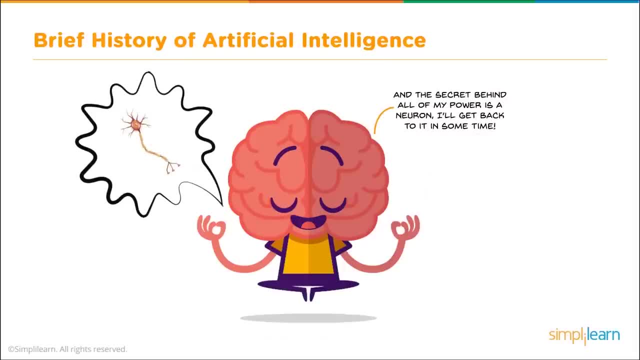 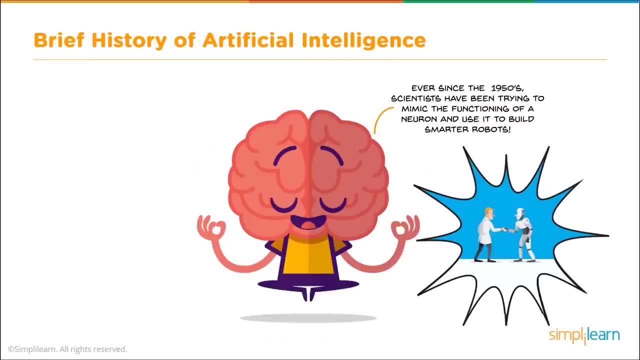 decisions, And the secret behind all my power is a neuron. I'll get back to that in some time. Ever since the 1950s, scientists have been trying to mimic the functioning of a neuron and use it to build smarter robots. After a lot of trial and error, humans finally designed a computer. 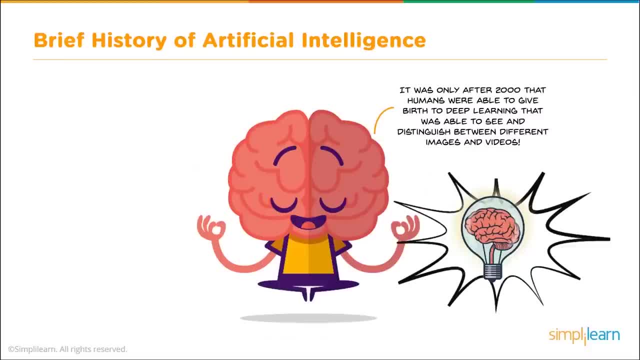 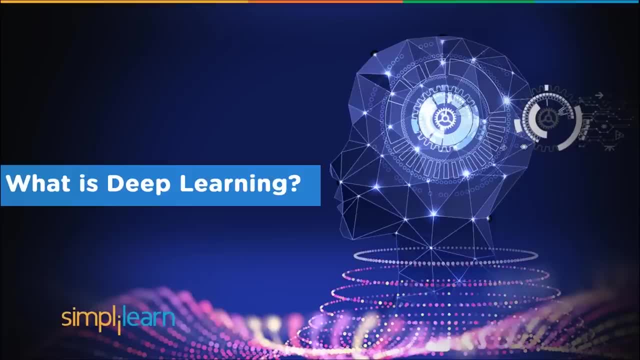 that can recognize human speech. It was only after 2000 that humans were able to give birth to deep learning, that was able to see and distinguish between different images and videos. So, looking at that, let's dive into what is deep learning. Now your first thought might be: it's the opposite. 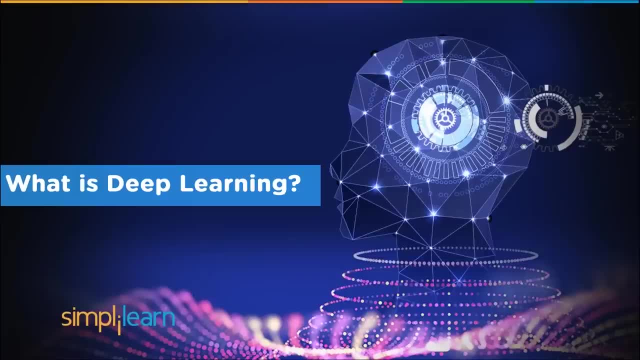 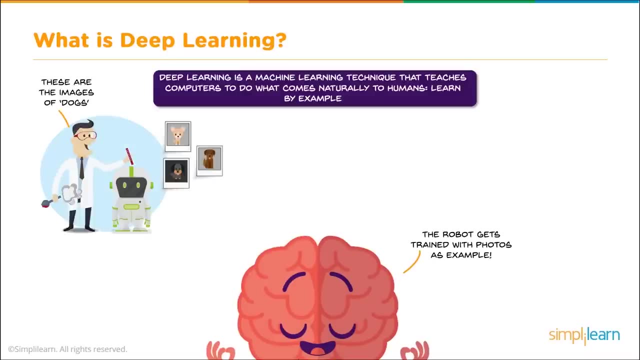 of shallow learning, No Deep learning. I liken to a magic box, And let's go in there and just take a look as to why it's kind of a magic box. So what exactly is deep learning? These are the images of dogs. Deep learning is a machine learning technique that teaches computers. 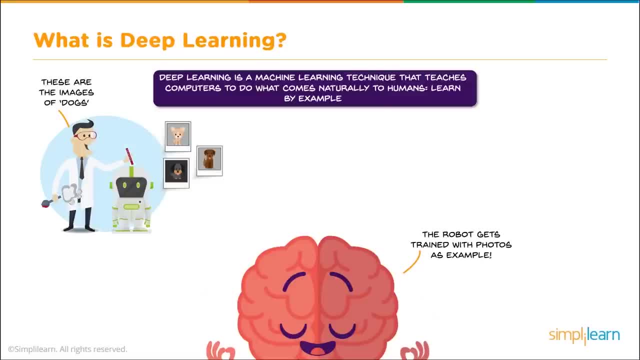 to do what comes naturally to humans: Learn by example. The robot gets trained with photos as example. Now, this is very different than hardwiring a computer program so that it recognizes something It actually learns, And that's where it's a magic box, because you don't really control how it learns. 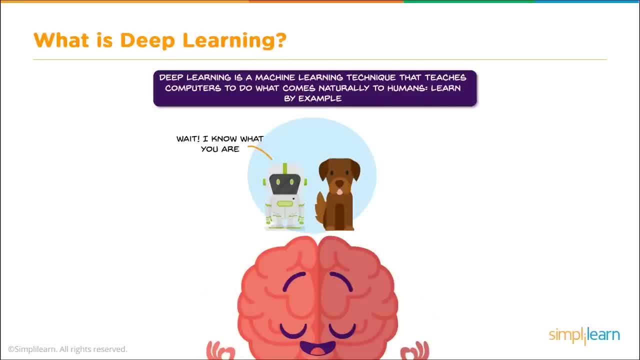 You control the aspects that go in, The computer comes back and says: wait, I know what you are. It looks at the photograph of the dog and it's able to identify that it saw in the images It says are a dog, Woof, woof. So that's an example of deep learning. You'll notice we didn't go in. 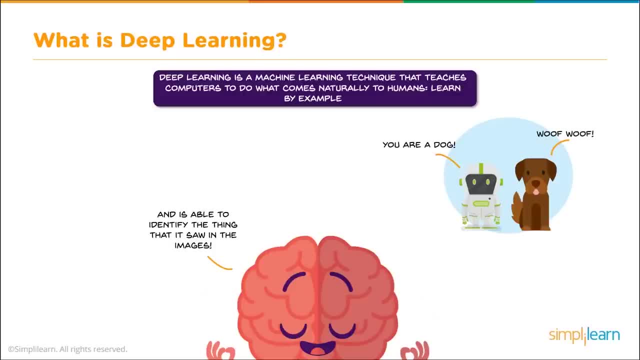 we'll go into the actually how it works behind the scenes for a neural network. But there's a bit of feeling of magic And that's where the term deep learning comes in, And that's also the term where I like to call it a magic box. You put these things in here into the program and it starts. 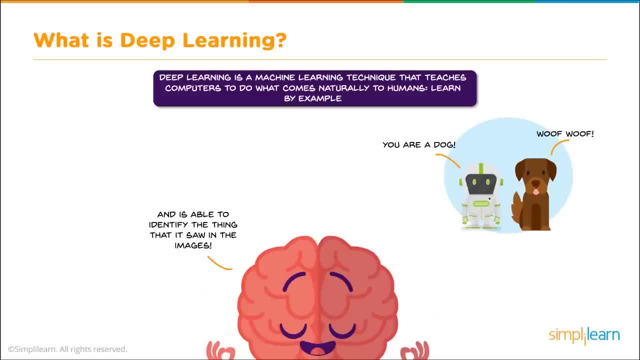 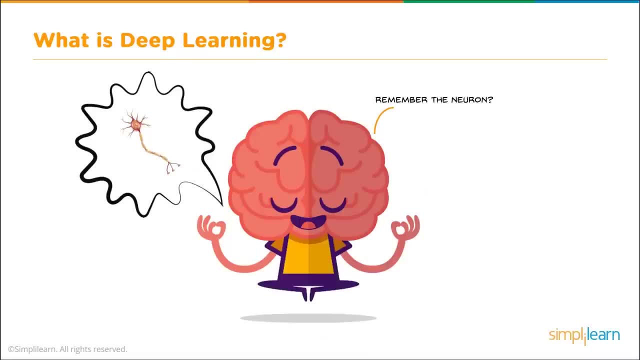 running the deep learning and you have to understand those settings, But you don't have to follow the exactly what's going on in the deep learning model. That brings us to the question: how does deep learning do it? Remember, the neuron Scientists managed to. 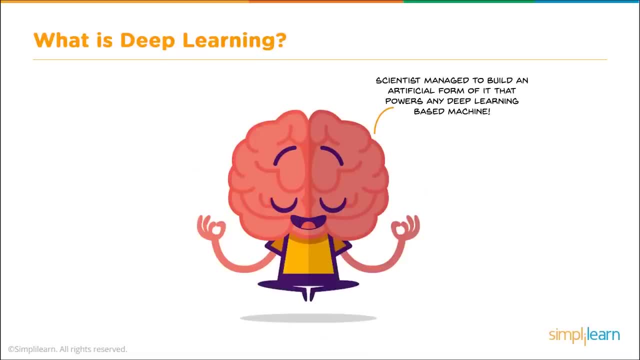 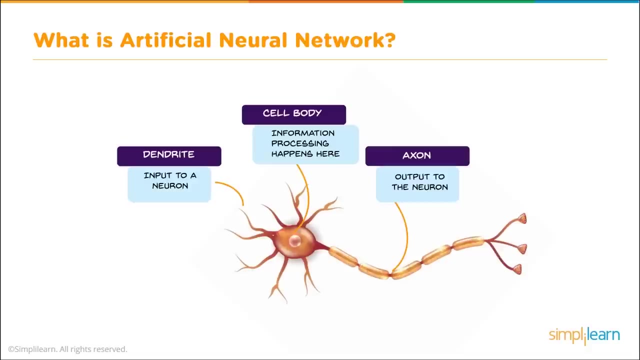 build an artificial form of it that powers any deep learning based machine. So let's talk about artificial neural networks. What is an artificial neural network? To understand how an artificial neuron works, we need to understand how the real one works. First, we have a dendrite. 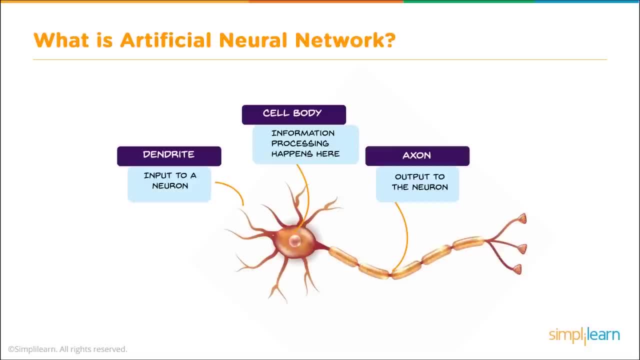 the input to the neuron And you can see these little hairs that come in and they receive information. Then we have the cell body. Information processing happens here. So it takes all these different dendrite and information coming in from the different dendrites And it looks at that information And then you have your axon, which is the output. 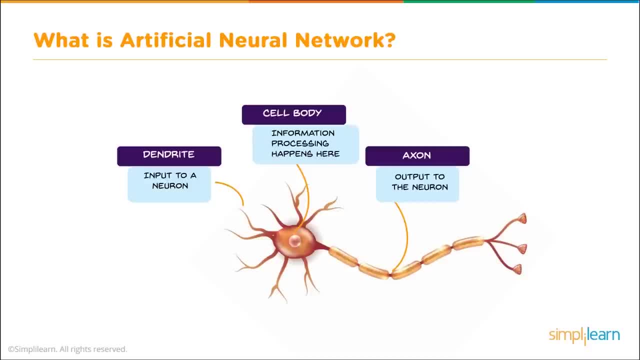 to the neuron. So there goes your axon And you see, it goes all the way out And at the very end it flanges out. Each one of those little flanges connects to the dendrite or the hairs on the next. 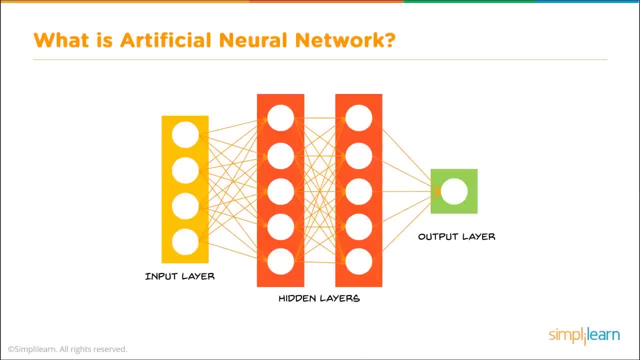 one. Now let's see what an artificial neural network looks like. So an artificial neural network, we have an input layer, So that could be an array of data. Each one of those white dots in the yellow bar would represent, say, a pixel in the picture. Then you have the lines that connect. 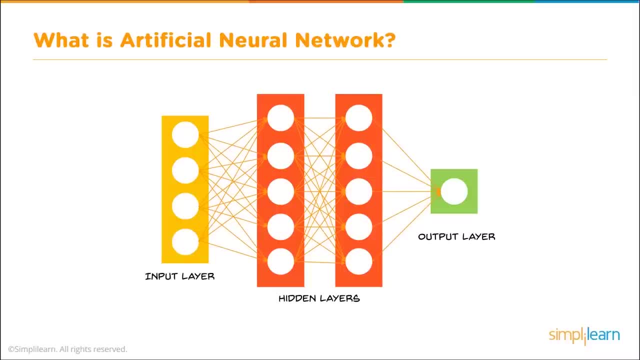 to your weights And they add all those up on the hidden layers And each one of those dots, kind of like a cell, does something with all the inputs And then it puts an output into the next hidden layer and so on into the output layer. So information processing happens here. Input to the. 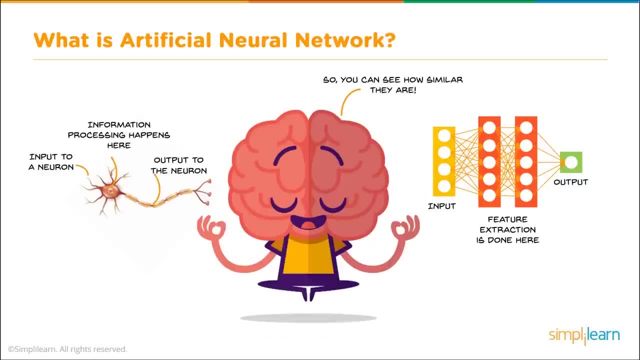 neuron output to the neuron So you can see how they are similar. We have an input, which is our yellow bar coming in, And then you liken each of the hidden layers to being a neuron And it passes it to the next one, and so on, And then you have an output to the next neuron or an output to the real 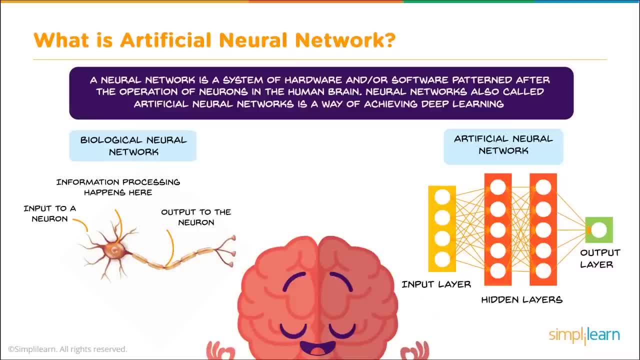 world. A neural network is a system of hardware and or software patterned after the operation of neurons in the human brain. Neural networks, also called artificial neural networks, is a way of achieving deep learning. How does artificial neural networks work? Let us find out. how does an artificial 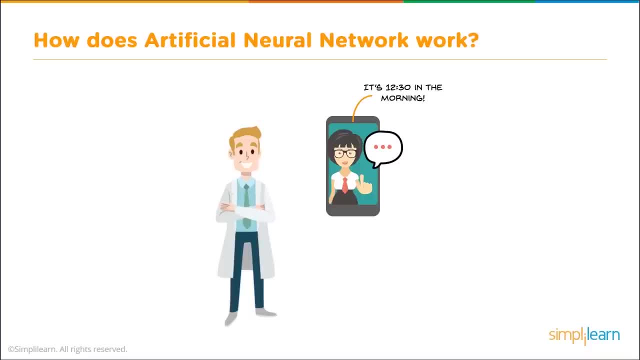 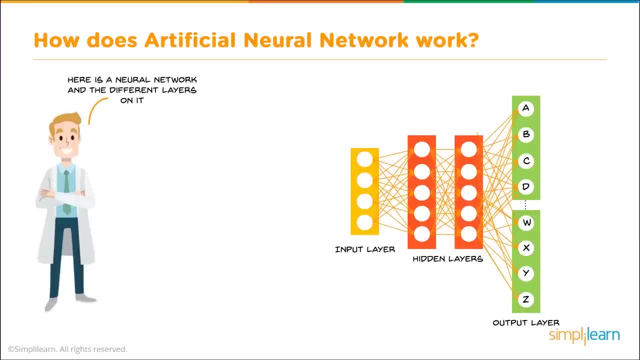 neural network work. Hey Siri, what is the time now? It's 1230 in the morning. Thanks, Let's find out how she recognizes speech. Here is a neural network and the different layers on it. So we have our input layer, our hidden layers, and the output layer. So we have our input layer, our 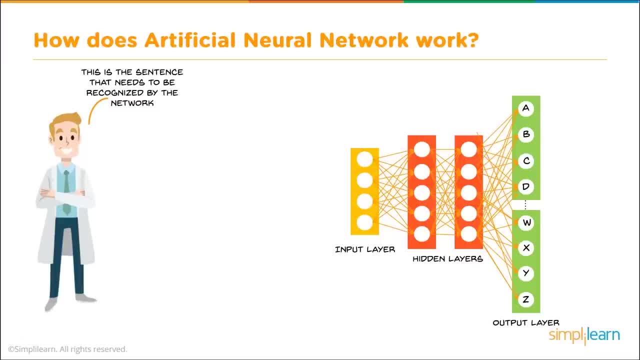 hidden layers and the output layer. So we have our input layer, our hidden layers and the output layer. This is the sentence that needs to be recognized by the network. What is the time? So, when it comes in, each one comes in as a pattern of sound. So what is the time? First, let's consider: 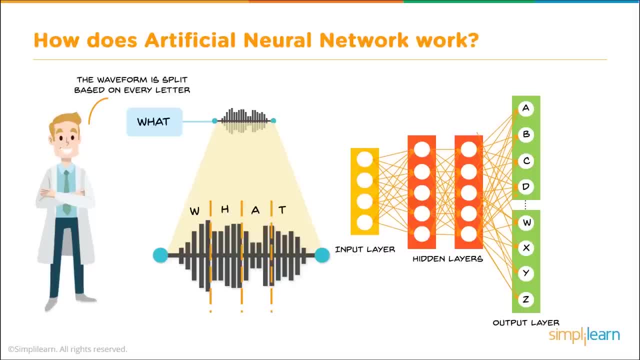 the word what And you have w-h-a-t And you can see each one of those in the sound bar Probably looks a little different than that. Just a representation Comes in as a different pattern. Now we will split the sound wave for the letter w into smaller segments. So we split off w and then we 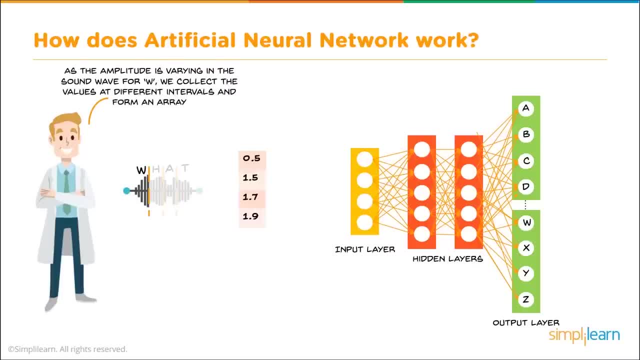 split the sound wave for w, As the amplitude is varying. in the sound wave for w, we collect the values at different intervals and form an array. So we have 0.5, 1.5, 1.7, 1.9.. That might be the. 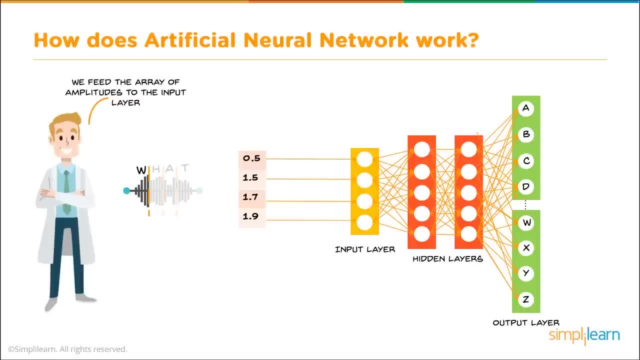 different amplitudes coming in And we feed the array of amplitudes to the input layer. So each one of those goes into its own box on the input layer. Random weights are assigned to each interconnection between input and hidden layer. So remember all those little lines. I said those. 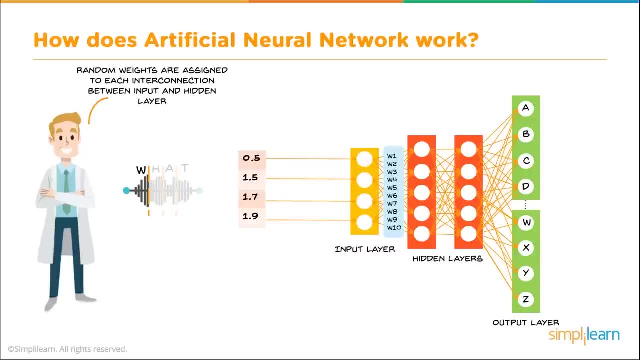 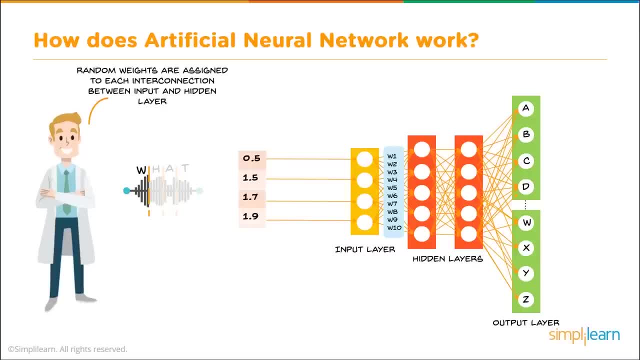 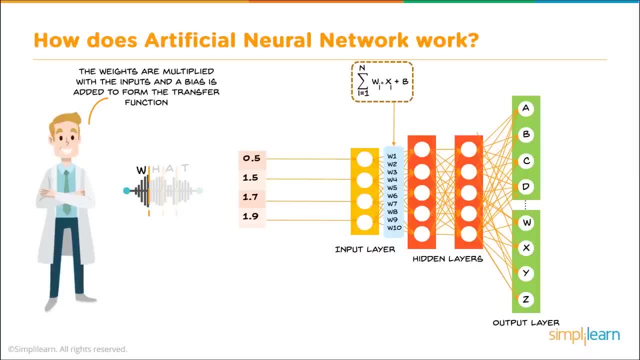 inputs and a bias is added to form the transfer function. So we make a sum of all the weights times a value. So you take .5, which is your x coming in, and we're going to multiply that by W1, W2, W3, so on, And then, when we get to the next level, we're going to add those together. 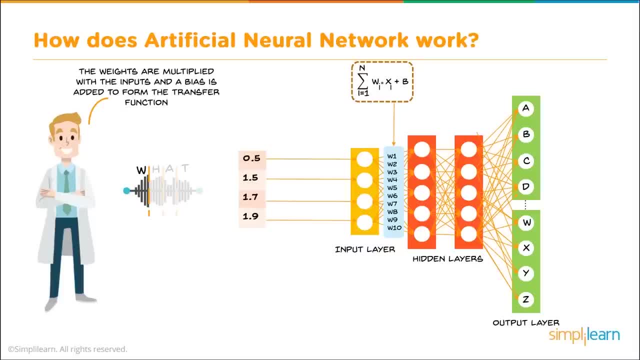 coming in, what's coming in, So we add the weight times x. There's always a bias added in. If you're, If you ever build your own neural network, don't forget to add the bias in, Otherwise it tends to not work quite as well. 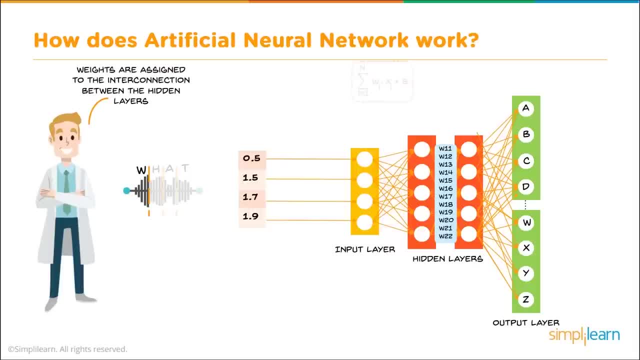 You need that extra layer in there to help it. Weights are assigned to the interconnection between the hidden layers. The output of the transfer function is fed as an input to the activation function. So the output from one hidden layer becomes the input to the next hidden layer. 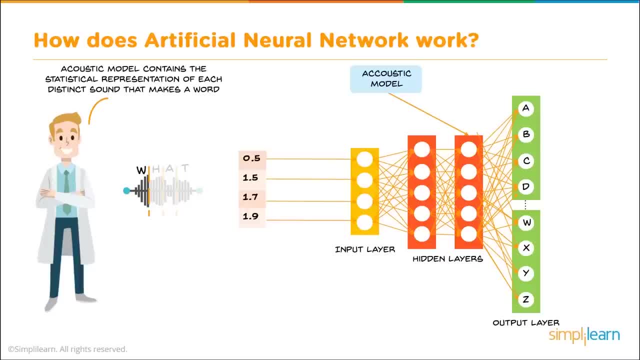 Acoustic model contains the statistical representation of each distinct sound that makes a word. As we start building these acoustical models and as these layers separate them out, they'll start learning what the different models are for the different letters. Lexicon contains the data for different pronunciations of every word. 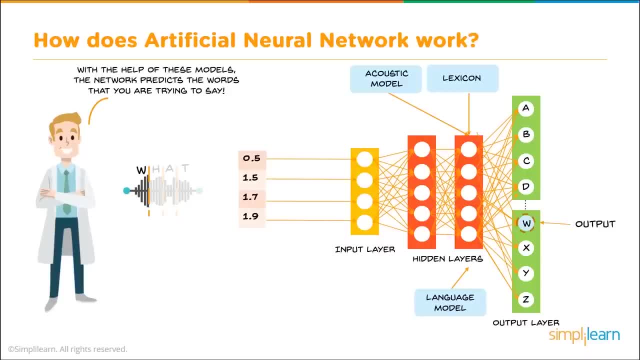 So we have the lexicon at the end, where we end up with the A, B, C, D, and it identifies the different letters in there. Now, the term acoustic model and the term lexicon are specific to this domain, the domain of 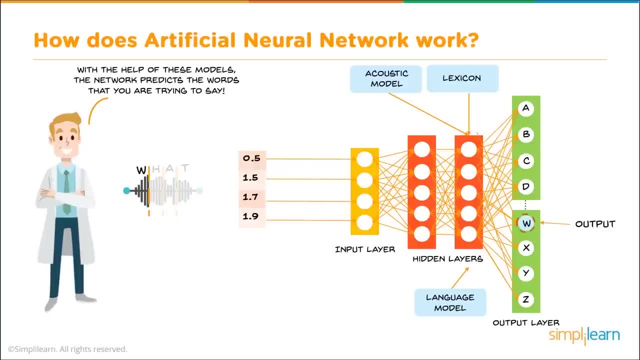 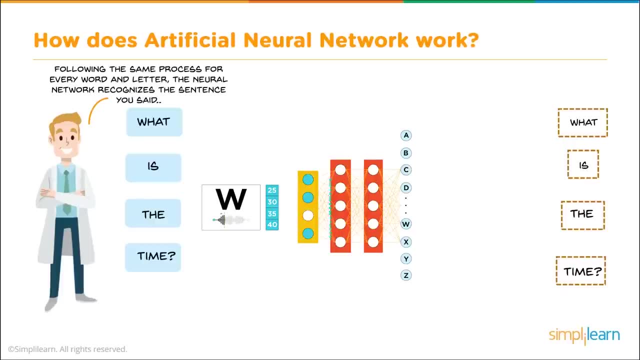 understanding speech. Certainly, when you're doing photographs and other things, you'll have different labels on here, But the process is going to be the same And finally we get our output layer. Following the same process For every word and letter, the neural network recognizes the sentence you said. 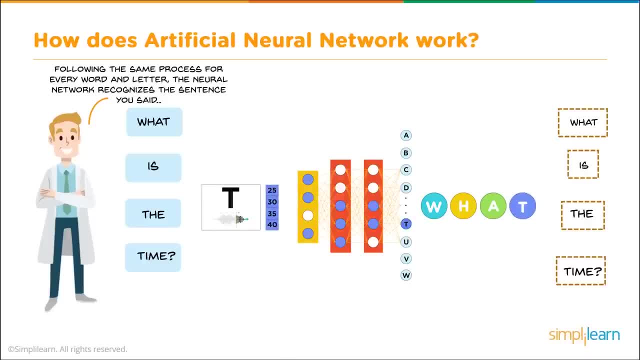 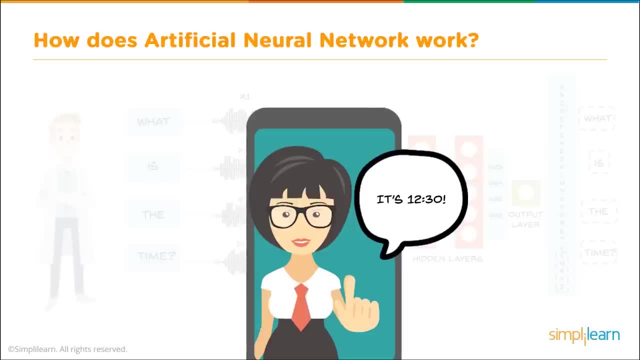 What is the time? So it identifies the W, H, A, T and then identifies that that's one word. What is the time? And so on. It's 1230.. That way, Siri can look up the time and read it back to you. 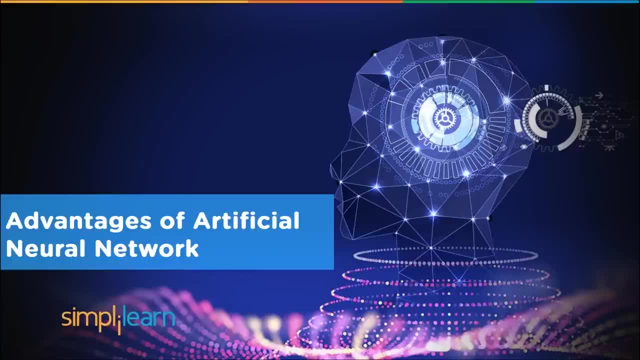 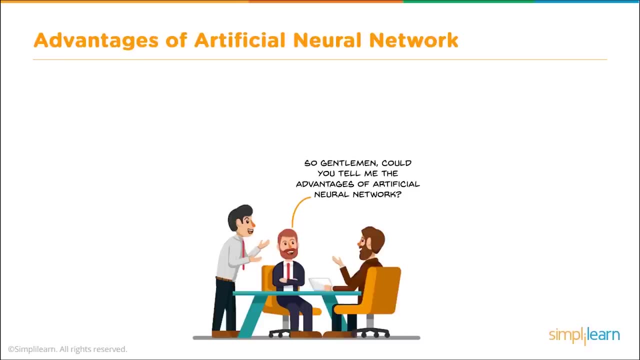 So let's look at the advantages of an artificial neural network. So, gentlemen, could you tell me the advantages of an artificial neural network? It's amazing how many times I've been in that situation where I have to explain to the people making the decisions in the company. it's amazing how many times I've been in that space. 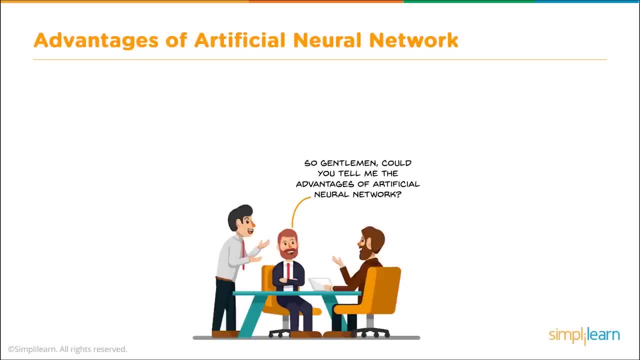 where I have to explain to the owner of the company what the artificial intelligence and the neural network actually do, What are the advantages of an artificial neural network and what it can do for them and how it works. So an artificial neural network outputs aren't limited entirely by inputs and results given. 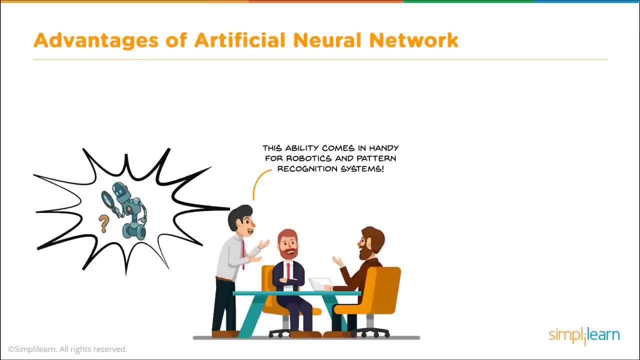 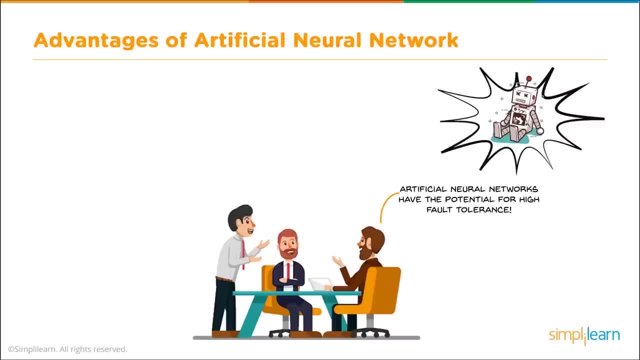 to them, initially by an expert system. This ability comes in handy for robotics and pattern recognition systems. Artificial neural networks have the potential for high-tech, high-tech, high-tech, high-tech, high-tech, High fault tolerance. Artificial neural networks are capable of debugging or diagnosing a network on their 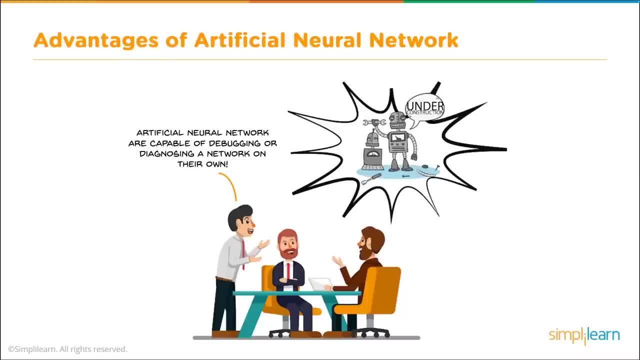 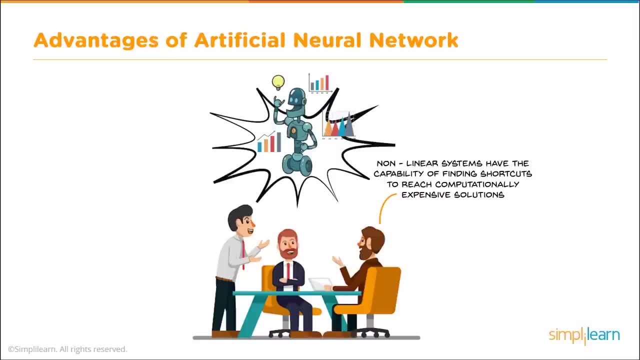 own. Very common use these days is to go through all the log files and sort them out- thousands of log files if you're working as an admin. Nonlinear systems have the capability of finding shortcuts to reach computational expensive solutions. So we see this in banking, where by hand they have an Excel spreadsheet and then they start. 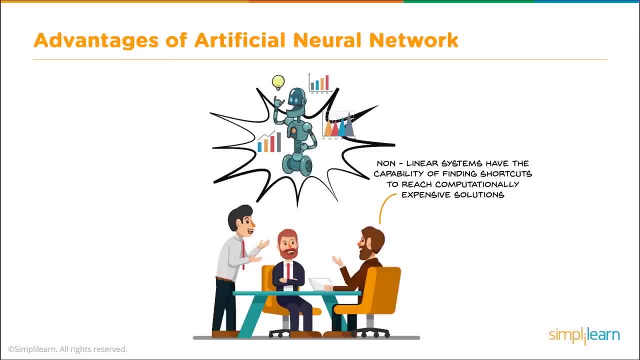 building codes around that Excel spreadsheet and over 20 years they might build a repertoire of all these functions. So an artificial neural network comes up with the same answers done in days, weeks or even a month for a huge bank. So let's take a look a little bit more, because I mentioned a couple applications of artificial 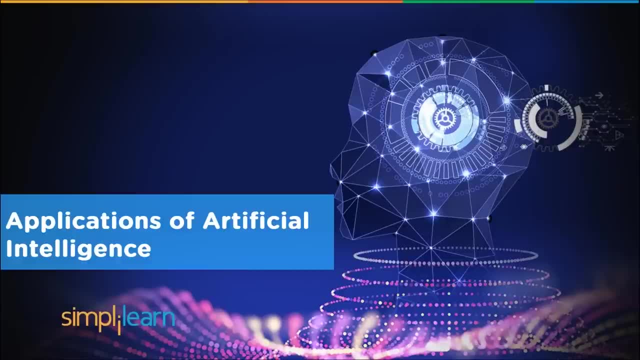 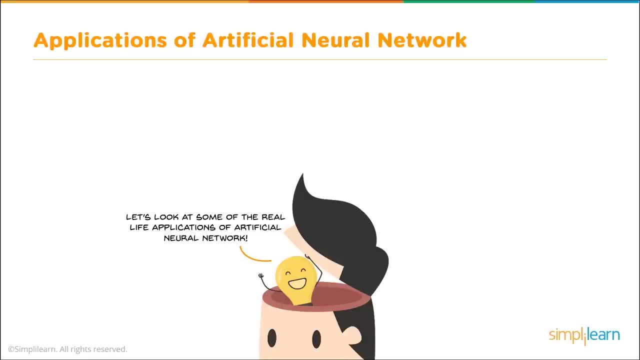 intelligence there. but let's dig deeper into the applications of artificial intelligence. Let's look at some of the real life. This is stuff going on right now in our world and we're in such an exciting time with the neural networks and the machine learning and the artificial intelligence development. 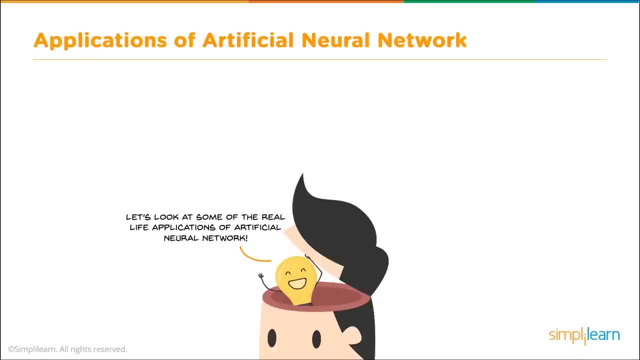 So let's take a little look at some of the current applications going on in real life And you can use your imagination, You can use your imagination to dig for some new ones that we don't have listed here because it's so limitless the amount of applications that are being worked on right now or being 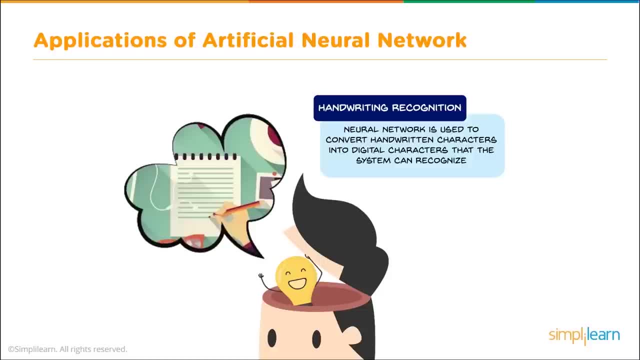 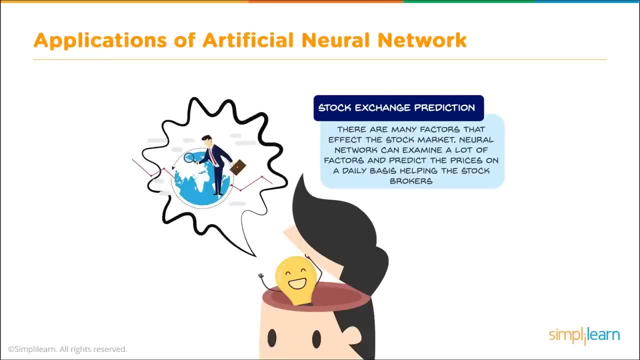 implemented Handwriting recognition Neural network is used to convert handwritten characters into digital characters that the system can recognize. Stock exchange prediction. If you've ever worked with stock exchange, which I have, it is so fickled to track. I mean it is really hard to understand. 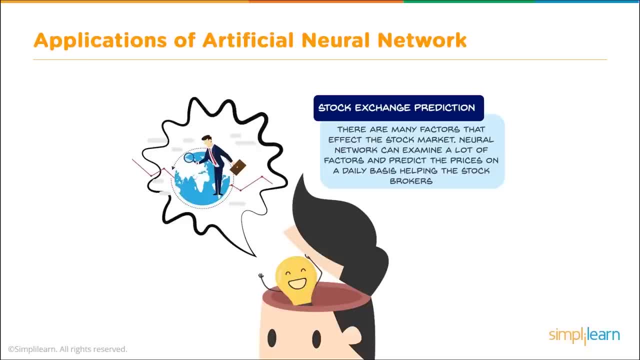 There are many factors that affect the stock market. Neural network can examine a lot of factors And predict the prices on a daily basis, helping the stock brokers. So right now it's still at the intro phase where it helps them and they really have to. 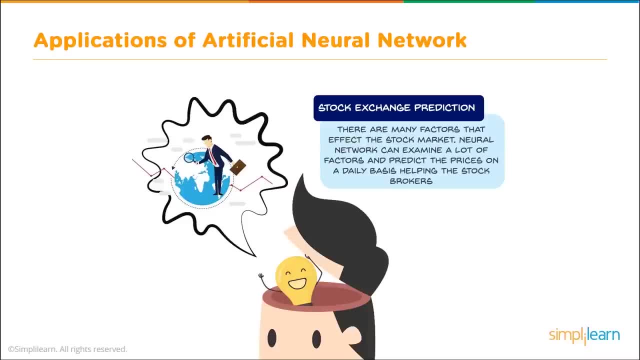 look closely at it When you realize that we generate over three terabytes a day just from the stock exchange here in the United States. that's a lot of data to dig through and you have to sort it out before you even start focusing on even one stock. 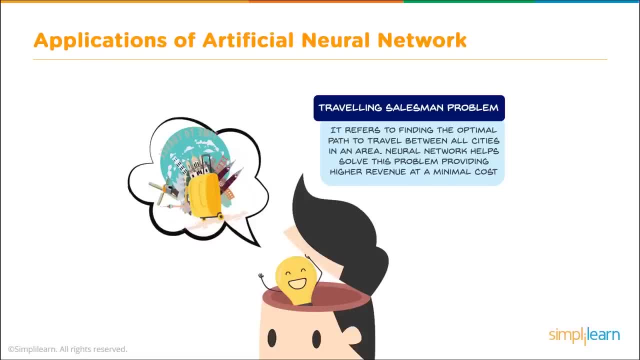 Traveling salesman problem. It refers to finding the optimal path to travel between all cities in an area. Neural network helps solve the problem, Providing higher revenue at a minimal cost. Logistics is huge, Just the logistics that we talk about: salesman traveling from town to town. 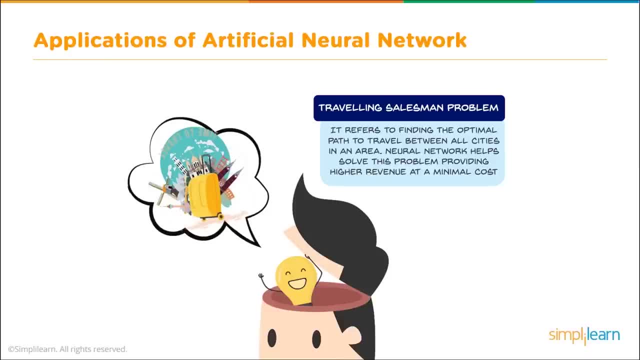 Logistics are used by Amazon. Amazon loves to ship their packages and they have empty space on their trucks, So they'll pre-ship packages and fill that empty space on who they think will buy it Saves them a lot of time and people are a lot happier because they get that tomorrow. 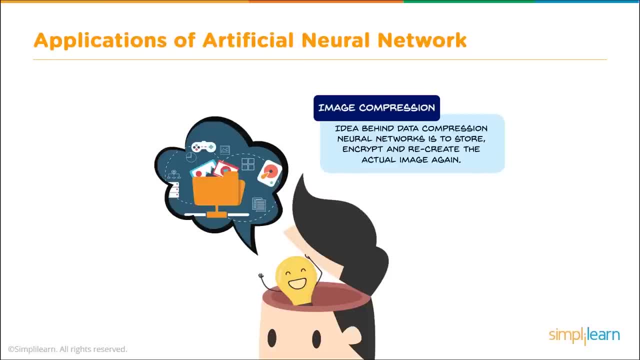 instead of having to wait three weeks. Image compression: The idea behind data compression in neural network is to store, encrypt and recreate an actual image again So we can optimize our compression. and data Images are the biggest one, but it's used in all kinds of data. 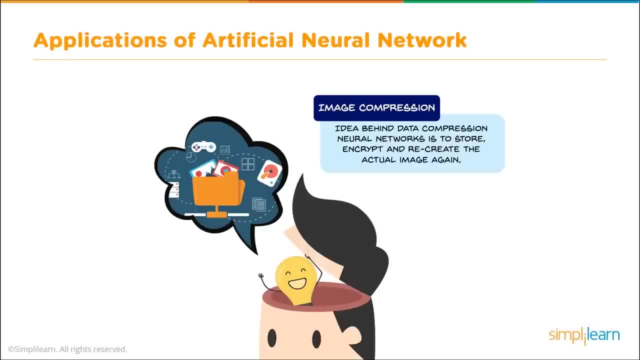 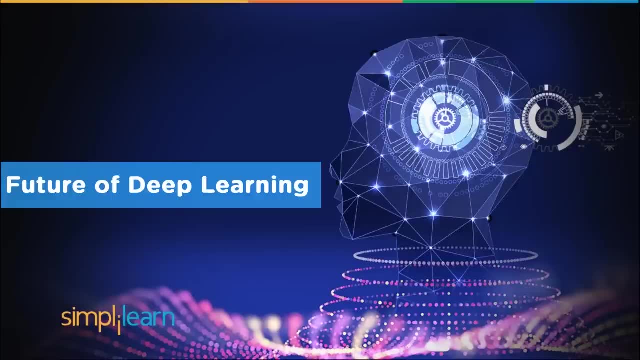 Wonderful application to save a hard drive and to optimize being able to read it back out again. Those are just a few and, like I said, use your mind to dig deeper and let's take it even further. We're going to go a step further here and let's look at the future of deep learning. 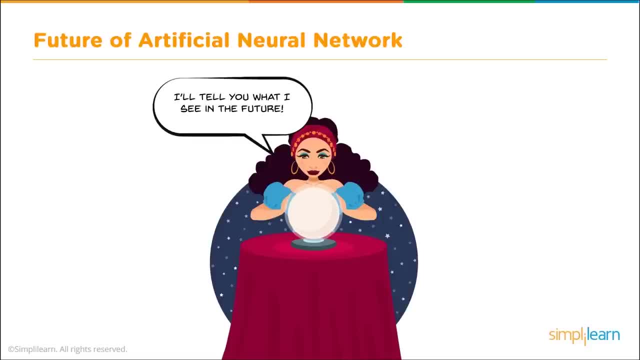 Here we are. That's not me, Thank goodness. Wonderful person there reading her crystal ball. I'll tell you what I see in the future: More personalized choices for users and customers all over the world. I certainly like that When I go in there and whatever online ordering system starts referring stuff to me local. 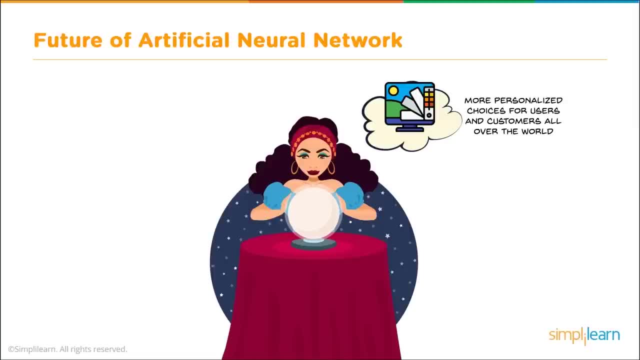 company here where I live that uses this, where you can take a picture, and it starts looking for what you want based on your picture. So if you see a couch you like, it starts looking for furniture like that or clothing- I think it's mainly clothing. 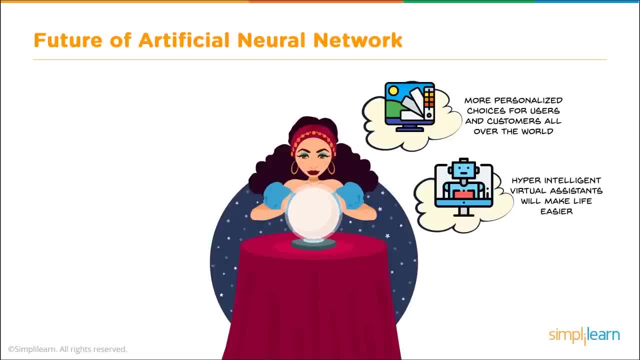 Hyper intelligent virtual assistants will make life easier. If you played with Google Assistant or Siri or any of those, you can see how they're slowly evolving, and they're just now getting over that hump where a virtual assistant can do all kinds of things. 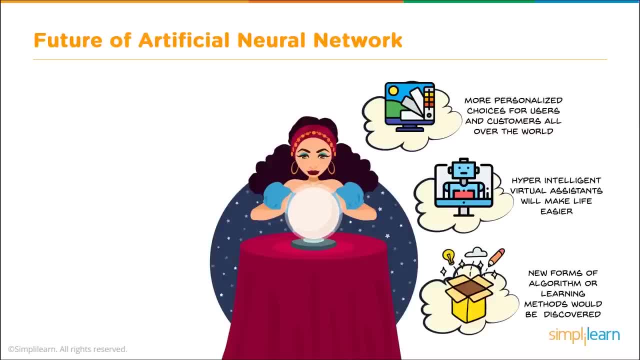 Even pre-write your email response for you, New forms of algorithm for learning methods would be discovered. There's always something rolling out, and they've had some really cool research in this area. Again, this stuff is such a we're just in the infant stage of artificial intelligence. 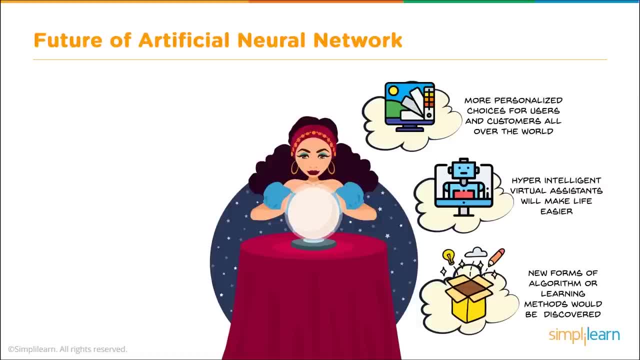 and neural networks and actually applying them to the real world. Wonderful time to jump in Neural networks will be a lot faster in the future. Neural network tools will be embedded in every design surface. We already see that. that you can buy a little mini neural network that plugs into a real 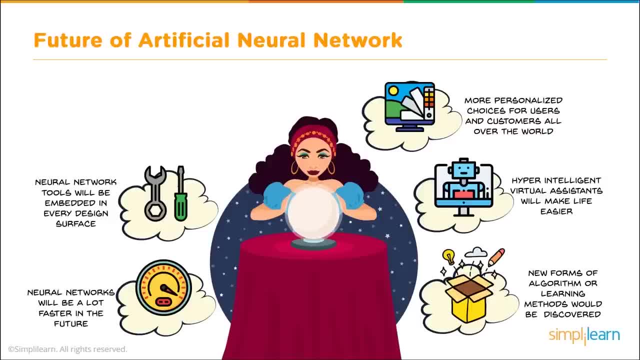 into a really cheap processing board or into your laptop. So the hardware is starting to come out that goes right in there where you can dump it on there, and that makes it all so faster. So because it's on the hardware instead of the software side. 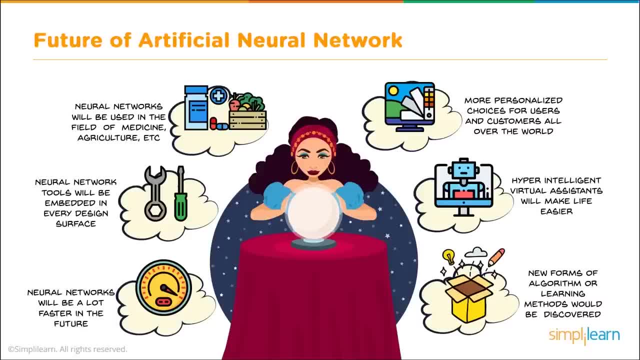 Neural networks will be used in the field of medicine, agriculture, physics, discoveries, just everything you can imagine. We see this today, where it's going from a PhD student in medicine trying to understand T cells and understand the statistic analysis of that to cure people. 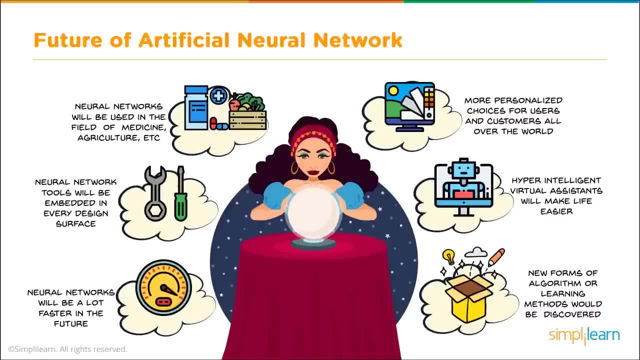 To help keep them healthy, to help find out how we heal, to something that anybody can go, access and process the data on. They're working on shared data systems. This concept of it being used in these different fields and these different domains is huge. 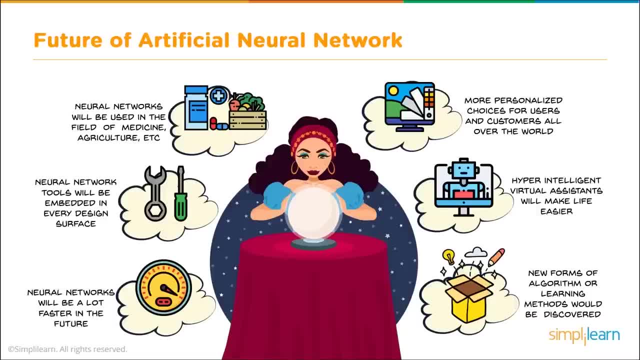 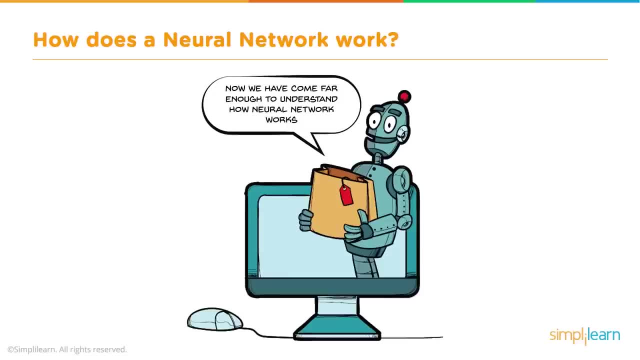 The world's wide open for anybody jumping out there to start exploring them and start learning neural networks. Let's dive in and say: how does a neural network work? So now we've come far enough to understand how neural network works. let's go ahead and 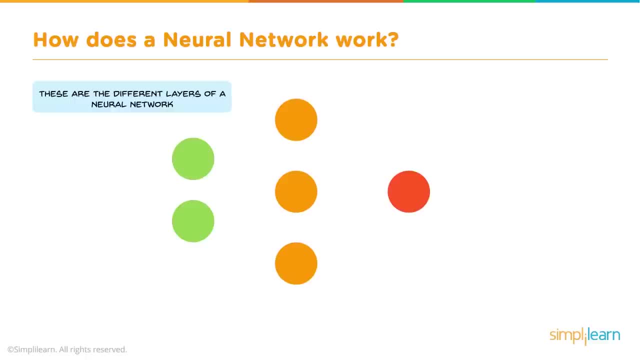 walk through this. They're nice graphical representations. They usually describe a neural network as having different layers. You'll see that we've identified a green layer, an orange layer and a red layer. The green layer is the input, so you have your data coming in. 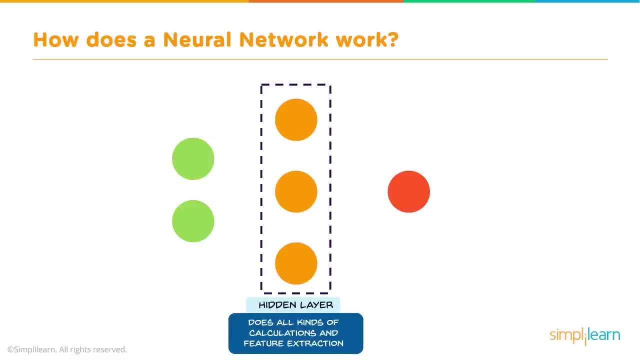 It picks up the input signals and passes them to the next layer. The next layer does all kinds of calculations and feature extraction. it's called the hidden layer. A lot of times there's more than one hidden layer. We're only showing one in this picture, but we'll show you how it looks like in more detail. 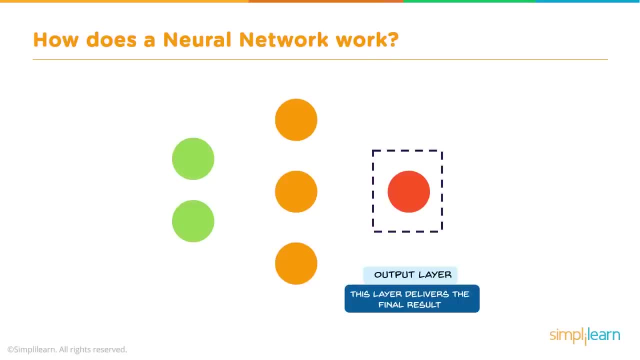 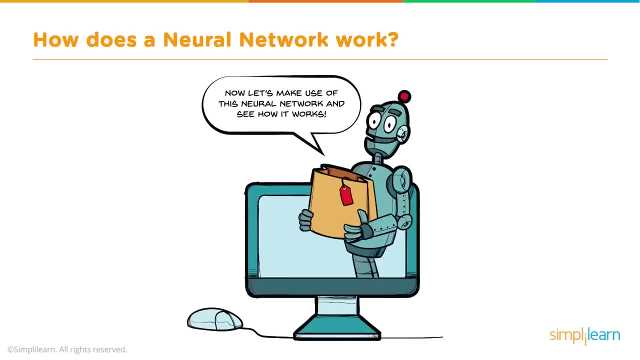 in a little bit. And then, finally, we have an output layer. This layer delivers the final result. So the only two things we see is the input layer and the output layer. Now let's make use of this neural network and see how it works. 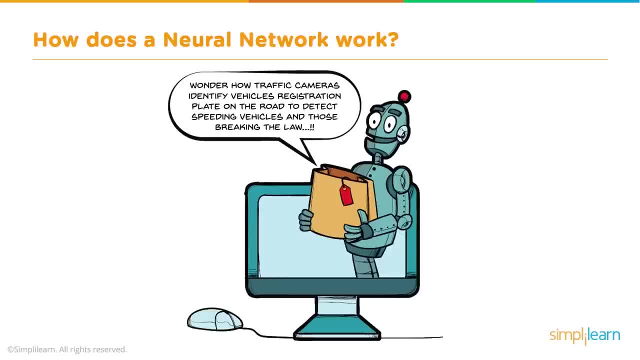 Wonder how traffic cameras identify vehicles' registration plate on the road to detect speeding vehicles and those breaking the law. They got me going through a red light the other day, Well, last month. That's like the horrible thing. They send you this picture of you and all your information because they pulled it up. 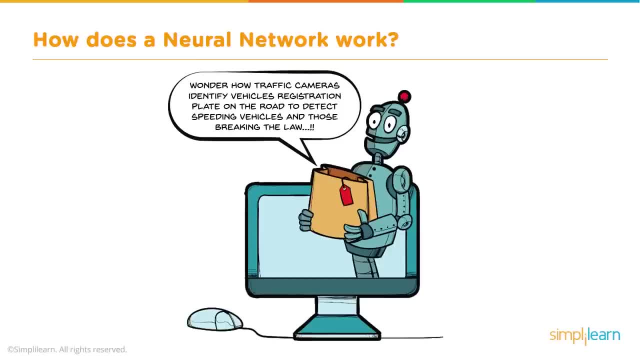 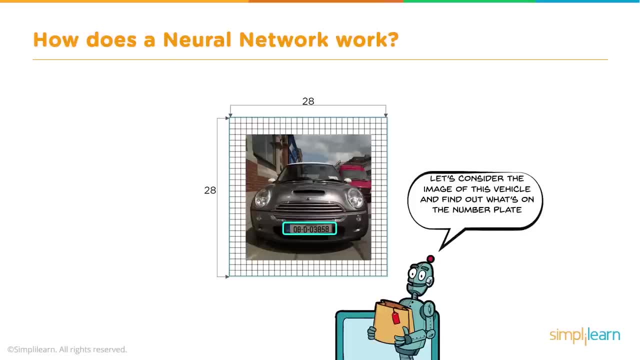 off of your license plate and your picture. I shouldn't have gone through the red light. So here we are and we have an image of a car and you can see the license plate's on there. So let's consider the image of this vehicle and find out what's on the number plate. 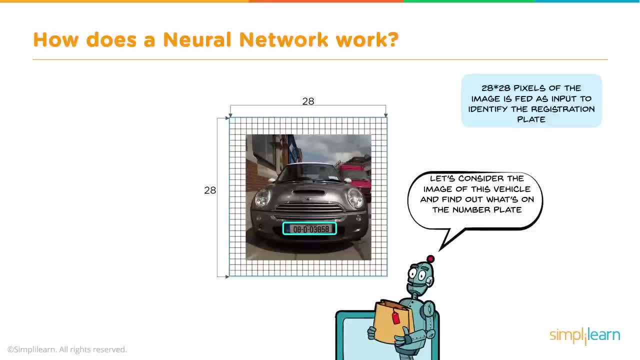 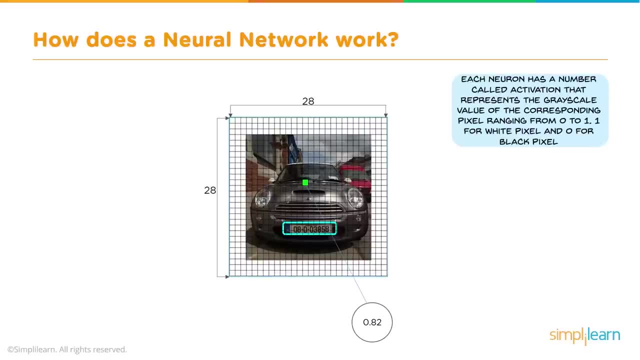 The picture itself is 28 by 28 pixels and the image is fed as an input to identify the registration plate. Each neuron has a number called activation that represents the grayscale value of the corresponding pixel range, And we range it from zero to one. 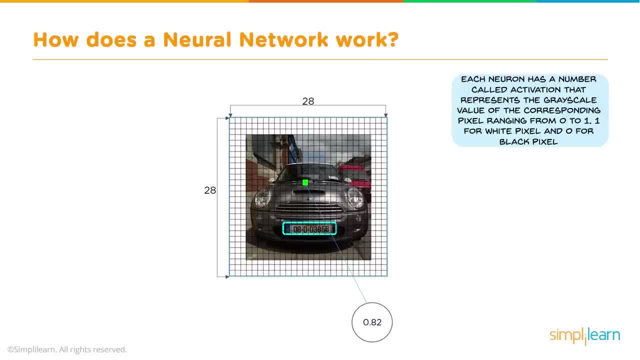 One for a white pixel and zero for a black pixel, And you can see down here. We have an example where one of the pixels is registered as like .82, meaning it's probably pretty dark. Each neuron is lit up when its activation is close to one. 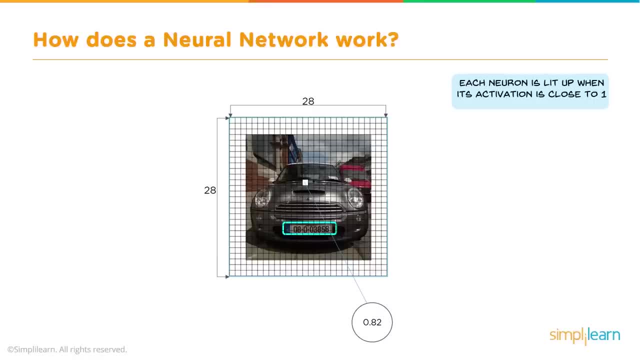 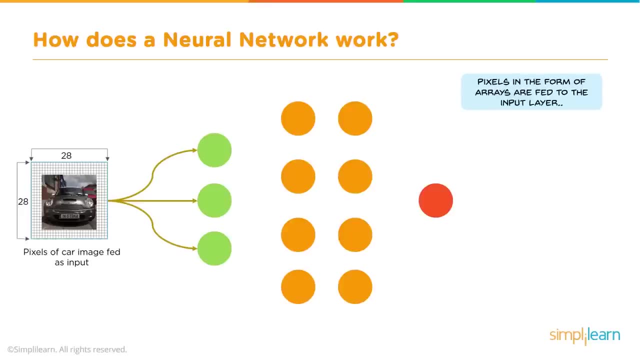 So as we get closer to black on white, we can really start seeing the details in there And you can see again. the pixel shows us one up there. It's like part of the car And so it lights up. So pixels in the form of arrays are fed to the input layer. 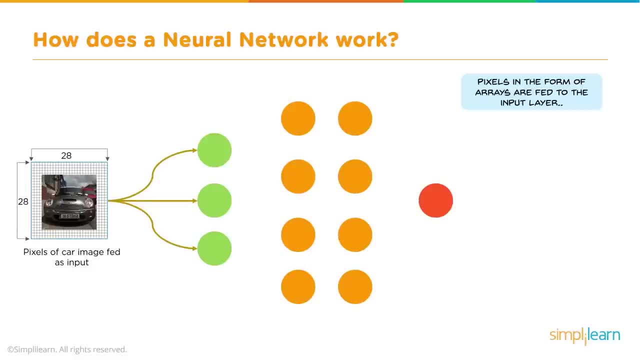 And so we see here the pixel of a car image fed as an input, And you're going to see that the input layer, which is green, is one dimension, while our image is two dimension. Now, when we look at our setup that we're programming in Python, it has a cool feature. 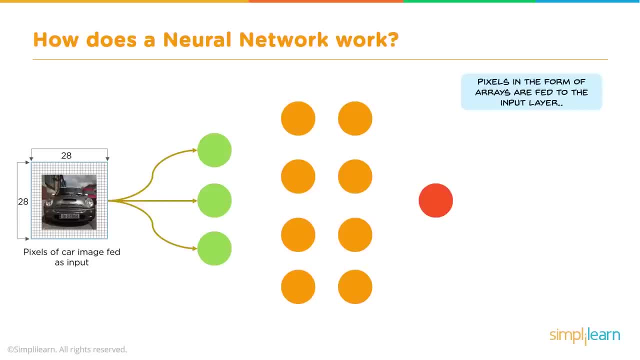 that automatically does the work for us. If you're working with an older neural network pattern package, you then convert each one of those rows so it's all one array. So you'd have like row one and then just tack row two onto the end. 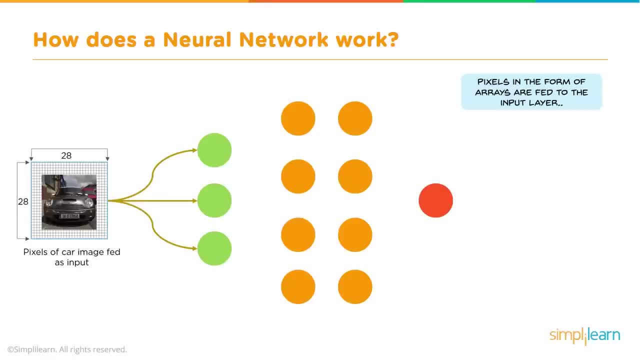 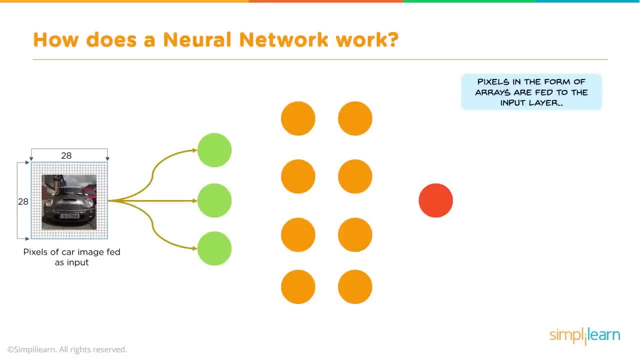 So you can't increase the number of input, in this case green dots. It's very important to remember when you work on neural networks. And let's name the inputs x1,, x2, x3, respectively, So each one of those represents one of the pixels coming in. 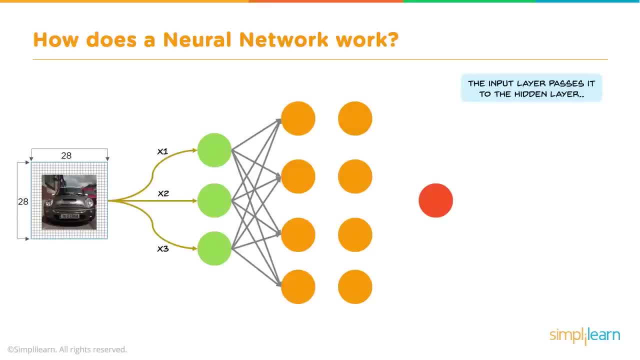 And the input layer passes it to the hidden layer. And you can see here we now have two hidden layers in this image, in the orange, And each one of those pixels connects to each one of those hidden layers And the interconnections are assigned weights at random. 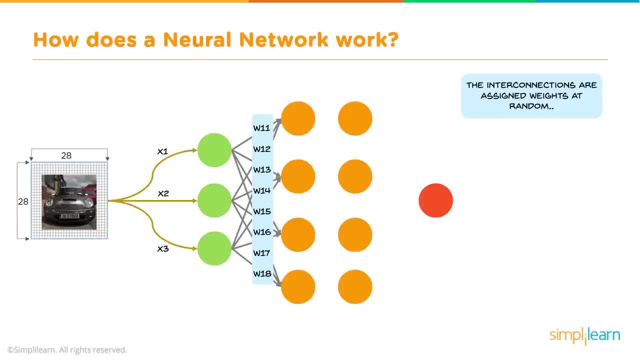 So it gets these random weights that come through that if x1 lights up, then it's going to be x1 times this weight going into the hidden layer And we sum those weights, The weights are multiplied with the input signal And a bias is added to all of them. 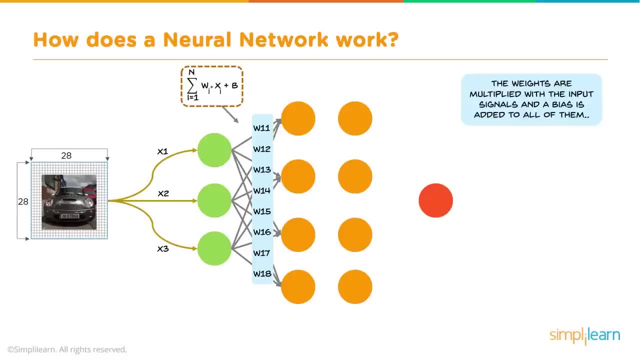 So, as you can see, here we have, x1 comes in And it actually goes to all the different hidden layer nodes, or, in this case, whatever you want to call them, network setup, the orange dots- And so you take the value of x1.. 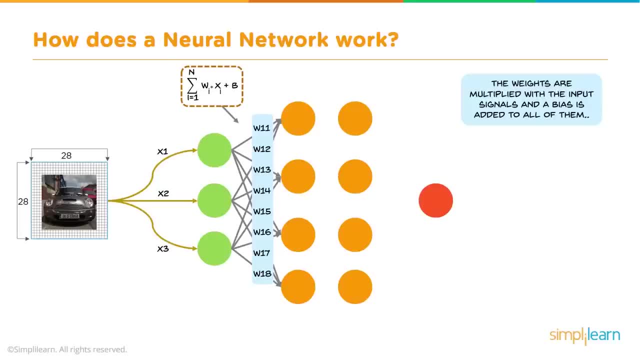 You multiply it by the weight for the next hidden layer. So x1 goes to hidden layer 1.. x1 goes to hidden layer 2.. x1 goes to hidden layer 3.. x1 goes to hidden layer 1, node 2, hidden layer 1, node 3, and so on. 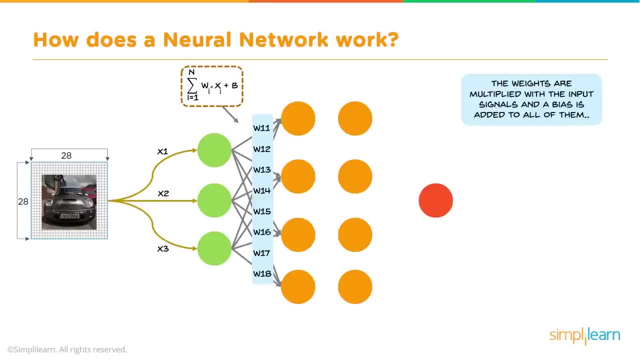 And the bias. a lot of times they just put the bias in as like another green dot or another orange dot And they give the bias a value 1.. And then all the weights go in from the bias into the next node, So the bias can change. 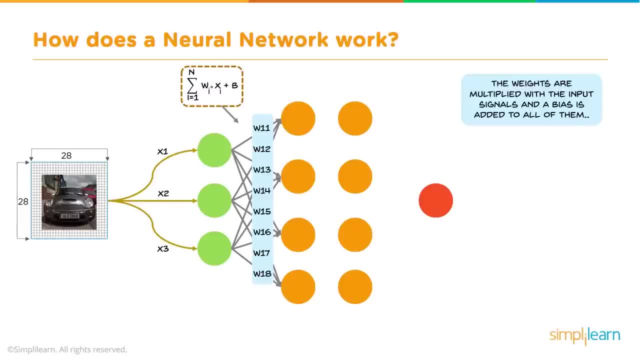 We always just remember that you need to have that bias in there. There's things that can be done with it. Generally, most of the packages out there control that for you, So you don't have to worry about figuring out what the bias is. 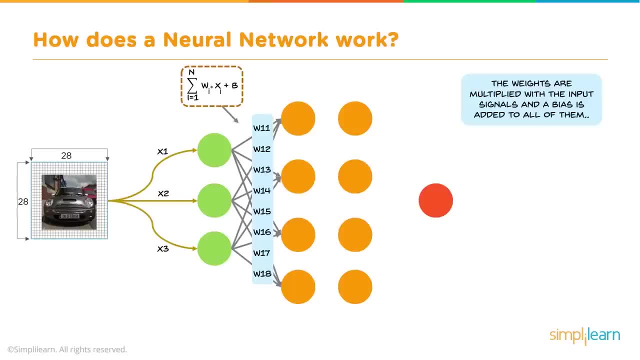 But if you ever dive deep into neural networks you've got to remember there's a bias or the answer won't come out correctly. The weighted sum of the input is fed as an input to the activation function to decide which nodes to fire and for feature extraction. 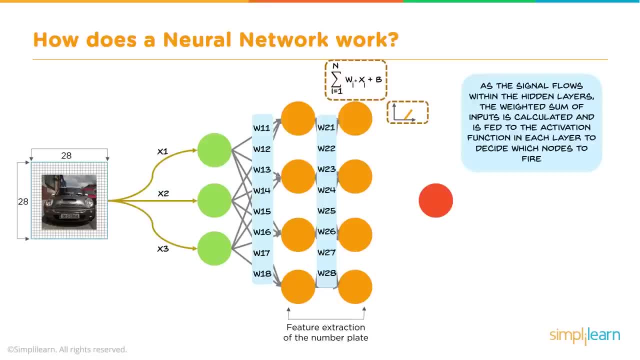 As a signal flows within the hidden layers, the weighted sum of inputs is calculated and is fed to the activation function in each layer to decide which nodes to fire. So here's our feature: extraction of the number plate And you can see these are still hidden nodes in the middle. 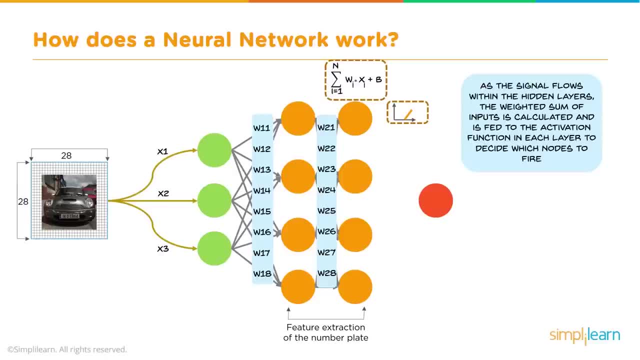 And this becomes important. We're going to take a little detour here and look at the activation. So we're going to dive just a little bit into the math So you can start to understand where some of the games go on when you're playing with neural networks in your programming. 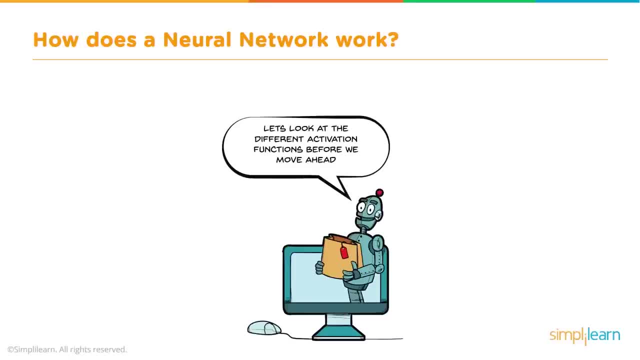 So let's look at the different activation functions before we move ahead. Here's our friendly red tag shopping robot. And so one is a sigmoid function, And the sigmoid function, which is 1 over 1, plus e to the minus x, takes the x value. 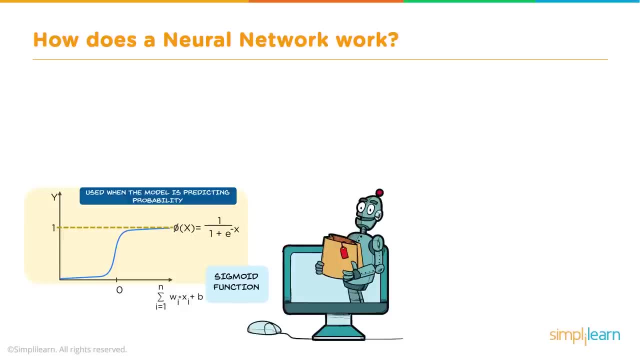 And you can see where it generates almost a 0 and almost a 1, with a very small area in the middle where it crosses over, And we can use that value to feed into another function. So if it's really uncertain, it might have a 0.1 or 0.2 or 0.3. 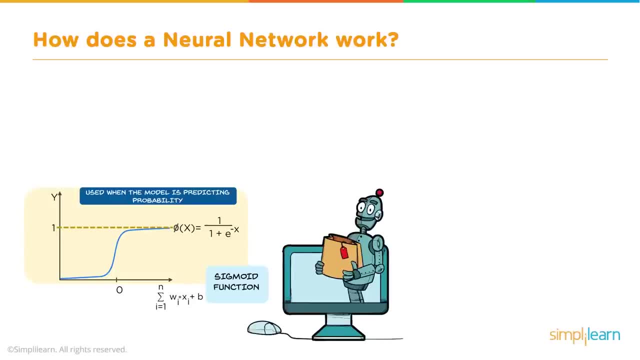 But for the most part it's going to be really close to 1 and really close to, in this case, 0, 0 to 1.. The threshold function. So if you don't want to worry about the uncertainty in the middle, you just say: oh, if x is greater than or equal. 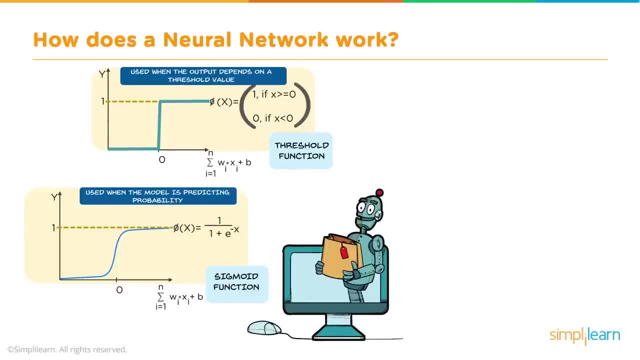 to 0, if not, then x is 0. So it's either 0 or 1.. Really straightforward. There's no in between in the middle. And then you have what they call the RELU function, And you can see here where it puts out the value. 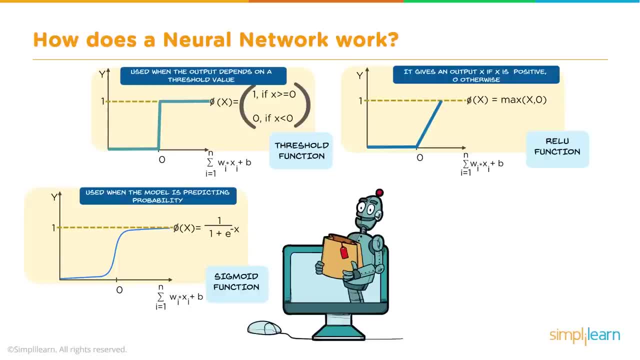 But then it says, well, if it's over 1, it's going to be 1., And if it's less than 0, it's 0. So it kind of just dead ends it on those two ends, but allows all the values in the middle. 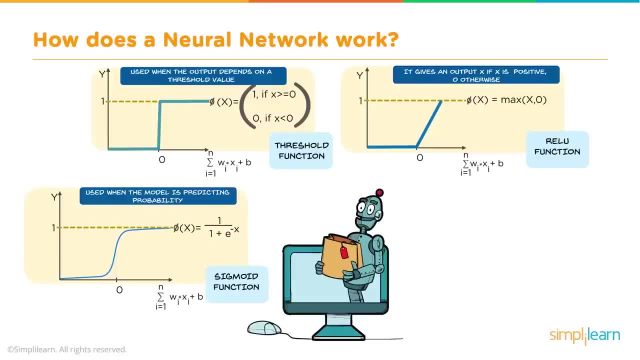 And again, this, like the sigmoid function, allows that information to go to the next level. So it might be important to know if it's a 0.1 or a minus 0.1.. The next hidden layer might pick that up and say: 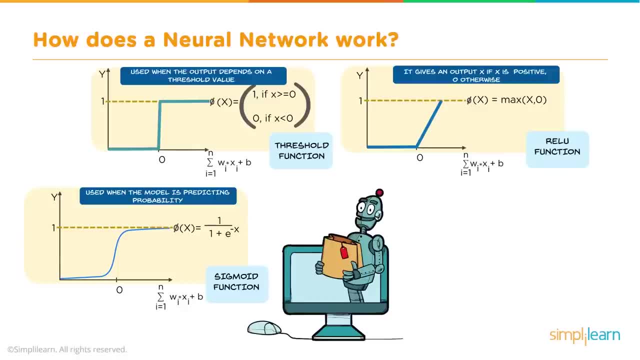 oh, this piece of information is uncertain, Or this value has a very low certainty to it. And then the hyperbolic, The tangent function, And you can see here it's 1 minus e to the minus 2x over 1. 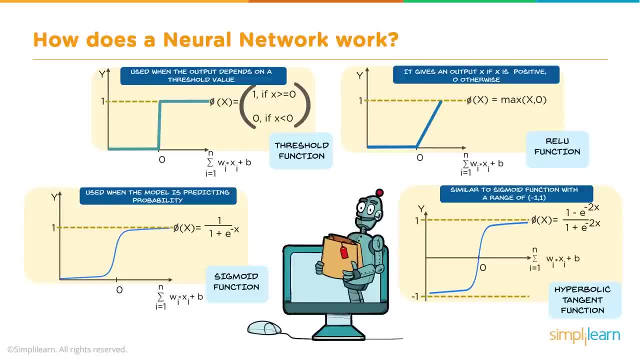 plus e to the minus 2x And it's very much along the same theme, A little bit different in here in that it goes between minus 1 and 1.. So you'll see some of these. they go 0 to 1.. 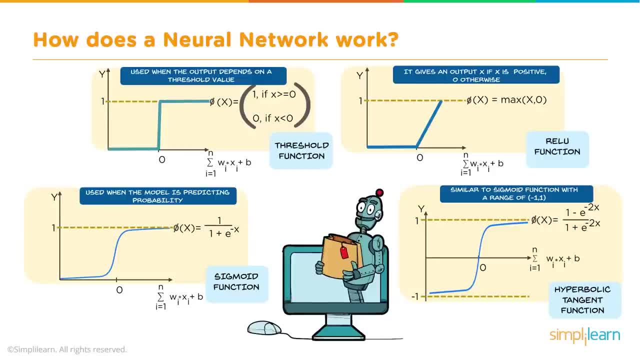 But this one goes minus 1 to 1. And if it's less than 0, it doesn't fire, And if it's over 0, it fires And it also still puts out a value. So you still have a value you can get off of that. 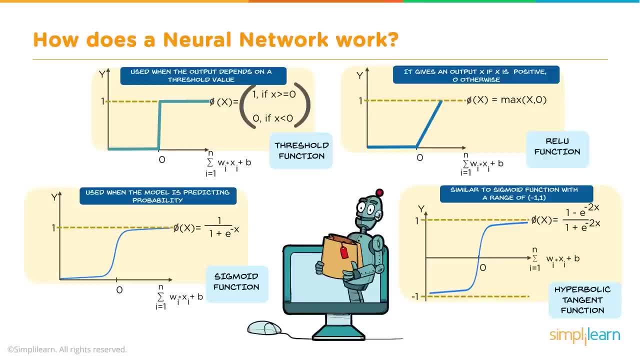 just like you can, with the sigmoid function and the RELU function. Very similar in use And I believe they originally used to be. everything was done in the sigmoid function That was the most commonly used And now they just kind of use more the RELU function. 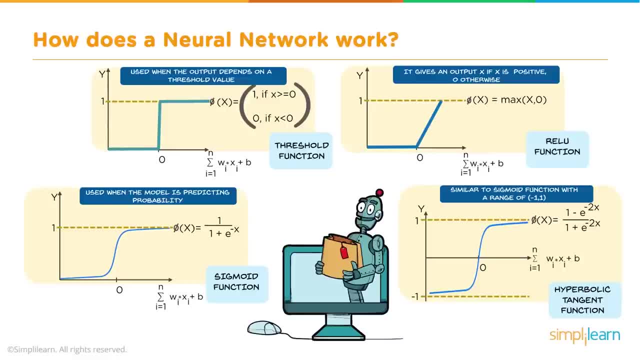 The reason is one: it processes faster Because you already have the value And you don't have to add another, compute the 1 over 1, plus e to the minus x for each hidden node, And the data coming off works pretty good. 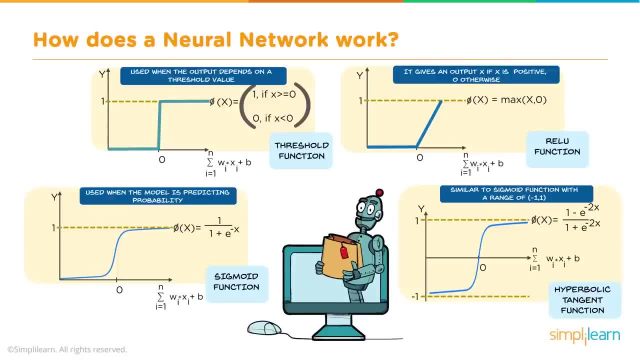 as far as putting it into the next level, if you want to know just how close it is to 0.. How close is it not to functioning? Is it minus 0.1, minus 0.2?? Usually they're float values. 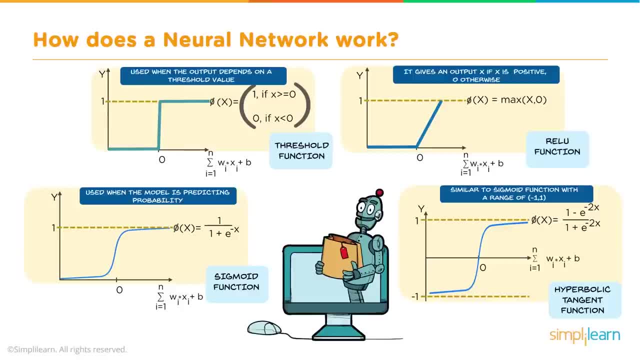 So you get like minus 0.00138 or something So important information. But the RELU is most commonly used these days as far as the setup we're using, But you'll also see the sigmoid function very commonly used also, Now that you know what an activation function is. 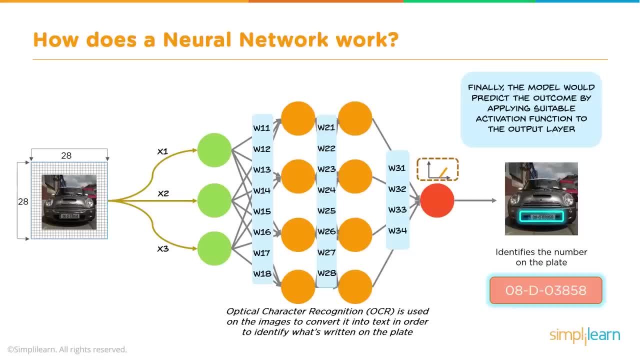 let's get back to the neural network. So, finally, the model would predict the outcome of applying a suitable activation function to the output layer. So we go in here, we look at this and we have the optical character recognition. OCR is used on the images to convert it into a text. 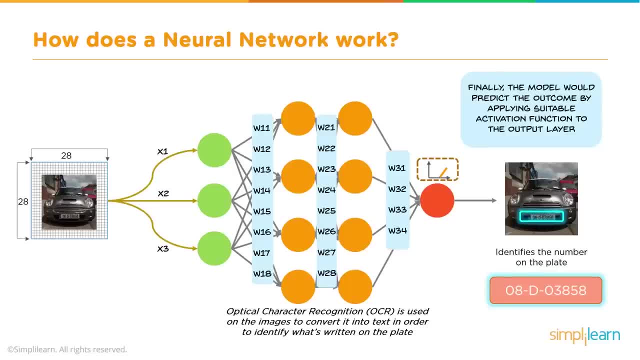 in order to identify what's written on the plate, And as it comes out, you'll see the red node, And the red node might actually represent just the letter A, So there's usually a lot of outputs when you're doing text identification. 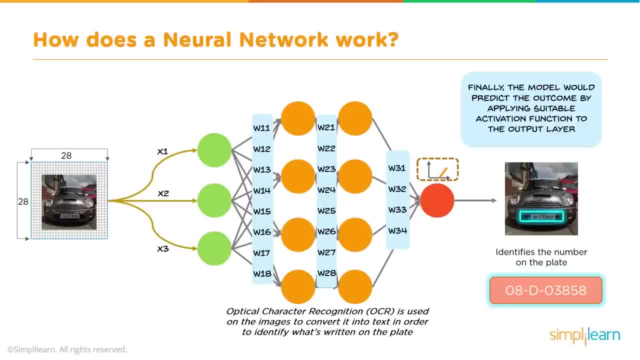 We're not going to show that on here, But you might have it even in the order. It might be what order the license plate's in. So you might have A, B, C, D, E, F, G. you know the alphabet plus the numbers. 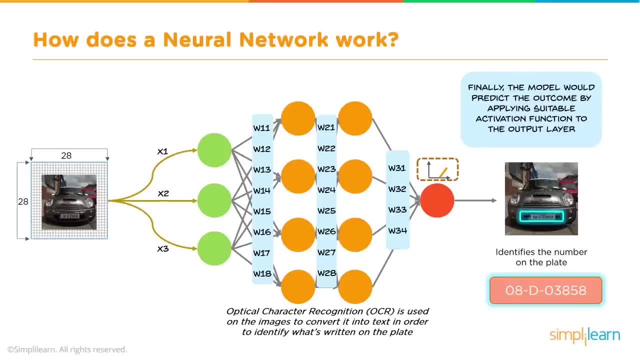 And you might have the 1,, 2,, 3,, 4,, 5,, 6,, 7,, 8,, 9,, 10 places. So it's a very large array that comes out. It's not a small amount. 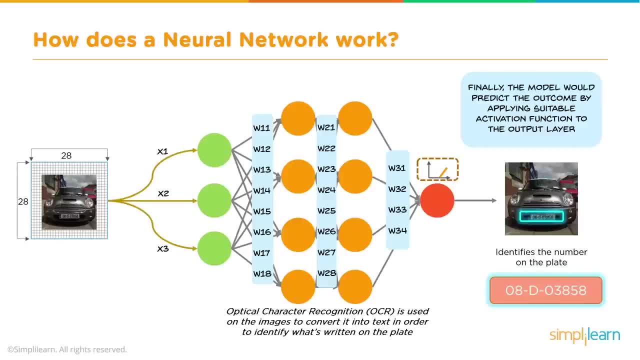 You know we show three dots coming in, eight hidden layer nodes. you know two sets of four. We just saw one red coming out. A lot of times this is, you know, 28 times 28.. If you did 30 times 30, that's 900 nodes. 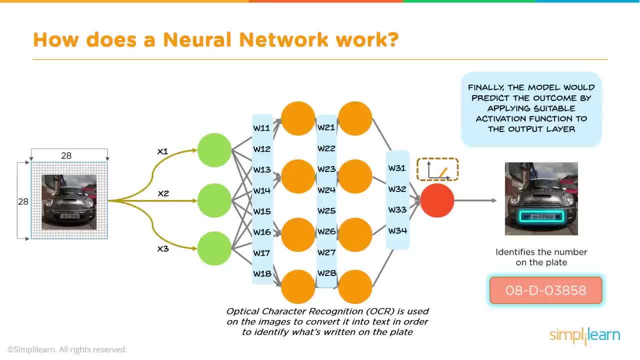 So 28 is a little bit less than that, just on the input, And so you can imagine. the hidden layer is just as big, Each hidden layer is just as big, if not bigger, And the output is going to be. there's so many digits. 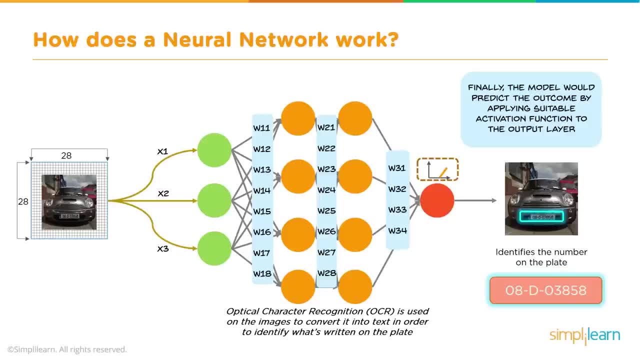 You know it's a huge amount of input and output, But we're only showing you just. you know it would be hard to show in one picture, And so it comes up and this is what it finally gets out on the output is it identifies a number on the plate. 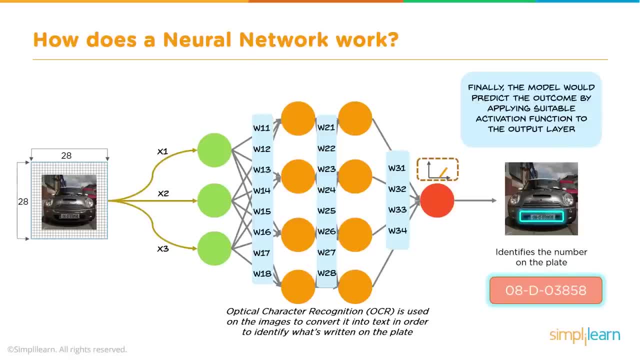 And in this case we have 08-D-03858.. Error in the output is back propagated through the network And weights are adjusted to minimize the error rate. This is calculated by a cost function. When we're training our data, this is what's used. 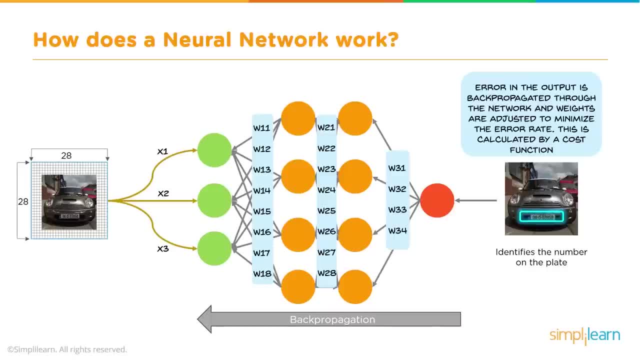 And we'll look at that in the code when we do the data training. So we have stuff we know the answer to And then we put the information through and it says yes, that was correct or no, Because, remember, we randomly set all the weights to begin with. 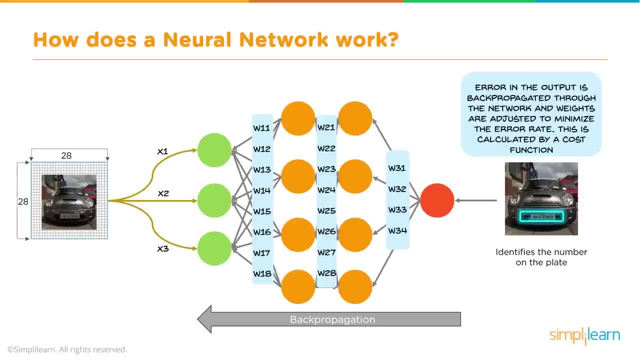 And if it's wrong, we take that error. How far off are you? You know? are you off by? is it? if it was like minus 1, you're just a little bit off. If it's like minus 300 was your output. 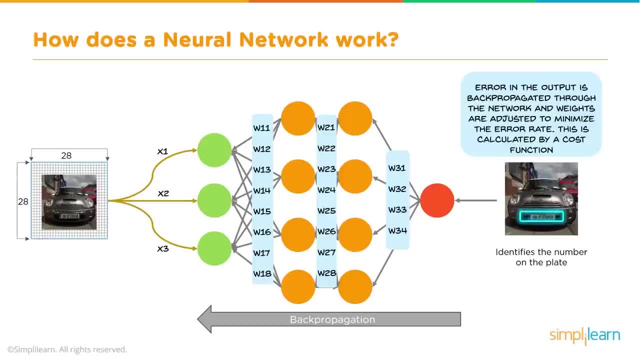 remember when we're looking at those different options- you know hyperbolic or whatever- And we're looking at the REL. The REL doesn't have a limit on top or bottom, It actually just generates a number. So if it's way off you have to adjust those weights a lot. 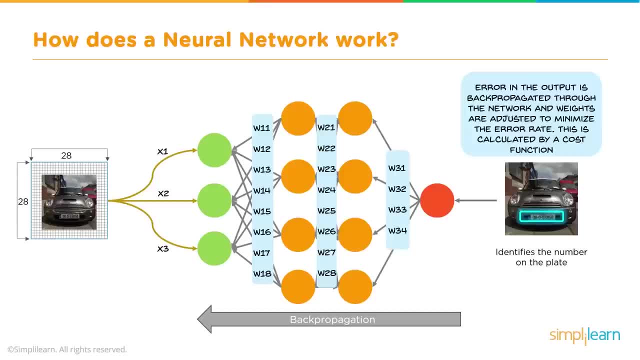 But if it's pretty close you might adjust the weights just a little bit And you keep adjusting the weights until they fit all the different training models you put in. So you might have 500 training models and those weights will adjust using the back propagation. 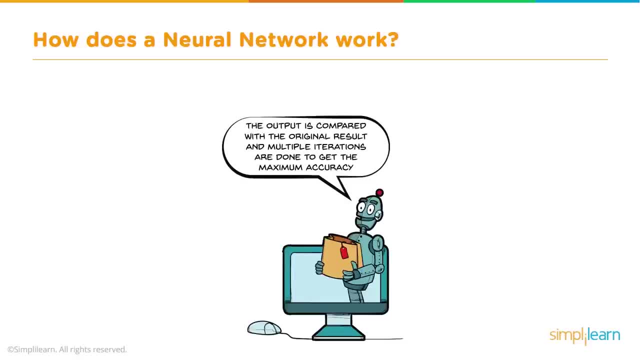 It sends the error backward, The output is compared with the original result, And multiple iterations are done to get the maximum accuracy. So not only does it look at each one, but it goes through it and just keeps cycling through the data, making small changes in the network. 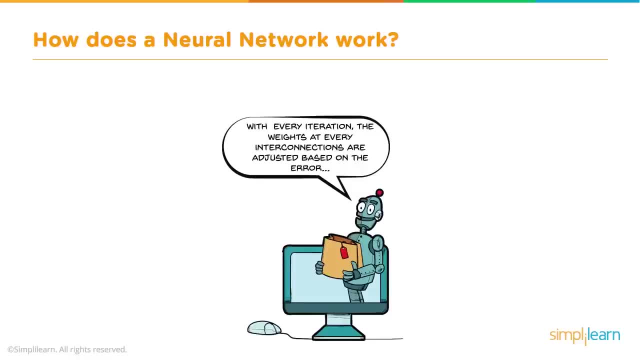 until it gets the right answers. With every iteration the weights at every interconnection are adjusted based on the error. We're not going to dive into that math because it is a differential equation And it gets a little complicated. But I will talk a little bit about some. 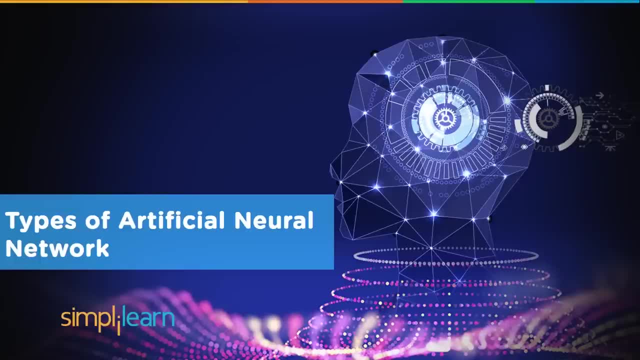 of the different options they have when we look at the code. So we've explored a neural network. Let's look at the different types of artificial neural networks. And this is like the biggest area growing is how these all come together. Let's see the different types of neural network. 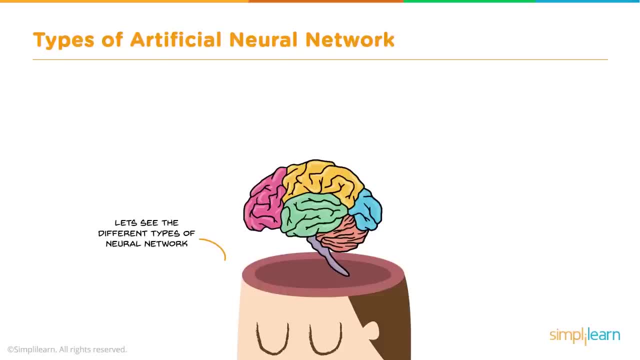 And again we're comparing this to human learning. So here's a human brain. I feel sorry for that poor guy. So we have a feed forward neural network, Simplest form of a. they call it ANN. a neural network. Data travels only in one direction: input to output. 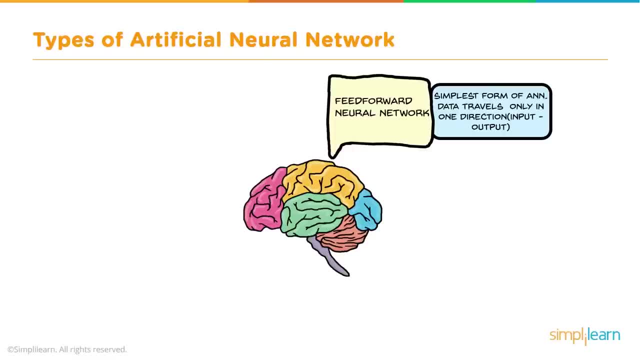 This is what we just looked at. So, as the data comes in, all the weights are added. It goes to the hidden layer, All the weights are added, It goes to the next hidden layer, All the weights are added And it goes to the output. 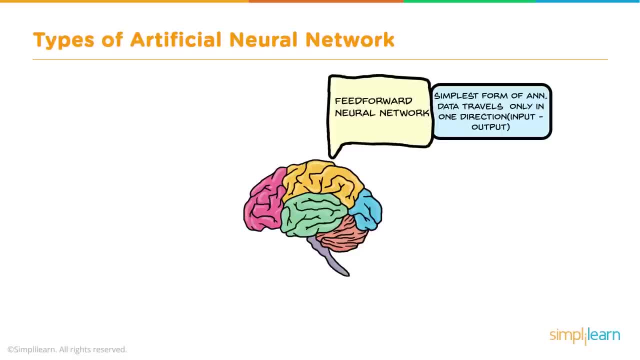 The only time you use the reverse propagation is to train it. So when you actually use it it's very fast. When you're training it, it takes a while because it has to iterate through all your training data And you start getting into big data. 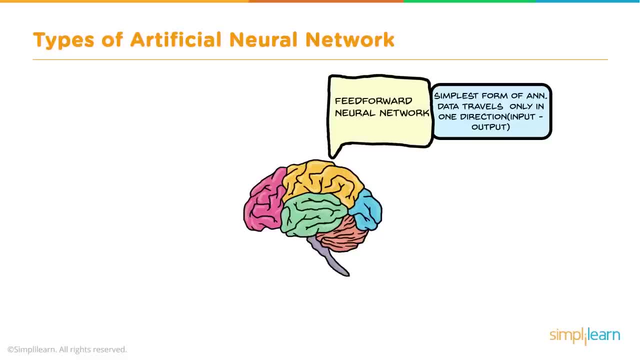 because you can train these with a huge amount of data. The more data you put in, the better train they get. The applications- vision and speech recognition- actually they're pretty much everything we talked about. Almost all of them use this form of neural network at some level. 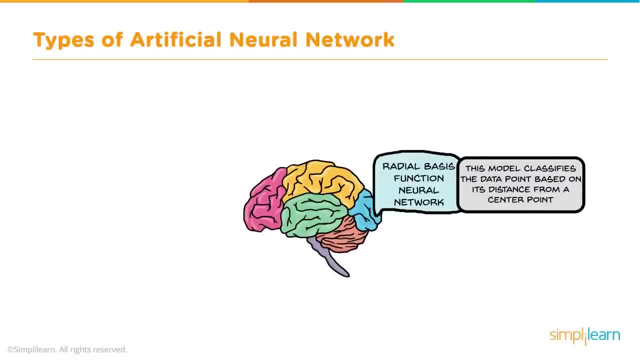 Radial basis function neural network. This model classifies the data point based on its distance from a center point. What that means is that you might not have training data, So you want to group things together And you create central points And it looks for all the things. 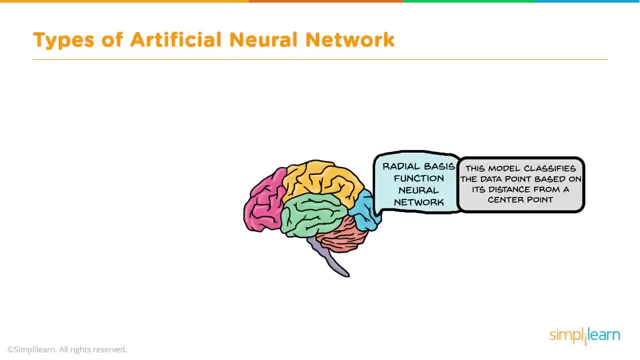 Some of these things are just like the other. If you've ever watched the Sesame Street as a kid, that dates me. So it brings things together And this is a great way. if you don't have the right training model, you can start finding things. 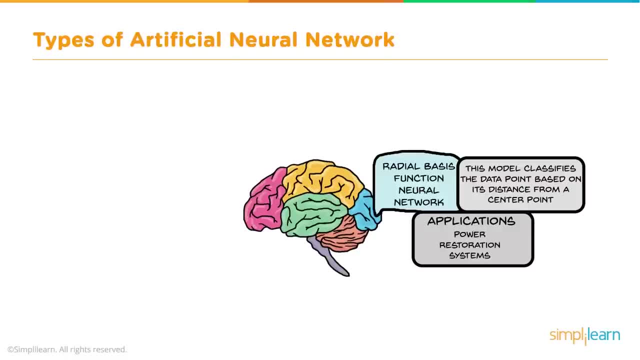 that are connected. you might not have noticed before Applications, power restoration systems. They try to figure out what's connected And then, based on that, they can fix the problem If you have a huge power system, Cajon and self-organizing neural network. 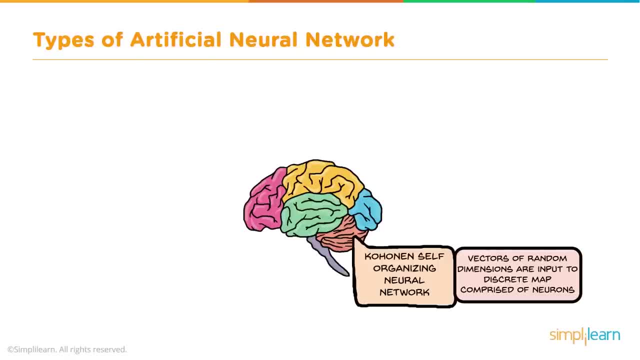 Vectors of random dimensions are input to discrete map comprised of neurons. So they basically find a way to draw and they call them. they say dimensions or vectors or planes, Because they actually chop the data in one dimension, two dimension, three dimension, four, five, six. 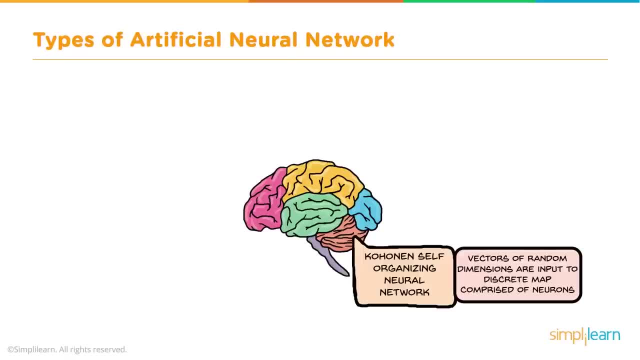 They keep adding dimensions and finding ways to separate the data and connect different data pieces together- Applications used to recognize patterns in data, like in medical analysis. The hidden layer saves its output to be used for future prediction- Recurrent neural networks. So the hidden layers remember its output from last time. 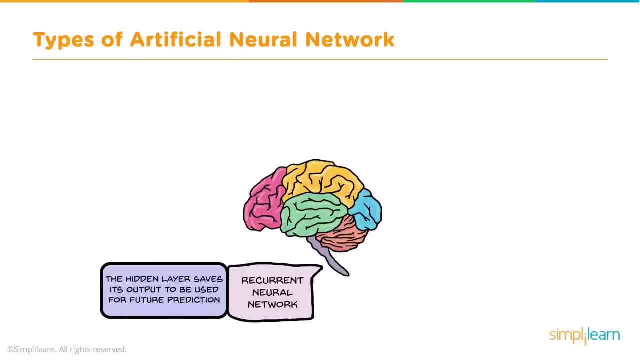 and that becomes part of its new input. You might use that, especially in robotics or flying a drone. You want to know what your last change was and how fast it was going, to help predict what your next change you need to make is to get. 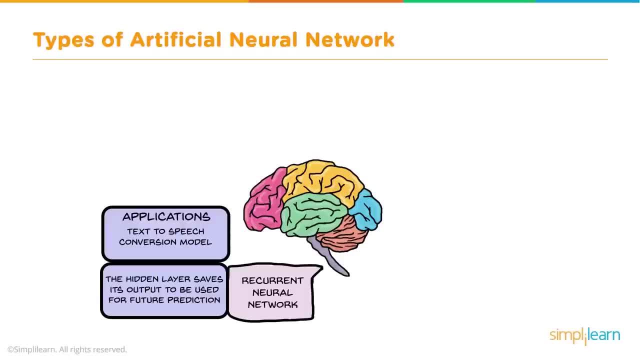 to where the drone wants to go. Applications: text to speech conversation model. So I talked about drones, but just identifying on Lexus or Google Assistant or any of these they're starting to add in. I'd like to play a song on my Pandora. 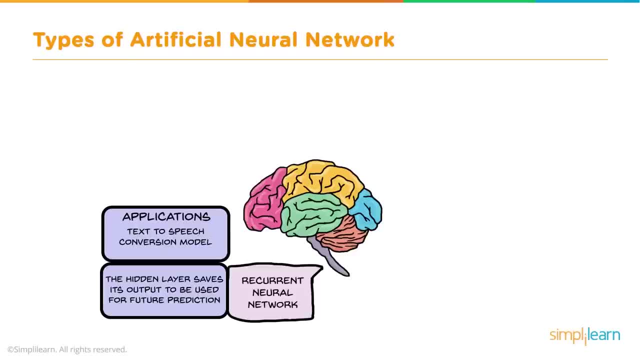 and I'd like it to be at volume 90%, So you now can add different things in there and it connects them together. The input features are taken in batches like a filter. This allows a network to remember an image in parts: Convolution, neural network. 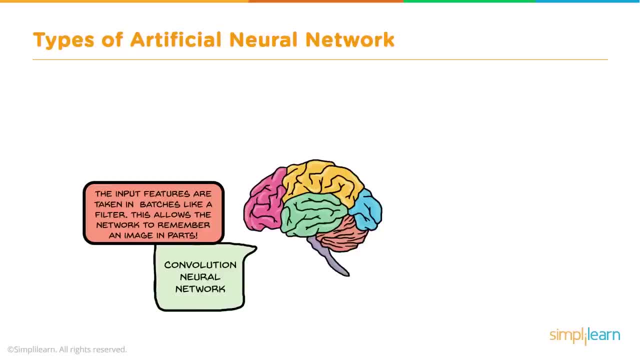 Today's world in photo identification and taking apart photos and trying to. you know, have you ever seen that on Google, where you have five people together? This is the kind of thing: separates all those people so that it can do a face recognition on each person. 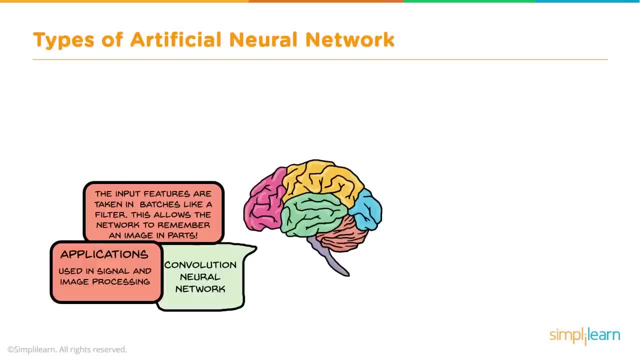 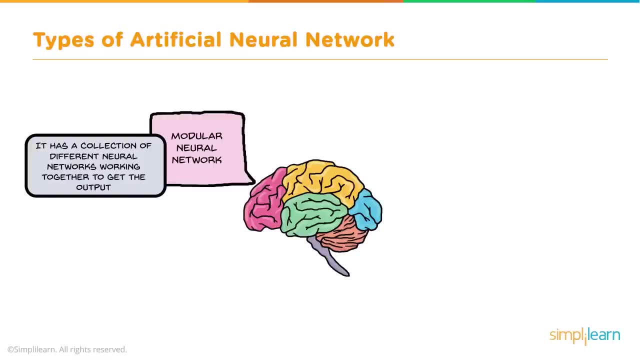 Applications used in signal and image processing. In this case, I used facial images or Google picture images as one of the options. Modular neural network: It has a collection of different neural networks working together to get the output. So, wow, we just went through all these different types. 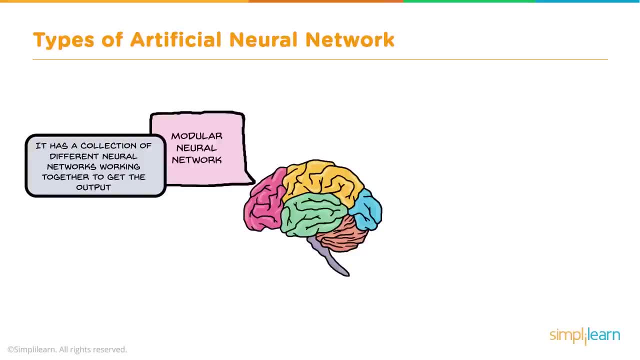 of neural networks And the final one is to put multiple neural networks together. I mentioned that a little bit when we separated people in a larger photo, individuals in the photo, and then do the facial recognition on each person. So one network is used to separate them. 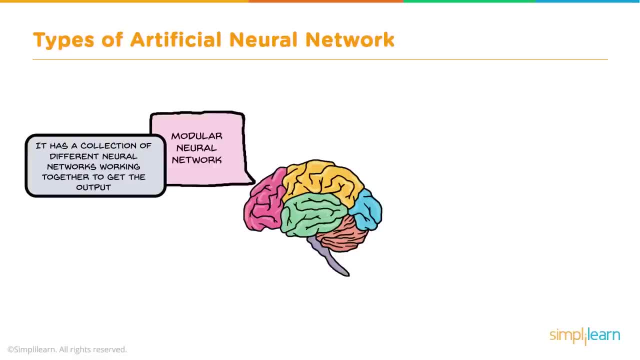 and the next network is then used to figure out who they are and do the facial recognition Applications still undergoing research. This is a cutting edge. You hear the term pipeline and there's actual in Python code and in almost all the different neural network setups. 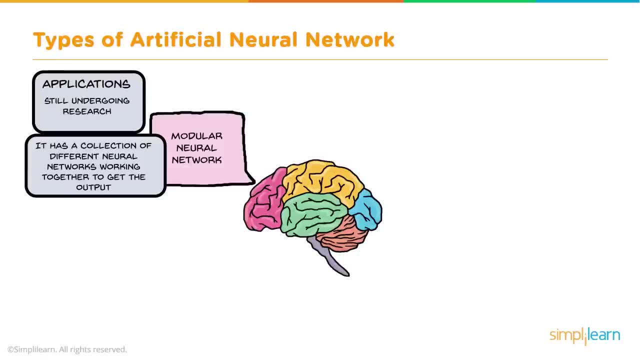 out there. they now have a pipeline feature usually, And it just means you take the data from one neural network and maybe another neural network, or you put it into the next neural network and then you take three or four other neural networks and feed them into another one. 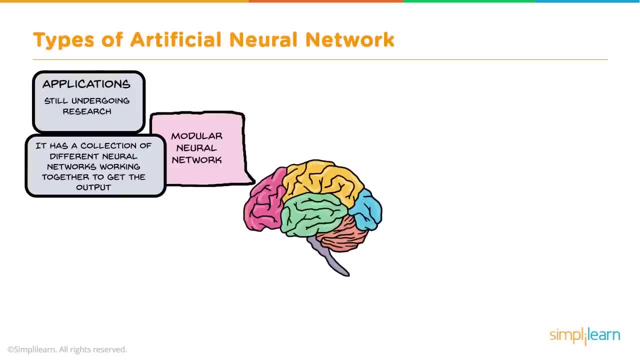 So how we connect the neural networks is really just cutting edge, And it's so experimental- I mean it's almost creative in its nature. There's not really a science to it because each specific domain has different things it's looking at. So if you're in the banking domain, 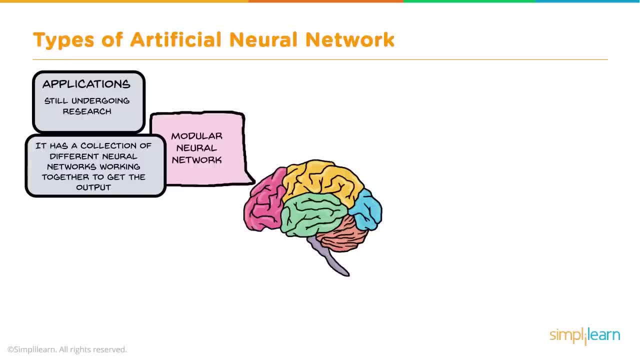 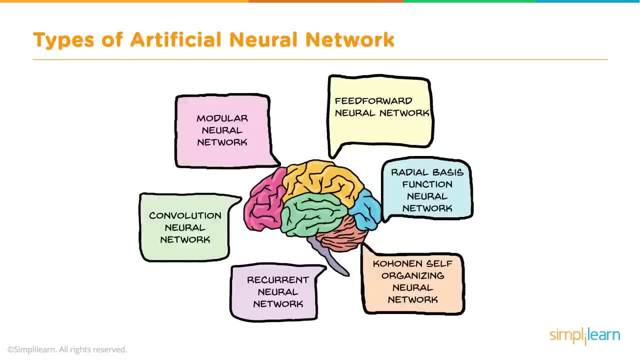 it's going to be different than the medical domain, than the automatic car domain, And suddenly figuring out how those all fit together is just a lot of fun And really cool. So we have our types of artificial neural network, We have our feed forward neural network. 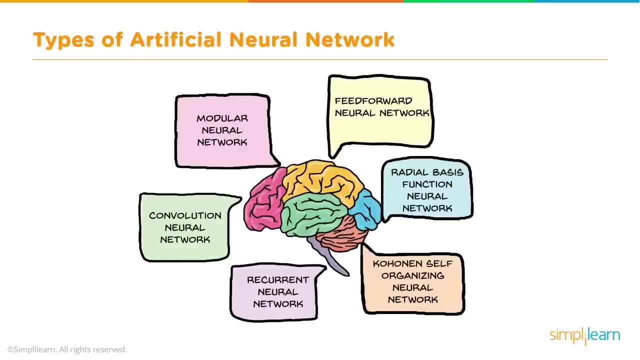 We have a radial basis function neural network. We have our cohenin self organizing neural network, recurrent neural network, convolution neural network and modular neural network where it brings them all together And know the colors on the brain do not match what your brain actually does. 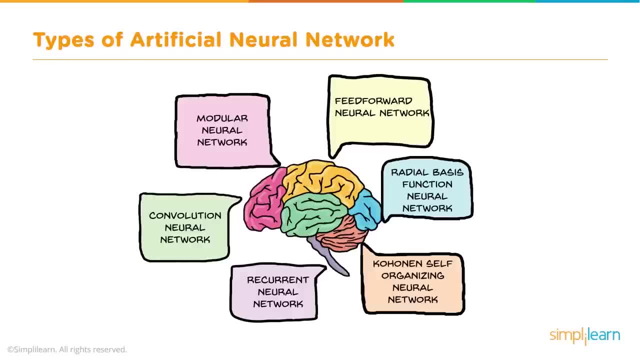 But they do bring it out that most of these were developed by understanding how humans learn, And as we understand more and more of how humans learn, we can build something in the computer industry to mimic that, to reflect that, And that's how these were developed. 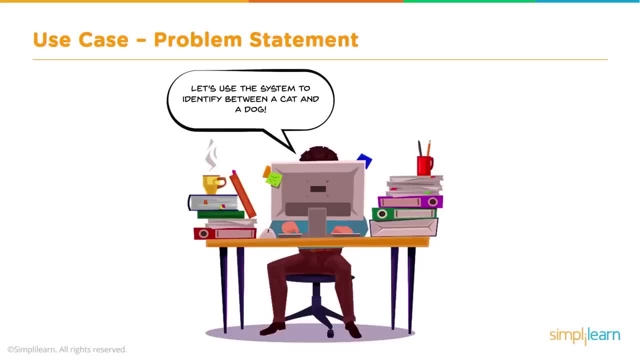 So exciting part: use case problem statement. So this is where we jump in. This is my favorite part. Let's use the system to identify between a cat and a dog. If you remember correctly, I said we're going to do some Python code. 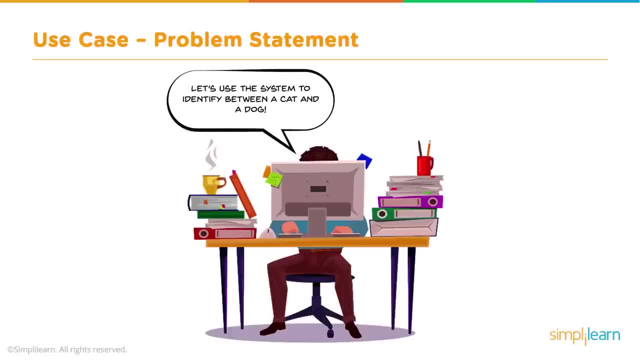 And you can see over here my hair is kind of sticking up over the computer. a cup of coffee on one side and then a little bit of old school- a pencil and a pen on the other side. Most people now take notes. 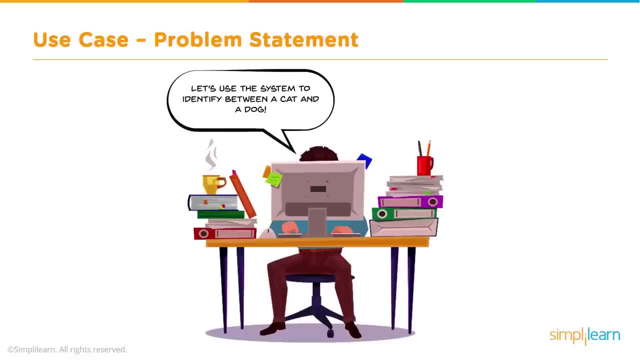 Yeah, I love the stickies on the computer. That's great. That is my computer. I have sticky notes on my computer in different colors, So not too far from today's programmer. So the problem is, is we want to classify photos of cats? 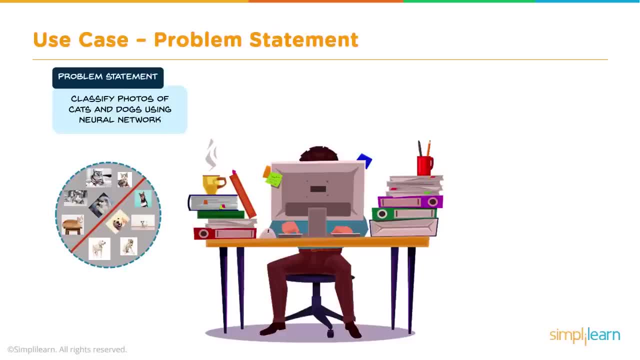 and dogs using a neural network And you can see over here we have quite a variety of dogs in the pictures and cats, And just sorting out it is a cat is pretty amazing, And why would anybody want to even know the difference between a cat and a dog? 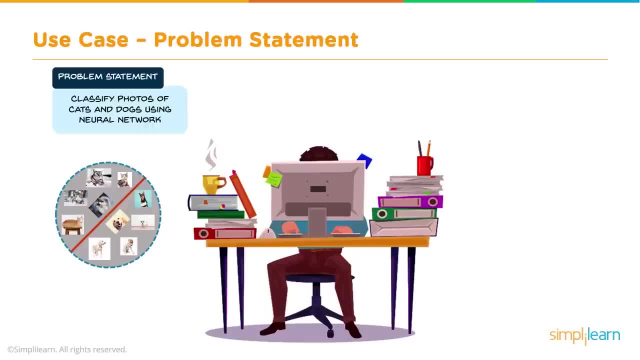 OK, why? Well, I have a cat door. It'd be kind of fun That, instead of it identifying, instead of having like a little collar with a magnet on it- which is what my cat has- the door would be able to see. 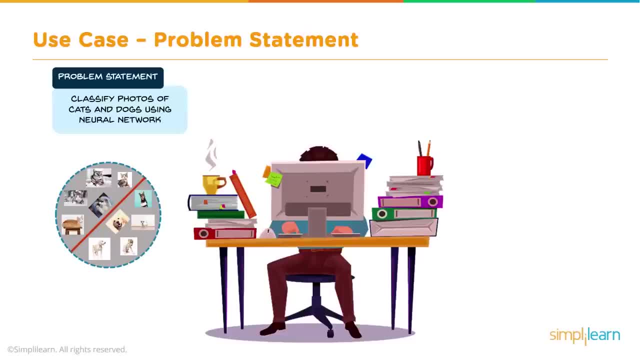 oh, that's the cat. That's our cat coming in. Oh, that's the dog. We have a dog too. That's the dog I want to let in. Maybe I don't want to let this other animal in because it's a raccoon. 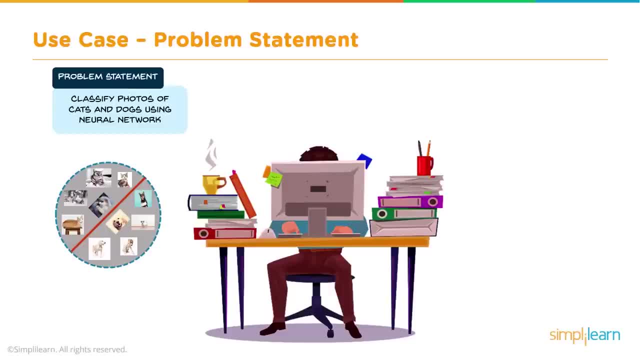 So you can see where you could take this one step further and actually apply this. You could actually start a little startup company idea, a self-identifying door. So this use case will be implemented on Python. I am actually in Python 3.0.. 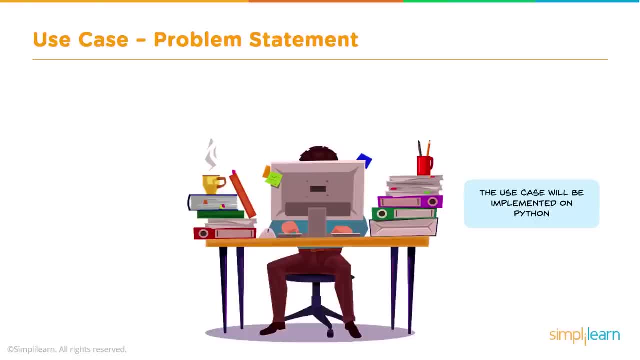 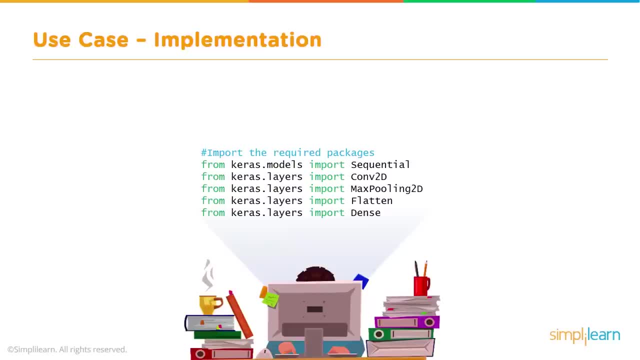 3.6.. It's always nice to tell people the version of Python, because it does affect sometimes which modules you load and everything. And we're going to start by importing the required packages. I told you we're going to do this in Keras. 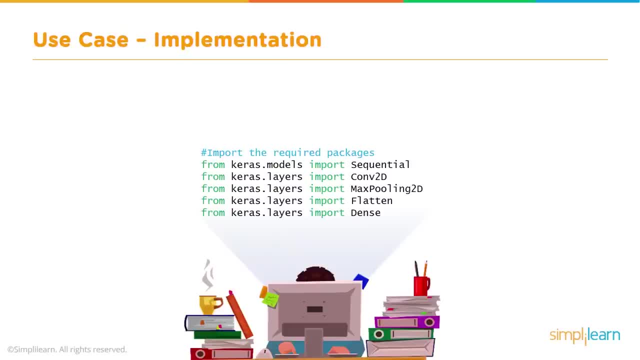 So we're going to import from Keras models a sequential from the Keras layers: conversion 2D or CONV 2D, max pooling 2D, flatten and dense, And we'll talk about what each one of these do in just a second. 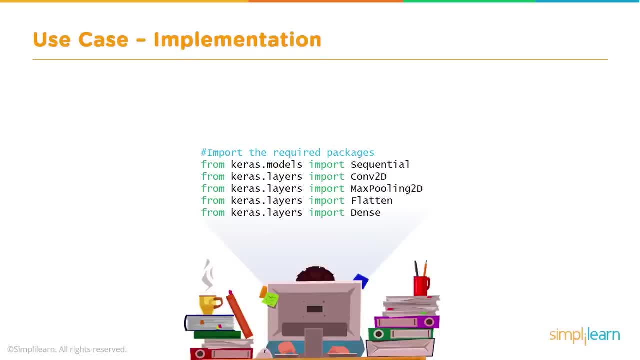 But before we do that, let's talk a little bit about the environment we're going to work in And, in fact, let me go ahead and open the website, Keras's website, so we can learn a little bit more about Keras. 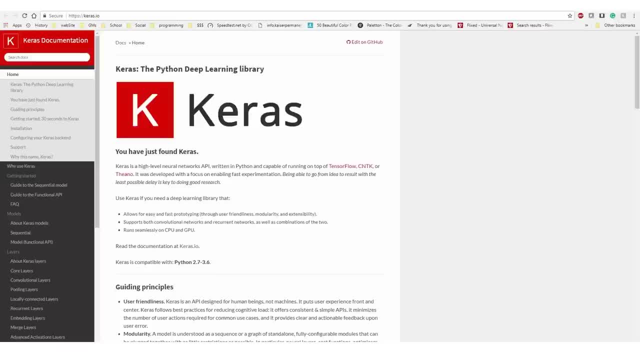 So here we are on the Keras website, And it's K-E-R-A-S dot I-O. That's the official website for Keras, And the first thing you'll notice is that Keras runs on top of either TensorFlow, CNTK, and I think 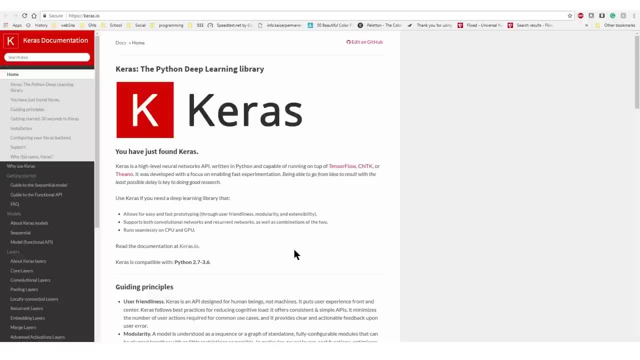 it's pronounced Thano or Theano. What's important on here is that TensorFlow- and the same is true for all these, but TensorFlow is probably one of the most widely used currently- Package is out there with the Keras And, of course, tomorrow this is all going to change. 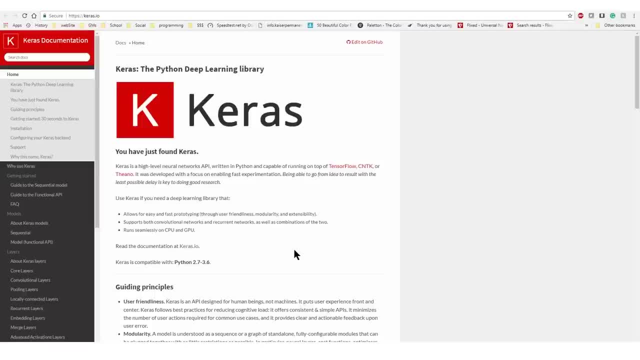 It's all going to disappear and they'll have something new out there. So make sure, when you're learning this code, that you understand what's going on and also know the code. I mean when you look at the code, it's not as complicated once you understand what's going on. 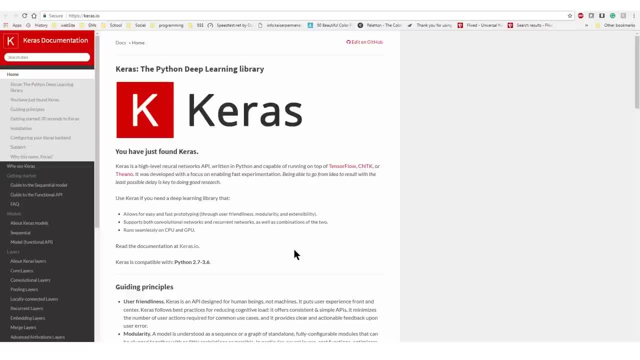 The code itself is pretty straightforward And the reason we like Keras and the reason that people are jumping on it right now and it's such a big deal, is if we come down here. Let me just scroll down a little bit. 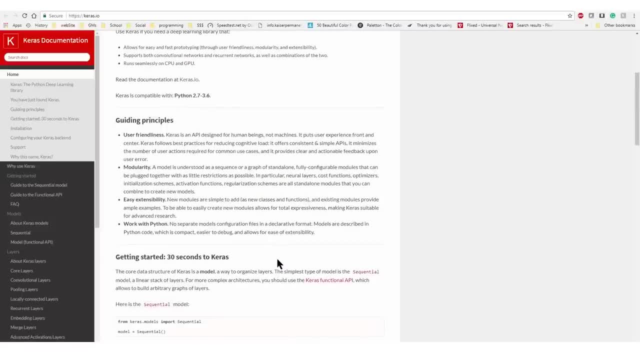 They talk about user friendliness, modularity, easy extensibility, Work with Python. Python's a big one because a lot of people in data science now use Python. although you can actually access Keras other ways- If we continue down here is layers. 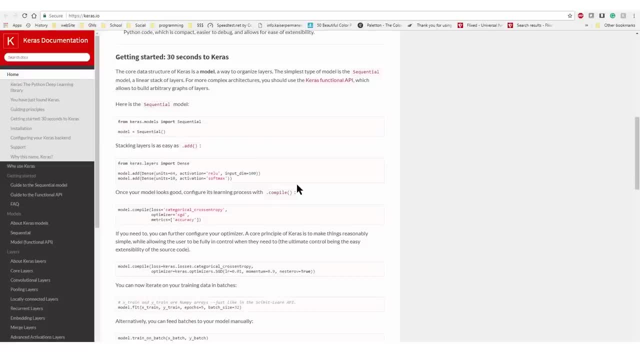 And this is where it gets really cool When we're working with Keras, you just add layers on. Remember those hidden layers we were talking about? And we talked about the RELU activation You can see right here. Let me just up that a little bit in size. 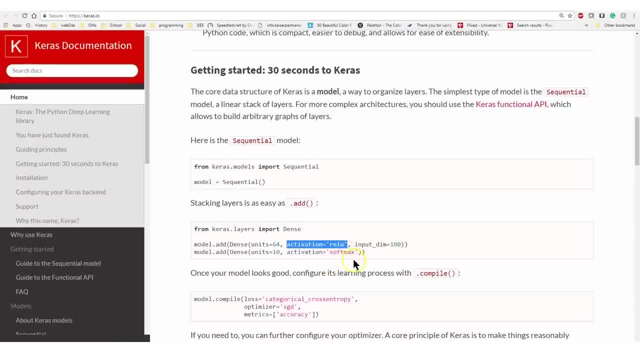 There we go. That's big, I can add in an RELU layer and then I can add in a softmax layer. in the next instance We didn't talk about softmax, So you can do each layer separate. Now, if I'm working in some of the other kits I use, 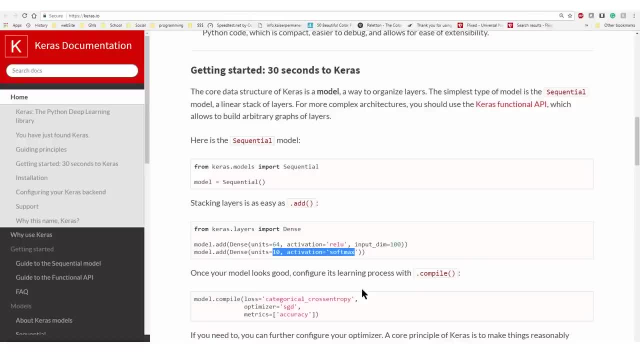 I take that and I have one setup and then I feed the output into the next one- This one, I can just add hidden layer after hidden layer with the different information in it, which makes it very powerful and very fast to spin up and try. 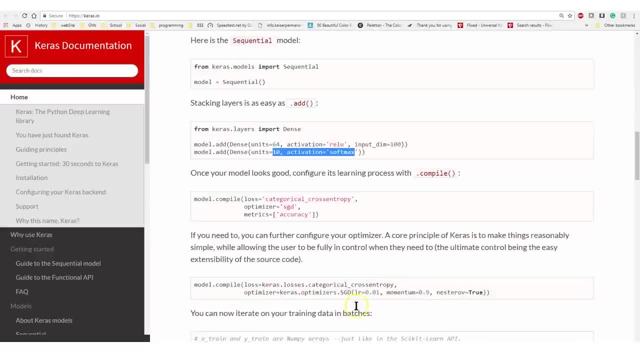 different setups and see how they work with the data you're working on, And we'll dig a little bit deeper in here, And a lot of this is very much the same. So when we get to that part, I'll point that out to you also. 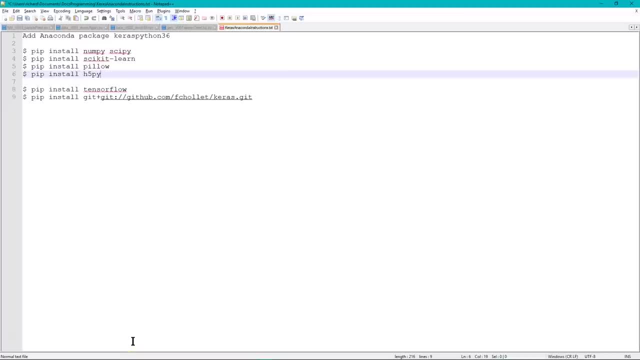 Now Just a quick side note. I'm using Anaconda with Python in it And I went ahead and created my own package And I called it the KerasPython3.6, because I'm in Python 3.6.. Anaconda is cool that way. 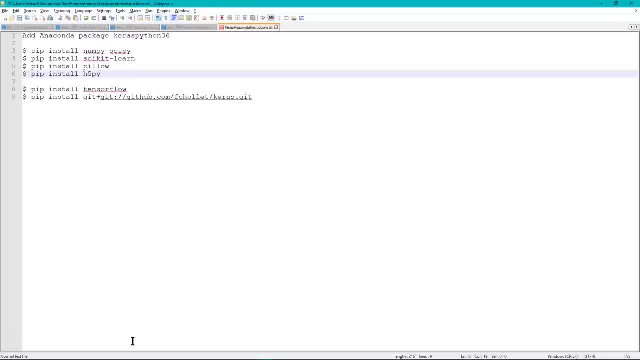 You can create different environments really easily. If you're doing a lot of different, experimenting with these different packages, you probably want to create your own environment in there, And the first thing is: you can see right here there's a lot of dependencies. 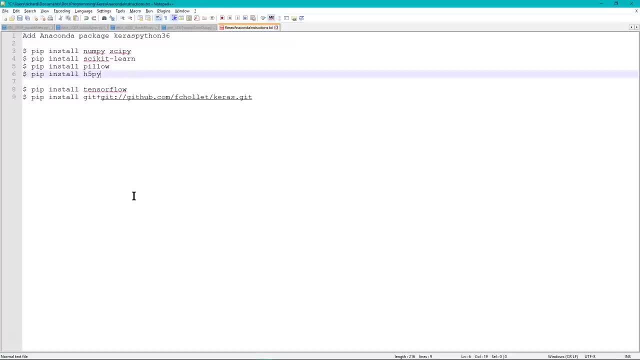 A lot of these. you should recognize by now if you've done any of these videos. If not, kudos for you for jumping in today. pip, install numpy scipy. The scikit-learn Pillow and h5py are both needed for the TensorFlow. 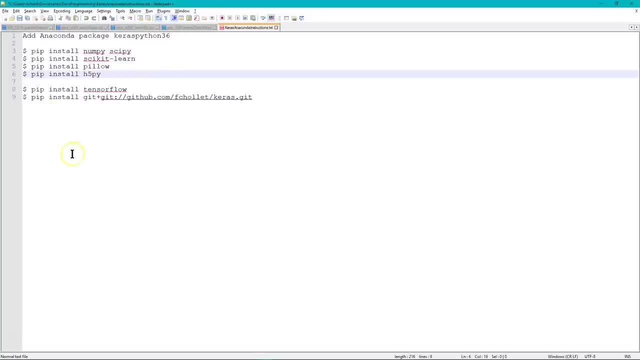 and then putting the Keras on there, And then you'll see here- and pip is just a standard installer that you use with Python. You'll see here that we did pip install TensorFlow, Since we're going to do Keras on top of TensorFlow. 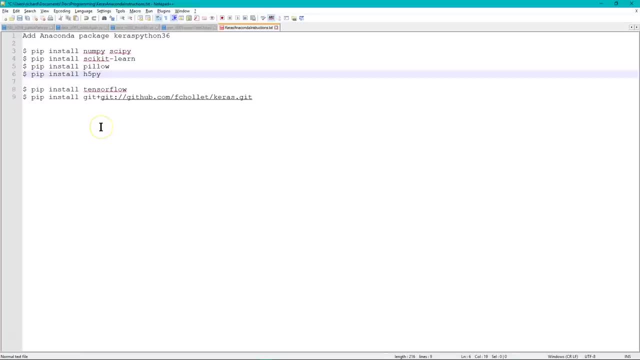 And then pip install And I went ahead and used the GitHub. So git plus git And you'll see here githubcom. This is one of their releases, one of the most current release on there that goes on top of TensorFlow, And you can look up these instructions. 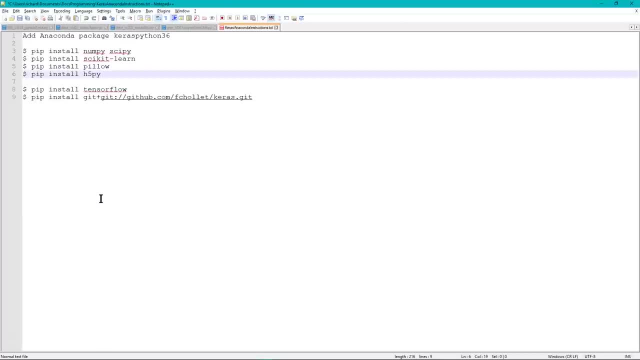 pretty much anywhere. This is for doing it on Anaconda. Certainly you'd want to install these. if you're doing it in Ubuntu server setup, You'd want to get. I don't think you need the h5py in Ubuntu, But you do need the rest in there because they. 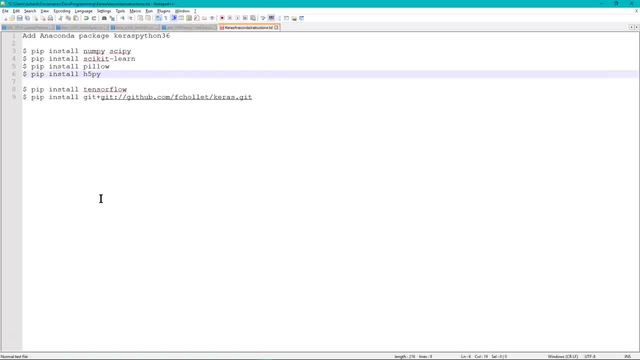 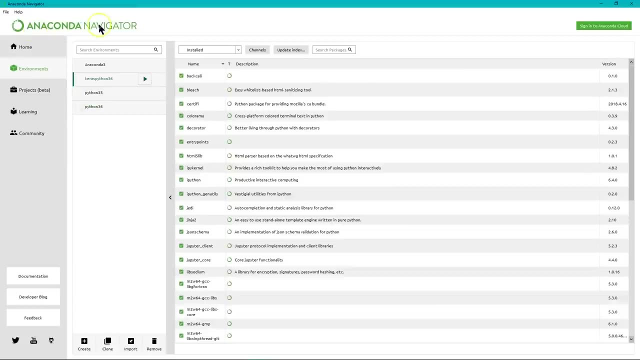 are dependencies in there And it's pretty straightforward And that's actually in some of the instructions they have on their website, So you don't have to necessarily go through this, Just remember their website on there. And then when I'm under my Anaconda navigator, which 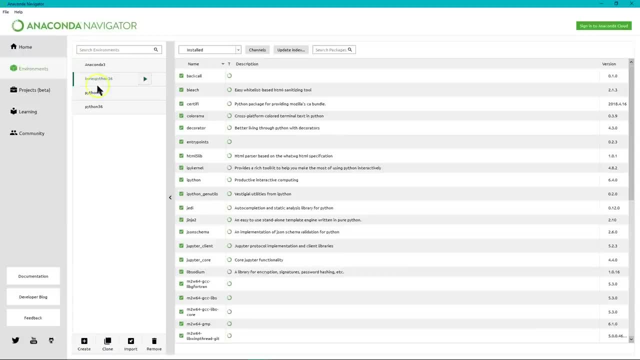 I like. you'll see where I have environments And on the bottom I created a new environment And I called it Keras. It's Python 36, just to separate everything You can say, I have Python 30.5 and Python 36.. 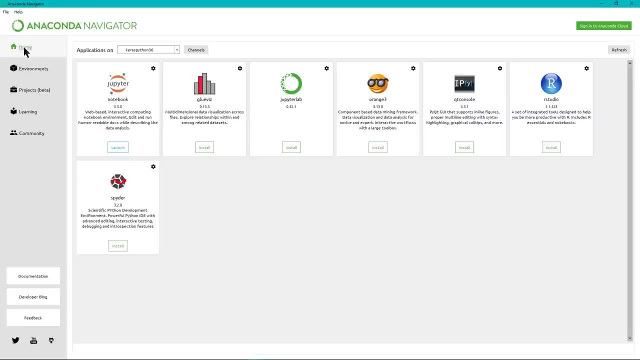 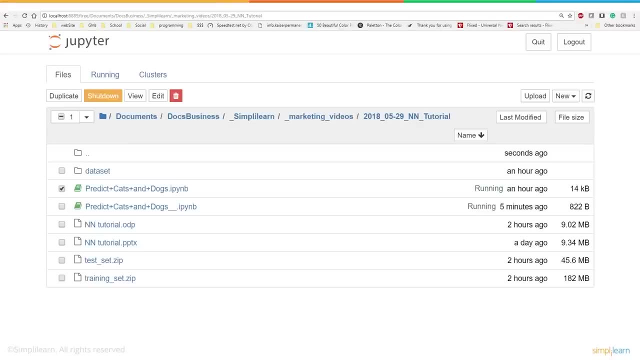 I used to have a bunch of other ones, but it kind of cleaned house recently And, of course, once I go in here, I can launch my Jupyter Notebook, making sure I'm using the right environment that I just set up. This, of course, opens up my, in this case. 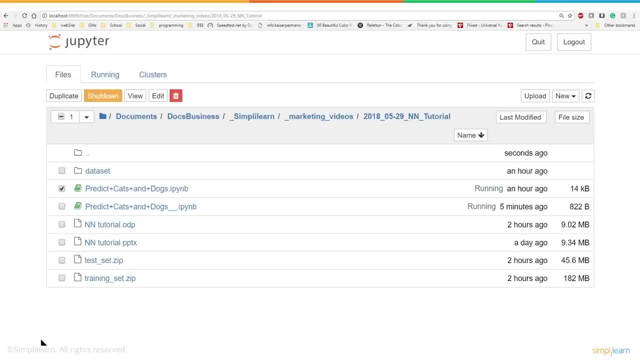 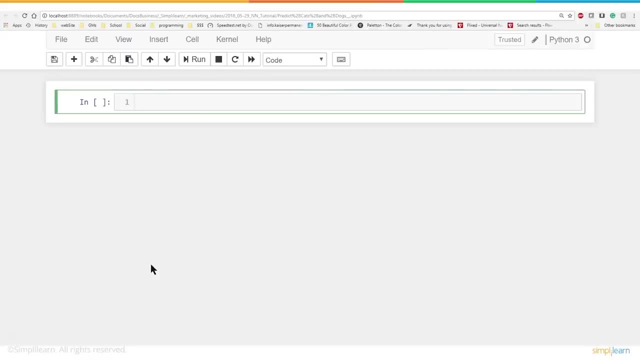 I'm using Google Chrome And in here I could go and just create a new document in here And this is all in your browser. when you use the Anaconda, Do you have to use Anaconda and Jupyter Notebook? No, You can use any kind of Python editor, whatever setup. 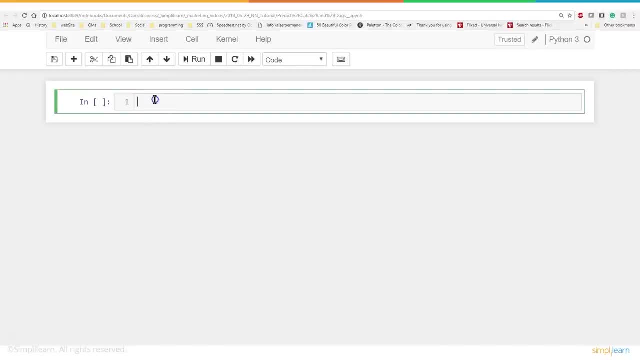 you're comfortable with and whatever you're doing in there. So let's go ahead and go in here and paste the code in And we're importing a number of different settings in here. We have import sequential. That's under the models, because that's the model we're going to use as far as our neural network. 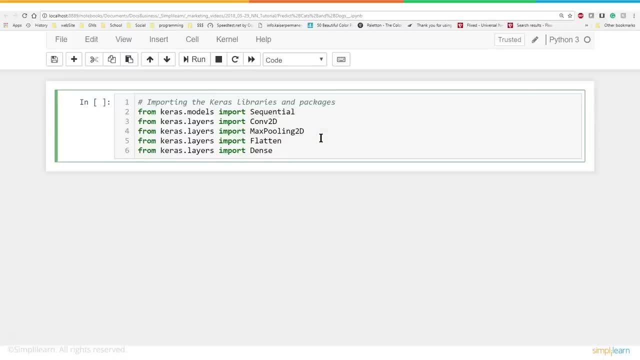 And then we have layers And we have conversion, 2D max pooling, 2D, flatten, dense- And you can actually just kind of guess at what these do. We're talking, We're working, We're in a 2D photograph. 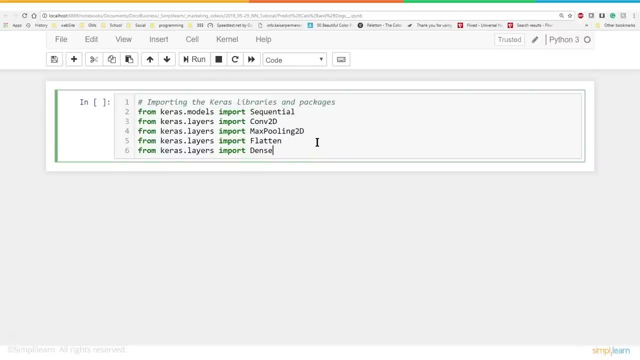 And, if you remember correctly, I talked about how the actual input layer is a single array. It's not in two dimensions, It's one dimension. All these do is these are tools to help flatten the image. So it takes a two-dimensional image and then it creates its own proper setup. 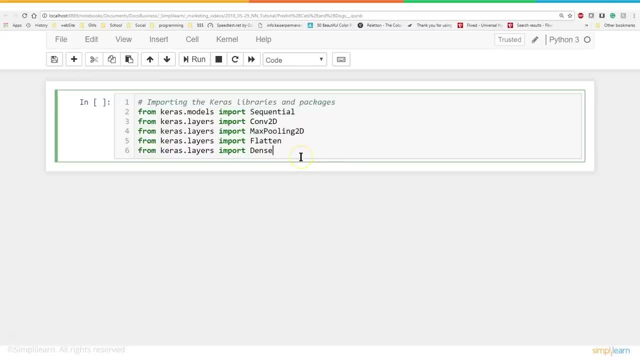 You don't have to worry about any of that. You don't have to do anything special with the photograph. You let the Keras do it And we're going to run this And you'll see right here they have some stuff that is going to be depreciated and changed. 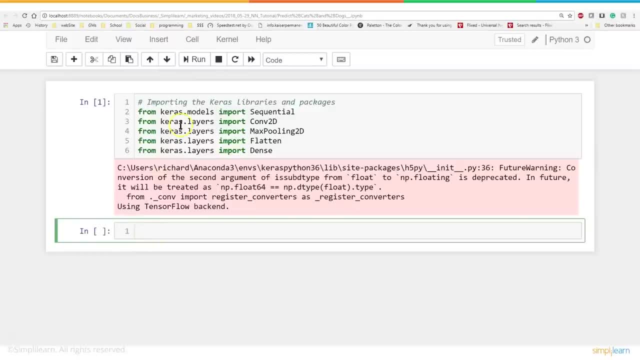 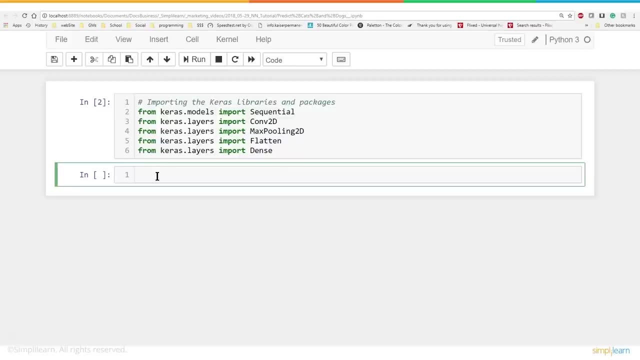 because that's what it does. Everything's being changed as we go. You don't have to worry about that too much If you have warnings. if you run it a second time, the warning will disappear, And this has just imported these packages for us to use. 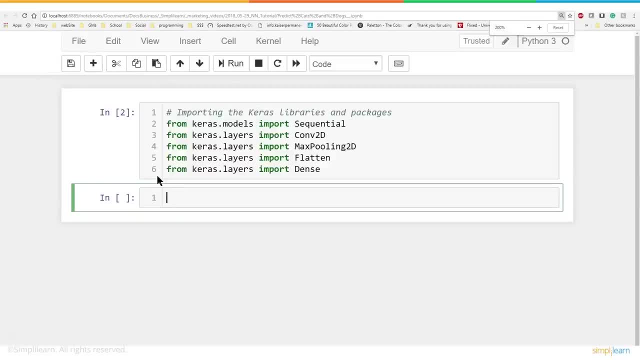 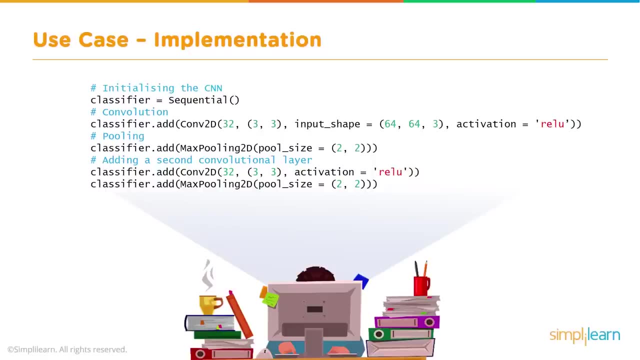 Jupyter's nice about this that you can do each thing step-by-step, And I'll go ahead and also zoom in there a little control plus. That's one of the nice things about being in a browser environment. So here we are back. 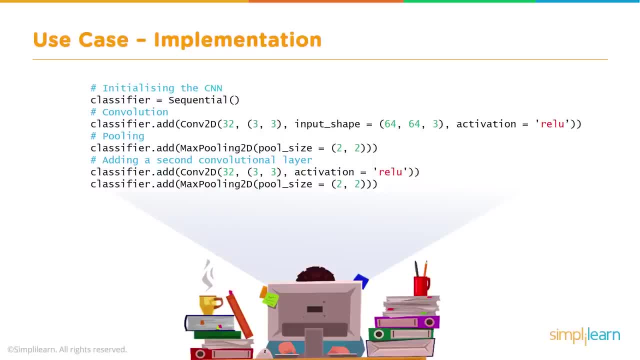 Another sip of coffee. If you're familiar with my other videos, you'll notice I'm always sipping coffee. I always have a- in my case latte- next to me an espresso. So the next step is to go ahead and initialize. 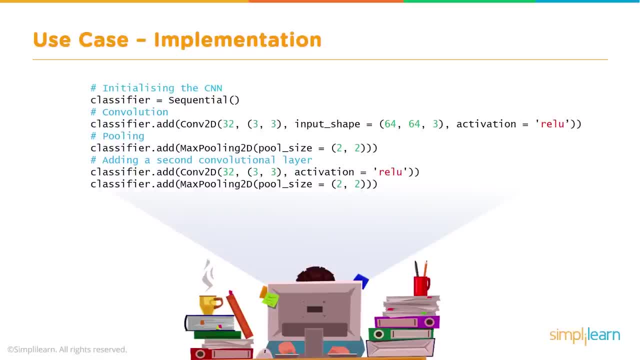 We're going to call it the CNN, Our classifier neural network. And the reason we call it a classifier is because it's going to classify it between two things: It's going to be cat or dog. So when you're doing classification, you're picking specific objects. 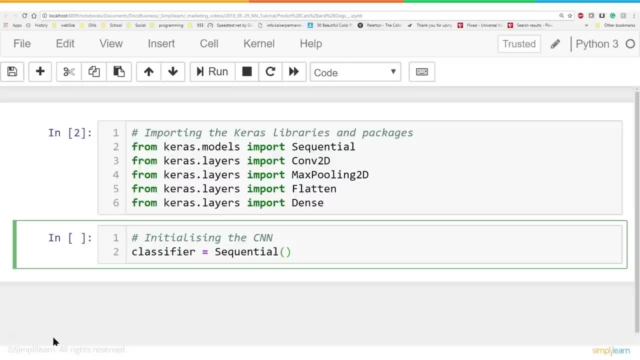 It's a true or false, yes, no, it is something or it's not. So, first thing, we're going to create our classifier and it's going to equal sequential, So their sequential setup is the classifier. That's the actual model we're using. 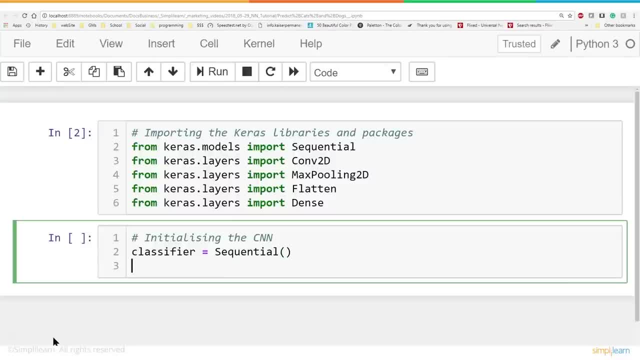 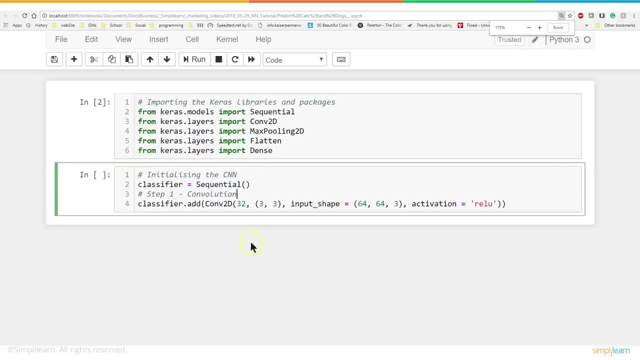 That's the neural network. So we call it a classifier And the next step is to go ahead and initialize. The next step is to add in our convolution. And let me just do a, let me shrink that down in size so you can see the whole line. 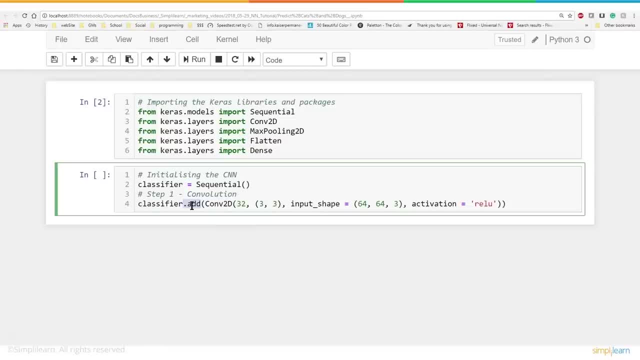 And let's talk a little bit about what's going on here. I have my classifier and I add something. What am I adding? Well, I'm adding my first layer. This first layer we're adding in is probably the one that takes the most work to make sure. 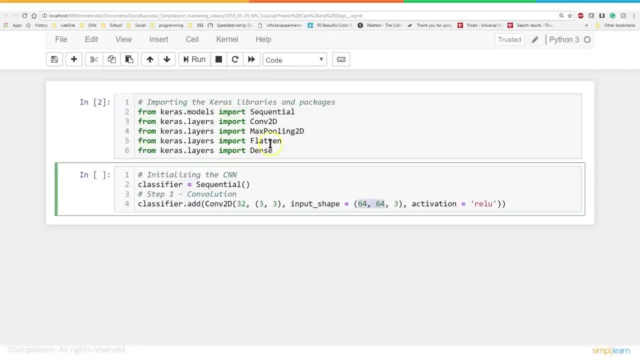 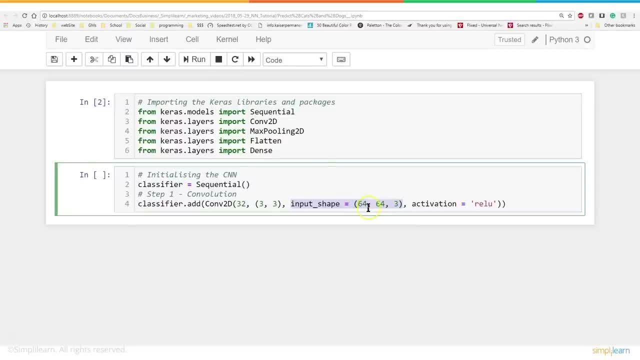 What does that mean? Well, that means that our picture's coming in. And there's these pictures. Remember, we had, like the picture of the car was 128 by 128 pixels. Well, this one is 64 by 64 pixels. 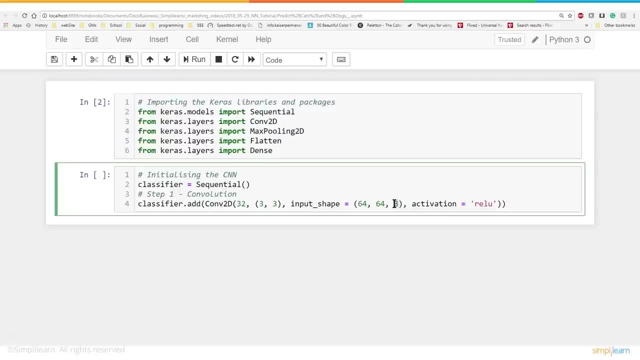 And each pixel has three values. That's where these numbers come from And it is so important that this matches. I mentioned a little bit that if you have like a larger picture, you have to reformat it to fit this shape. If it comes in as something larger, there's no input nodes. 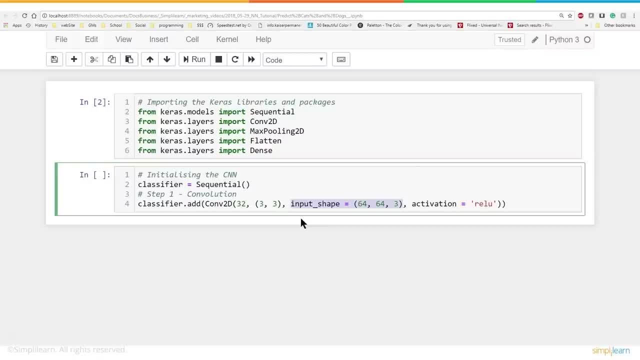 There's no input nodes, There's no input neural network there that will handle that extra space. So you have to reshape your data to fit in here. Now, the first layer is the most important, Because after that Keras knows what your shape is coming in here. 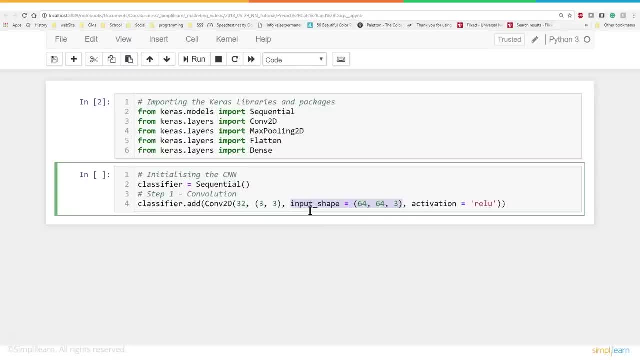 And it knows what's coming out, And so that really sets the stage. Most important thing is that input shape matches your data coming in, And you'll get a lot of errors. if it doesn't, You'll go through there and picture number 55 doesn't match it correctly. 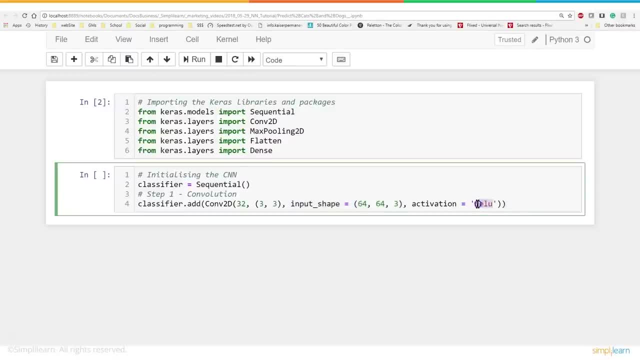 And guess what it does? It usually gives you an error. And then the activation. if you remember, we talked about the different activations on here. We're using the RELU model. Like I said, that is the most commonly used now. 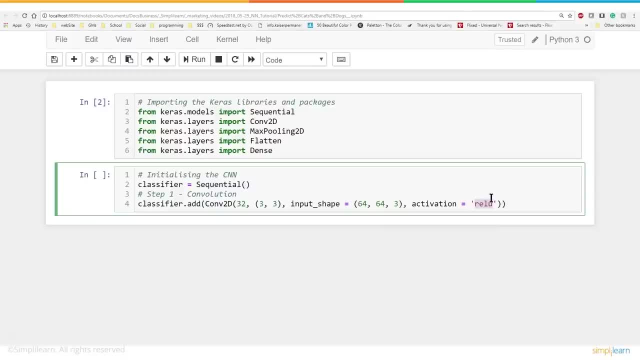 Because one it's fast. It doesn't have the added calculations in it, It just says: here's the value coming out based on the weights and the value going in, And from there, if it's over 1, then it's good. 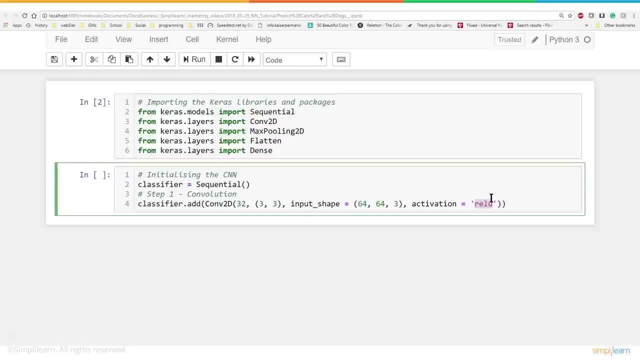 Or over 0, it's good. If it's under 0, then it's considered not active, And then we have this conversion 2D. What the heck is conversion 2D? I'm not going to go into too much detail in this, because this has a couple of things. 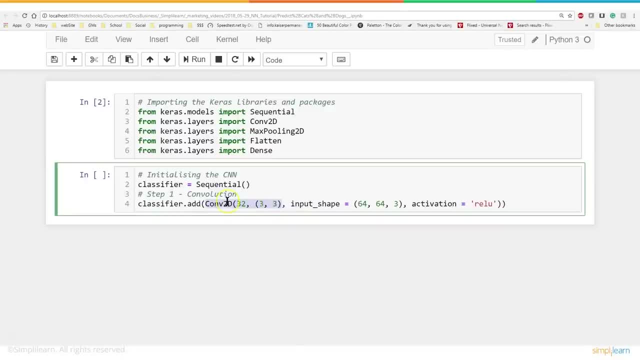 it's doing in here A little bit more in-depth than we're ready to cover in this tutorial. But this is used to convert from the photo because we have 64 by 64 by 3. And we're just converting it to two-dimensional kind of setup. 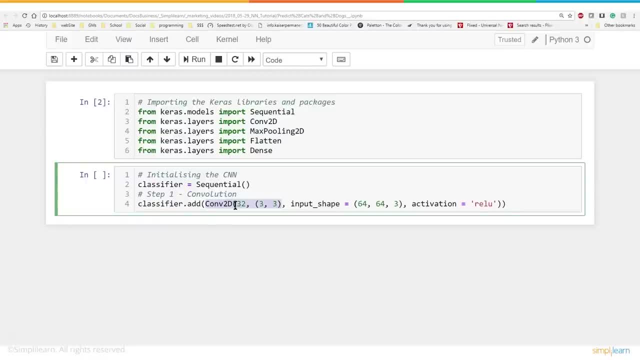 So it's very aware that this is a photograph and that different pieces are next to each other. And then we're going to add in a second convolutional layer- That's what the C-O-N-V stands for- 2D. So these are hidden layers. 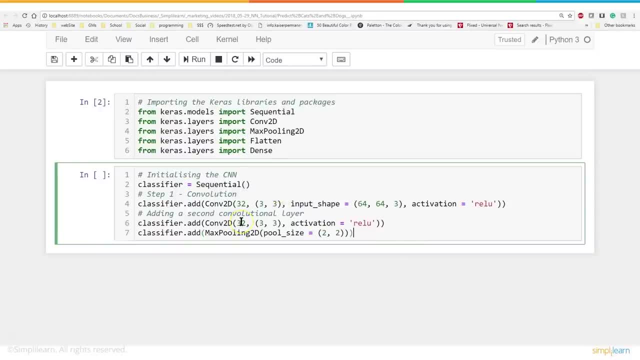 So we have our input layer and our two hidden layers And they are two-dimensional because we're doing it with a two-dimensional photograph And you'll see down here that on the last one we add a max pooling 2D And we put a pool size equals 2, 2.. 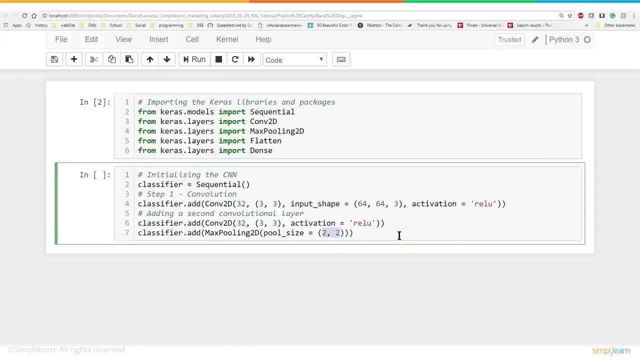 And so what this is is that, as you get to the end of these layers, one of the things you always want to think of is what they call mapping and then reducing- Wonderful terminology- from the big data. We're mapping this data through all these layers and now we want to reduce it to only. 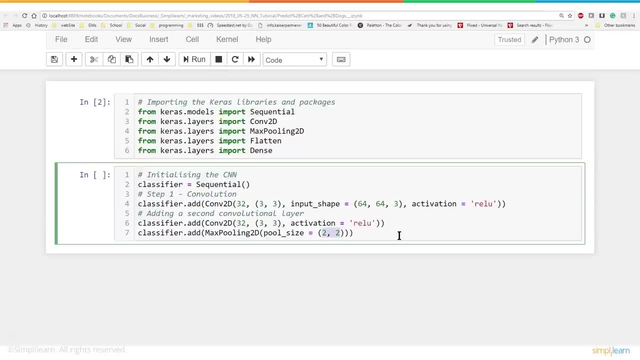 two sets. In this case it's already in two sets because it's a 2D photograph, But we had, you know, two dimensions by. we actually have 64 by 64 by 3. So now we're just getting it down to a 2 by 2.. 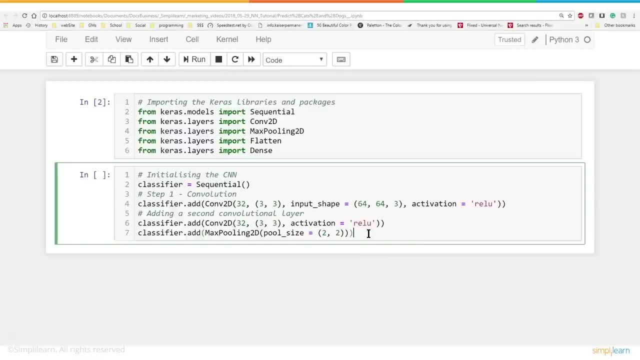 Just the two-dimension- two-dimensional instead of having the third dimension of colors, And we'll go ahead and run these. We're not really seeing anything on our run script because we're just setting up. This is all set up And this is where you start playing, because maybe you'll add a different layer in here. 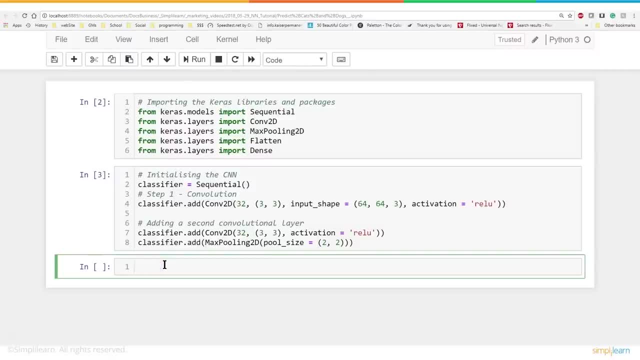 to do something else, to see how it works and see what your output is. That's what makes Keras so nice- As I can, with just a couple flips of code, put in a whole new layer that does a whole new processing and see whether that improves my run or makes it worse. 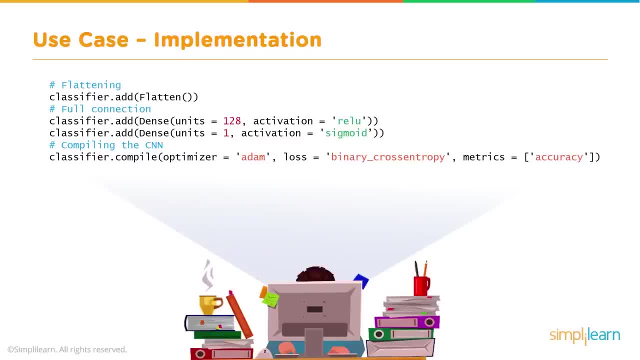 And finally, we're going to do the final setup, which is to flatten classifier, add a flatten setup, And then we're going to also add a layer, a dense layer, And then we're going to add in another dense layer And then we're going to build it. 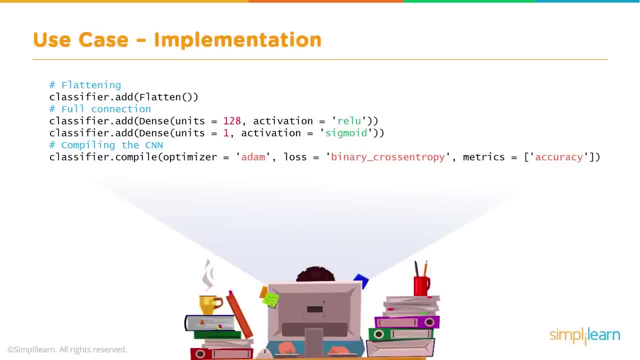 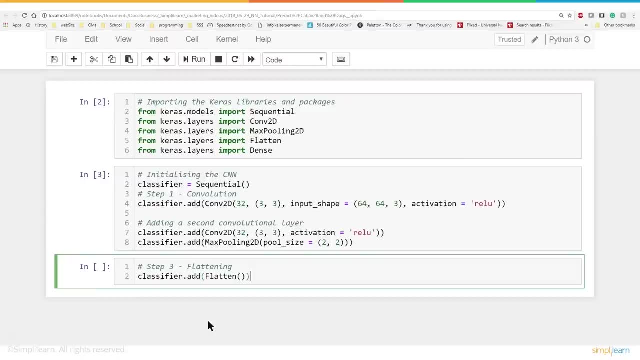 We're going to compile this whole thing together. So let's flip over and see what that looks like, And we've even numbered them for you. So we're going to do the flattening. Flatten is exactly what it sounds like. We've been working in a two-dimensional array of picture which actually is in three dimensions. 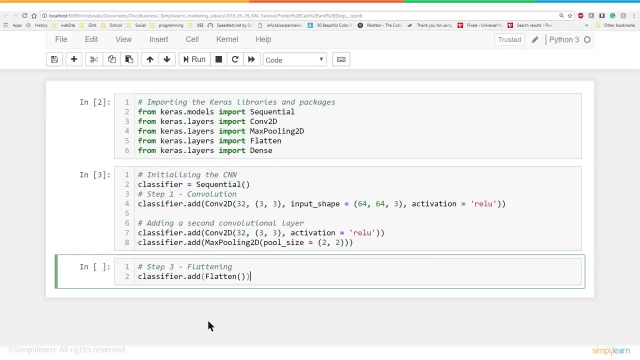 because of the pixels. The pixels have a whole other dimension to it of three different values And we've kind of resized those down to two by two. But now we're just going to flatten it. I don't want to have multiple dimensions being worked on by tensor and by Keras. 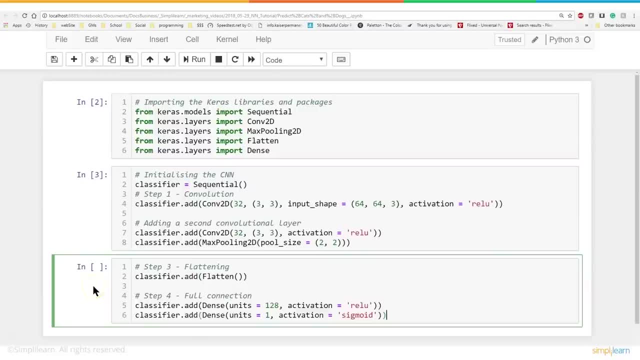 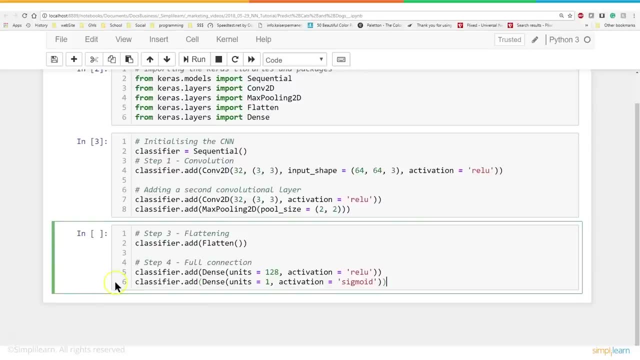 I want just a single array, so it's flattened out, And then step four, full connection. So we add in our final two layers And you could actually do all kinds of things with this. You could actually leave out some of these layers and play with them. 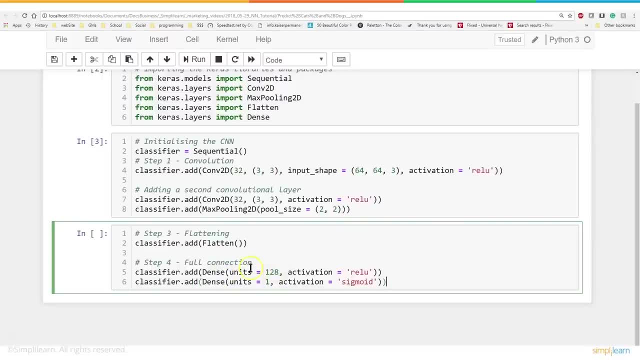 You do need to flatten it. That's very important. Then we want to use the dense Again. we're taking this and we're taking whatever came into it. So once we take all those different two dimensions or three dimensions as they are, and we flatten, 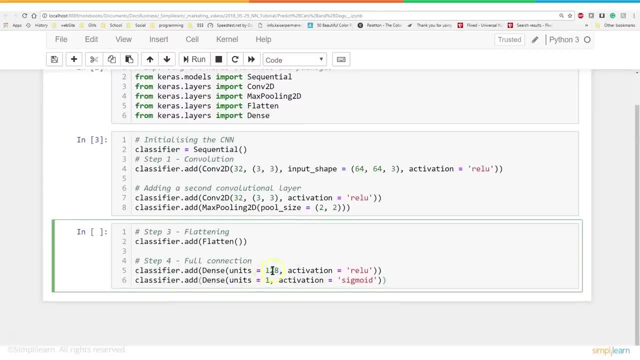 it to one dimension. we want to take that and we're going to pool it into units of 128.. They got that. You're going to say: where did they get 128 from? You could actually play with that number and get all kinds of weird results. 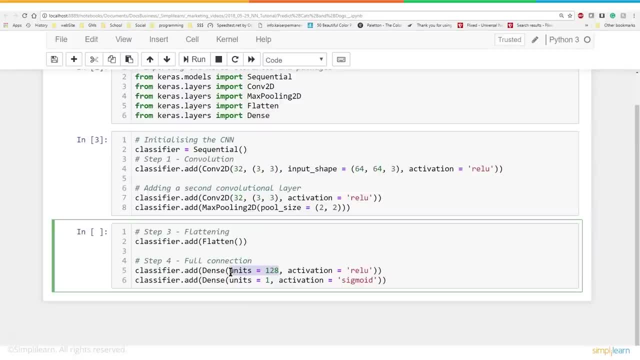 But in this case we took the 64 plus 64 is 128.. You could probably even do this with 64 or 32.. Usually you want to keep it in the same multiple, whatever the data shape you're already using is in. 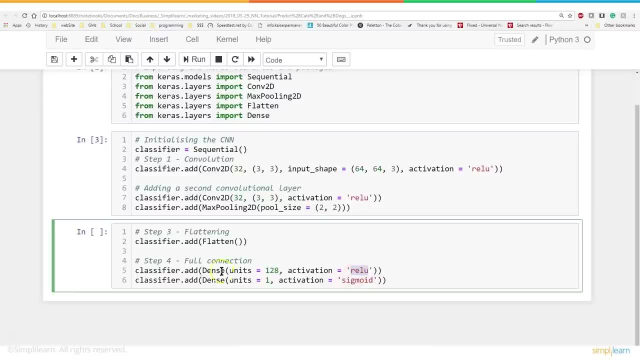 And we're using the activation, the R-E-L-U, just like we did before, And then we finally filter all that into a single output, And it has how many units One Why? Because we want to know whether true or false. 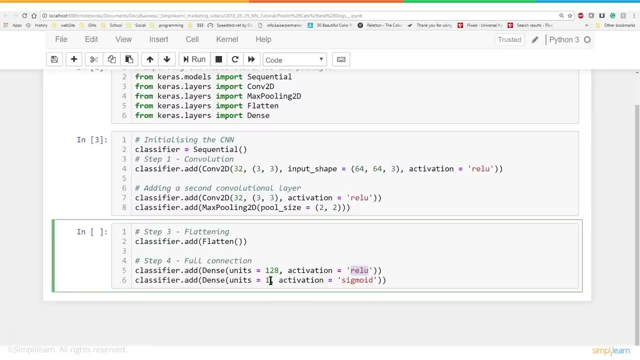 It's either a dog or a cat. You could say one is dog, zero is cat. Or maybe you're a cat lover And it's one is cat and zero is dog. If you love both dogs and cats, you're going to have to choose. 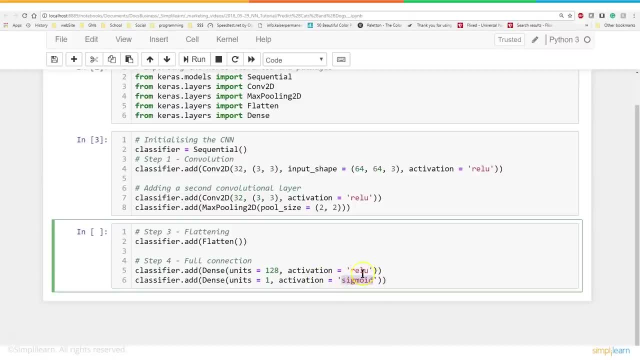 And then we use the sigmoid activation. If you remember from before, we had the R-E-L-U and there's also the sigmoid. The sigmoid just makes it clear It's yes or no. We don't want any kind of in-between number coming out. 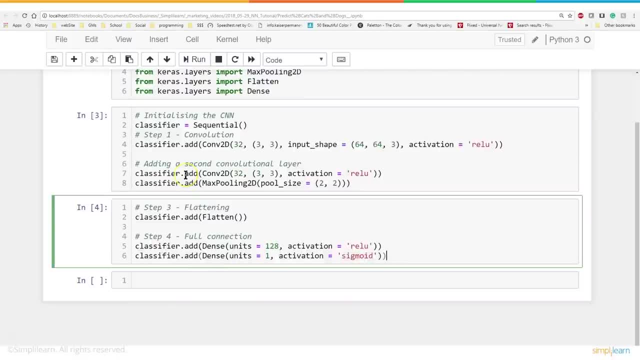 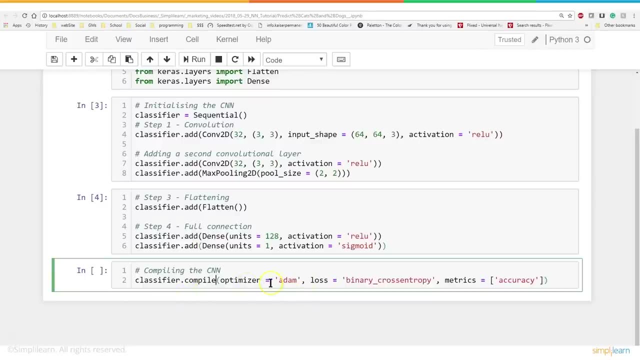 And we'll go ahead and run this And you'll see it's still all in setup. And then, finally, we want to go ahead and compile And let's put the compiling, our classifier neural network, And we're going to use the optimizer. 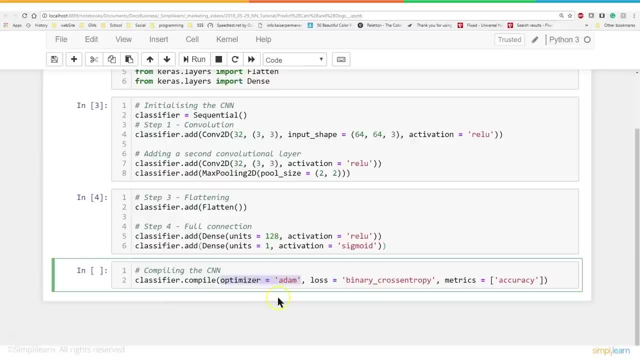 Atom, And I hinted at this just a little bit before. Where does Atom come in? Where does an optimizer come in? Well, the optimizer is the reverse propagation. When we're training it, it goes all the way through and says error. 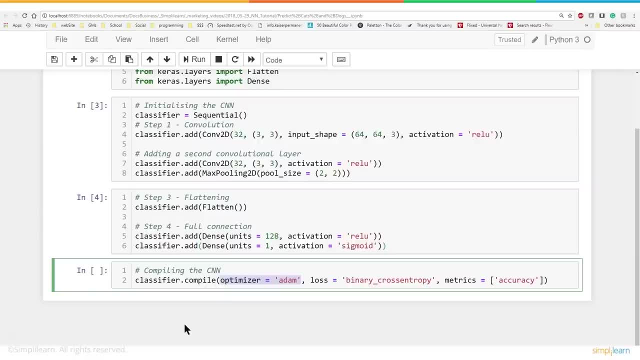 And then how does it readjust those weights? There are a number of them. Atom is the most commonly used And it works best on large data. Most people stick with the Atom because when they're testing on smaller data, see if their model is going to go through and get all their errors out before they run it on larger data. 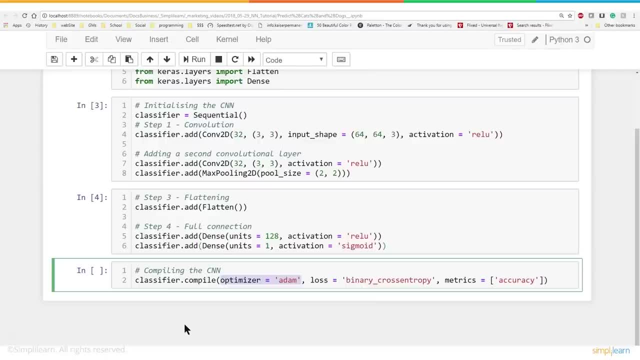 They're going to run it on Atom anyway, so they just leave it on Atom, most commonly used. But there are some other ones out there. You should be aware of that that. you might try them if you're stuck in a bind or you. 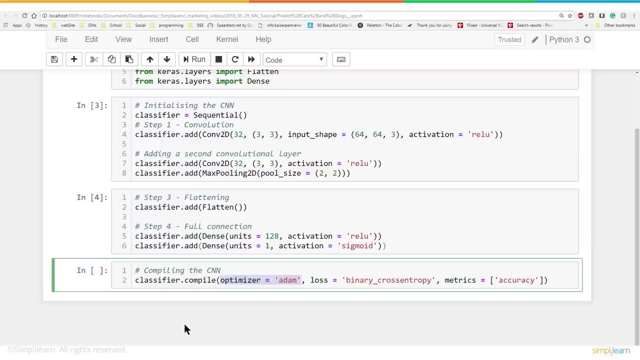 might floor that in the future, But usually Atom is just fine on there. And then you have two more settings. You have loss and metrics. We're not going to dig too much into loss or metrics. These are things you really have to explore cross because there are so many choices. 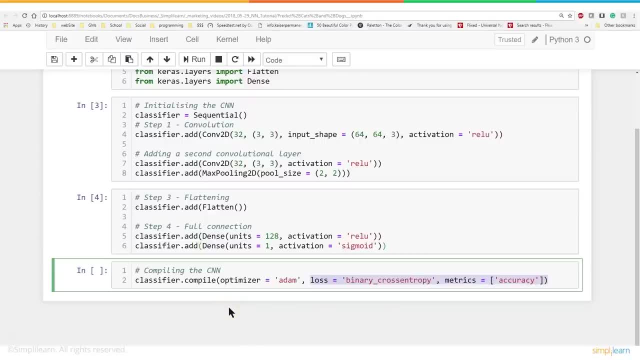 This is how it computes the error. There's so many different ways to on your back propagation and your training, So we're using this. We're using the Atom model, but you can compute the error by standard deviation. standard deviation squared. They use binary cross entropy. 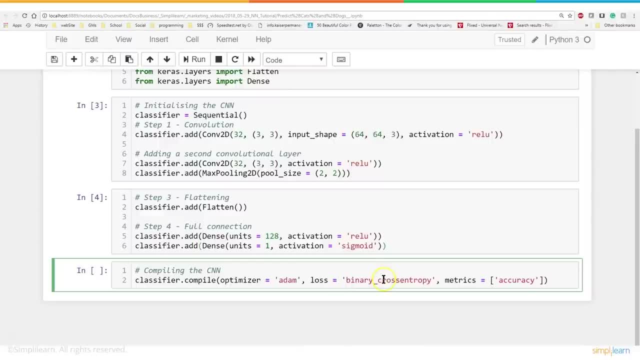 I'd have to look that up to even know what that is. There's so many of these. A lot of times you just start with the ones that look correct, that are most commonly used, and then you have to go read the Keras site and actually see what these different. 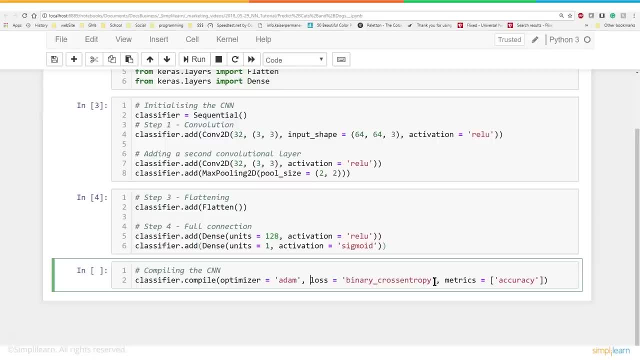 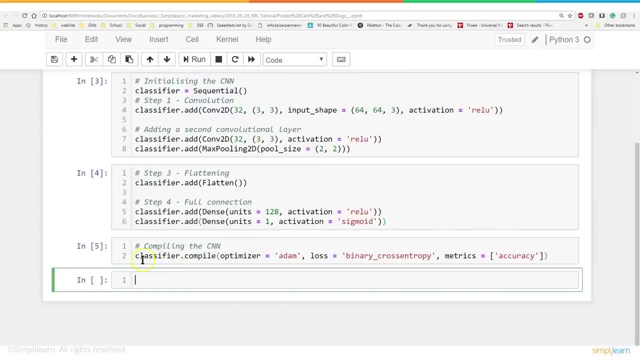 losses and metrics and what different options they have. So we're not going to get too much into them, other than to reference you over to the Keras website to explore them deeper. But we are going to go ahead and run them, And now we've set up our classifier. 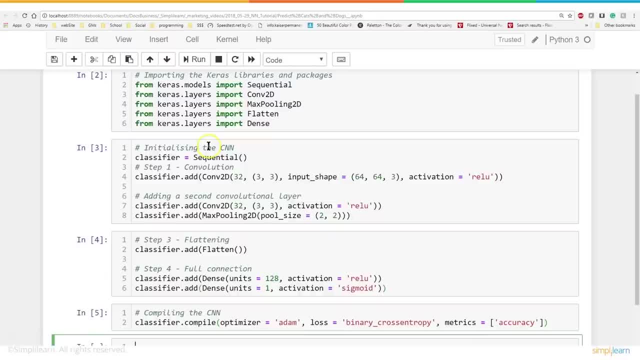 So we have an object classifier And if you go back up here you'll see that we've added in step one. we added in our layer for the input. We added a layer that comes in there and uses the RELU for activation. 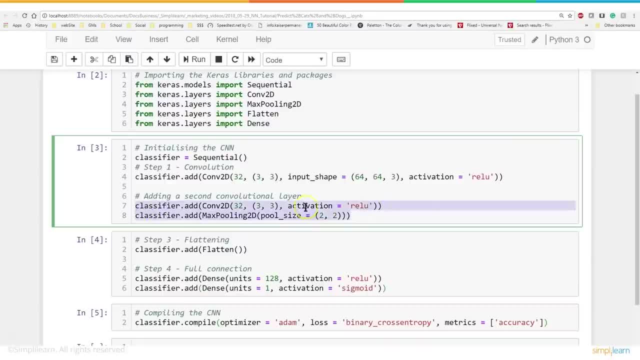 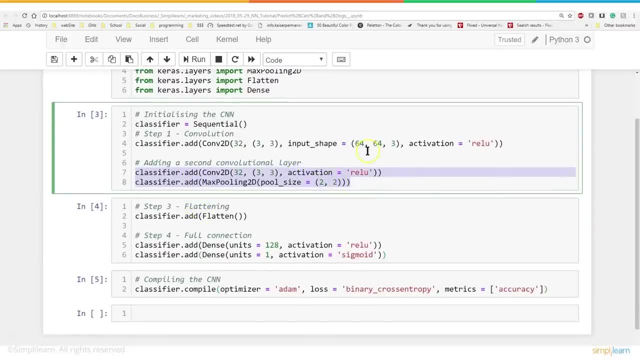 And then it pulls the data. So this is even though these are two layers- the actual neural network layer is up here- and then it uses this to pull the data into a two by two, So into a two dimensional array, from a three dimensional array with the colors. 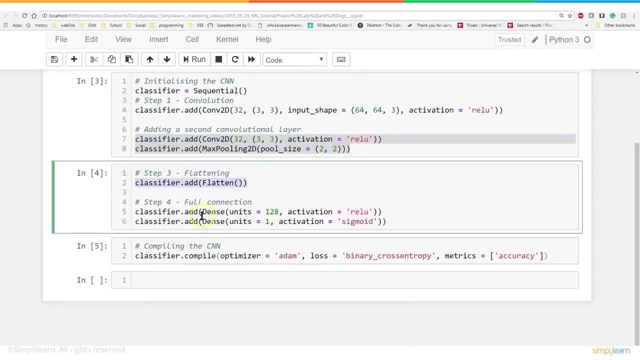 Then we flatten it. So there's our add or flatten And then we add another dense, what they call dense layer. This dense layer goes in there and it downsizes it to 128. It reduces it. So you can look at this as we're mapping all this data down, the two dimensional setup. 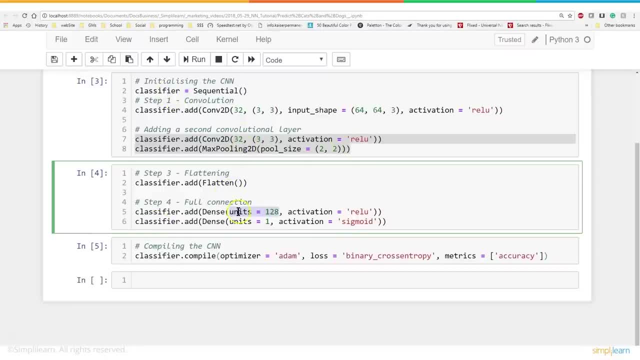 And then we flatten it, So we map it to a flatten map, And then we take it and reduce it down to 128. And we use the RELU again And then finally, we reduce that down to just a single output And we use the sigmoid to do that, to figure out whether it's yes, no, true, false. 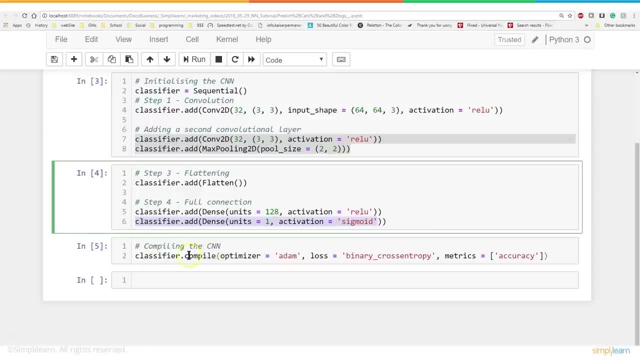 In this case, cat or dog, And then finally, once we put all these layers together, we compile them. That's what we've done here, And we've compiled them as far as how it trains to use these settings for the training back. 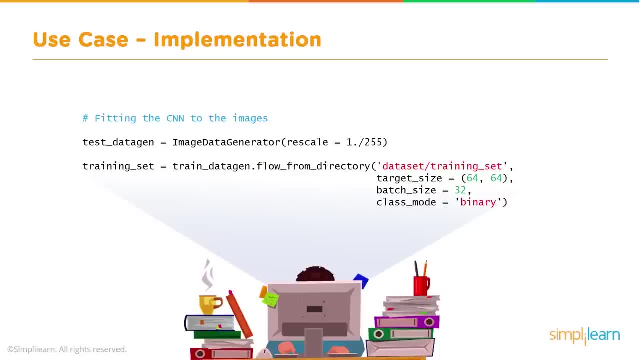 propagation. So, if you remember, we talked about training our setup And when we go into this, you'll see that we have two data sets. We have one called the training set and the testing set, And that's very standard in any data processing is you need to have? that's pretty common. 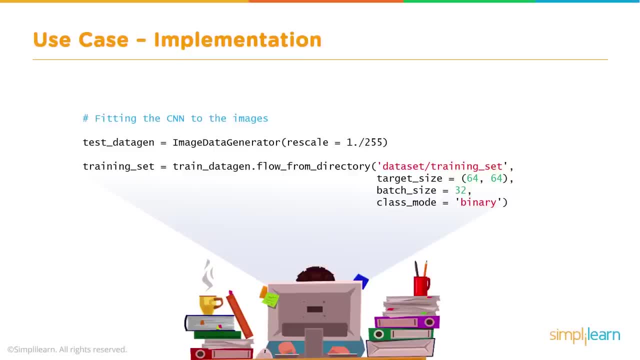 in any data processing. is you need to have a certain set, And that's pretty common in any data processing. is you need to have a certain set, And that's pretty common in any data processing. is you need to have a certain set, And that's pretty common in any data processing. is you need to have a certain amount of data? 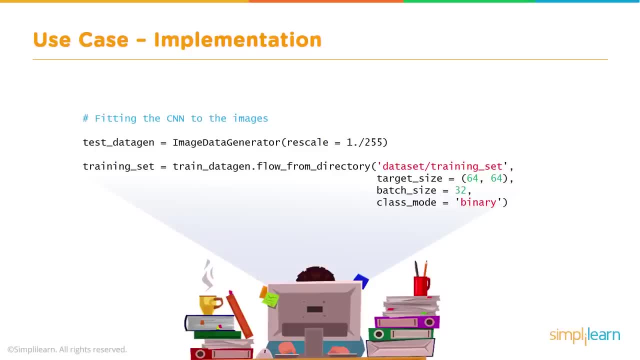 to train it, And then you've got to know whether it works or not. Is it any good? And that's why you have a separate set of data for testing it, where you already know the answer, but you don't want to use that as part of the training set. 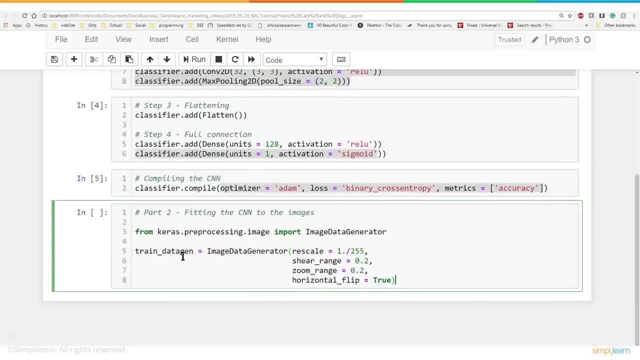 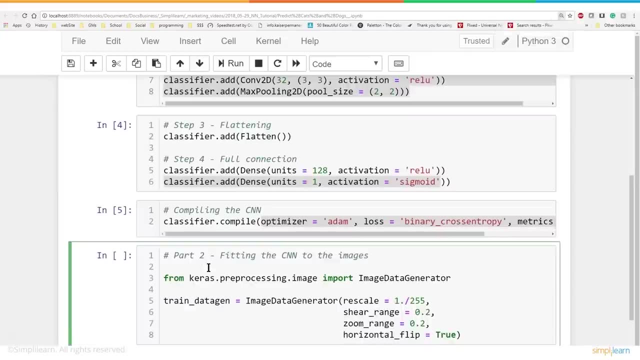 So in here we jump into part two, fitting the classifier neural network to the images. And then from Keras, let me just zoom in there. I always love that about working with Jupyter Notebooks. You can really see We're going to come in here. 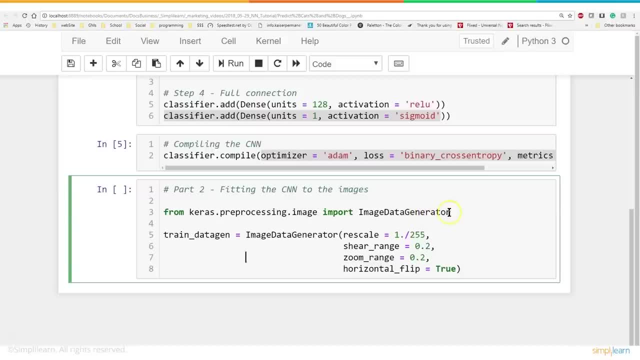 We do the Keras pre-processing an image and we import image data generator. So nice of Keras. It's such a high-end product right now going out and since images are so common, they already have all this stuff to help us process the data, which is great. 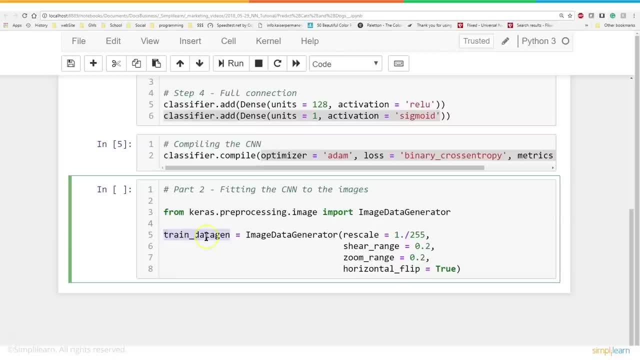 And so we come in here, We do train data gen and we're going to create our object for helping us train it, for reshaping the data so that it's going to work with our setup, And we use an image data generator and we're going to rescale it. and you'll see, here we 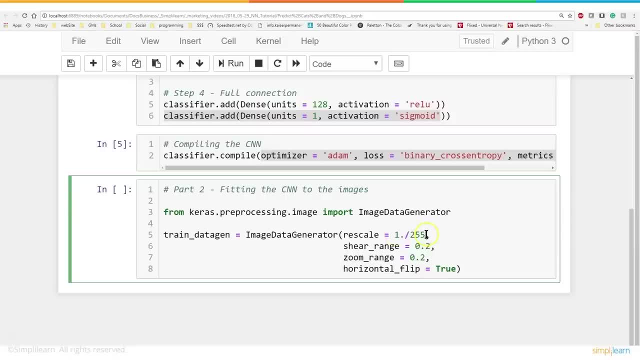 have one point which tells us it's a float value on the rescale over 255.. Where does 255 come from? Well, that's the scale in the colors of the pictures. we're using their value from 0 to 255.. 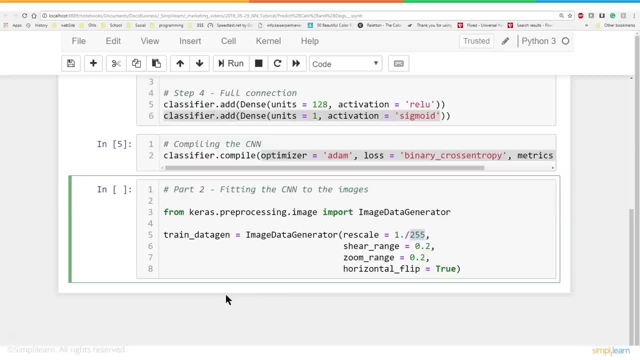 So we want to divide it by 255, and it'll generate a number between 0 and 1.. They have shear range and zoom range. horizontal flip equals true, and this of course has to do with if the photos are different shapes and sizes. 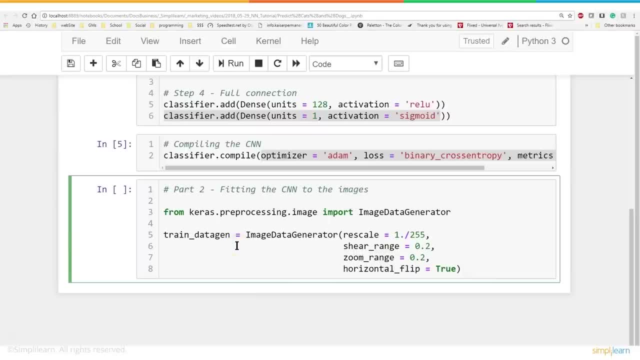 Like I said, it's a wonderful package. You really need to dig in deep to see all the different options you have for setting up your images. For right now, though, we're going to just stick with some basic stuff here and let. 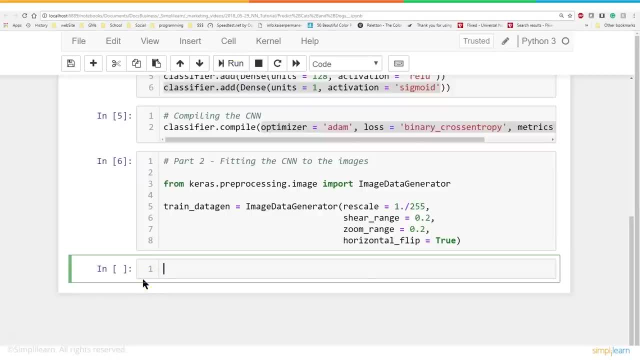 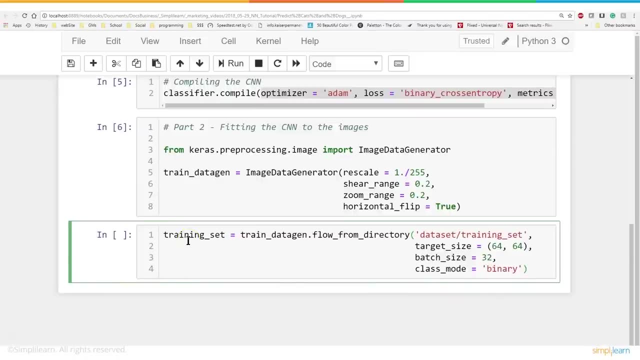 me go ahead and run this code And again it doesn't really do anything because we're still setting up the pre-processing. Let's take a look at this next set of code, and this one is just huge. We're creating the training set. 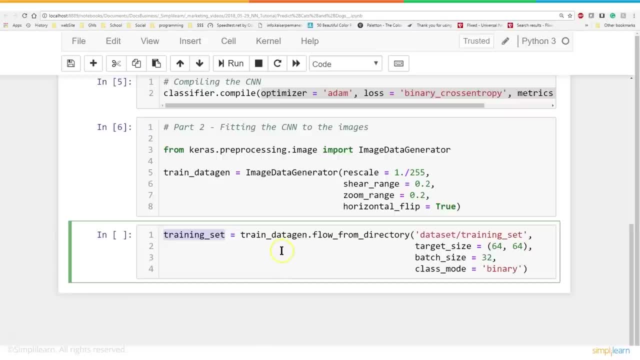 So the training set is going to go in here and it's going to use our train data gen. we just created flow from directory. It's going to access, in this case, the path data set: training set. That's a folder. 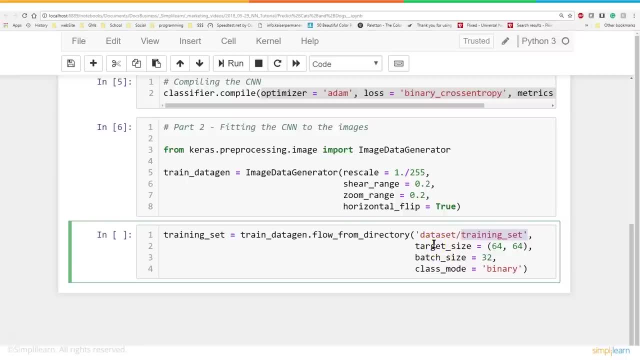 So it's going to pull all the images out of that folder. Now I'm actually running this flow from directory. It's a folder that the data sets in. So if you're doing the same setup and you load your data in there and you're doing 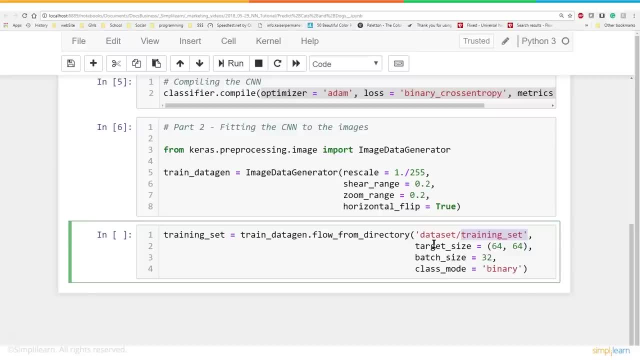 this: make sure, wherever your Jupyter notebook is saving things to, that you create this path, or you can do the complete path if you need to. you know C, colon slash, et cetera. And the target size, the batch size and class mode is binary. 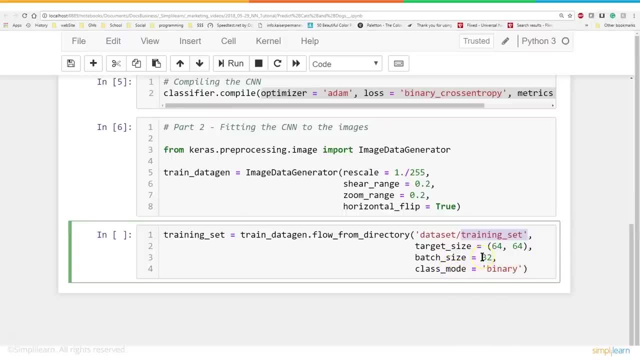 So the class is: we're switching everything to a binary value: Batch size. what the heck is batch size? Well, that's how many pictures we're going to batch through the training each time, And the target size 64.. 64 by 64, a little confusing, but you can see right here that this is just a general. 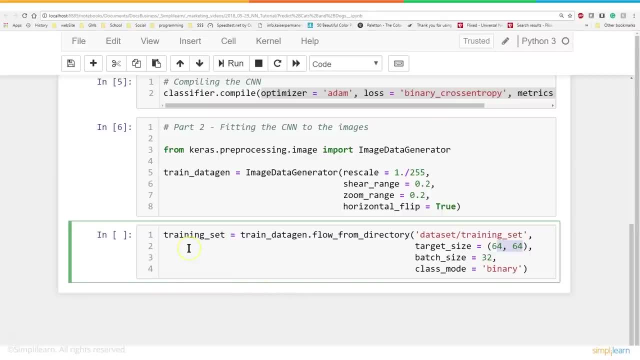 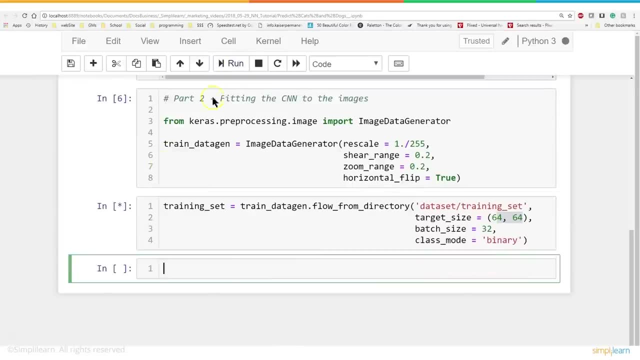 training And you can go in there and look at all the different settings for your training set And, of course, with different data, we're doing pictures. There's all kinds of different settings depending on what you're working with. Let's go ahead and run that and see what happens. 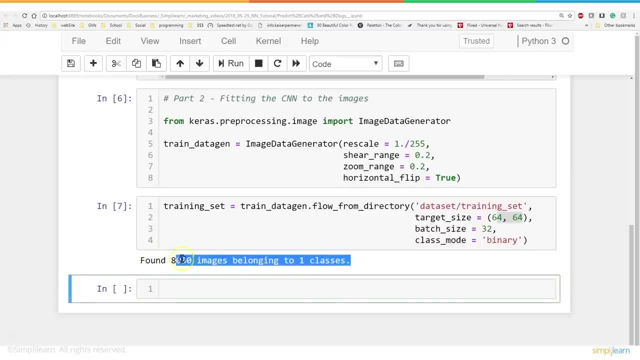 And you'll see that it found 800 images belonging to one classes. So we have 800 images in the training set And if we're going to do this with the training set, we also have to format the pictures in the test set. 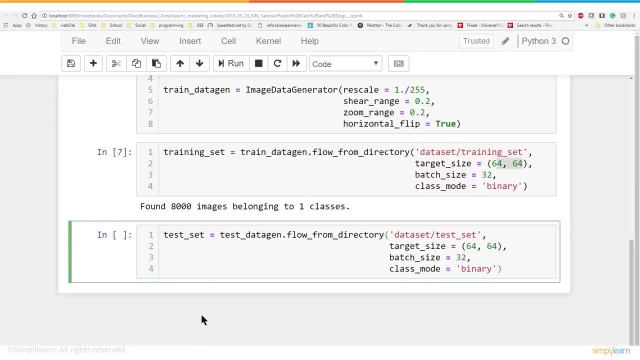 Now we're not actually doing any predictions, We're not actually programming the model yet. All we're doing is preparing the data. So we're going to prepare a training set and the test set. So any changes we make to the training set at this point also have to be made to the 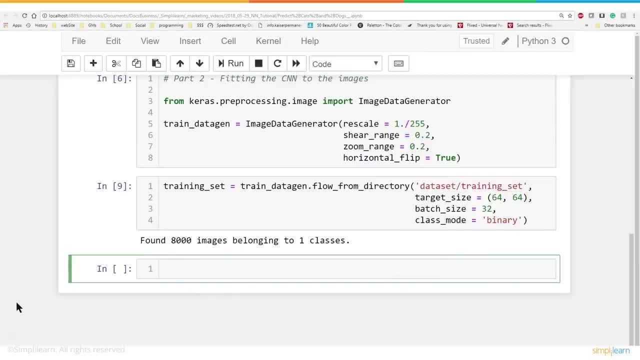 test set. So we've done this thing where we've done a train data generator, We've done our training set, And then we also have- remember- our test set of data. So I'm going to do the same thing with that. 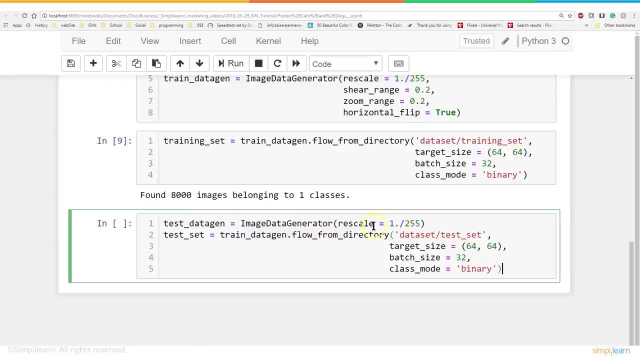 I'm going to create a test data gen And we're going to do this image data generator. Run that test. we're going to rescale 1 over 255.. We don't need the other settings, just the single setting for the test data gen And we're going to create our test set. We're going to do the same thing we did. 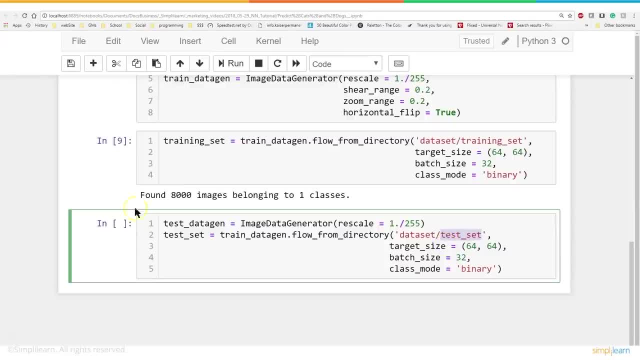 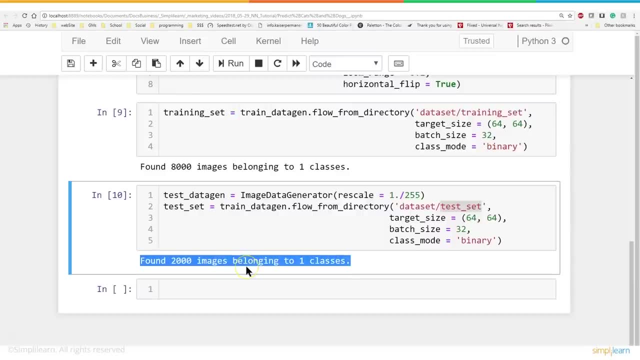 with the test set, except that we're pulling it from the test set folder And we'll run that and you'll see, in our test set we found 2,000 images. That's about right. We're using 20% of the images as test and 80% to train it, And then, finally, we've set up all our data. 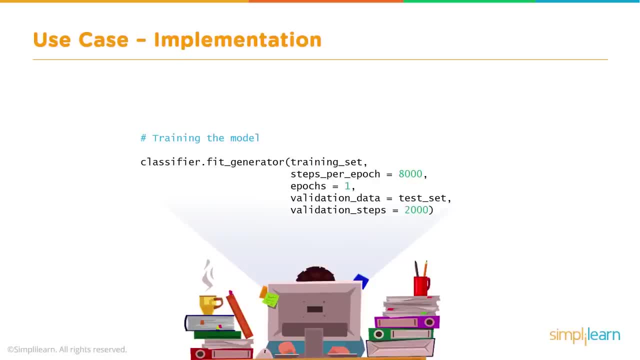 We've set up all our layers, which is where all the work is is cleaning up that data and making sure it's going in there correctly And we're actually going to fit it. We're going to train our data set And let's see what that looks like. And here we go, Let's put the information in here. 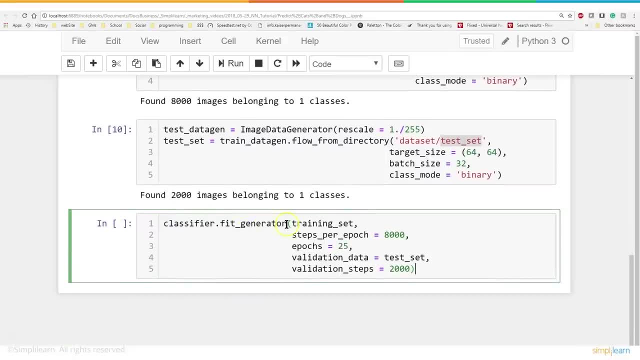 And let's just take a quick look at what we're looking at with our fit generator. We have our classifierfit generator, That's our back propagation. So the information goes through forward with a picture And it says: oh, you're either right or you're wrong. And then the 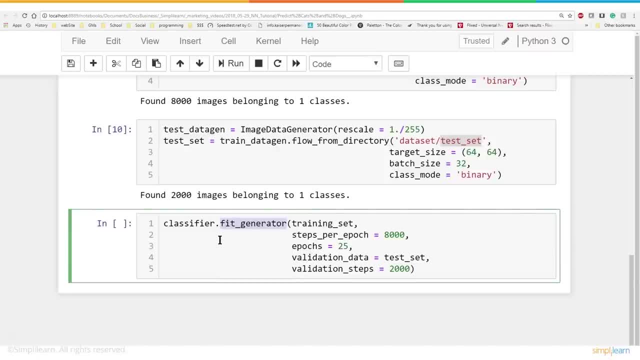 error is going to be the error, And then the error is going to be the error. And then the error goes through forward with a picture And it says, oh, you're either right or you're wrong. And then the error goes backward and reprograms all those weights. So we're training our neural network And of 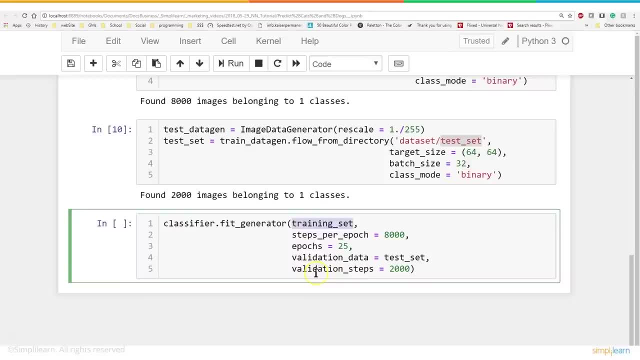 course we're using the training set- Remember, we created the training set up here- And then we're going steps per epic. So it's 8,000 steps. Epic means that that's how many times we go through all the pictures. So we're going to rerun each of the pictures And we're going to go. 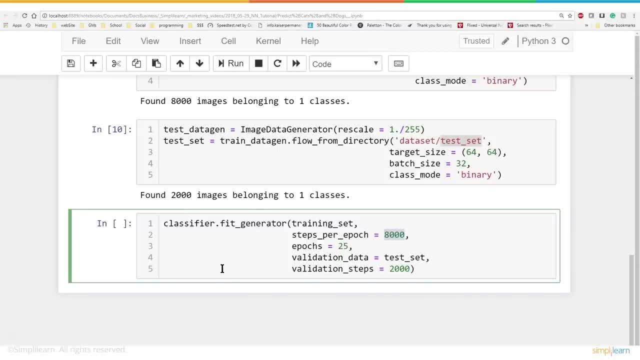 through the whole data set 25 times, But we're going to look at each picture during each epic 8,000 times, So we're really programming the heck out of this and going back and forth back over it. And then they have validation data equals test set. So we have our training set. 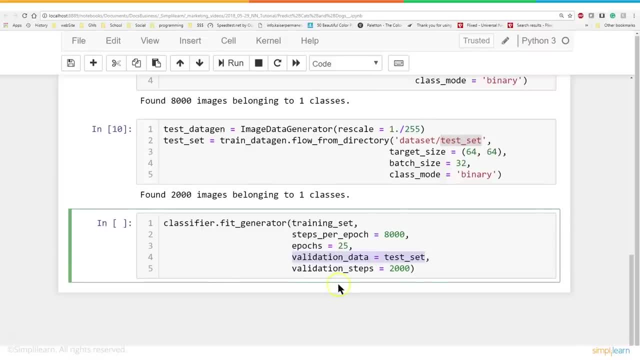 And then we're going to have our test set to validate it. So we're going to do this all in one shot And we're going to look at that, And they're going to do 200 steps for each validation And we'll see what that looks like in just a minute. Let's go ahead and run our training here. 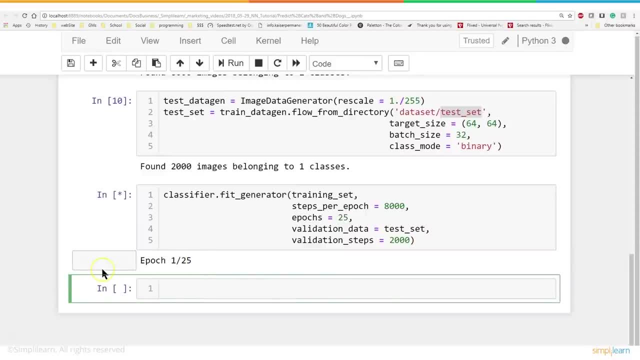 And we're going to fit our data And as it goes, it says epic 1 of 25.. You start realizing that this is going to take a while. On my older computer it takes about 45 minutes. I have a dual. 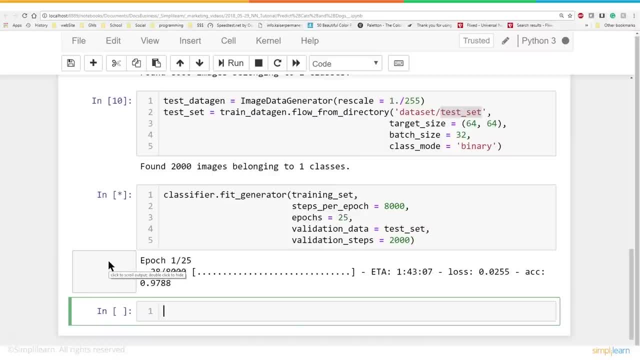 processor And we're processing 10,000 photos. That's not a small amount of photographs to process. So if you're on your laptop, which I am, it's going to take a while. So let's go ahead and go get our cup of coffee and a sip, And we'll come back and see what this looks like. 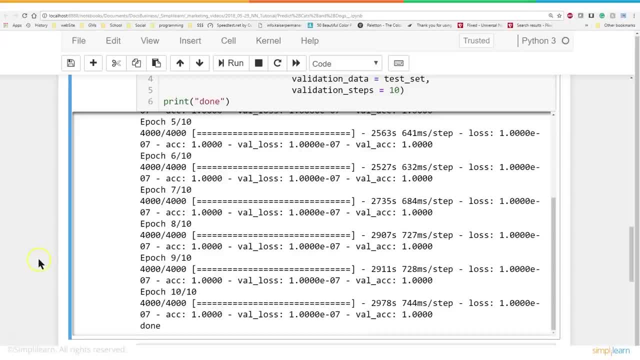 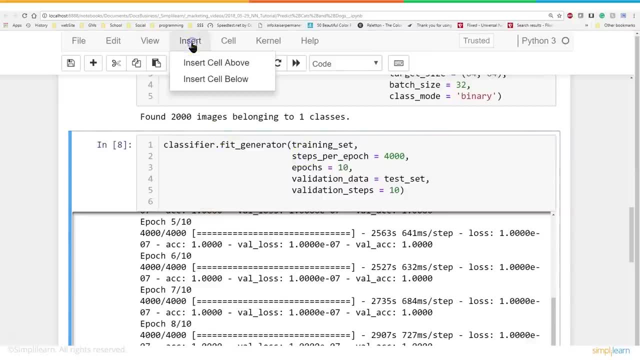 So I'm back. You didn't know I was gone. I was actually a lengthy pause there. I made a couple changes And let's discuss those changes real quick and why I made them. So the first thing I'm going to do is I'm going to go up here and insert a cell above And let's paste the original. 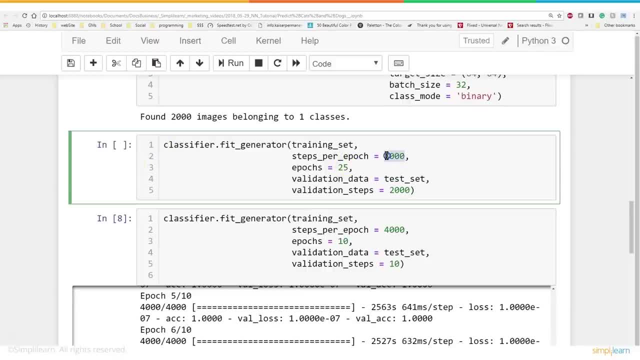 code back in there And you'll see that the original thing was steps per epic: 8,000, 25 epics and validation steps 2,000.. And I changed these to 4,000 epics, or 4,000 steps per epic, 10 epics. 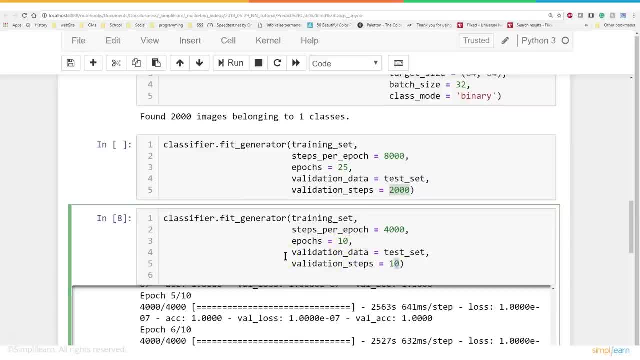 and just 10 validation steps, And this will cause problems if you're doing this as a commercial release, But for demo purposes, this should work. And if you remember our steps per epic, that's how many photos we're going to process. In fact. let me go ahead and get my drawing pen out And 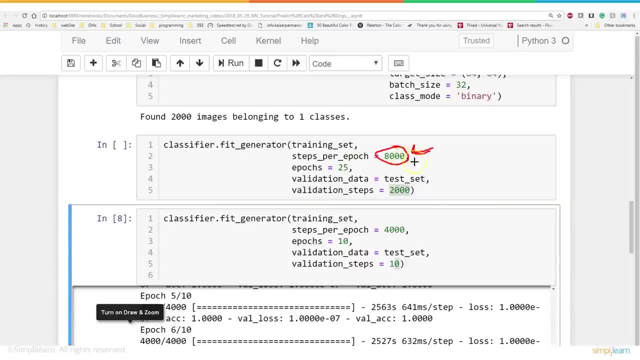 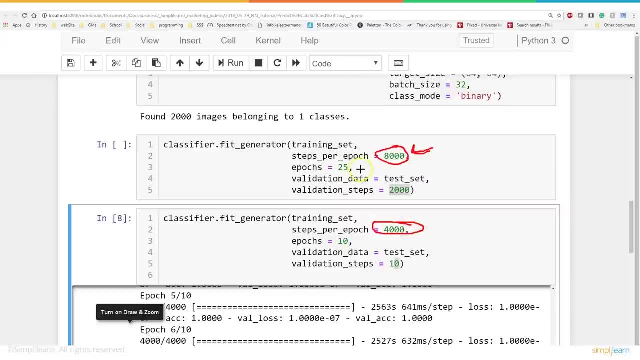 4,000 pictures each time it goes through an epic, And the epic is how many processes? So this is 25. And I'm just going to cut that to 10. So, instead of doing 25, runs through 8,000 photos each. 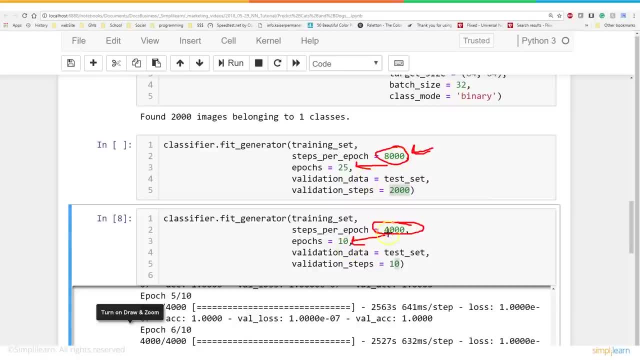 which you can do the math of 25 times 8,000, I'm only going to do 10 through 4,000.. So I'm going to run this 40,000 times through the processes And the next thing you'll want to notice is that I also changed the validation step And this would cause some 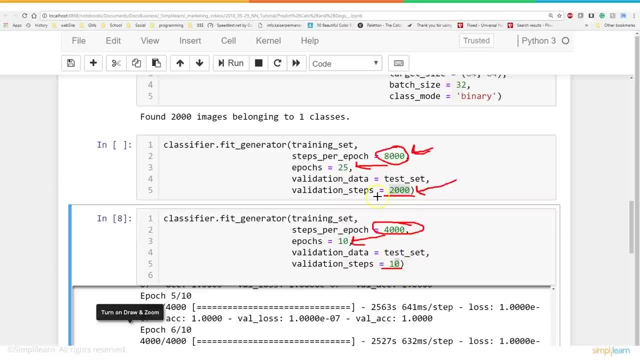 major problems in releasing because I dropped it all the way down to 10.. What the validation step does is: it says we have 2,000 photos in our trainings or in our testing set And we're going to use that for validation. Well, I'm only going to use a random 10 of those to validate. 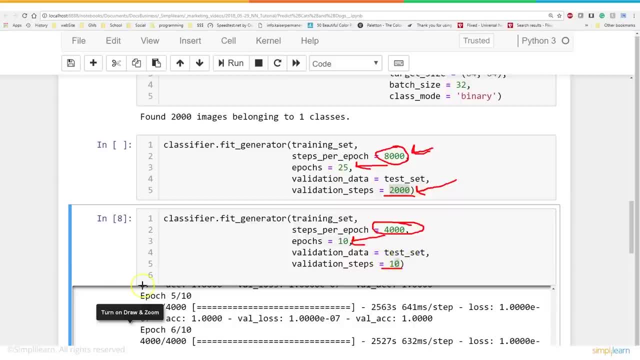 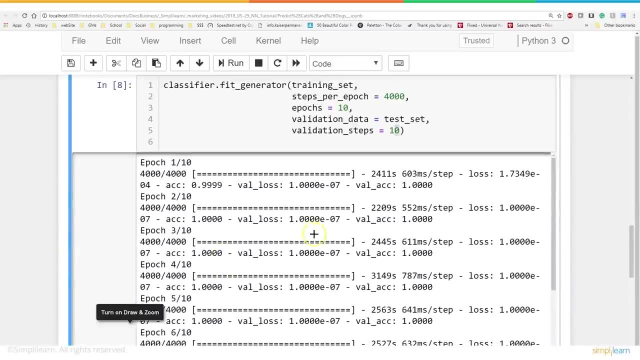 So not really the best settings, But let me show you why we did that. Let's scroll down here just a little bit And let's look at the output here and see what's going on there. So I've got my drawing tool back on And you'll see here it lists a run. So each time it goes through an epic. 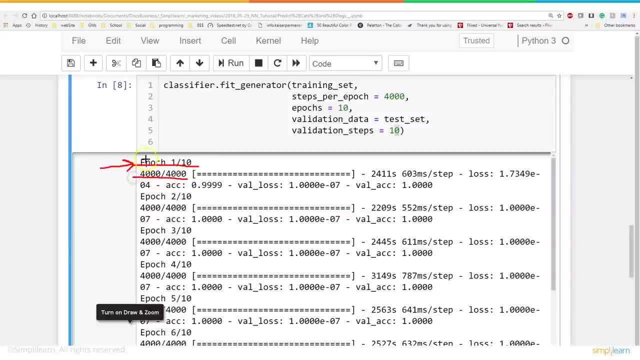 it's going to do 4,000 steps And this is where the 4,000 comes in. So that's where we have. We have epic 1 of 10, 4,000 steps. So it's randomly picking half the pictures in the file and going. 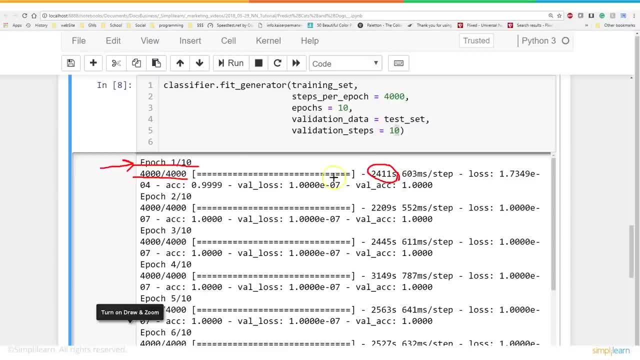 through them And then we're going to look at this number right here. That is for the whole epic And that's 2,411 seconds And if you remember correctly, you divide that by 60, you get minutes. If you divide that by 60,, you get hours, Or you can just divide the whole thing. 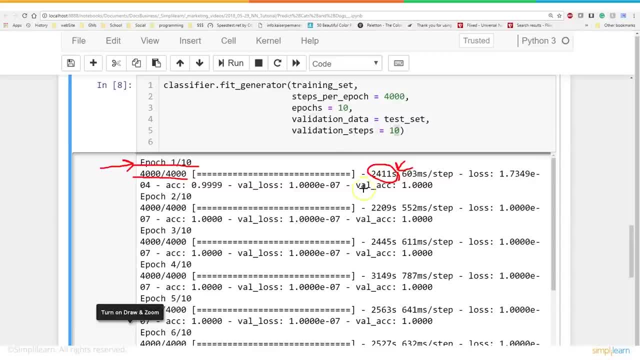 By 60 times 60, which is 3,600.. If 3,600 is an hour, this is roughly 45 minutes right here And that's 45 minutes to process half the pictures. So if I was doing all the pictures, 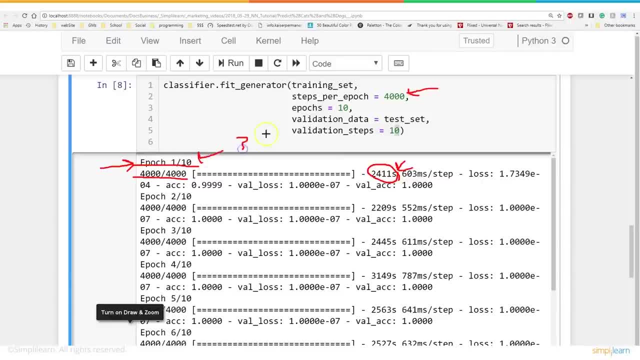 we're talking an hour and a half per epic times 36. Or no 25. They had 25 up above 25.. So that's roughly a couple days, A couple days of processing. Well, for this demo. we don't want to do that. I. 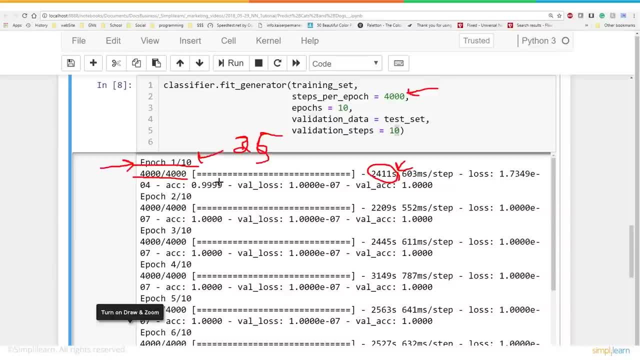 don't want to come back the next day. Plus, my computer did a reboot in the middle of the night. So we look at the output And we're going to look at the output, And we're going to look at the output And we're going to look at this And we say, okay, we're just testing this out. My 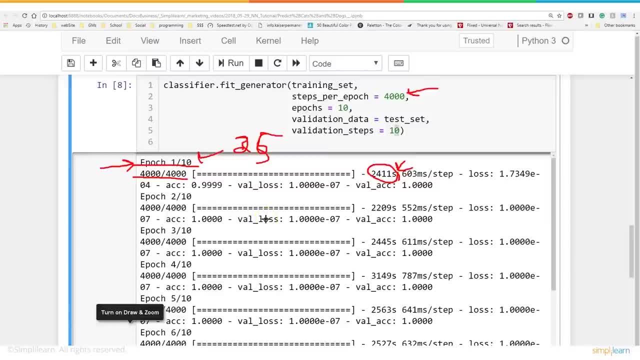 computer that I'm running this on is a dual core processor. It runs 0.9 gigahertz per second. For a laptop it was good about four years ago, But for running something like this it's probably a little slow. So we cut the times down, And the last one was validation. We're only validating. 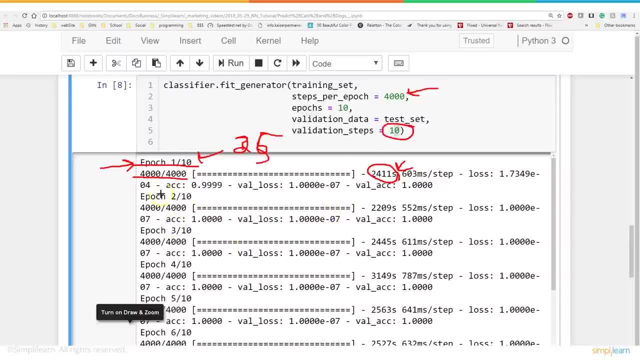 it on a random 10 photos. And this comes into effect Because you're going to see down here where we have accuracy, value, loss, value, accuracy and loss. Those are very important numbers to look at. So the 10 means I'm only validating across 10 pictures. That is where 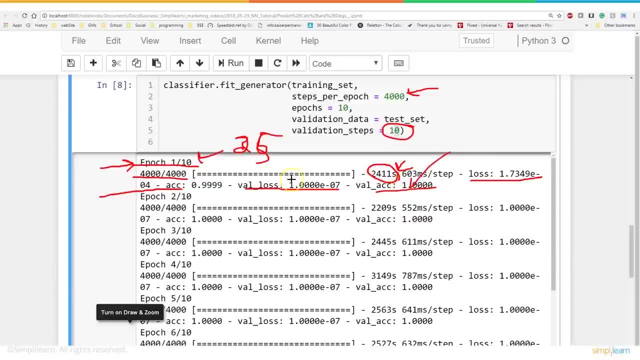 here we have value. This is ACC is for accuracy, Value loss. we're not going to worry about that too much. And accuracy Now, accuracy is while it's running. it's putting these two numbers together. That's what accuracy is And value accuracy is at the end of the epic. What's our? 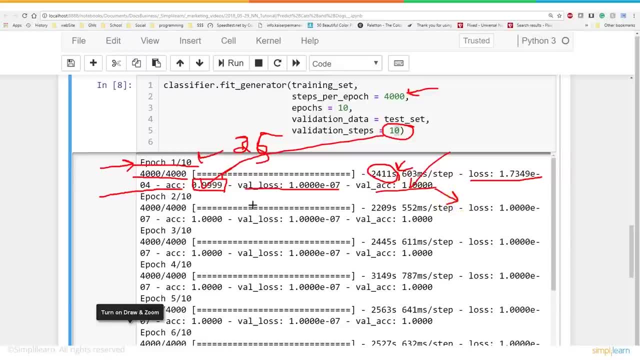 accuracy. end of the epic. What is it looking at? In this tutorial? we're not going to go so deep, But these numbers are really important. when you start talking about these two, these two numbers reflect bias. That is really important. Let me just put that up there. 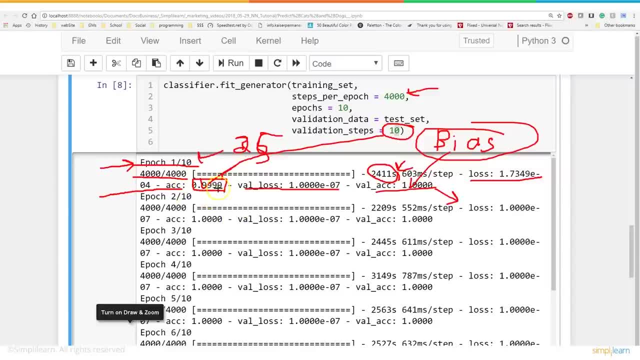 And bias is a little bit beyond this tutorial, But the short of it is is: if this accuracy, which is being our validation per step, is going down and the value accuracy continues to go up, that means there's a bias. That means I'm memorizing the photos, I'm looking 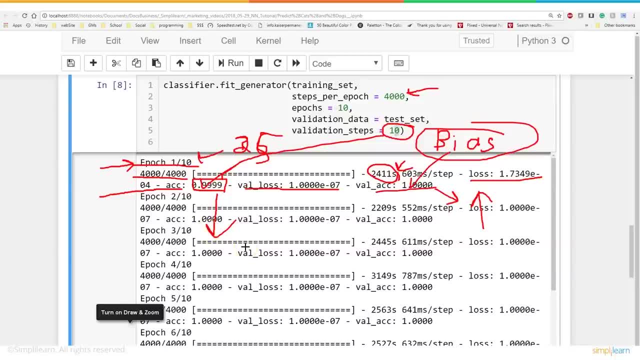 at. I'm not actually looking for what makes a dog a dog, what makes a cat a cat, I'm just memorizing them, And so the more this discrepancy grows, the more I'm going to be able to see the photos, the bigger the bias is, And that is really the beauty of the cross neural network. 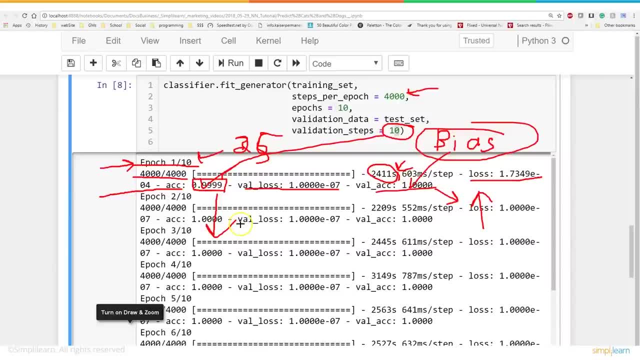 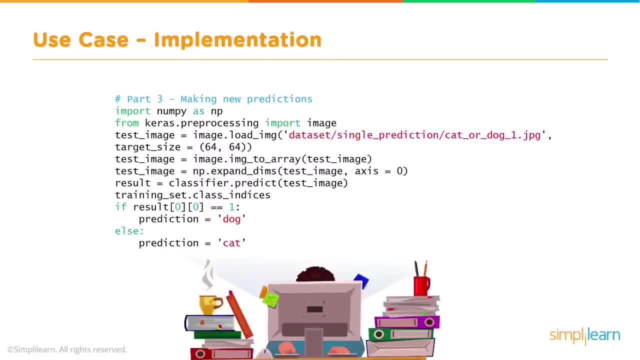 It has a lot of built-in features like this that make that really easy to track. So let's go ahead and take a look at the next set of code. So here we are into part three. We're going to make a new prediction, And so we're going to bring in a couple tools for that. 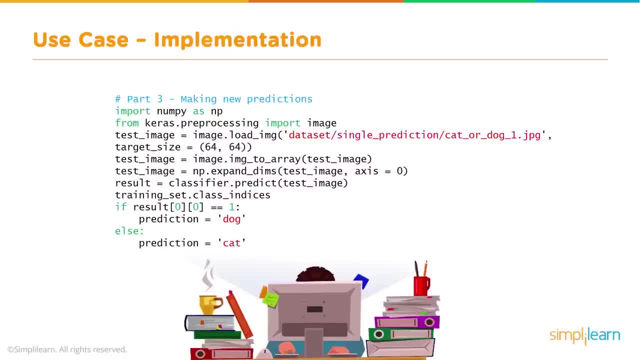 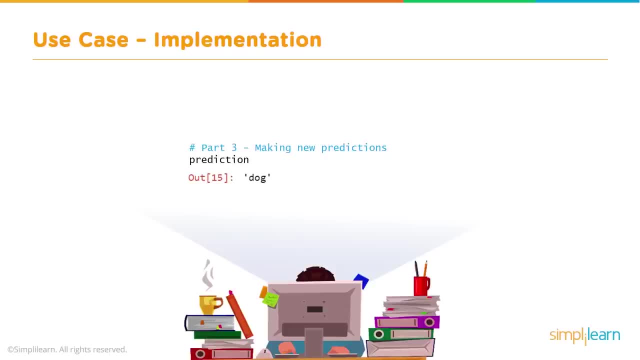 And then we have to process the image coming in and find out whether it's an actual dog or cat. We can actually use this to identify it. And of course, the final step of part three is to print predictors. We'll go ahead and combine these And of course you can see me there adding a more sticky. 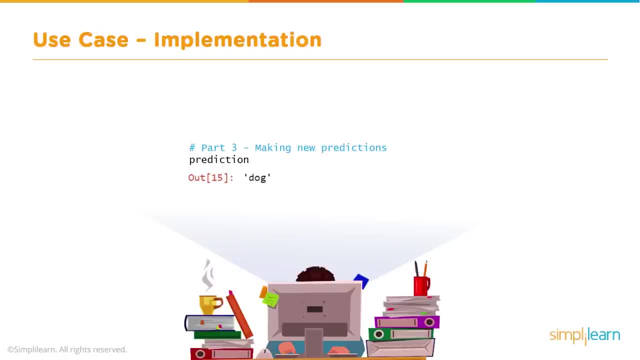 nose to my computer screen hidden behind the screen. And the last one was: don't forget to feed the cat and the dog. So let's go ahead and take a look at that and see what that looks like in code and put that in our Jupyter notebook. All right, And let's paste that. 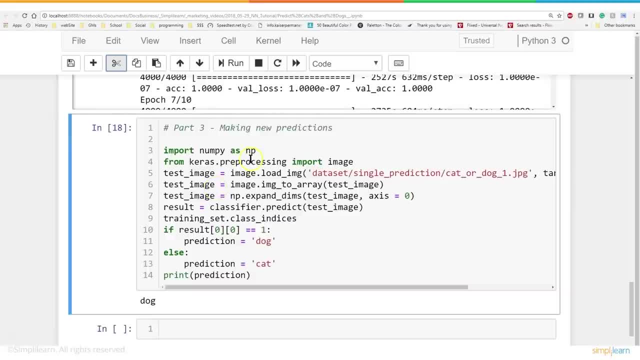 in here And we'll start by importing numpy. as np Numpy is a very common package. I pretty much import it on any Python project I'm working on. Another one I use regularly is pandas. They're just ways of organizing the data. 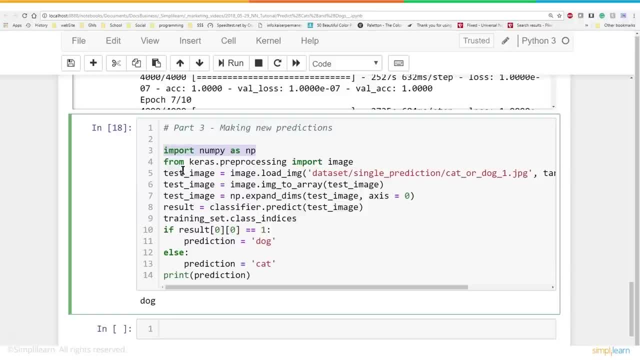 And then np is usually the standard in most machine learning tools as a return for the data array, Although you know you can use the standard data array from Python- And we have cross pre-processing import image. This should all look familiar because we're 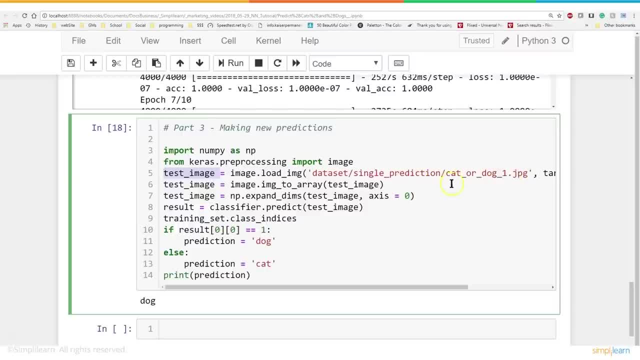 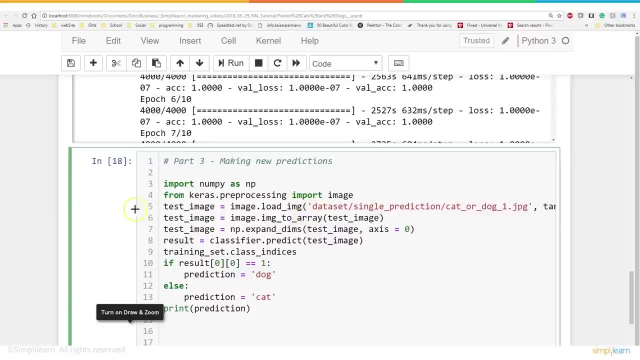 going to take a test image and we're going to set that equal to, in this case, cat or dog one, as you can see over here- And you know, let me get my drawing tool back on. So let's take a look at this. We have our test image, we're loading And in here we have 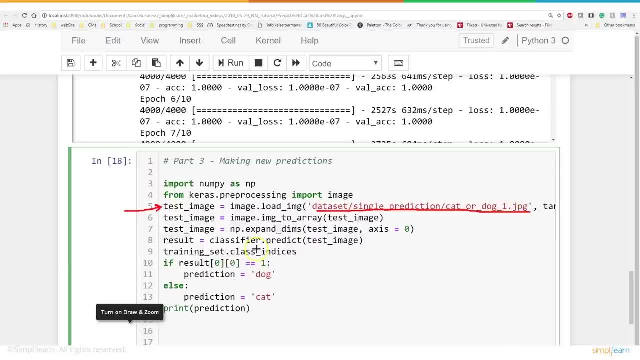 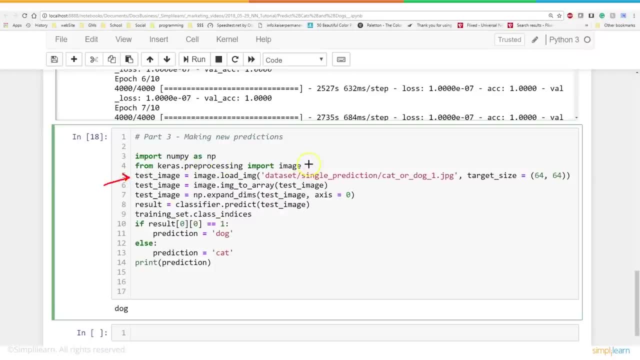 test image one, And this one hasn't data, hasn't seen this one at all. So this is all new. Oh, let me shrink the screen down. Let me start that over. So here we have my test image And we went ahead, and the cross-processing has this nice. 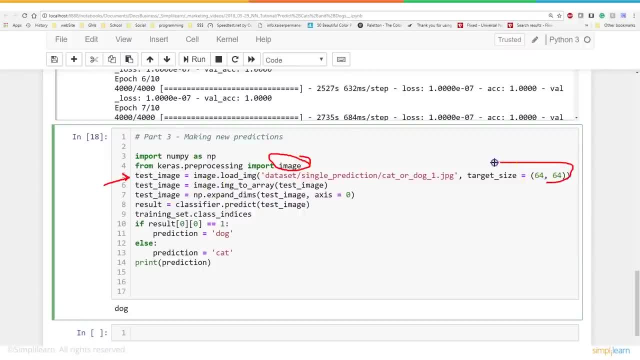 image setup. So we're going to load the image and we're going to alter it to 64 by 64 print. So right off the bat we're going to cross is nice that way. It automatically sets it up for us so we don't have to redo all our images and find a way to reset those. 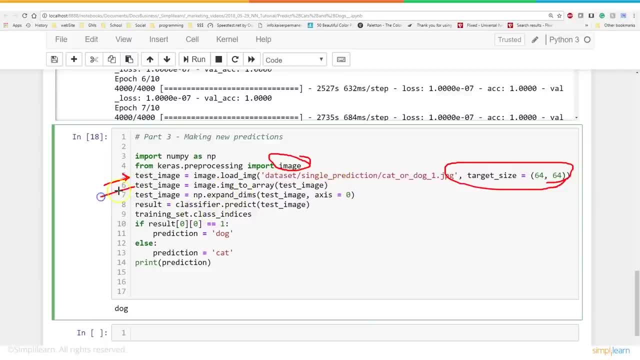 And then we use also to set the image to an array. So again we're all in pre-processing the data We pre-processed before with our test information and our training data, And then we use the NumPy. Here's our NumPy, that's from our right up here: import NumPy as in P. 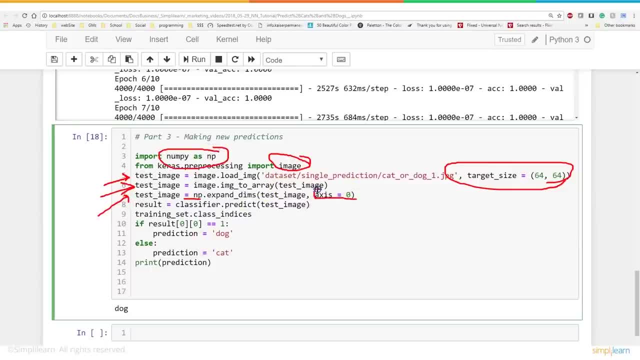 Expand the dimensions. test image: axis equals zero, So it puts it into a single array. And then, finally, all that work, all that pre-processing, and all we do is we run the result, We click on here and we go. result equals classifier: predict test image. 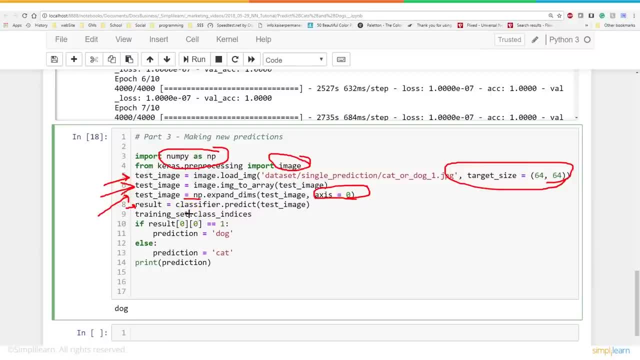 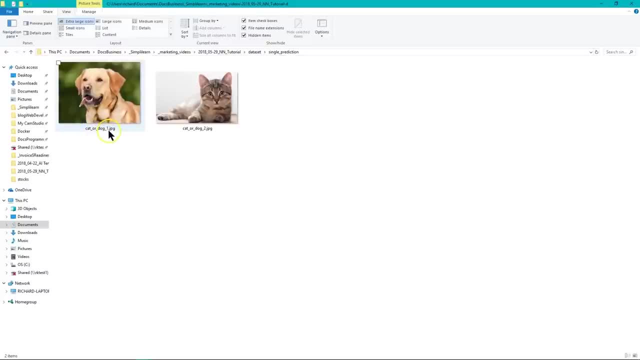 And then we find out: well, what is the test image? And let's just take a quick look and just see what that is. And you can see when I ran it it comes up dog. And if we look at those images there, it is cat or dog. image number one: 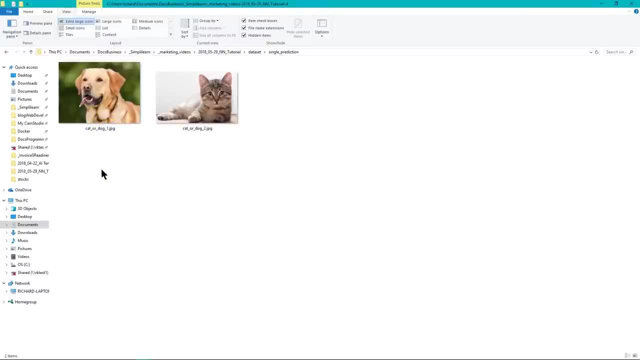 That looks like a nice floppy-eared lab, friendly, with his tongue hanging out. It's either that or a very floppy-eared cat, I'm not sure which, But according to our software it says it's a dog. And we have a second picture over here. 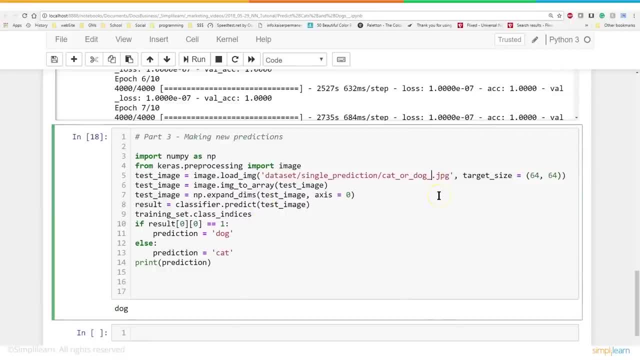 Let's just see what happens when we run the second picture. We can go up here and change this from dog image one to two. We'll run that And it comes down here and says cat. You can see me highlighting it down there as cat. 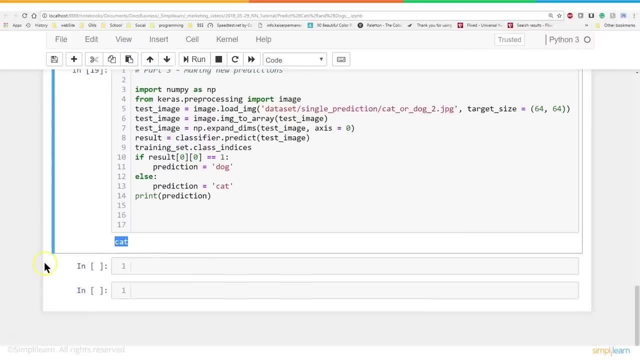 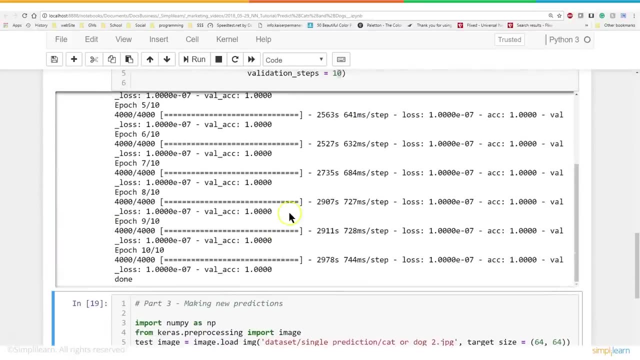 So our process works. We are able to label a dog a dog and a cat a cat just from the pictures. There we go, Cleared my drawing tool And the last thing I want you to notice when we come back up here to when I ran it, you'll. 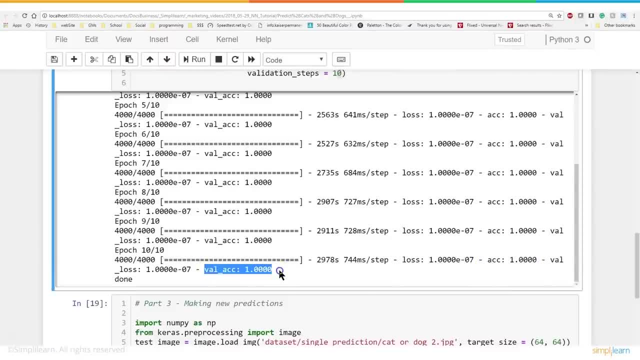 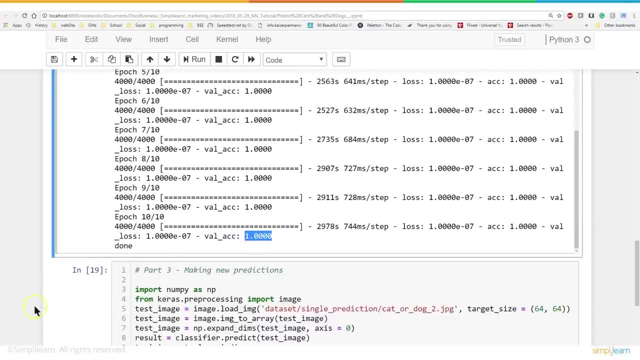 see, it has an accuracy of one and the value accuracy of one. Well, the value accuracy is the important one, because the value accuracy is what it actually runs on the test data. Remember, I'm only testing it on, I'm only validating it on a random ten photos. 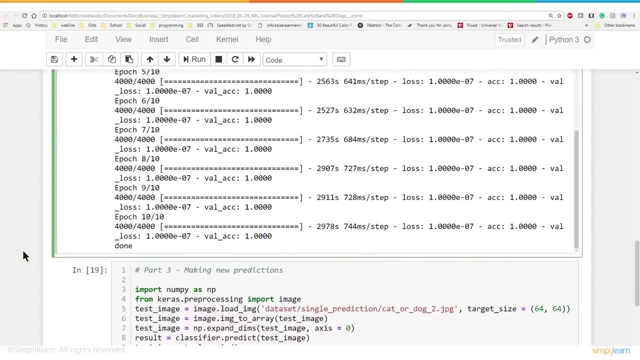 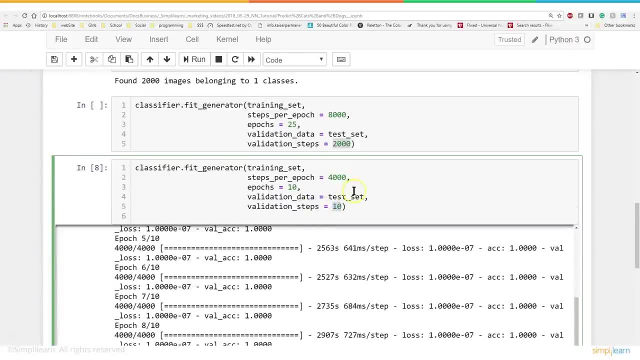 And those ten photos just happen to come up one. Now, when they ran this on the server, it actually came up about 86%. This is why cutting these numbers down so far for a commercial release is bad. So you want to make sure you're a little careful of that when you're testing your stuff. that 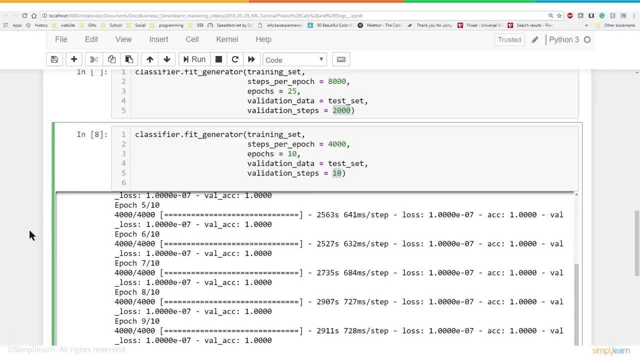 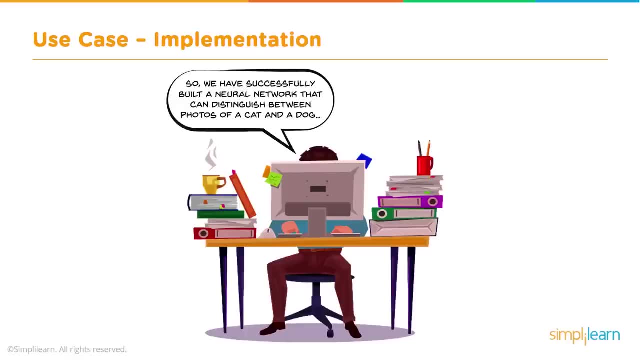 you change these numbers back when you run it on a more enterprise computer other than your old laptop that you're just practicing on or messing with, And we come down here and again. you know we had the validation of cat, And so we have successfully built a neural network that could distinguish between photos. 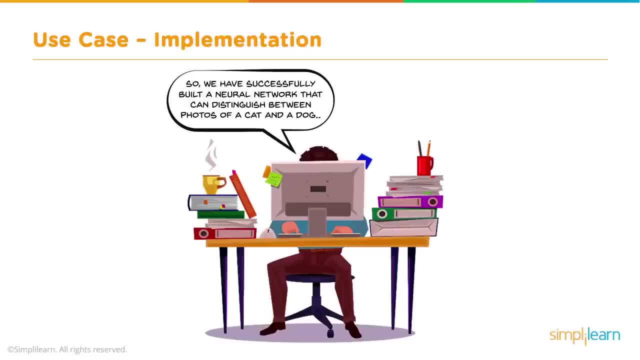 of a cat and a dog. Imagine all the other things You could distinguish. Imagine all the different industries you could dive into with that, Just being able to understand those two difference of pictures. What about mosquitoes? Could you find the mosquitoes that bite versus the mosquitoes that are friendly? 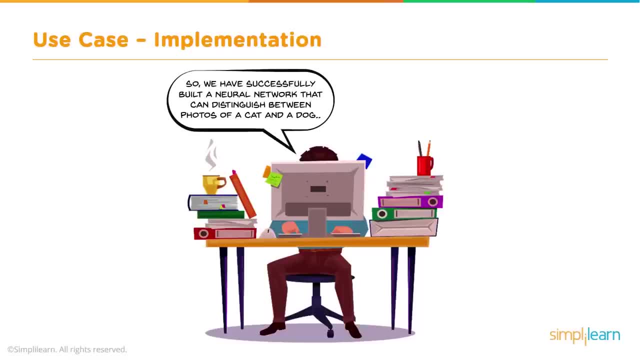 It turns out, the mosquitoes that bite us are only 4% of the mosquito population, if even that, maybe 2%. There's all kinds of industries that use this, and there's so many industries that are just now realizing how powerful these tools are. 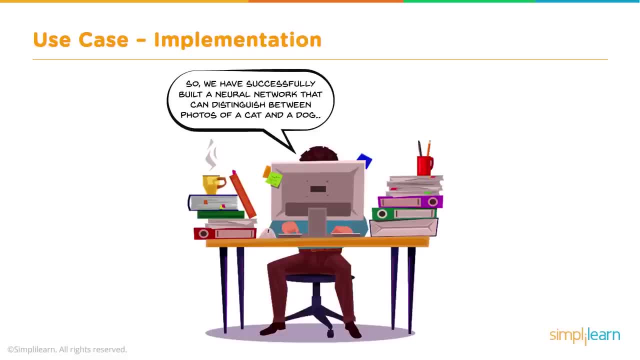 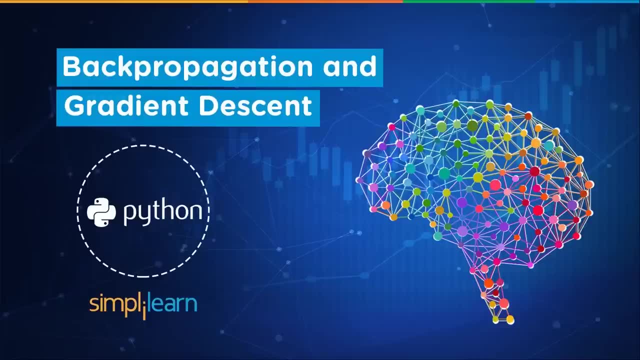 Just in the photos alone, there is a myriad of industries sprouting up. And I said it before, I'll say it again: What an exciting time to live in with these tools that we get to play with Back propagation and gradient descent. we're talking neural networks. 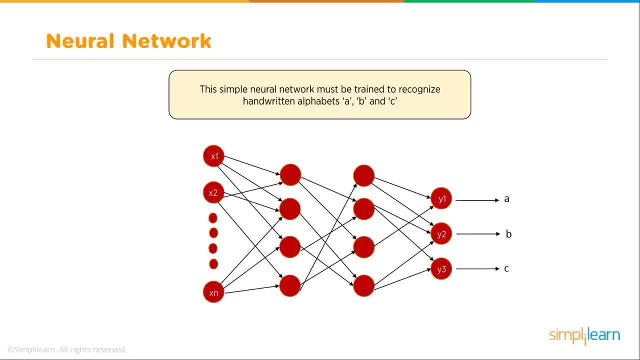 So we talk about the neural network. This is a simple neural network which must be trained to recognize handwritten alphabets A, B and C, And you can see, here we have our input coming in. In this case we'll look at the letter A written out on a 28 by 28 pixels. 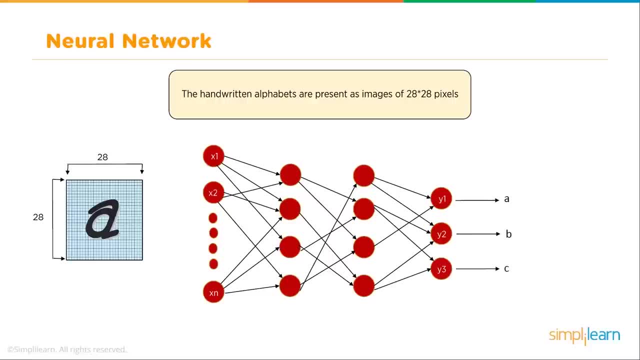 So the handwritten alphabets are presented as images of 28 by 28 pixels And that image comes in. In this case, we have 784 neurons, that's 28 times 28.. And the initial prediction is made using random weights assigned to each channel. 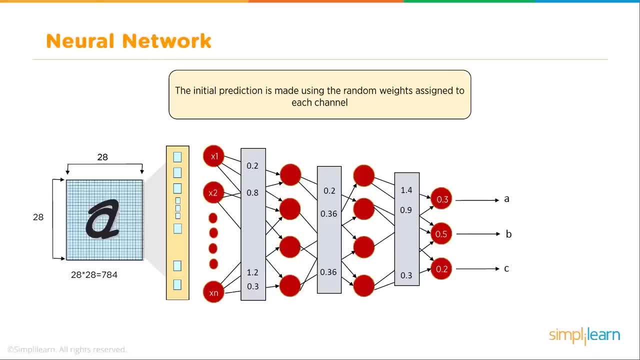 And so we have our forward propagation, as you see here. So each node is then- their values are added up, and added up and so on, going across, And our network predicts the input to be B, with a probability of 0.5. 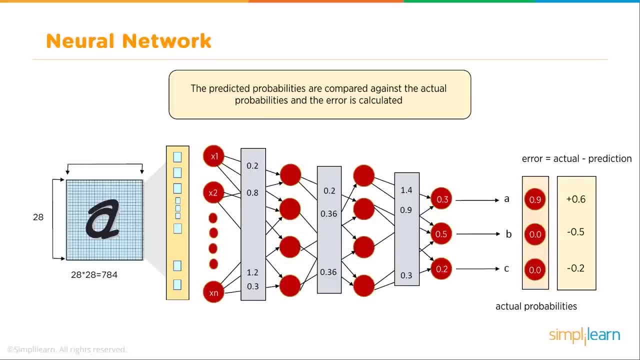 The predicted probabilities are compared against the actual probabilities and the errors calculated. So the error is simply the actual minus predicted, And you can see here where we know it's 0.5.. And the error is simply the actual minus predicted, And you can see here where we know it's 0.5.. 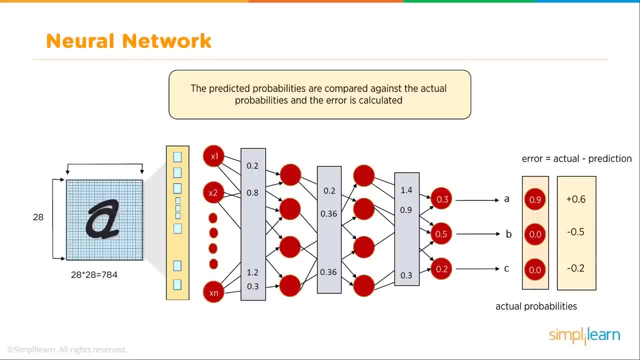 And the error is simply the actual minus predicted. And you can see here where we know it's 0.5.. It's not C, so it's a minus 2.. We know it's not B, so it's a minus 0.5.. 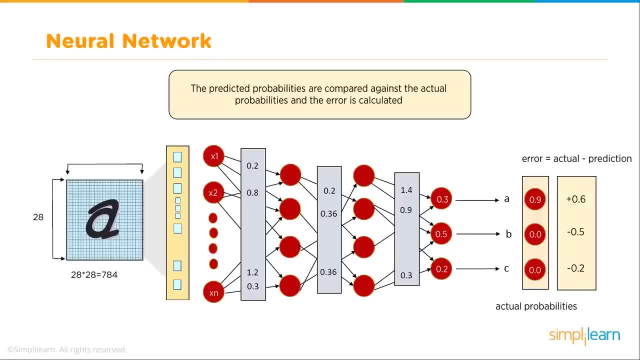 But we do know that it is an A, so we go ahead and adjust that by 0.6.. The magnitude indicates the amount of change, while the sign indicates an increase or decrease in the weights. The information is transmitted back through the network. 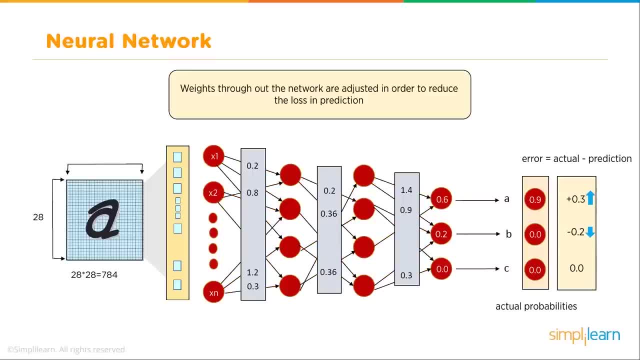 So here comes our back. propagation Weights throughout the network are adjusted in order to reduce the loss in prediction. So if we look at this setup right here, here comes our error, In this case 0.6, minus 0.5, minus 0.2.. 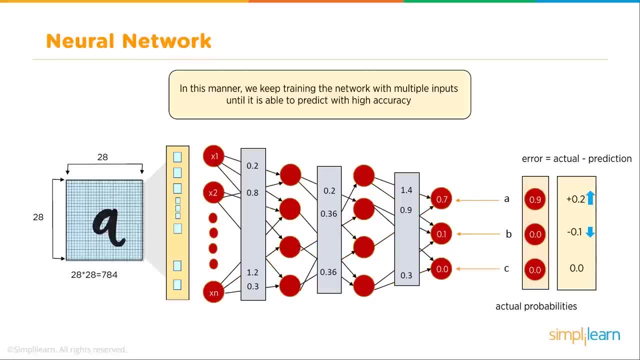 That comes up and adjusts our 1.4,, 0.9, all our multipliers In this manner. we keep training the network with multiple inputs until it is able to predict with a high accuracy And you can see here we have a different A- quickly switches from cursive A to maybe a more elongated A. 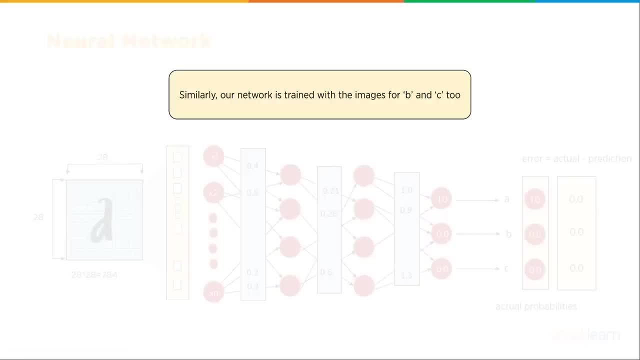 Similarly, our network is trained with the images for B and C too, So let's take a look at this. Here's a straightforward data set. Let's build a neural network to predict the outputs, given that the output is 0.6.. 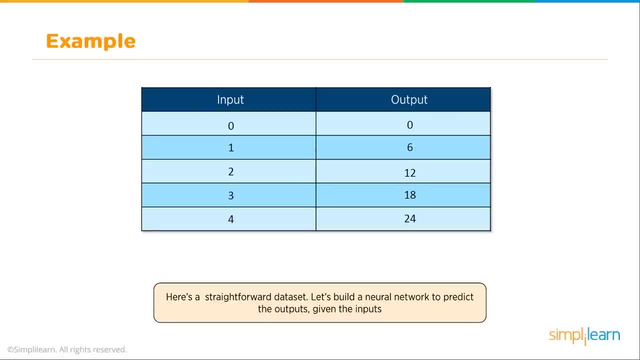 So we have an input 0,. we expect an output of 0,. we have an input of 1, we expect 6,. 2 equals 12,, 3 should come out as 18, and 4 as 24.. 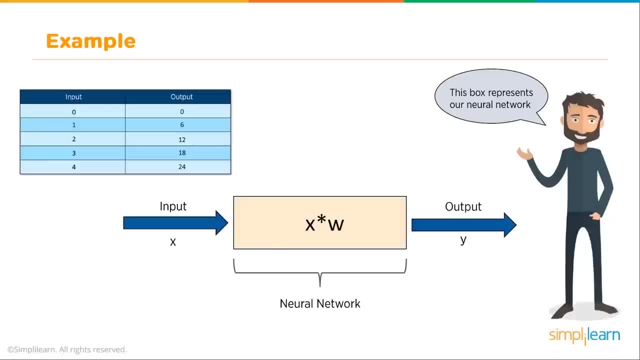 And we're just doing multiples of 6, if you take the time to look at it. So in our example we have our input and it goes into our neural network. So this box represents our neural network. One of the cool things about neural networks is there's always this little black box that you kind of train to do what you want. 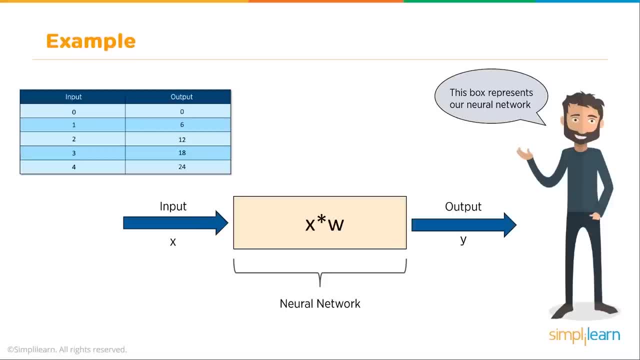 And you really don't have to know exactly what the weights are, Although there are some very high-end setups that start looking at those weights and how they work and what they do- And then you get your output, which is going to be, in this case, our input's going to be x and our output's going to be y. 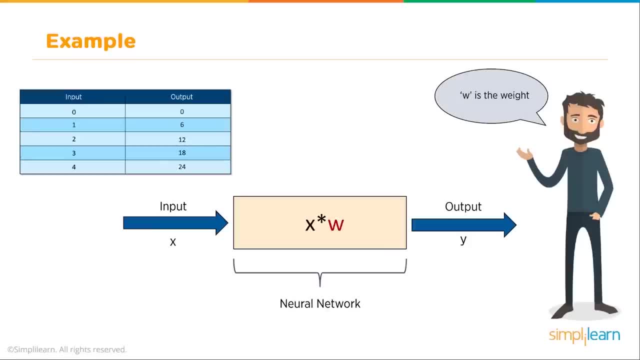 And w is the weight. So we have a value times the weight. So if we're doing in this case, just a single neuron going through, we have x times w. The network starts training itself by choosing a random value for w. 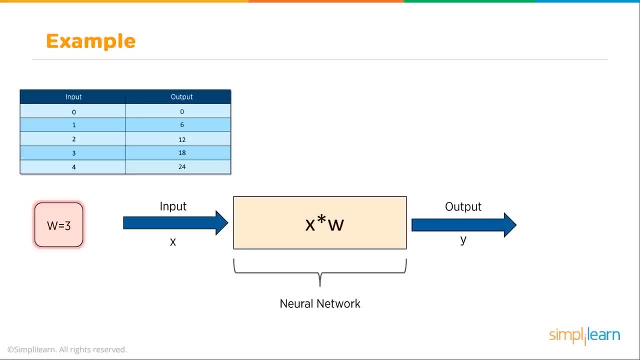 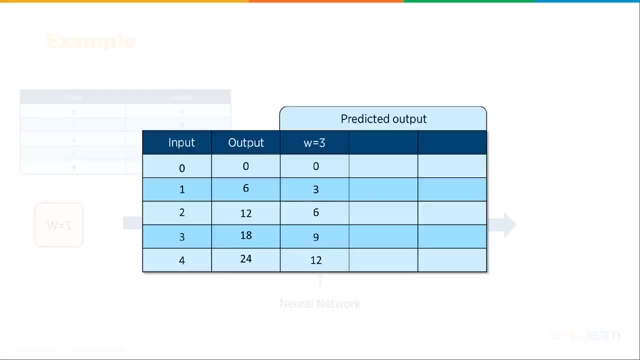 We're going to guess that w equals 3.. Just roll the dice randomly, generate the number 3 for w And then we put w equals 3.. In here we have our input 0, our output 0, w equals 3 equals 0. 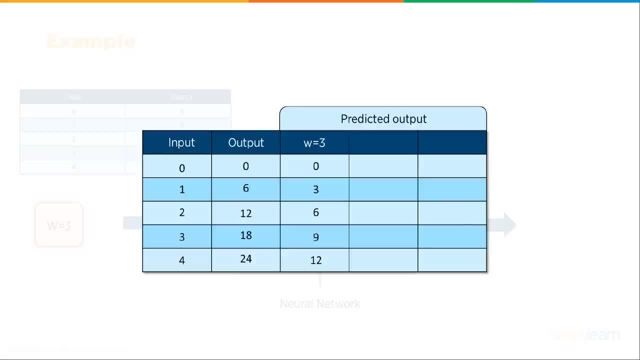 So we have no error on the first line That actually comes out correct. And then we have 1 times: we put the 1 in, We're looking for a 6,, but we get a 3 instead. And we put the 2 in: we're looking for a 12, and we get a 6 instead. 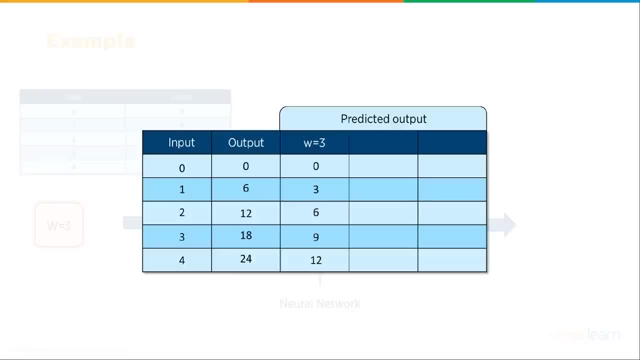 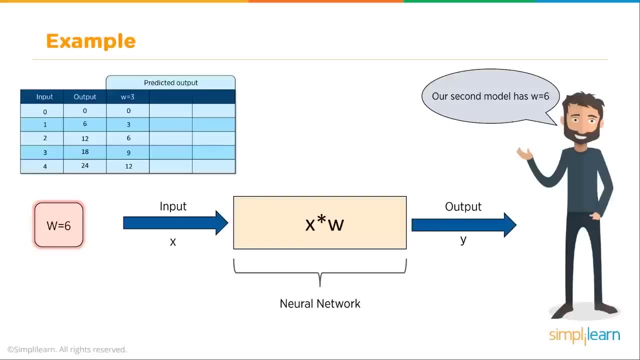 So you can see here our predicted output doesn't match the output we're looking for. And then we take this: we have our w equals 3, and we come up with a second model where the w equals 6.. Now we're going to look at how we figure out w equals 6 in just a minute. 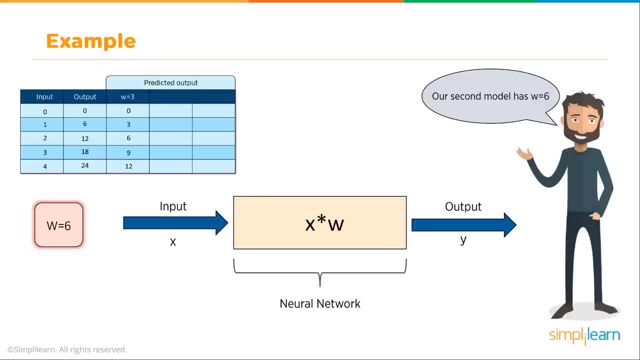 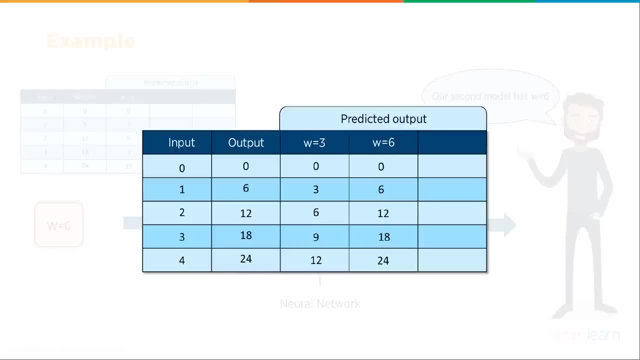 That is part of the math behind this, What you can see here. we put in w equals 6, and we build the w equals 6 chart. We end up with 0,, 6,, 12,, 18,, 24,, which is the output we're looking for. 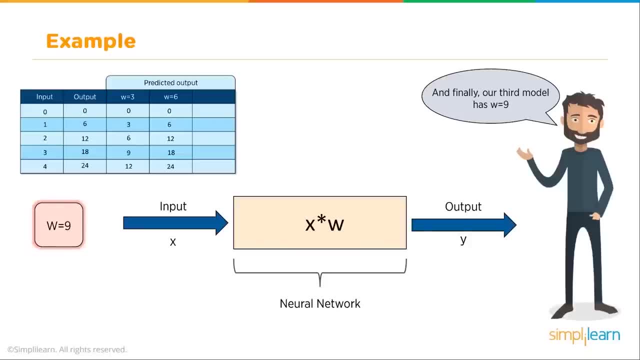 And in that manner we end up with the correct answer. But we'll go ahead and put in a third model where w equals 9.. So at this point one way of doing this is just to guess what w equals, And you can see: with w equals 9, we get the incorrect answer. 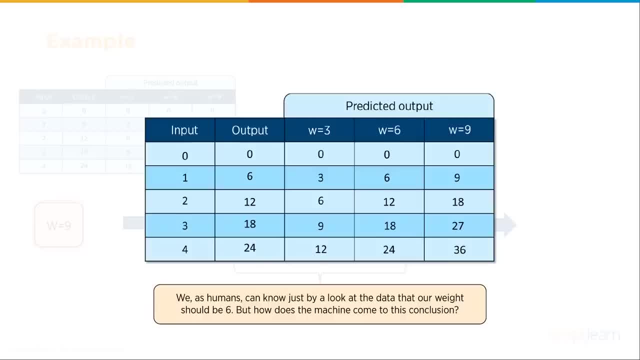 So we get 9,, 18,, 27,, 36.. We as humans can know just by taking a look at the data that our weight should be 6.. But how does the machine come to this conclusion? How do we program the computer to learn, instead of waiting for us to tell it it has the right answer or what the correct answer is? 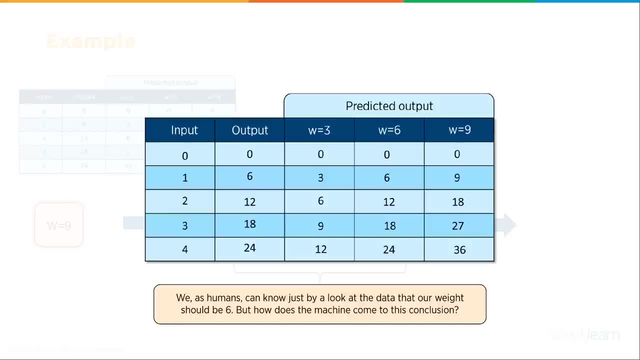 And you can imagine this is a very simple problem. If we're guessing w equals 3, we guess w equals 6,, we guess w equals 9.. And then we look at our results and we go, oh, it's got to be w equals 6.. 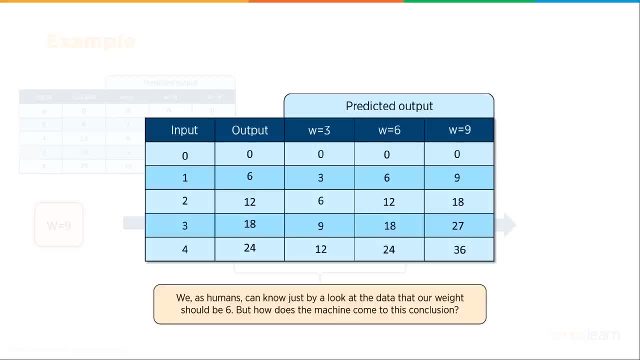 That's the best result. But as humans, we don't know, We don't know, We don't know. But as humans we want to take that element out and have the computer do that for us. So with that we're going to have a loss function. 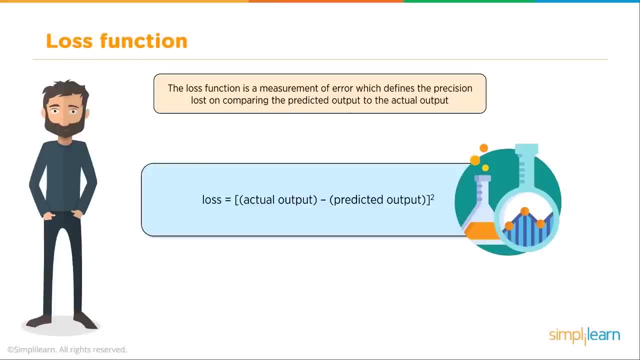 The loss function is a measure of error which defines the precision lost to comparing the predicted output to the actual output. And it's simply: loss equals actual output minus predicted output. and then we square the whole thing. So let's apply the loss function to the input value 2,. loss for our actual output: predicted. 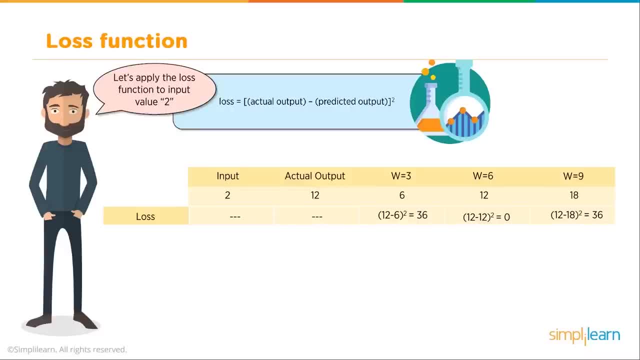 output squared And our loss function. for the input of 2,, we end up with an actual output of 12.. And you can see here W equals 3, 12 minus 6 squared equals 36.. So we end up with a loss of 36.. 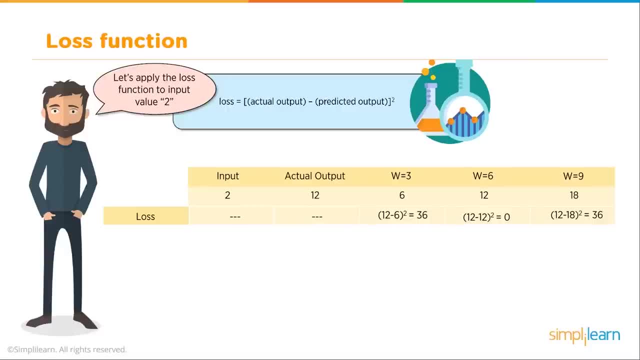 W equals 6, 12,. 12 times 12 squared equals 12 minus 12 squared equals 0.. Or 12 minus 18 squared equals 36.. And so you can see we have a huge loss on w equals 3 and w equals 9.. 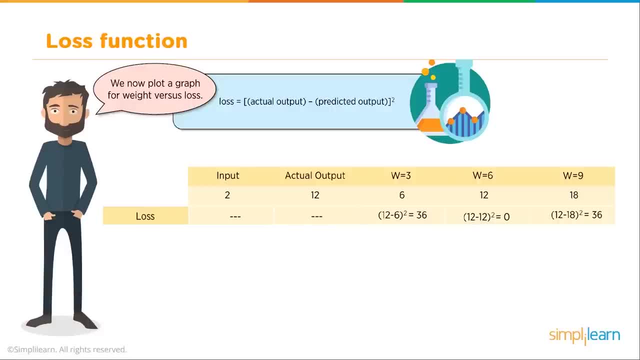 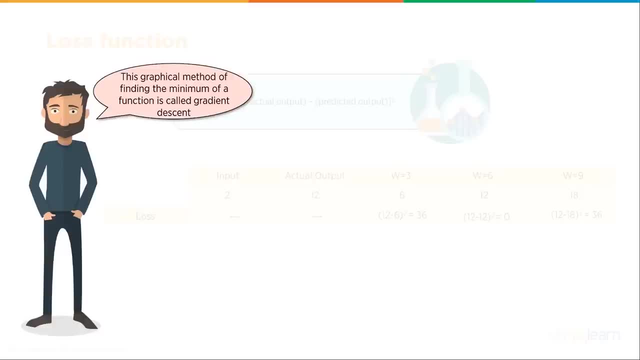 We now plot a graph for the weight versus loss, And it always helps to have a nice visual of what's going on here. So this graphical method of finding the minimal of a function is called gradient error, And this is the logic behind this. 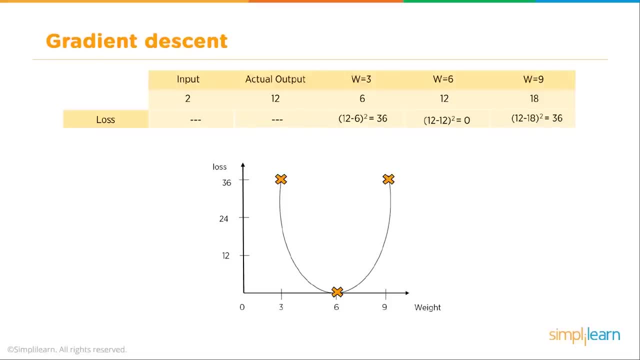 You can see, as we come in here we go ahead and graph the loss. We have 36 for 3 and 36 for 9.. We happen to guess 6, which was the correct answer. right in the middle And you can see, right here it forms a nice little parabola and you can see a nice mark. 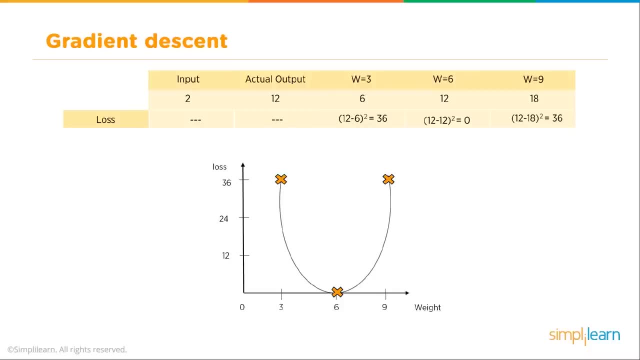 right in the middle, And as a human being, we can look at that and we go: ah, the answer is 6.. A random point on this curve is chosen and the slope at this point is calculated. So now we're getting away from the human aspect of just looking at it and saying what the 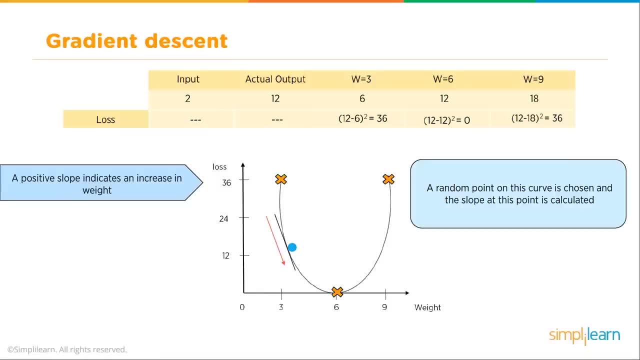 answer is, and we look at what's going on with the math, And so if we have a positive slope, it indicates an increase in the weight and a negative slope indicates a decrease in weight. This time the slope is negative. hence another random point towards its left is chosen. 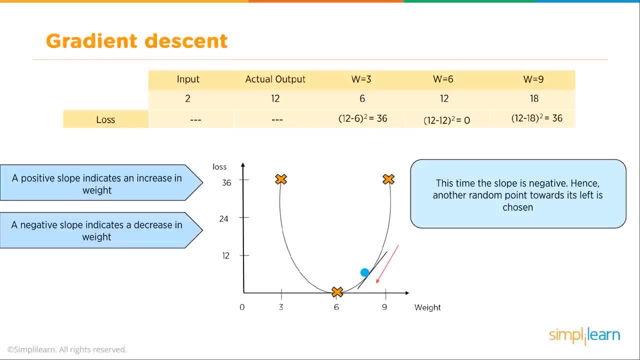 And you can see, here we're actually kind of just playing a little high-low game, going back and forth with the gradient descent. We continue checking slopes at various points in this manner. So we have our input, actual output, w3, w6, w9.. 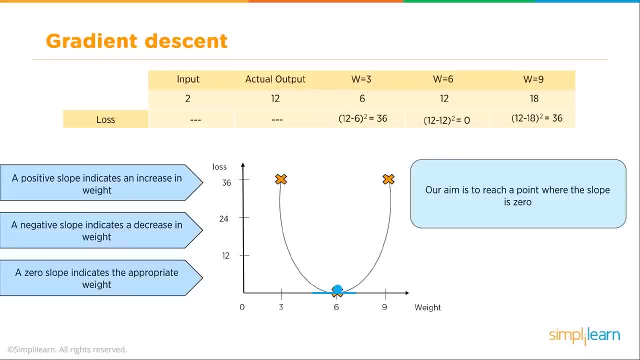 We found our positive slope increased an increase in weight. A negative slope indicates a decrease in weight. A zero slope indicates the appropriate weight. So our aim is to reach a point where the slope is zero. And when we talk about neural networks, you're usually processing a massive amount of information. 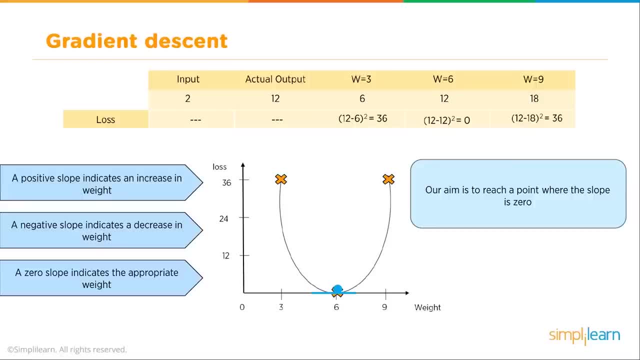 and data. So you're not going to have all your data nice and neat where it's just a multiple of 6. It's going to be messy, And so we're going to keep approaching that number, but you'll never get everything to. 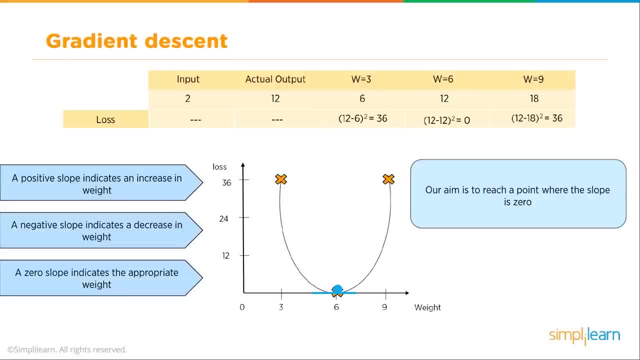 fit at zero. You're going to get stuff all over the place, and so you're really looking for the minimum value. You're not looking for an absolute zero because you're not going to get it, And so we're talking about gradient descent. 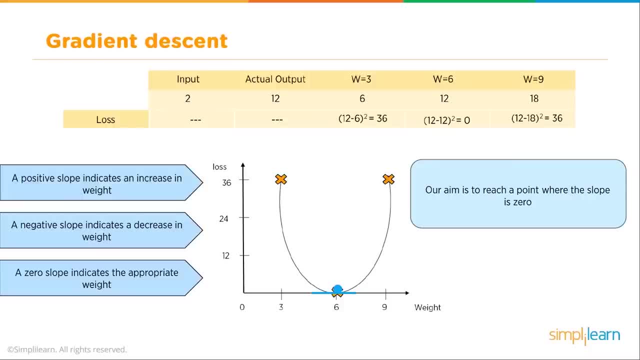 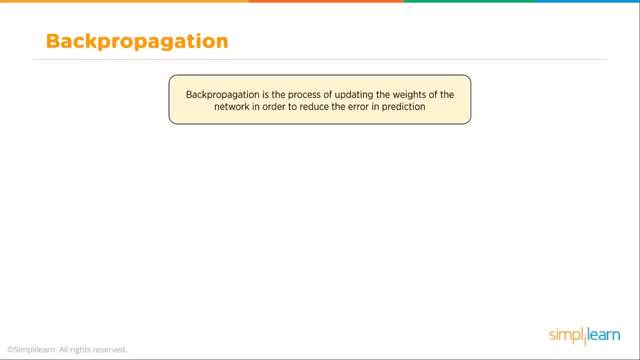 That's what we're talking about on there is finding the bottom of that curve, even if it doesn't go all the way to zero. So how do we apply that to our neural network? Well, we use back propagation. Back propagation is a process of updating weights of the network in order to reduce. 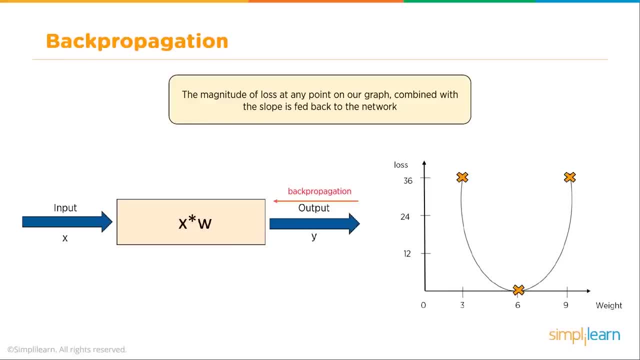 the error in prediction, And so the magnitude of loss of any point on our graph, combined with the slope, is fed back to the network And you can see here- here's our simple model, with just one node of x times w The input comes in, we have our x times w the output and then we're going to propagate. 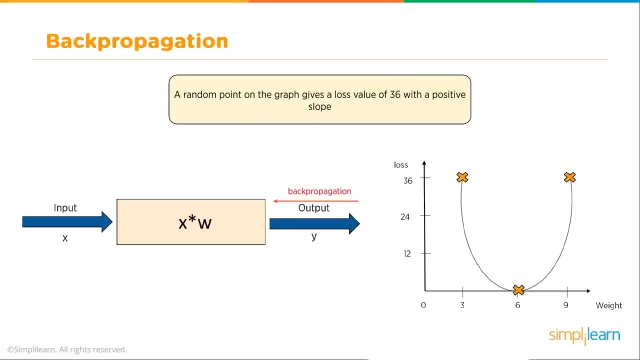 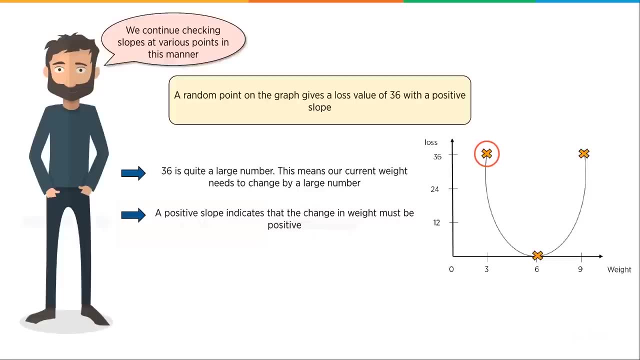 that loss going the other way, A random point on the graph gives a loss value of 36 with a positive slope, and we continue checking slopes at various points in this manner. So a random point on the graph gives a loss value of 36 with a positive slope. 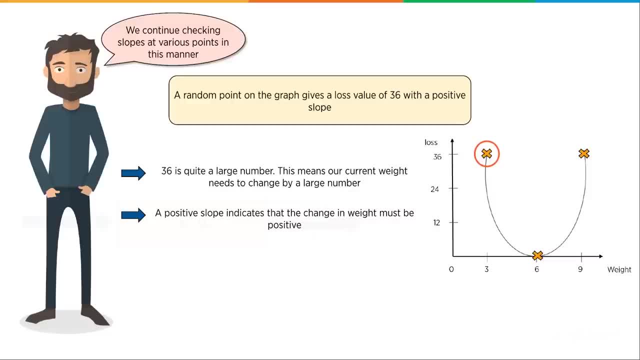 36 is quite a large number. This means our current weight needs to change by a large number. A positive slope indicates that the change of the weight must be positive. Similarly, another random point on the graph gives a loss value of 10 with a negative. 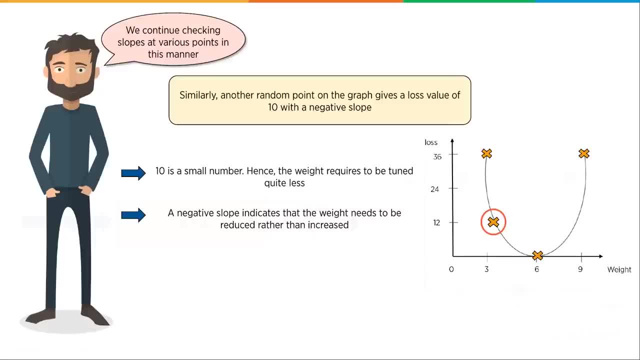 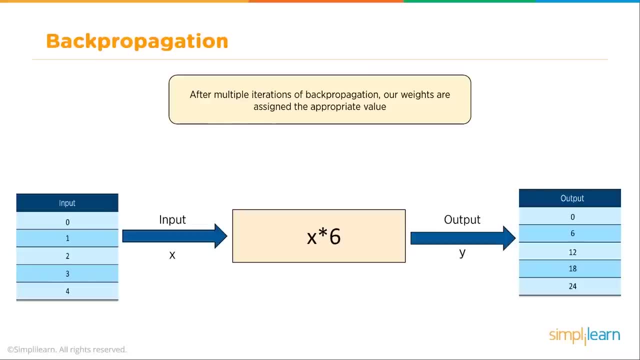 slope 10 is a small number, hence the weight requires to be tuned quite less. A negative slope indicates that the weight needs to be reduced rather than increased. After multiple iterations of back propagation, our weights are assigned the appropriate value. You can see, here we have our input. we just looked at x times 6 in our output and eventually 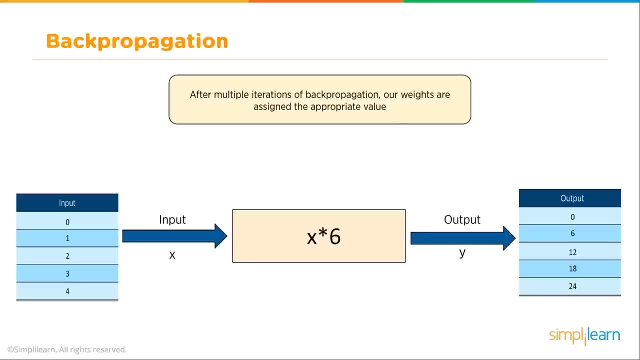 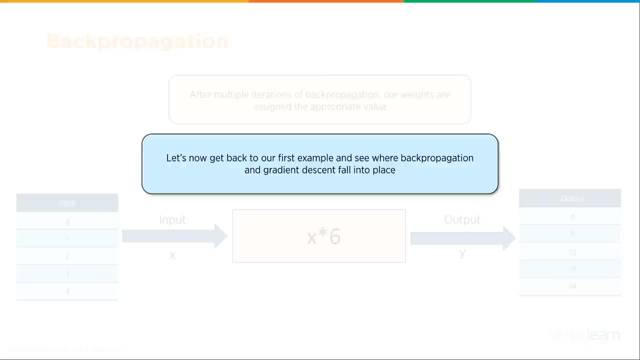 we get it that the weight is 6 for the single node problem that we're working on right now. At this point, our network is trained. It can be used to make predictions. Let's now get back to our first example and see where the back propagation and gradient 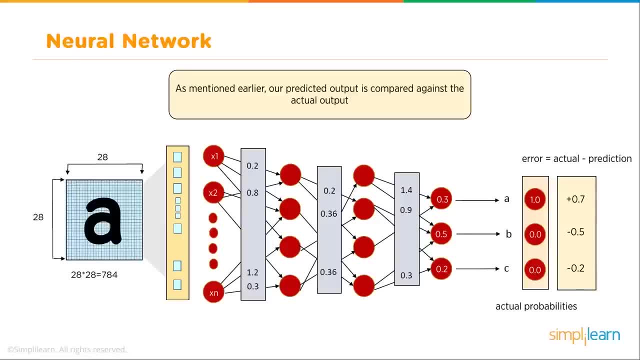 descent fall into place And you can see here we're not looking at a single node anymore. Now we have 28 by 28 grid or 784 inputs coming into the first level, which has 784 nodes, Depending on how you build your neural network. the next layer might also have 784 nodes. 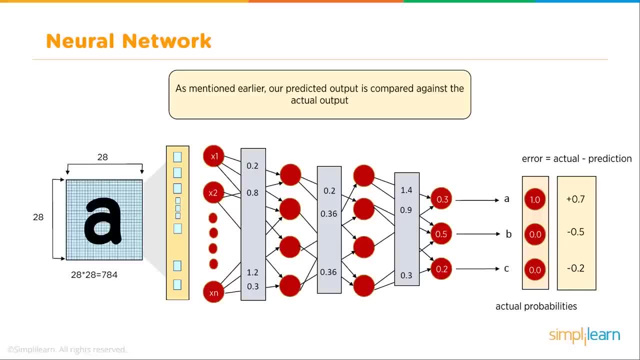 or it might continually smallen, depending on what you need and what's needed for that to work. So, as mentioned earlier, The predicted output is compared against the actual output. You can see our error over here: Actual minus prediction. And then we go ahead and compute our loss. 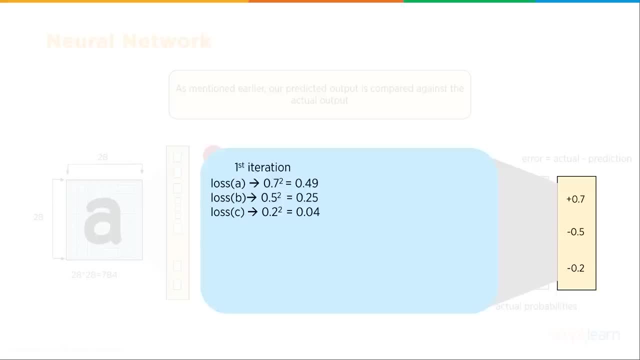 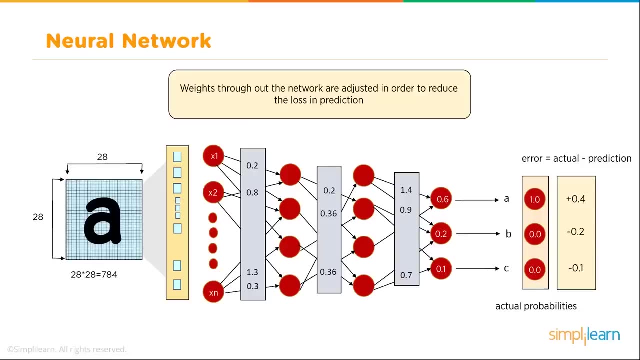 So the loss of A is 0.7 squared, equals 0.49.. Loss of B is 0.5 squared, or 0.25, and so on. So now we have our first iteration on there. So weights throughout the network are adjusted in order to reduce the loss in prediction. 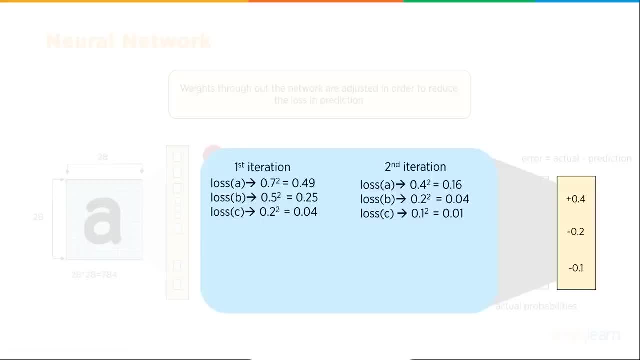 And of course we do that by doing a second iteration coming through with our different losses on there. Weights throughout the network are adjusted in order to reduce the loss in prediction, again underneath the second, And we do a third iteration And we just keep doing these iterations, going back until we get the right value. 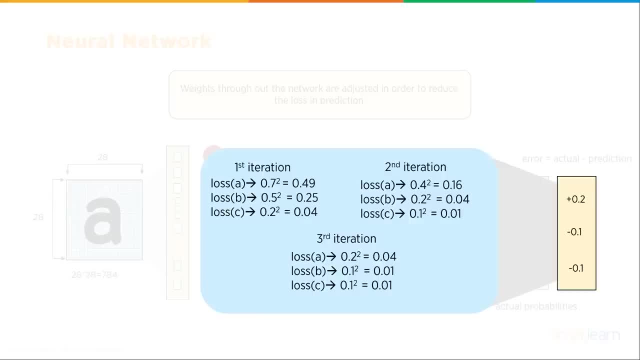 Now you've got to remember that when we're doing a reverse propagation, we're not looking at just one letter A, We're looking at hundreds of letter A's And usually when we propagate that loss going backwards, we only take a small piece of it. 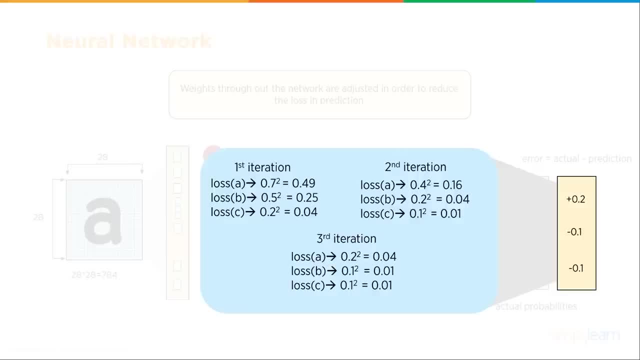 So our adjustments are very small because one of them is not correct. We don't want to create a bias. So when we talk about back propagation, we're talking about going through over and over and over this data until we get minimal loss for our letter A. 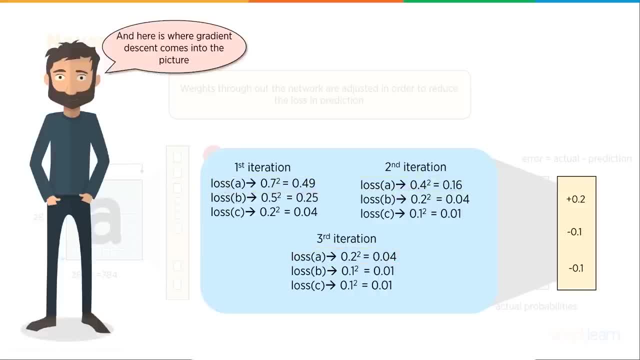 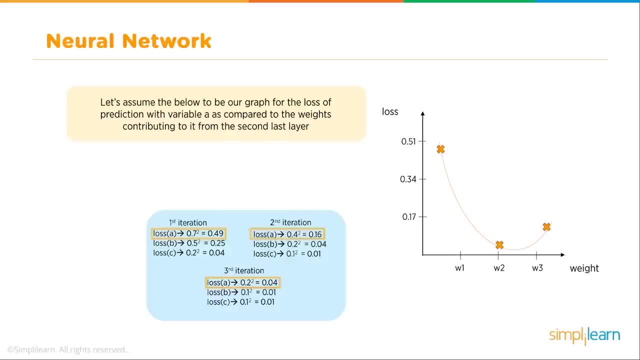 So let's focus on the minimal loss for our variable A And you can see here we look at that we end up. we'll assume for below to be our graph for the loss of prediction with the variable A as compared to the weights, continuing it from the second layer. 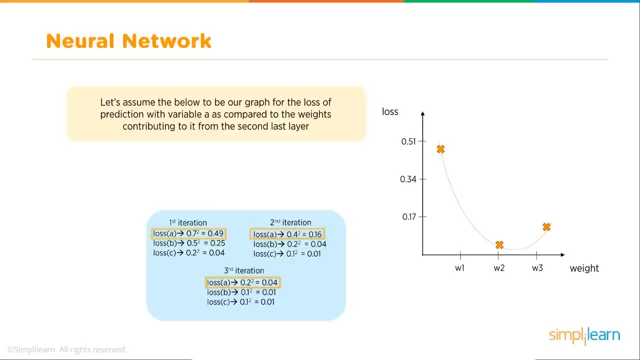 And we have our loss of A for 49,, for 16,, for 0.04.. And you can see it makes this nice curve where we can guess where the bottom of this curve is. And I like it on this graph that they show that the curve doesn't rest. yeah, on the. 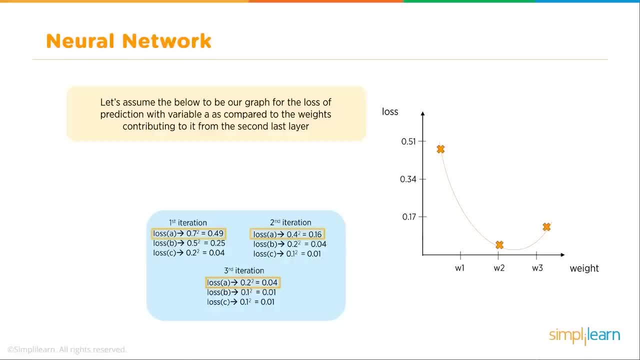 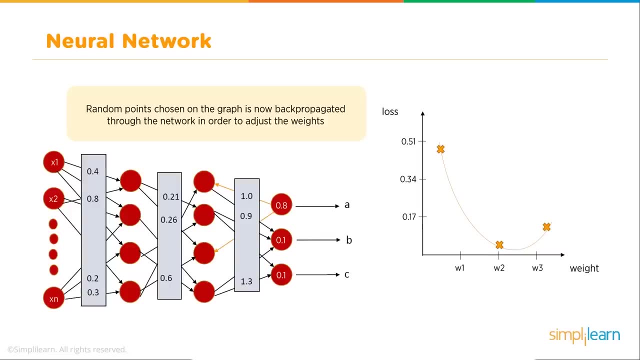 x-axis. It doesn't rest at where y equals 0, because you usually don't get that. You don't get a perfect fit on anything, or very rarely do you ever get a perfect fit, And so the random points chosen on the graph is now back propagated through the network. 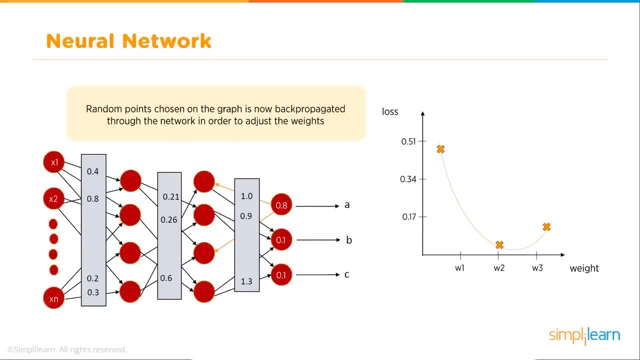 in order to adjust the weights. So we're able to go back through the network and readjust those weights. until we find that minimal value, The network is run once again with the new weights. This process is repeated multiple times until it provides accurate predictions. 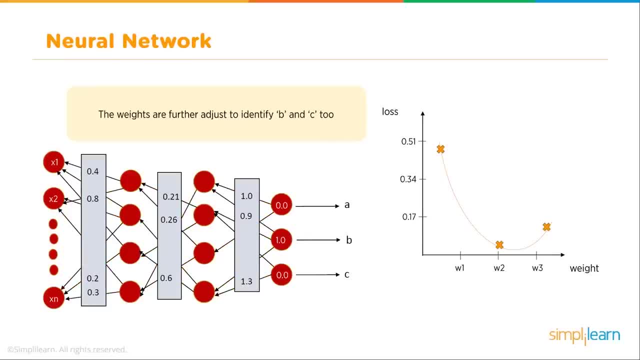 The weights are further adjusted to identify B and C, And this is interesting because you actually do them at the same time. So as the error goes back, you kind of find the overall error for all the inputs coming in and then that's what gets propagated going back, or the overall loss. 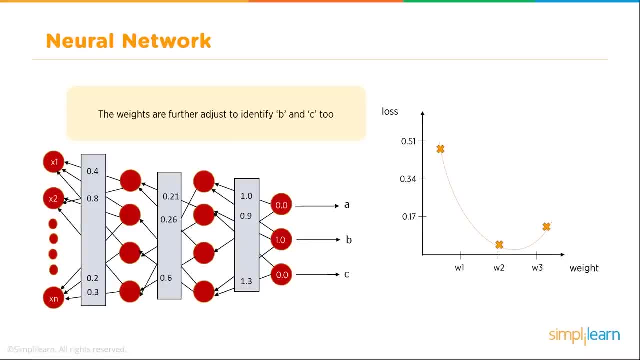 You kind of have to step away from that word error, because it's not just about the error, it's about the loss. The weights are further adjusted to identify B and C too, And so a lot of times you actually do them all at the same time. but you'll adjust those. 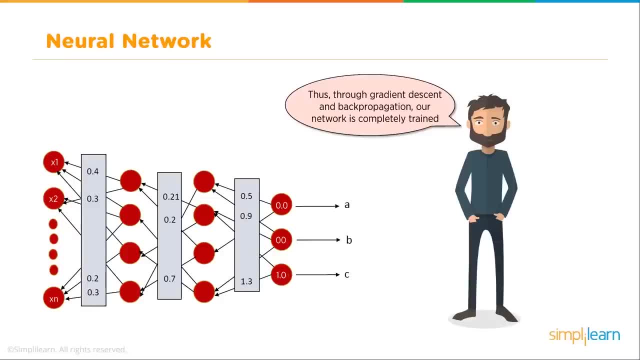 weights A, B and C, as I was just saying, Just through gradient descent and back propagation. our network is completely trained And we've taught it to identify A, B and C coming forward. One of the interesting things about neural networks is the training process takes a lot. 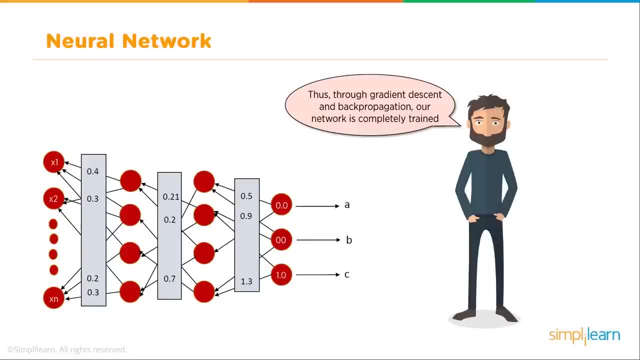 longer than the predicting process. So you can plan one of these training neural networks doing the back propagation to significantly longer, because you're going over thousands of data points And then when you actually run it forward it's very quick, which makes these things. 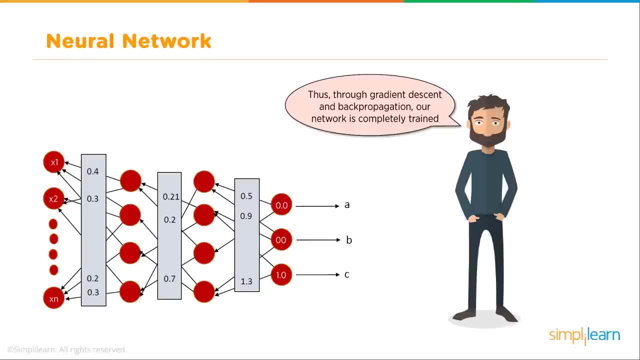 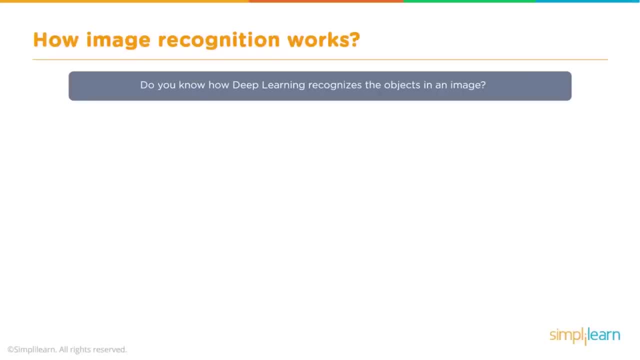 very useful And just really part of today's world in computing. Today we're going to be covering the convolutional neural network tutorial. Do you know how deep learning recognizes the objects in an image? And really this particular neural network is how image recognition works. 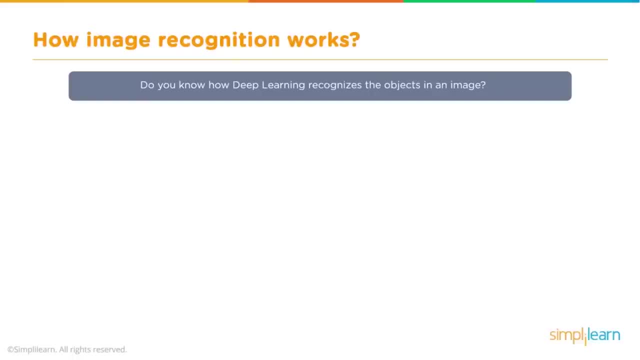 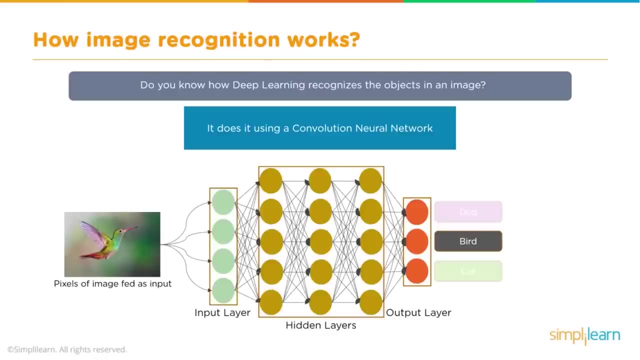 It's very central, one of the biggest building blocks for image recognition. It does it using convolution neural network. We over here, we have the basic picture of a hummingbird, Pixels of an image fed as input. You have your input layer coming in. 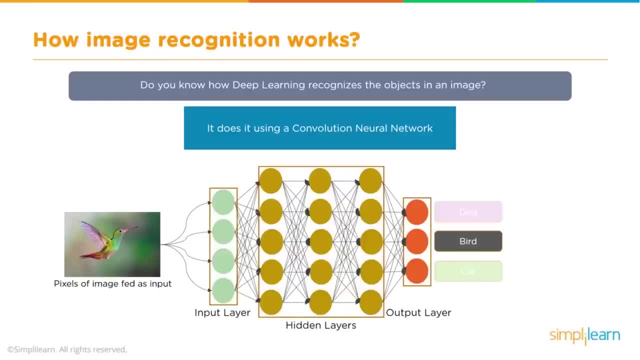 So it takes that graphic and puts it into the input layer. You have all your hidden layers And then you have your output layer and your output layer. One of those is going to light up and say, oh, it's a bird, We're going to go into depth. 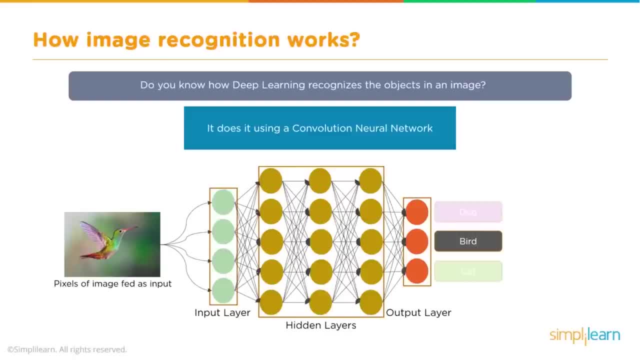 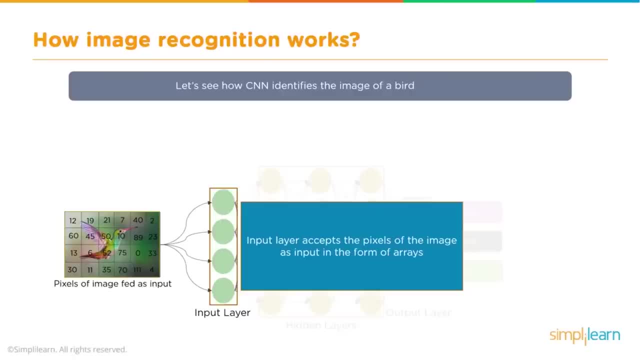 We're going to actually go back and forth on this a number of times today, So if you're not catching all the image, don't worry, we're going to get into the details. So we have, our input layer accepts the pixels of the image as input in the form of arrays. 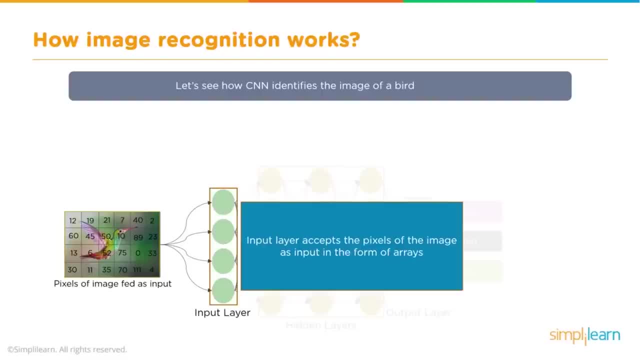 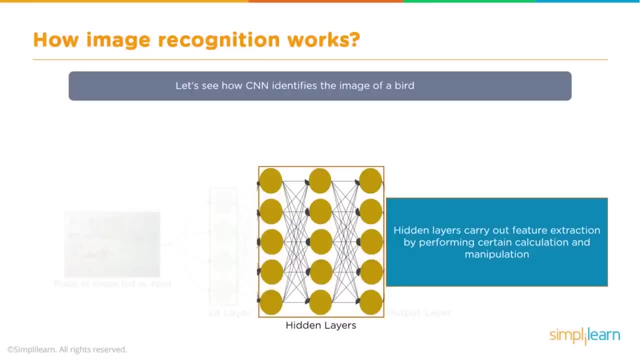 And you can see up here where they've actually labeled each block of the bird in different arrays. So we're going to go back and forth and see what that looks like and how those matrices are set up. Your hidden layer carry out feature extraction by performing certain calculations and manipulation. 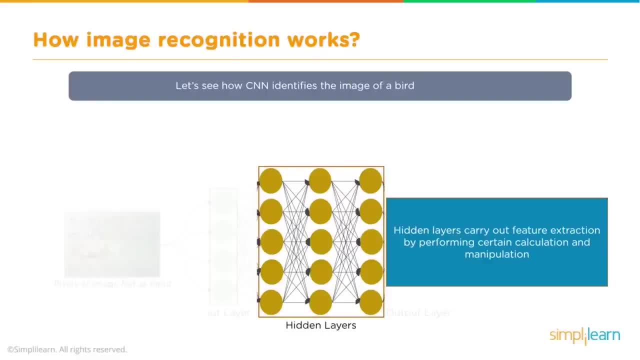 So this is the part that kind of reorganizes that picture multiple ways until we get some data that's easy to read for the neural network. This layer uses a matrix filter and performs convolution operation to detect patterns in the image. And if you remember that convolution means to coil or to twist, 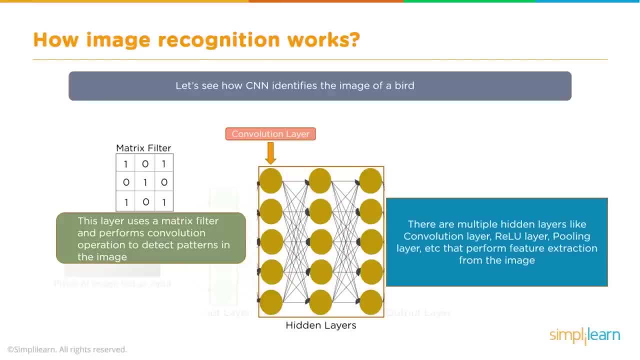 So we're going to twist the data around and alter it And use that operation to detect a new pattern. There are multiple hidden layers, like convolution layer. rel u is how that is pronounced, And that's the rectified linear unit That has to do with the activation function that's used. 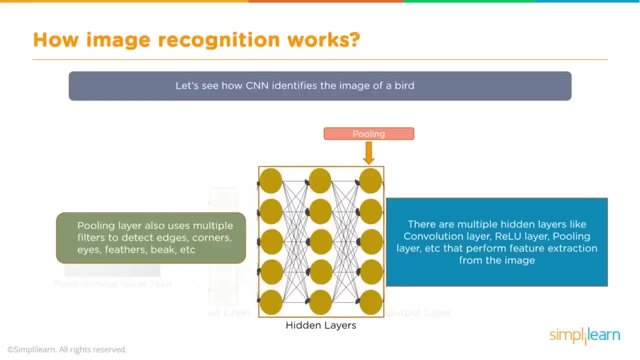 Pooling layer also uses multiple filters to detect edges, corners, eyes, feathers, beak, et cetera. And just like the term says, pooling is pooling information together, And we'll look into that a lot closer here. So if it's a little confusing now, we'll dig deeper. 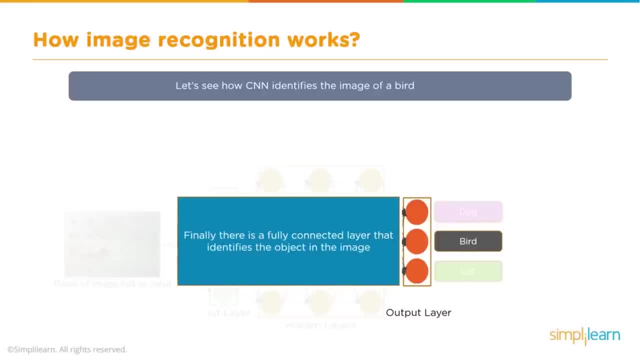 We'll dig in deep and try to get you squared away with that. And then, finally, there is a fully connected layer that identifies the object in the image. So we have these different layers coming through in the hidden layers And they come into the final area. 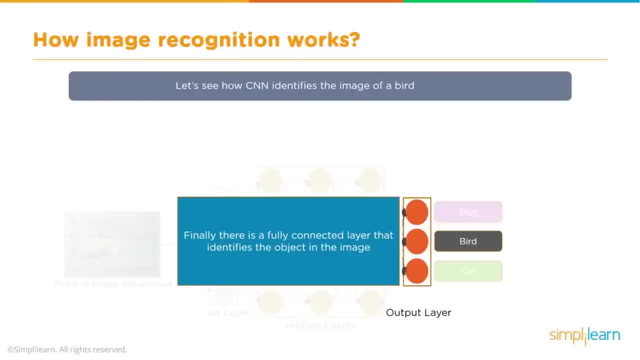 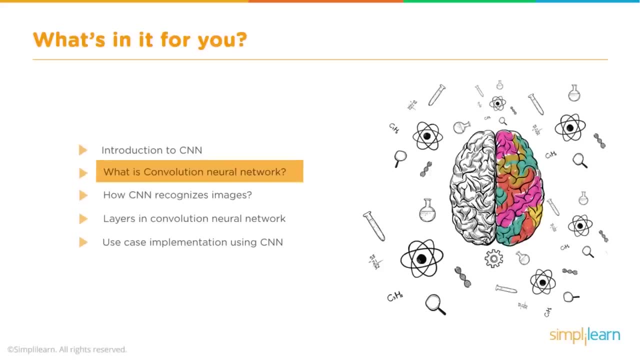 And that's where we have, say, one node or one neural network entity that lights up, that says it's a bird, What's in it for you? We're going to cover an introduction to the CNN. What is convolution neural network? How CNN recognizes images. 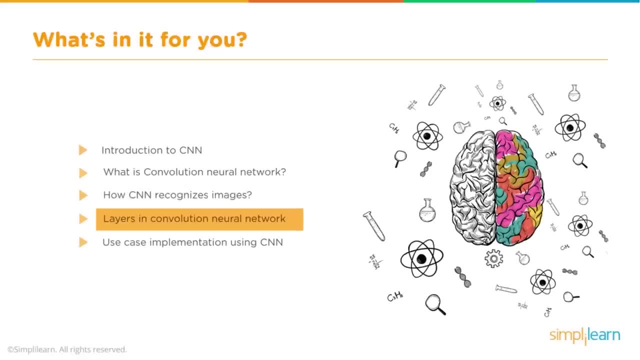 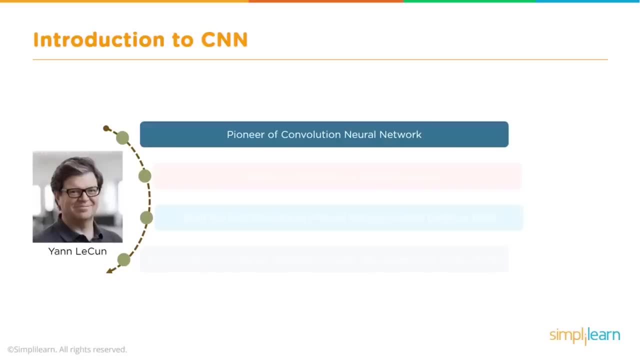 We're going to dig deeper into that And really look at the individual layers. We're going to look at the individual layers in the convolutional neural network And finally we do a use case implementation using the CNN. We'll begin our introduction to the CNN by introducing the pioneer of convolutional neural. 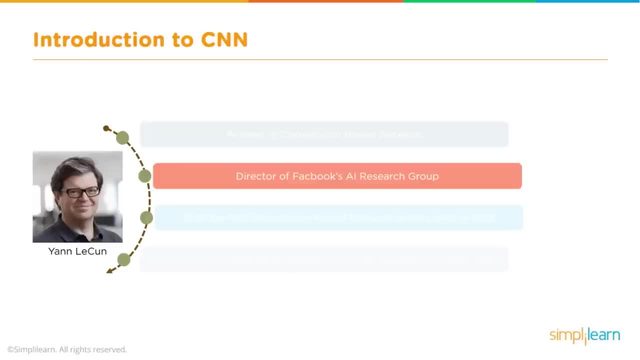 network. Yann LeCun- He was the director of Facebook AI research group- Built the first convolutional neural network called LeNet, in 1988. So these have been around for a while and have had a chance to mature over the years. 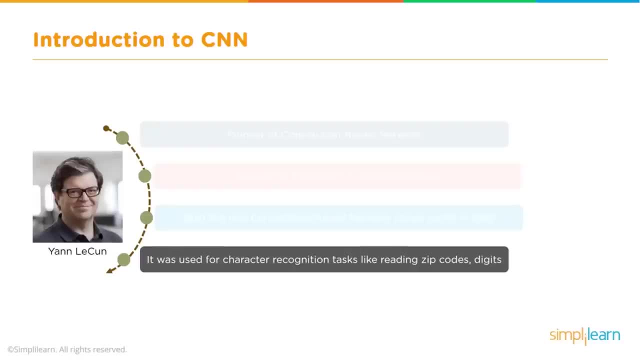 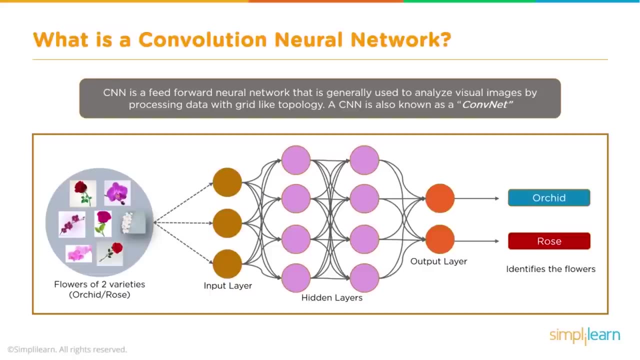 It was used for character recognition tasks like reading zip code digits. Imagine processing mail and automating that process. CNN is a feed forward neural network that is generally used to analyze visual images by producing data with a grid-like topology. A CNN is also known as a ConvNet. 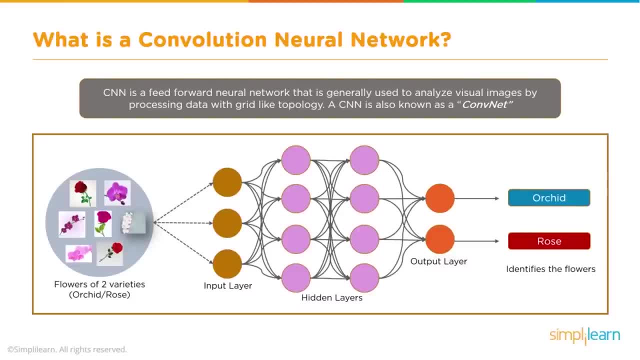 And very key to this is we are looking at images. That was what this was designed for, And you'll see the different layers as we dig in, mirror some of the other. Some of them are actually now used, since we're using TensorFlow and Keras in our code later. 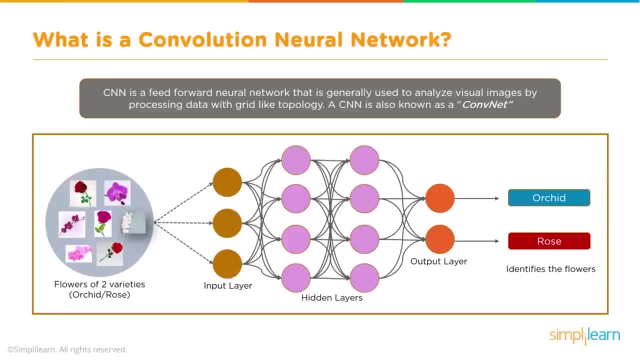 on, And some of those layers appear in a lot of your other neural network frameworks, But in this case this is very central to processing images and doing so in a variety that captures multiple images and really drills down into their different features. In this example, here you see flowers of two varieties: orchid and a rose. 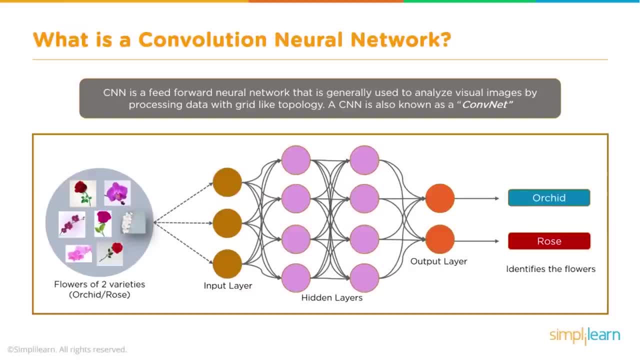 I think the orchid is much more dainty and beautiful and the rose smells quite beautiful. I have a couple of rose bushes in my yard. They go into the input layer. That data is then sent to all the different nodes in the next layer, one of the hidden. 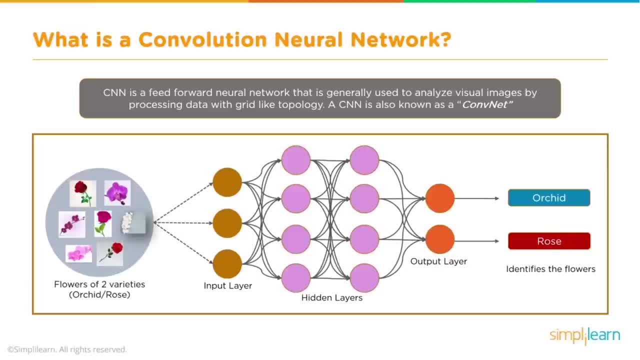 layers And, based on its different weights and its setup, it then comes out and gives those a new value. Those values then are multiplied by their weights and go to the next hidden layer, and so on, And then you have the output layer And one of those nodes comes out and says it's an orchid, and the other one comes out. 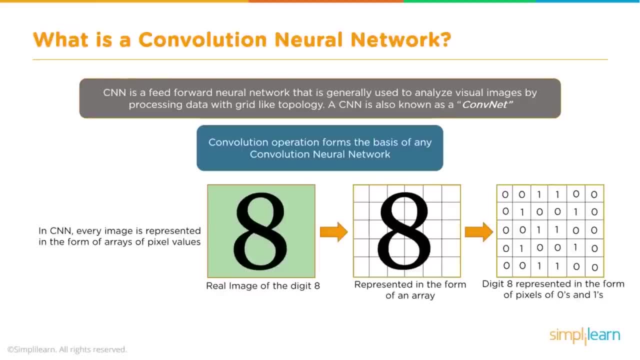 and says it's a rose, depending on how well it was trained. What separates the CNN or the convolutional neural network from other neural networks is a convolutional operation forms a basis of any convolutional neural network. In a CNN, N is represented in the form of arrays of pixel values. 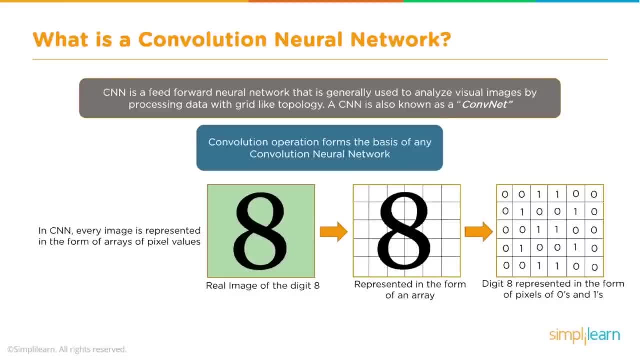 So here we have a real image of the digit 8.. That then gets put onto its pixel values, represented in the form of an array. In this case you have a two-dimensional array And then you can see in the final N form we transform the digit 8 into its representational form of pixels, of zeros and 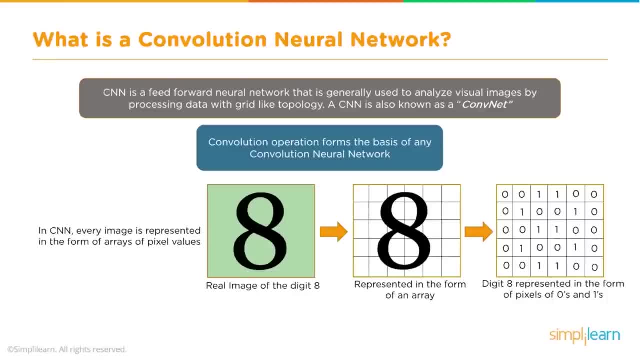 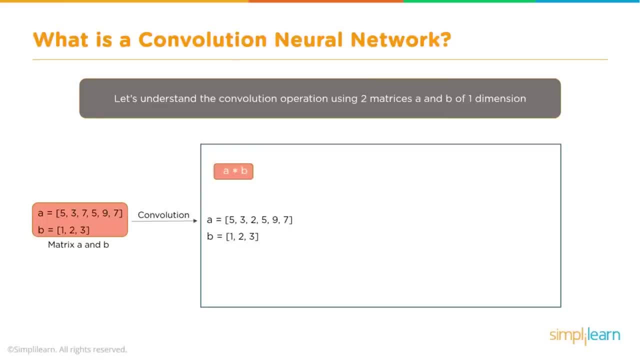 1, where the 1's represent, in this case, the black part of the 8 and the 0's represent the white background, To understand the convolution neural network or how that convolutional neural network works, network, or how that convolutional operation works. we're going to take a sidestep and 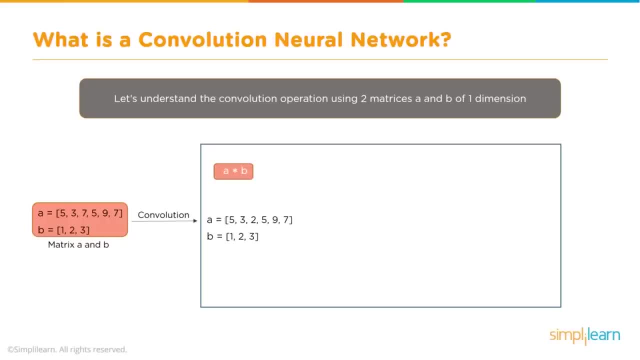 look at matrices In this case. we're going to simplify it and we're going to take two matrices, A and B, of one dimension. Now kind of separate this from your thinking as we learn that you want to focus just on the matrix aspect of this, And then we'll bring 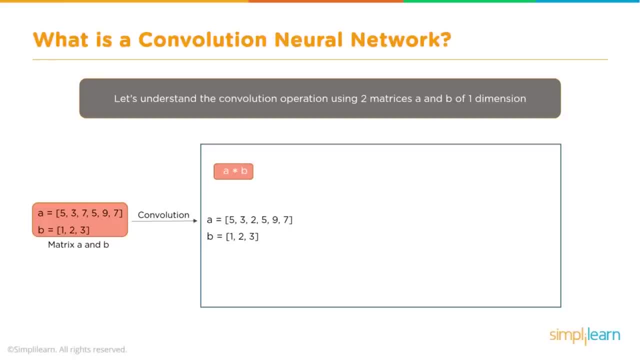 that back together and see what that looks like when we put the pieces for the convolutional operation. Here we've set up two arrays. We have in this case a single dimension matrix And we have A equals 5,, 3,, 7,, 5,, 9,, 7.. And we have B equals 1,, 2, 3.. So in the convolution 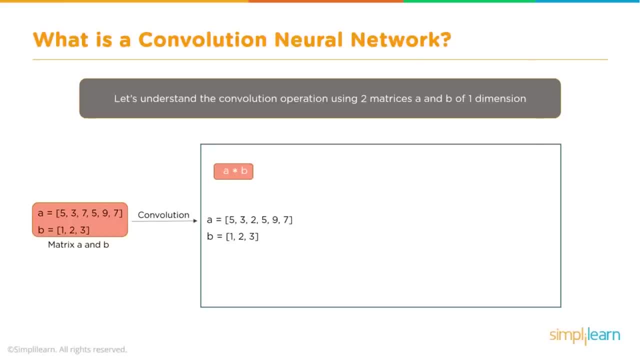 as it comes in there, it's going to look at these two and we're going to start by doing multiplying them A times B, And so we multiply the arrays element-wise and we get 5,, 6, 6, where 5 is the 5 times 1,, 6 is 3 times 2, and then the other 6 is 2 times 3.. And 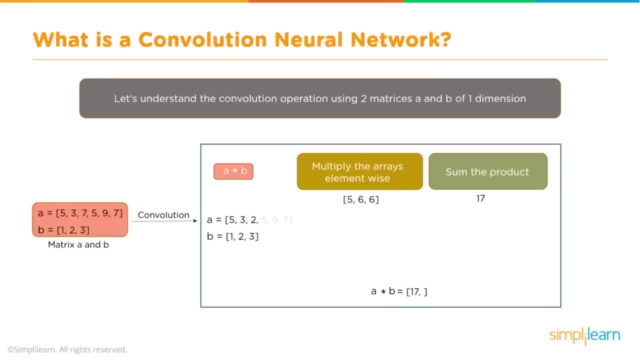 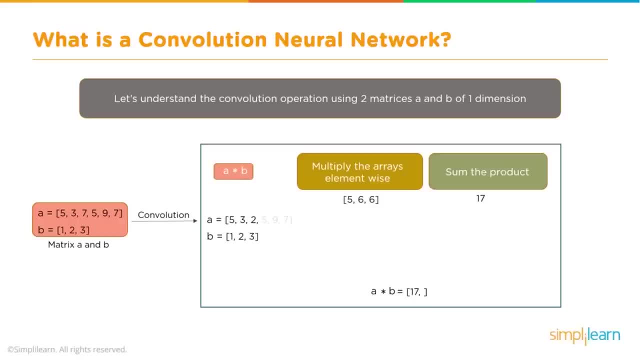 multiplied just by the first three elements of the first array. Now that's going to be a little confusing, Remember, a computer gets to repeat these processes hundreds of times. So we're not going to just forget those other numbers. later on We'll bring those back in And then we have. 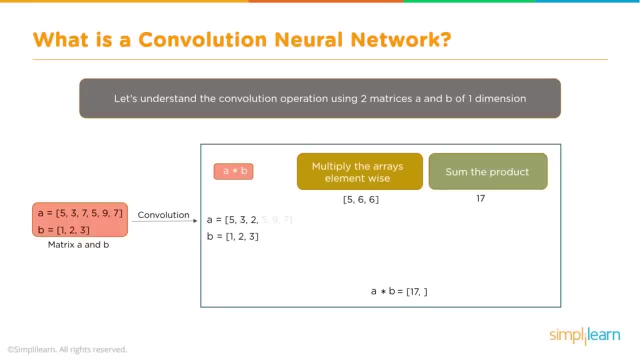 the sum of the product. In this case 5 plus 6 plus 6, equals 17.. So in our A times B, our very first digit in that matrix of A times B is 17.. And if you remember I said we're not going to. 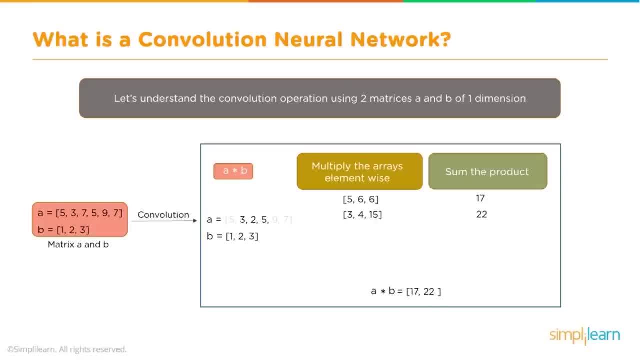 forget the other digits. So we now have 325.. We move one set over and we take 325, and we multiply that times B And you'll see that 3 times 1 is 3,, 2 times 2 is 4, and so on and so on. We. 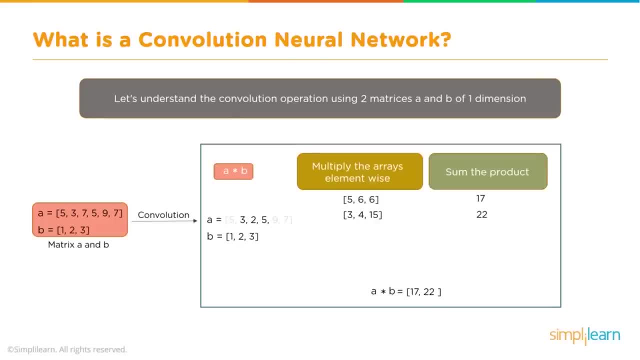 sum it up, So now we have the second digit of our A times B product in the matrix, And we continue on with that same thing, so on and so on. So then we would go from 375 to 759 to 597.. This short. 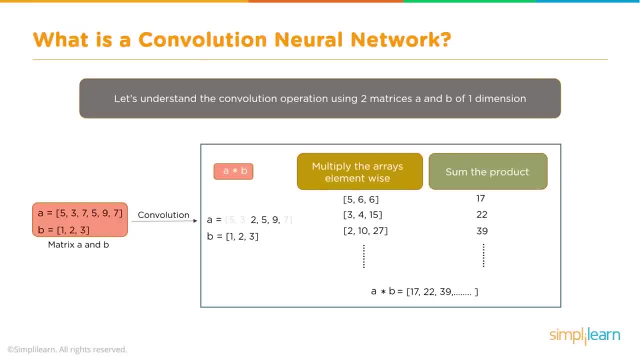 matrix that we have for A. We've now covered all the different entities in A that match three different levels of B. Now in a little bit we're going to cover where we use this math at this multiplying of matrices and how that. 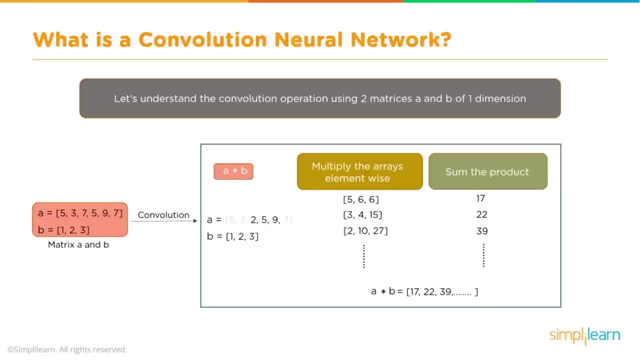 works, But it's important to understand that we're going through the matrix and multiplying the different parts to it to match the smaller matrix with the larger matrix I know a lot of people get lost at is you know what's going on here with these matrices? Oh, scary math, Not really that. 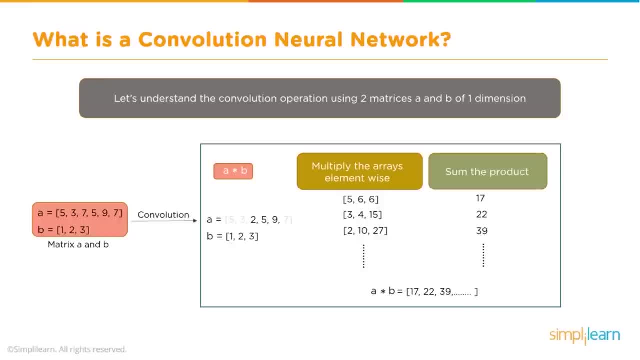 scary when you break it down. We're looking at a section of A and we're going to look at the matrix, We're comparing it to B. So when you break that down in your mind like that, you realize okay, so I'm just taking these two matrices and comparing them and I'm bringing the value down. 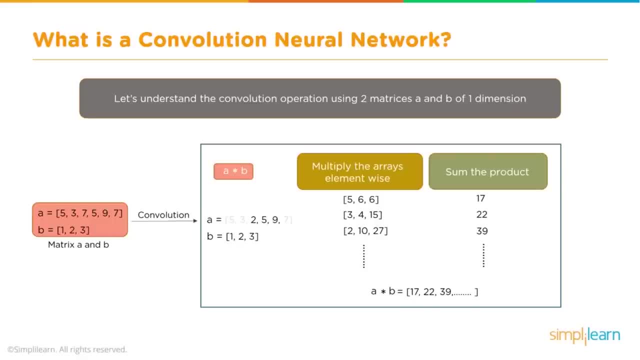 into one matrix A times B. We're deucing that information in a way that will help the computer see different aspects. Let's go ahead and flip over again back to our images. Here we are back to our images, Talking about going to the most basic two-dimensional image you can get to. 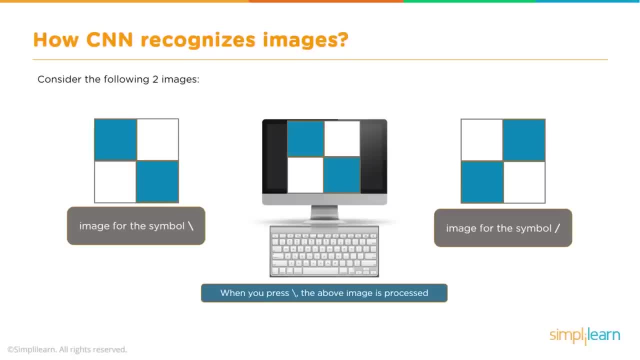 Consider the following two images. The image for the symbol backslash: When you press the backslash the above image is processed And you can see there. for the image for the forward slash is the opposite. So when we click the forward slash button, that flips. Very basic. 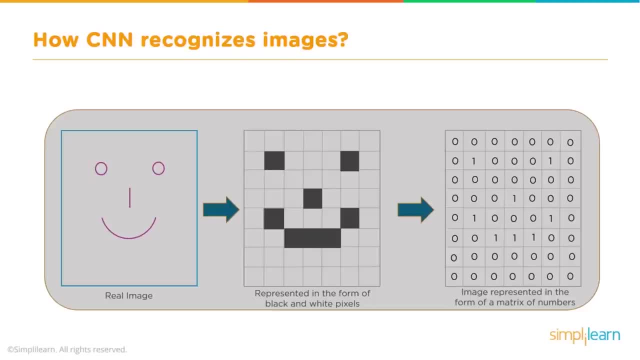 We have four pixels going in. Can't get any more basic than that. Here we have a little bit more complicated picture. We take a real image of a smiley face. Then we represent that in the form of black and white pixels. So if this was an image in the computer, it's black and white And, like we 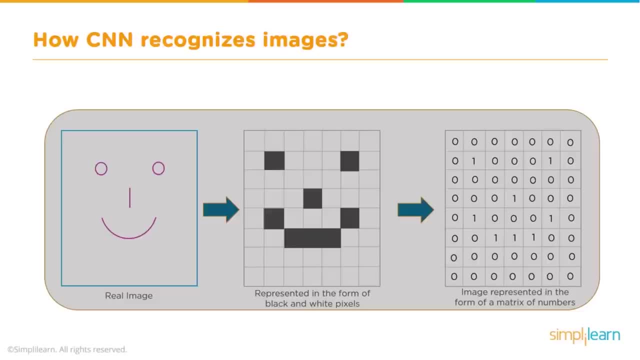 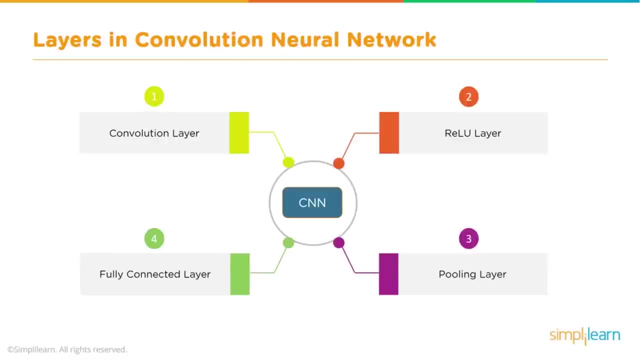 saw before we convert this into the zeros and ones, Where the other one would have just been a matrix of just four dots. now we have a significantly larger image coming in. So don't worry, we're going to bring this all together here in just a little bit. 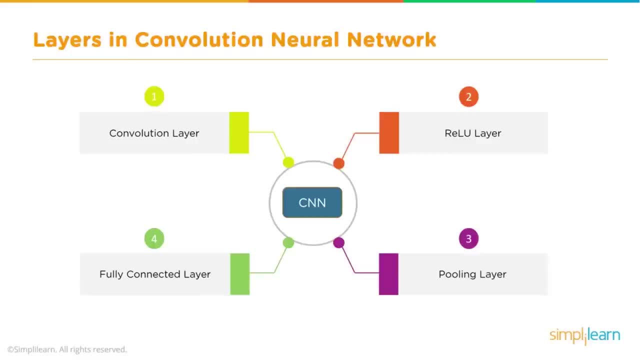 Layers in Convolutional Neural Network. When we're looking at this, we have our convolution layer And that really is the central aspect of processing images in the Convolutional Neural Network. That's why we have it. And then that's going to be feeding in And you have your relu layer, which is: 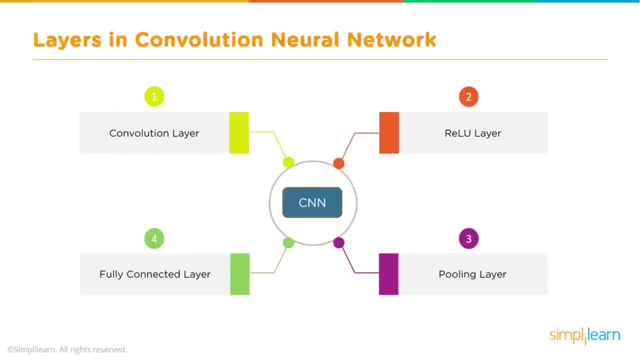 you know, as we talked about the rectified linear unit- We'll talk about that in a little bit later- The relu is how that layer is activated. is the math behind it what makes the neurons fire? You'll see that in a lot of other neural networks When you're using it just by itself. 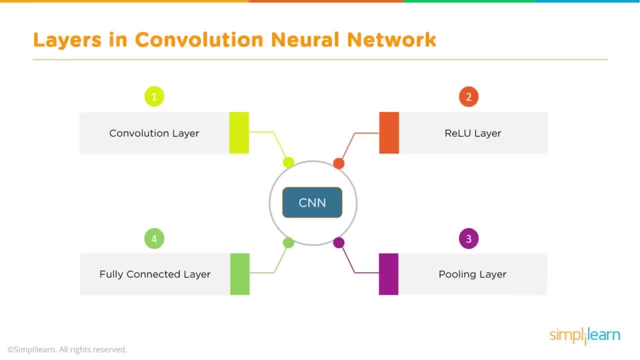 it's for processing smaller amounts of data, where you use the atom activation feature for large data. coming in Now, because we're processing small amounts of data in each image, the relu layer works great. You have your pooling layer. That's where you're pooling the data together. 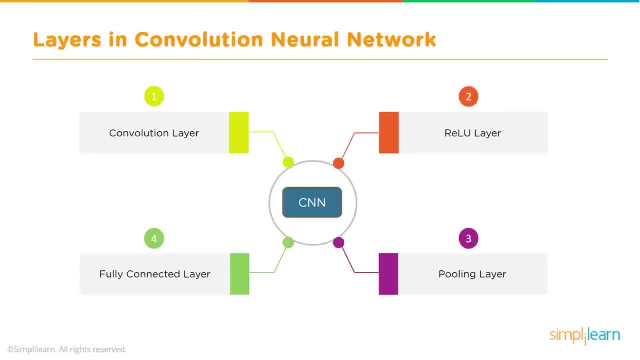 Pooling is a neural network term. It's very commonly used. I like to use the term reduce. So if you're coming from the map and reduce side, you'll see that we're mapping all this data through all these networks And then we're going to reduce it, We're going to pool it together And then finally we have the fully connected layer. 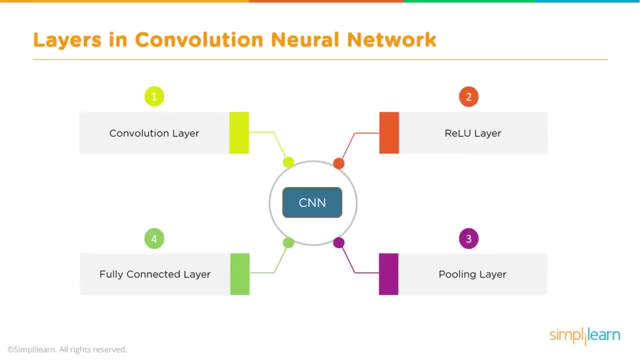 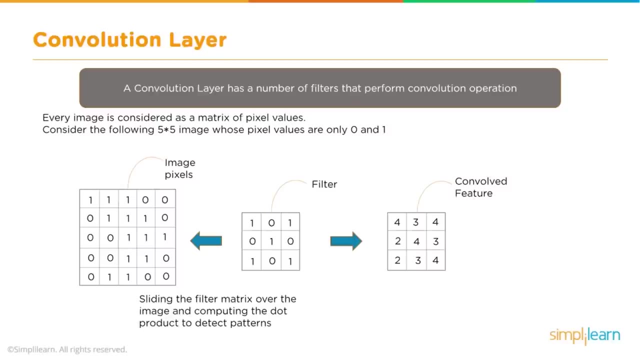 That's where our output is going to come out. So we have started to look at matrices, We've started to look at the convolutional layer and where it fits in and everything. We've taken a look at images. So we're going to focus more on the convolution layer, since this is a convolutional 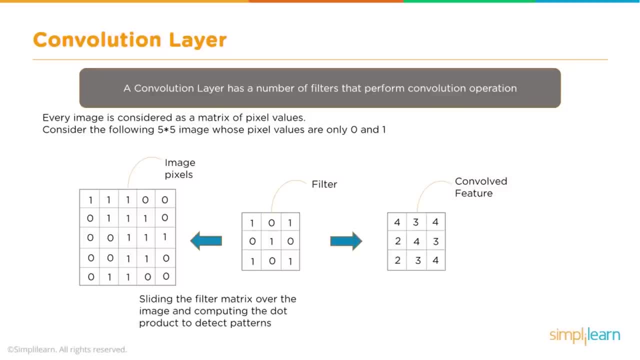 neural network, A convolution layer, has a number of filters and perform convolution operation. Every image is considered as a matrix of pixel values. Consider the following five by five image whose pixel values are only zero and one. Now, obviously, when we're dealing with color, there's all kinds of things that come in on color processing. 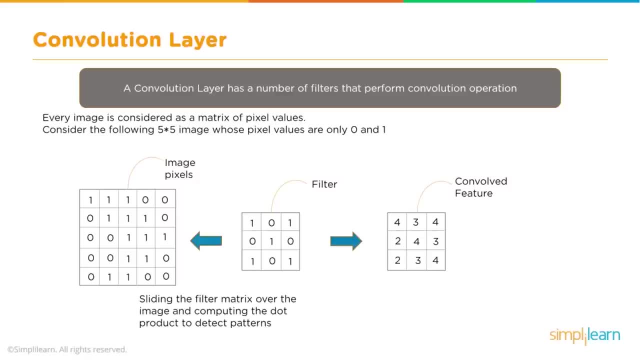 but we want to keep it simple and just keep it black and white. And so we have our image pixels, So we're sliding the filter matrix over the image and computing the dot product to detect the patterns. You're going to ask: where does this filter come from? 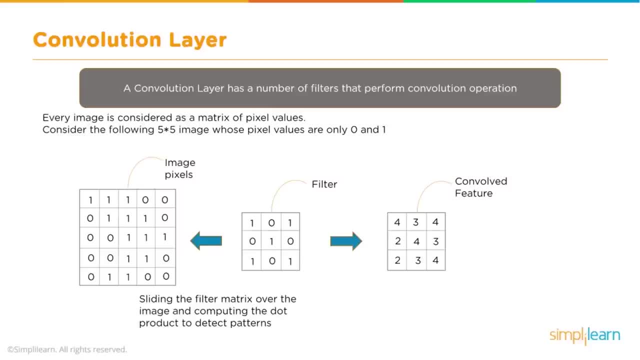 This is a bit confusing because the filter is going to be derived later on. We build the filters when we program or train our model, So you don't need to worry what the filter actually is, But you do need to understand how a convolution layer works. is what is the filter doing? 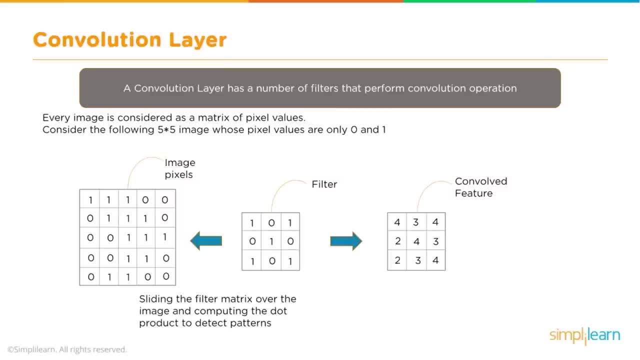 Filter And you'll have many filters. You don't have just one filter. You'll have lots of filters that are going to look for different aspects, And so the filter might be looking for just edges. It might be looking for different Parts. will cover that a little bit more detail in a minute. 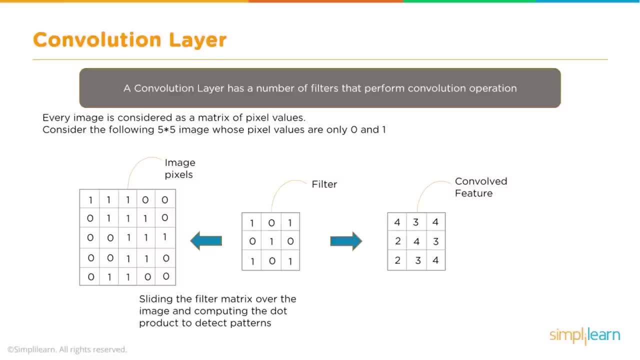 Right now we're just focusing on how the filter works as a matrix. Remember, earlier we talked about multiplying matrices together And here we have our two dimensional matrix And you can see we take the filter and we multiply it in the upper left image. 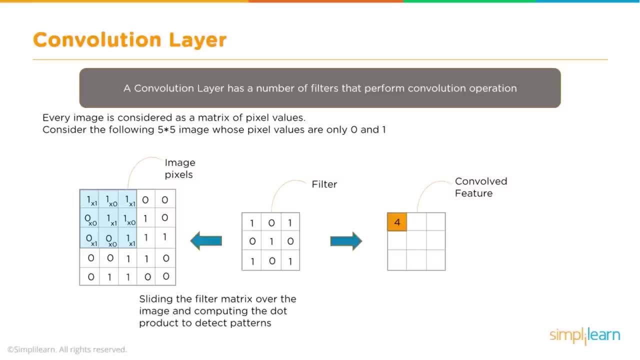 And you can see right here: one times one, one times zero, one times one. We multiply those all together, then some of them, and we end up with the convolved feature of four. We're going to take that and sliding the filter matrix over the image and computing the dot. 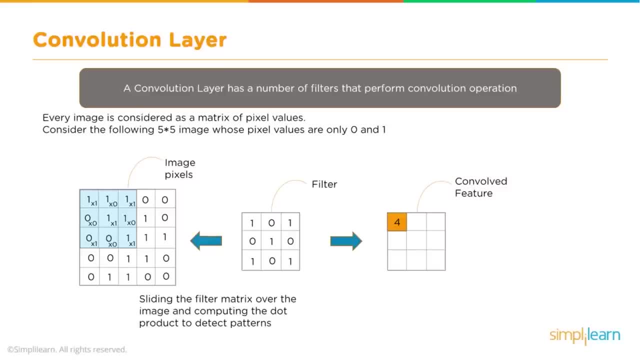 product to detect patterns. So we're just going to slide this over. We're going to predict the first one and slide it over one notch, Predict the second one, and so on and so on, all the way through until we have a new matrix. 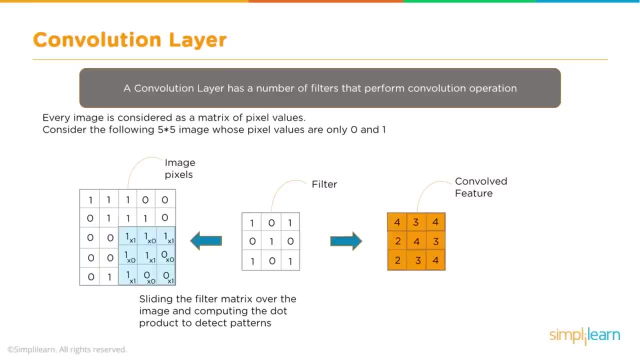 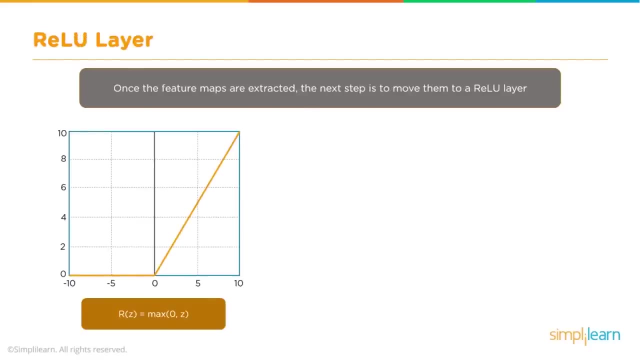 And this matrix, which is the same size as a filter, has reduced the image. And whatever filter, whatever that's filtering out, is going to be looking at just those features reduced down to a smaller matrix. So once the feature maps are extracted, the next step is to move them to the 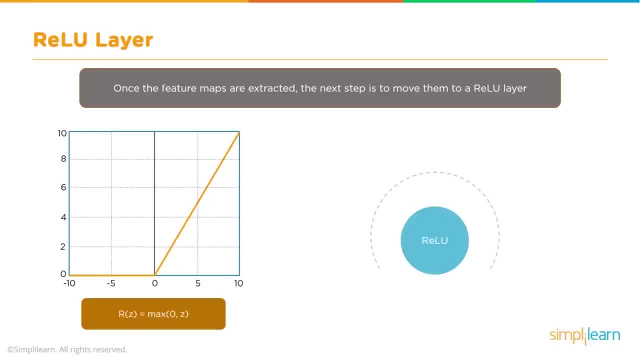 ReLU layer. So the ReLU layer. the next step first is going to perform an element wise operation. So each of those maps coming in, if there's negative pixels, so it sets all the negative pixels to zero And you can see this nice graph where it just zeroes out the negatives and then you have. 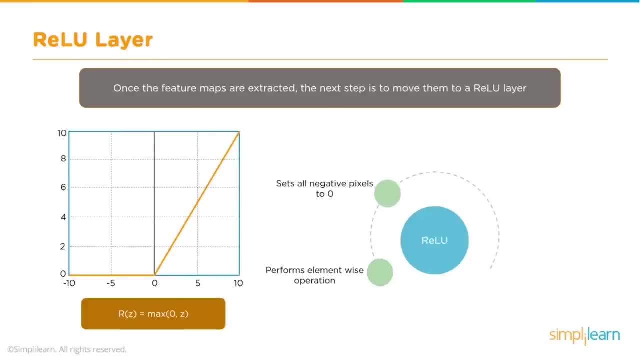 a value that goes from zero up to whatever value is coming out of the matrix. This introduces non-linearity to the network. So up until now we have a. we say linearity. We're talking about the fact, The fact that the feature has a value. 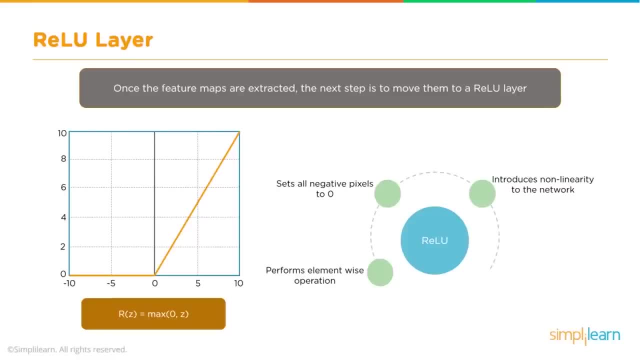 So it's a linear feature. This feature came up and it has. let's say, the feature is the edge of the beak or the backslash that we saw. You'll look at that and say, okay, this feature has a value from negative 10 to 10 in this. 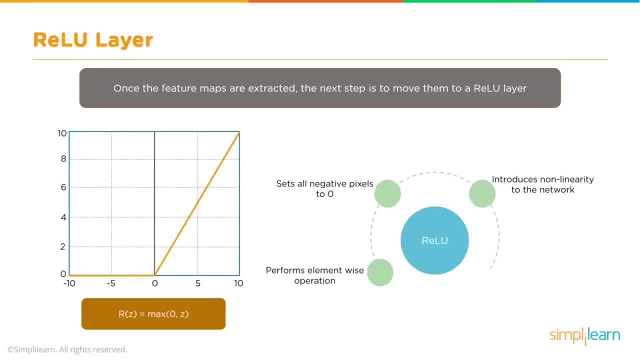 case. If it was one, it'd say, yeah, this might be a beak, It might not, It might be an edge right there. A minus five means no, we're not even going to look at it, It's a zero. 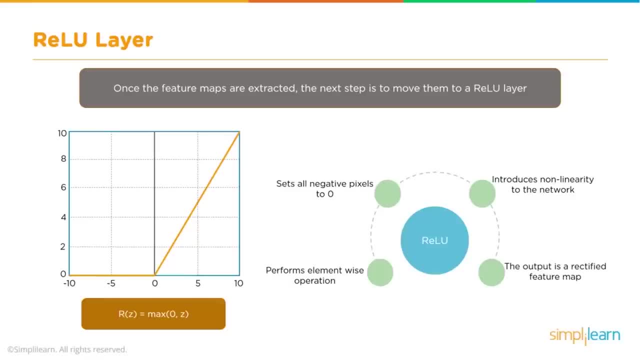 And so we end up with an output, and the output takes all these features, all these filtered features. Remember, we're not just running one filter on this, We're running a number of filters on this image, And so we end up with an rectified feature map that is looking at just the features coming. 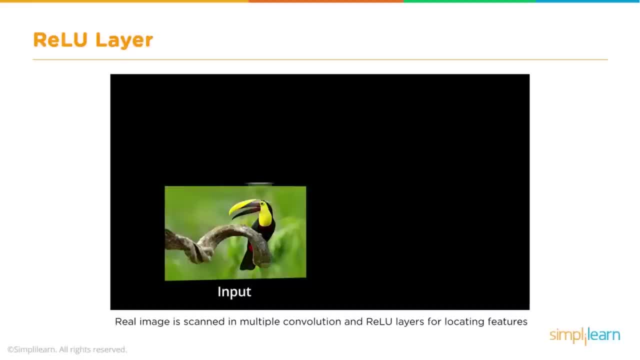 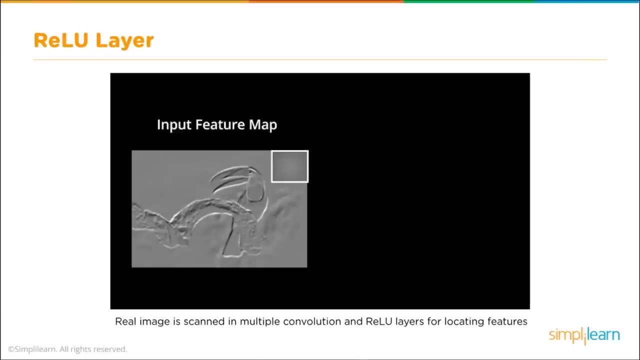 through and how they weigh in from our filters. So here we have an input of a. it looks like a toucan bird, very exotic looking Real image is scanned in multiple convolution and the relu layers for locating features And you can see up here is turn it into a black and white image. 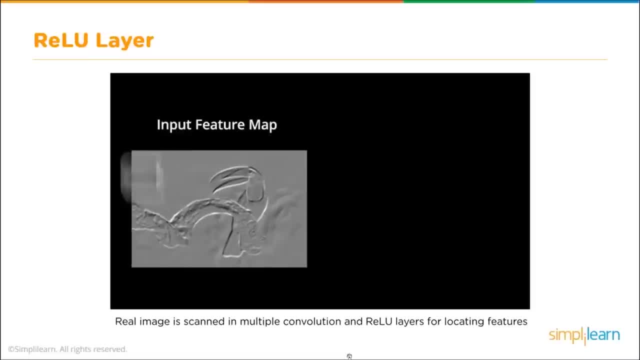 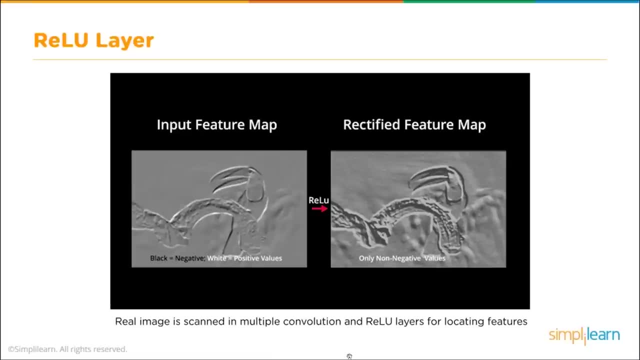 And in this case we're looking in the upper right-hand corner. We're looking in the upper right-hand corner for a feature and that box scans over A lot of times. it doesn't scan one pixel at a time. A lot of times it will skip by two or three or four pixels to speed up the process. 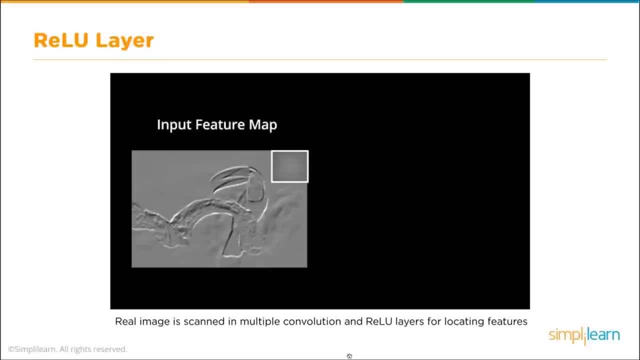 That's one of the ways you can compensate if you don't have enough resources on your computation for large images. And it's not just one filter slowly goes across the image. You have multiple filters that have been programmed in there, So you're looking at a lot of different filters going over the different aspects of the image. 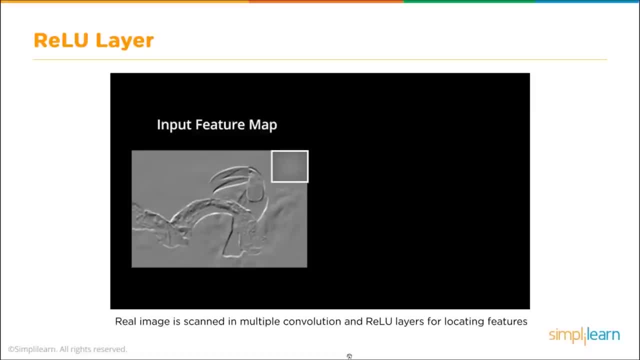 and just sliding across there and forming a new matrix. One more aspect to note about the relu layer is we're not just having one relu coming in, So not only do we have multiple features going through, but we're generating multiple relu layers for locating the features. 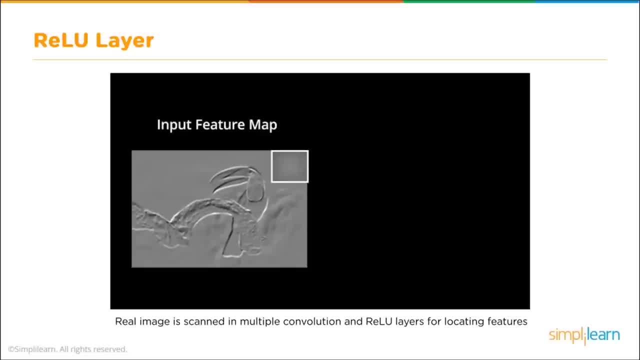 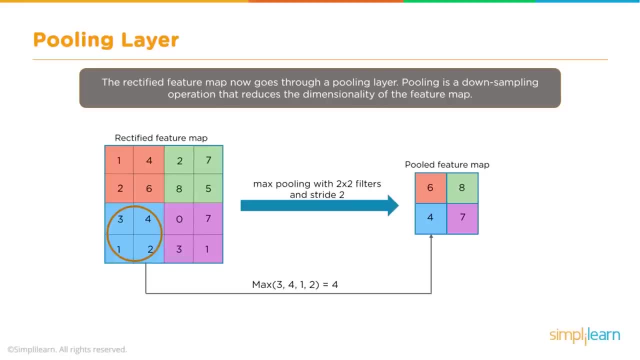 That's very important to note. So we have quite a bundle. We have multiple filters, multiple relu, which brings us to the next step: forward: propagation. Now we're going to look at the pooling layer. The rectified feature map now goes through a pooling layer. 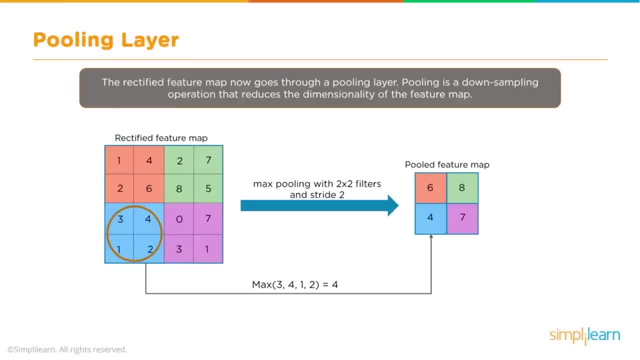 Pooling is a downsampling operation that reduces the dimensionality of the feature map. That's all we're trying to do. We're trying to take a huge amount of information and reduce it down to a single answer. This is a specific kind of bird. 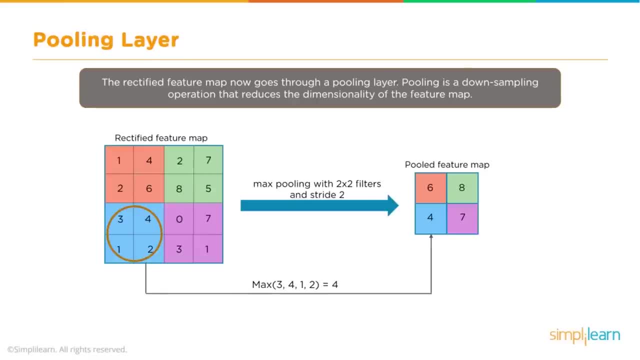 This is an iris, This is a rose. So you have a rectified feature map And you see, here we have a rectified feature map coming in. We set the max pooling with a two by two filters and a stride of two. And, if you remember correctly, I talked about not going one pixel at a time. 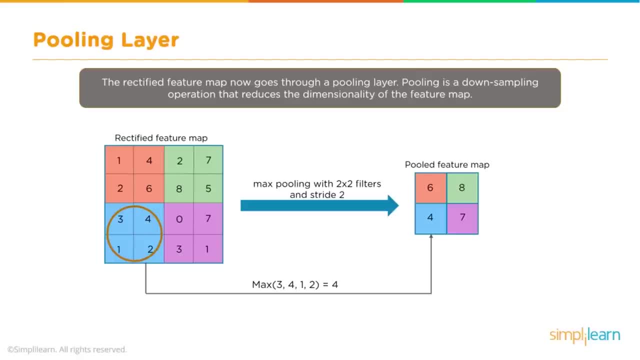 Well, that's where the stride comes in. We end up with a two by two pooled feature map, but instead of moving one over each time and looking at every possible combination, we skip a few. there, We go by two. We skip every other pixel. 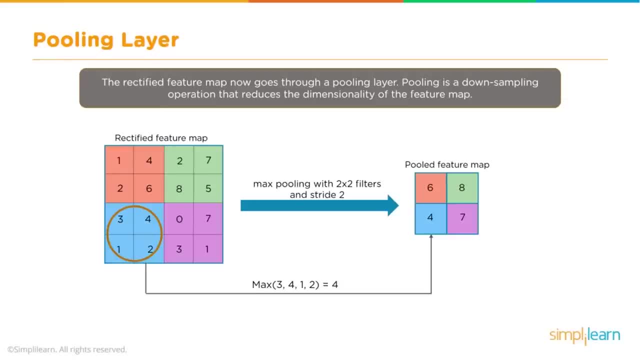 And we just do every other one, And this reduces our rectified feature map which, as you can see over here, 16 by 16 to a four by four. So we're continually trying to filter and reduce our data so that we can get to something. 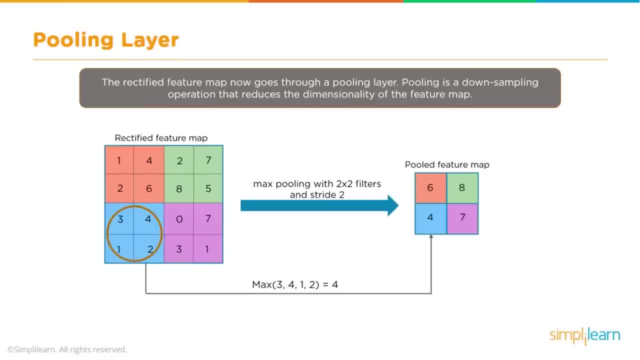 we can manage, And over here you see that we have the max filter And that's where the stride comes in. We have the max three, four, one and two, And in the max pooling we're looking for the max value a little bit different than 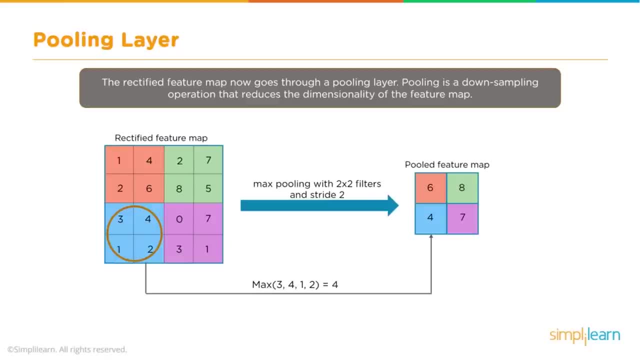 what we were looking at before. So, coming from the rectified feature, we're now finding the max value, and then we're pooling those features together. So, instead of thinking of this as image of the map, think of this as: how valuable is a feature in that area? 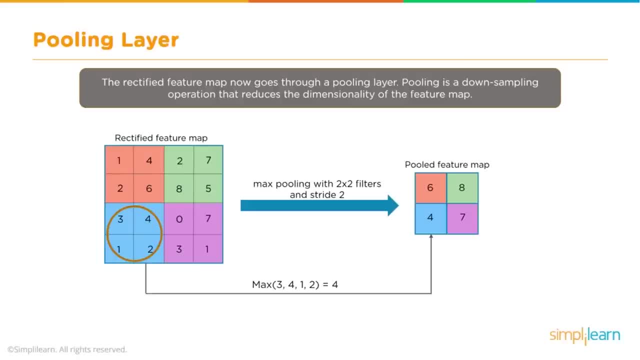 How much of a feature value do we have And we just want to find the best or the maximum feature for that area. It might have that one piece of the filter of the beak set up. I see a one in this beak, in this image, and then it skips over and says I see a three. 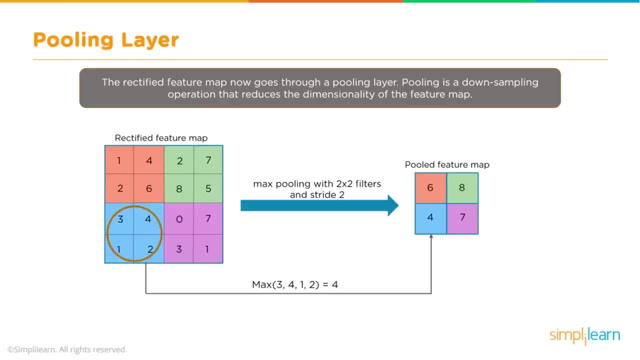 in this image and says: oh, this one is rated as a four. We don't want to sum it together because then you know you might have like five ones and it'll say, ah, five, but you might have four zeros and one 10.. 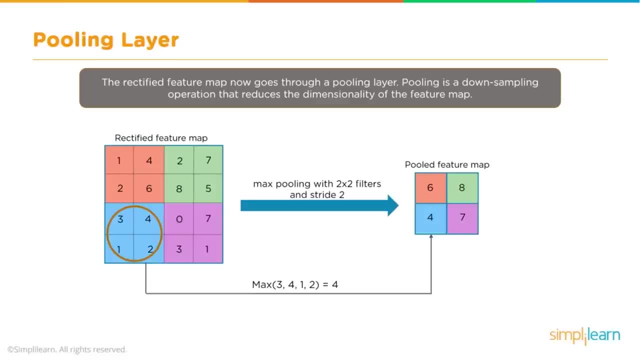 And that 10 says, well, this is definitely a beak, where the ones will say: probably not a beak. A little strange analogy, since we're looking at a bird, but you can see how that pooled feature map comes down and we're just looking for the max value in each one of those matrixes. 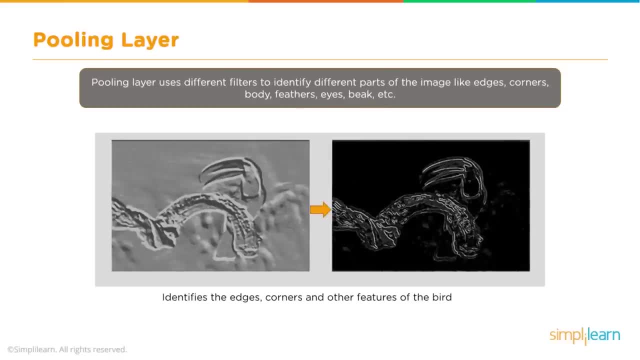 Cool. So this is different filters to identify different parts of the image, like edges, corners, body feathers, eyes, beak, et cetera. I know I focus mainly on the beak, but obviously each feature could be a different part of. 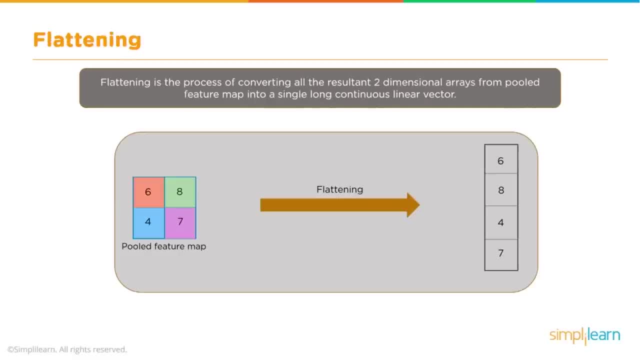 the bird coming in. So let's take a look at what that looks like. Structure of a convolution neural network. so far, This is where we're at right now. We have our input image coming in and then we use our filters, and there's multiple filters. 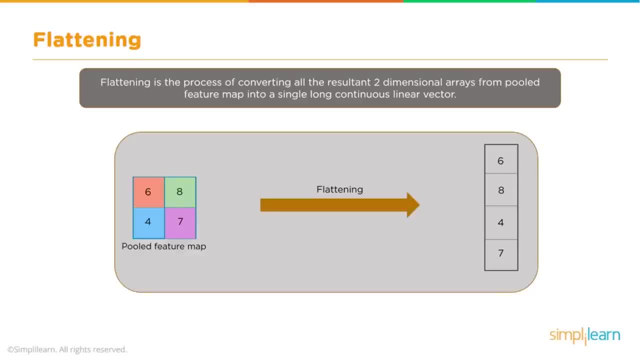 on there that are being developed To kind of twist. We're going to go ahead and change that data and so we multiply the matrixes. We take that little filter- Maybe it's a two by two- We multiply it by each piece of the image and if we step two then it's every other. 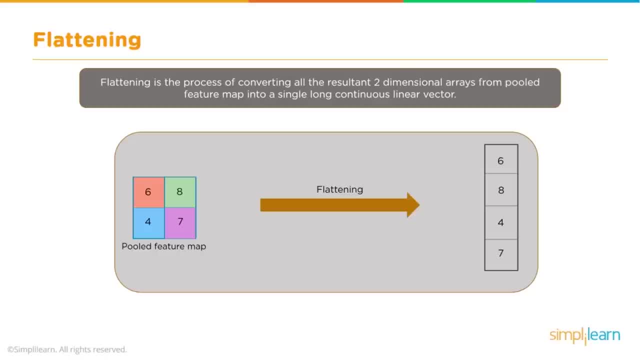 piece of the image That generates multiple convolution layers. So we have a number of convolution layers we have set up in there. just looking at that data, We then take those convolution layers, We run them through the ReLU setup and then, once we've done through the ReLU setup and 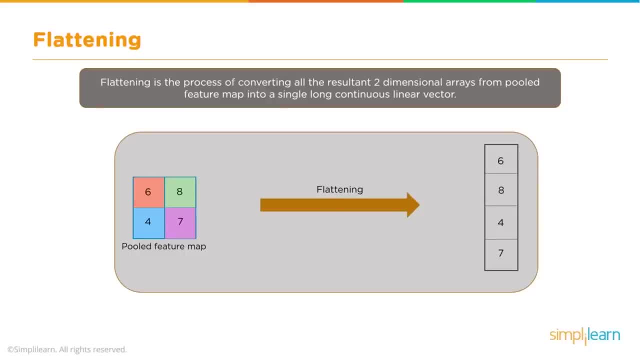 we have multiple ReLUs going on, multiple layers that are ReLU, Then we're going to take those multiple layers and we're going to be pooling them. So now we have the pooling layers, or multiple poolings, going on Up until this point we're dealing with- sometimes it's multiple dimensions- 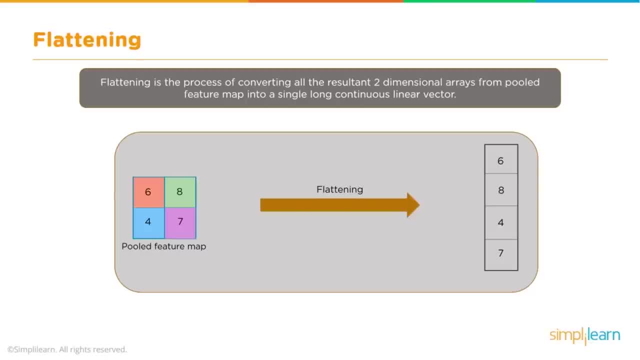 You can have three dimensions- some strange data setups that aren't doing images but looking at other things. They can have four, five, six, seven dimensions. So right now we're looking at 2D image dimensions coming in into the pooling layer. 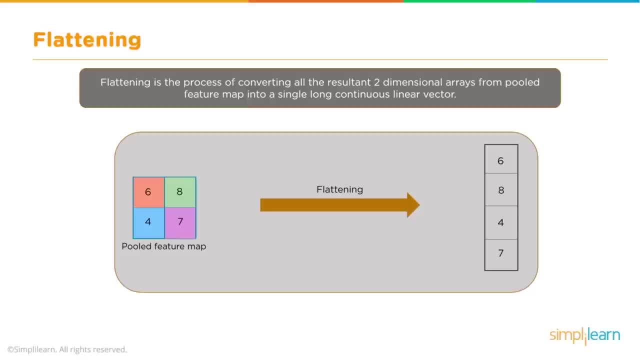 So the next step is: we want to reduce those dimensions or flatten them. So flattening. Flattening is a process of converting all of the resultant dimensions. Flattening is a process of converting all of the resultant dimensions. Flattening is a process of converting all of the resultant dimensions. 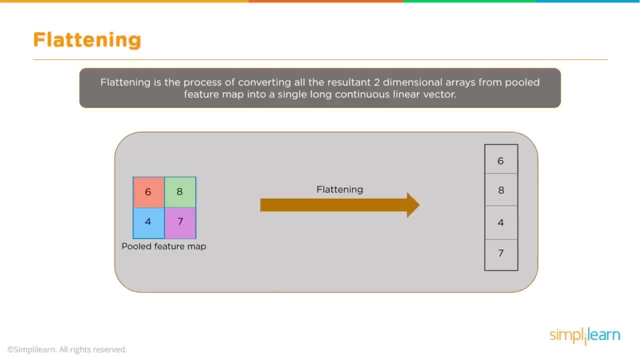 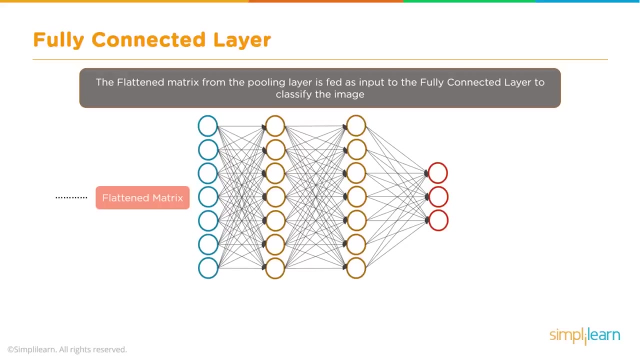 So flattening is a process of converting all of the resultant navigations and внимational dimensions into a single component. The second step of flattening is to refrigerate Error край over, and we'd like to get a convolutional worldview, and we don't need to do that right now. 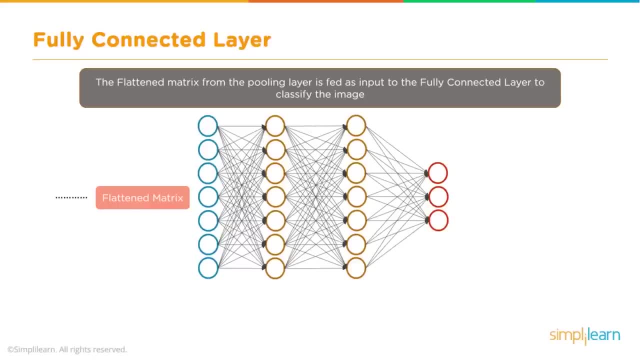 So we'll talk a little bit about transformation. So function has been found in the Hangout template namedßиш 2020, the most popular publication for visualization and Video Reels forks, and that is a tab that's at the top of your rating. 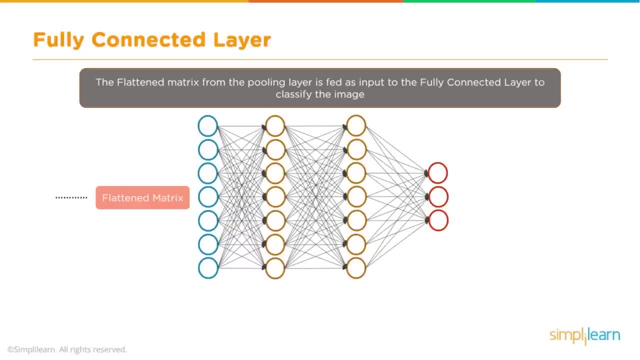 and we have the input layer into the next setup. All we've done is taken all those different pooling layers and we've flattened them out and combined them into a single linear vector going in. So after we've done the flattening we have just a quick recap. 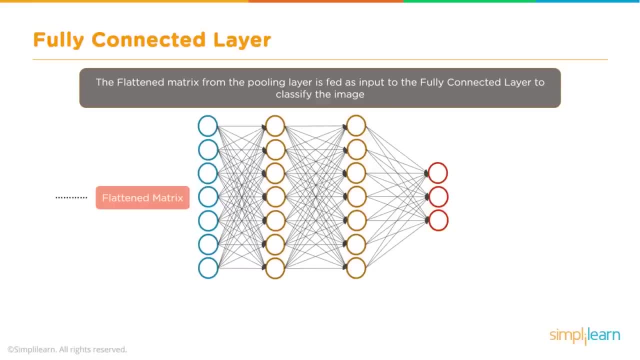 because we've covered so much. so it's important to go back and take a look at each of the steps we've gone through. The structure of the network so far is we have our convolution, where we twist it and we filter it and multiply the matrices. 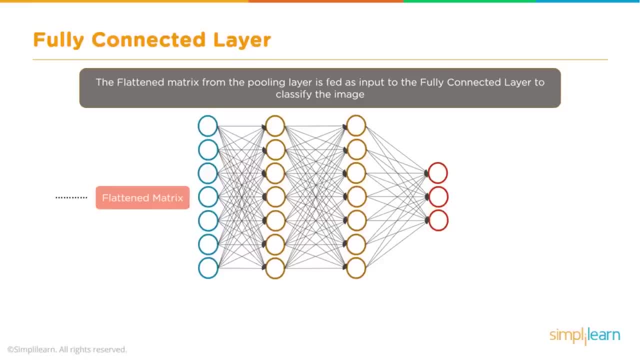 We end up with our convolutional layer, which uses the relu to figure out the values going out into the pooling, because you have numerous convolution layers that then create numerous pooling layers pooling that data together, which is the max value, which one we want to send forward. we want to send the best value. 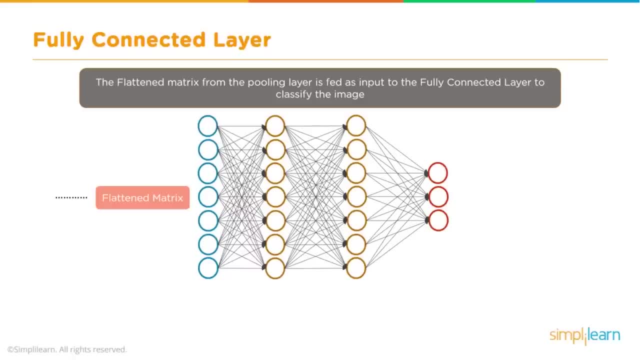 And then we're going to take all of that from each of the pooling layers and we're going to flatten it and we're going to combine them into a single input going into the final layer. Once you get to that step, you might be looking at that going. 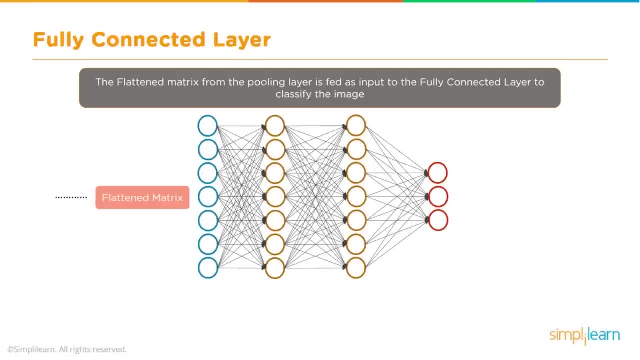 boy, that looks like the normal intuit. but to most neural network- and you're correct, it is So once we have the flattened matrix from the pooling layer, that becomes our input. so the pooling layer is fed as an input to the fully connected layer to classify the image. 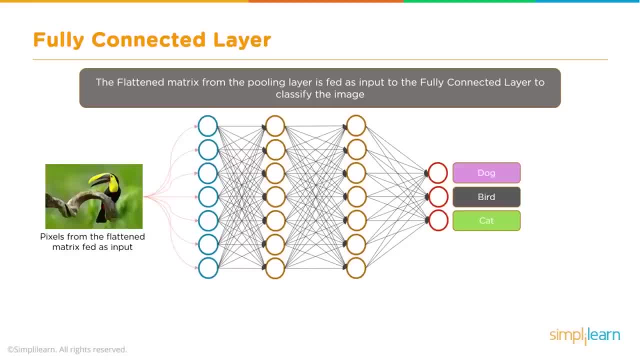 And so you can see as our flattened matrix comes in. in this case we have the pixels from the flattened matrix fed as an input back to our toucan or whatever that kind of bird that is. I need one of these to identify what kind of bird that is. 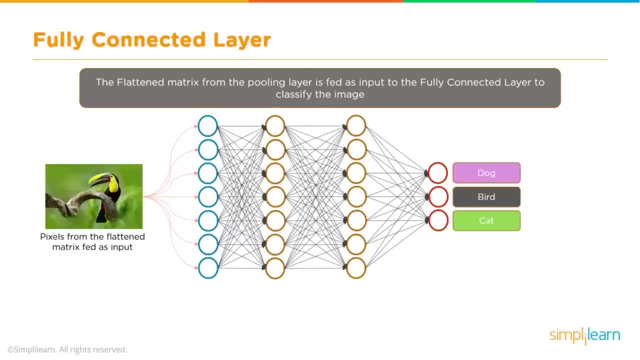 It comes into our forward propagation network and that will then have the different weights coming down across, and then finally it selects that that's a bird and that it's not a dog or a cat, in this case, Even though it's not labeled. the final layer there in red is our output layer. 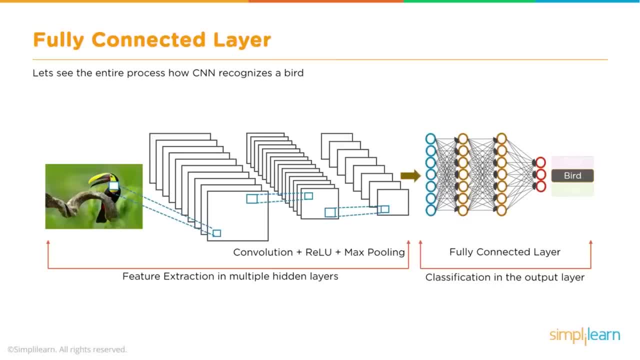 our final output layer that says bird, cat or dog. So quick recap of everything we've covered so far. we have our input image which is twisted and multiplied. the filters are multiplied times. the two matrices multiplied all the filters to create our convolution layer. 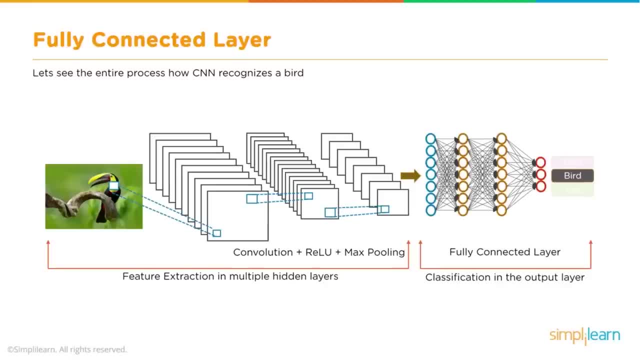 Our convolution layer. there's multiple layers in there because it's all building multiple layers off the different filters, then goes through the ReLU and this is activation and that creates our pooling. And so once we get into the pooling layer, 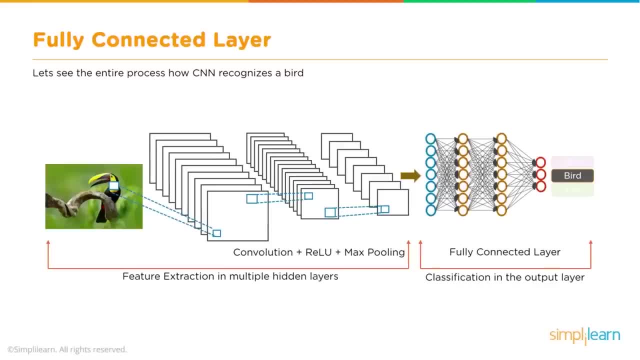 we then in the pooling, look for who's the best, what's the max value coming in from our convolution, and then we take that layer and we flatten it and then it goes into a fully connected layer, our fully connected neural network, and then to the output. 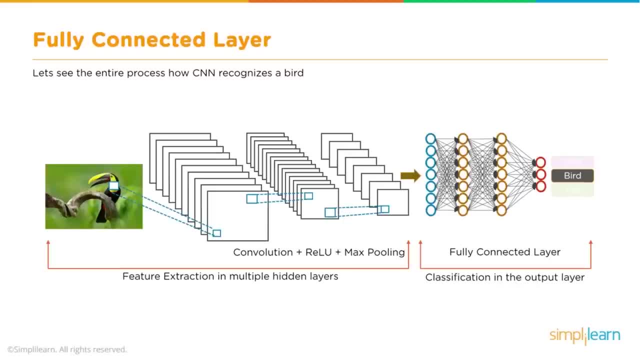 And here we can see the entire process: how the CNN recognizes a bird. This is kind of nice because it's showing the little pixels and where they're going. You can see the filter is generating this convolution network and that filter shows up in the bottom part of the convolution network. 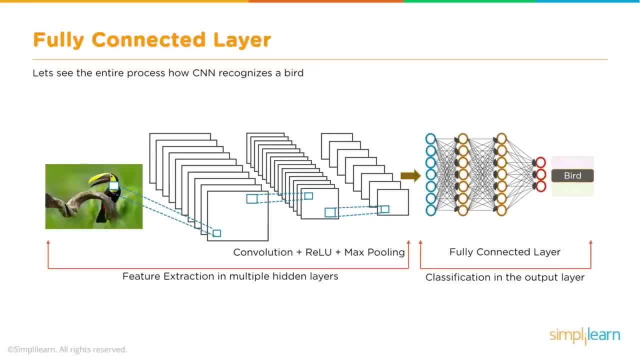 And then, based on that, it uses the ReLU for the pooling. the pooling then find out which one's the best, and so on all the way to the fully connected layer at the end, or the classification and the output layer. So that'd be a classification neural network at the end. 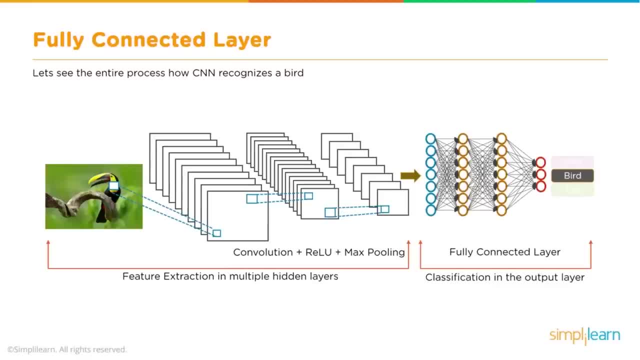 So we covered a lot of theory up till now and you can imagine each one of these steps has to be broken down in code, So putting that together can be a little complicated, not that each step of the process is overly complicated, but because we have so many steps. 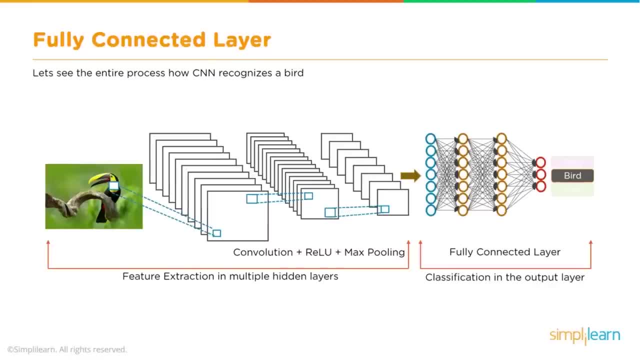 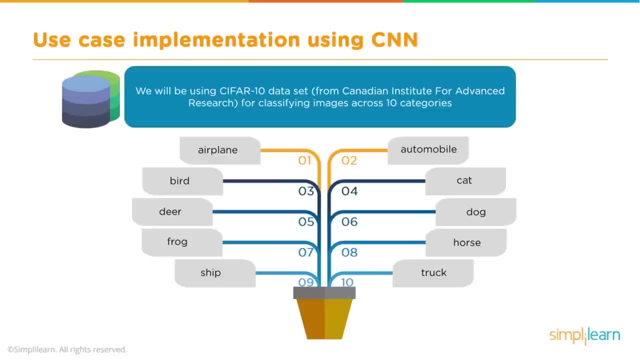 We have one, two, three, four, five different steps going on here with sub steps in there. We're going to break that down and walk through that in code. So in our use case implementation using the CNN, we'll be using the CIFAR-10 data set from Canadian Institute for Advanced Research. 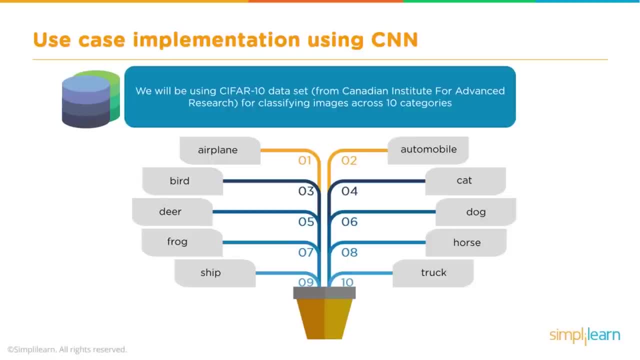 for classifying images across 10 categories. Unfortunately, they don't let me know whether it's going to be a toucan or some other kind of bird, but we do get to find out whether it can categorize between a ship, a frog. 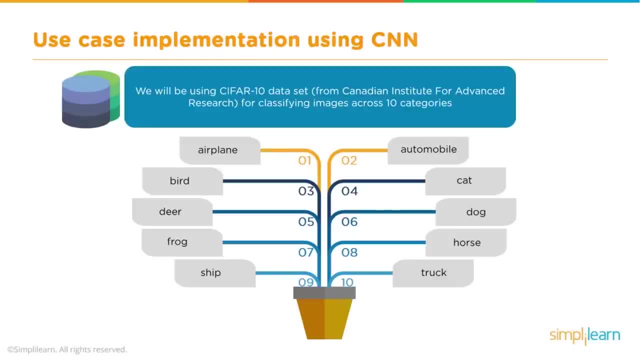 deer, bird, airplane, automobile, cat, dog, horse, truck, So that's a lot of fun. And then if you're looking anything in the news at all of our automated cars and everything else, you can see where this kind of processing is so important in today's world and very cutting edge. 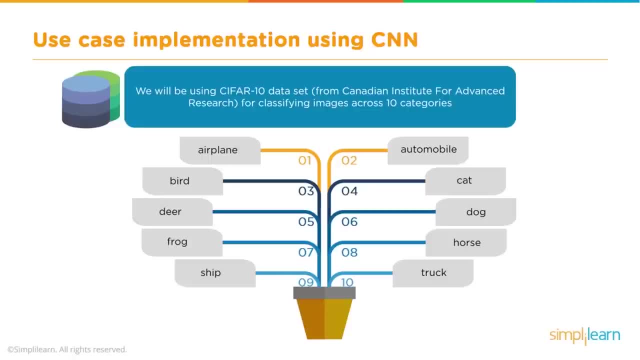 As far as what's coming out in the commercial deployment. I mean, this is really cool stuff. We're starting to see this just about everywhere in industry, So great time to be playing with this and figuring it all out. Let's go ahead and dive into the code and see what that looks like when we're actually writing our script. 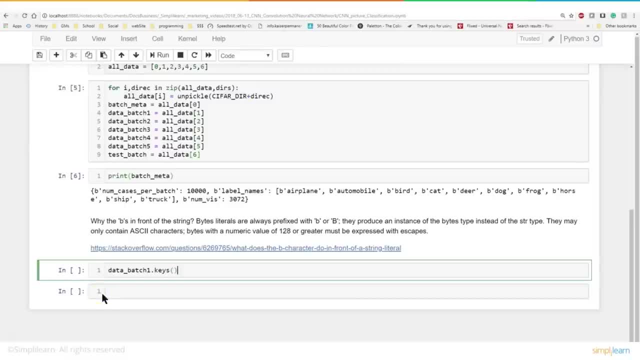 Before we go on, let's do one more quick look at what we have here. Let's just take a look at data batch one keys And remember Jupyter Notebook. I can get by with not doing the print statement If I put a variable down there. 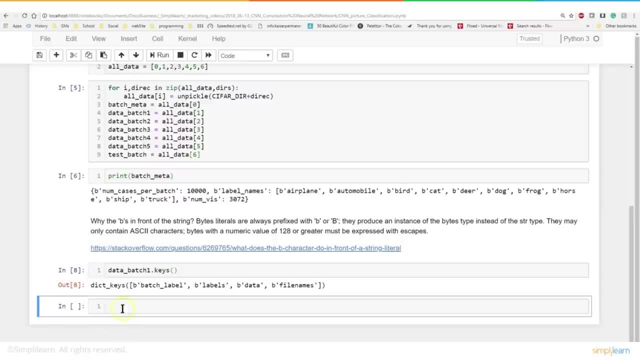 it'll just display the variable And you can see in our data batch one for the keys. since this is a dictionary, we have the batch one- label, data and file names. So you can actually see how it's broken up in our data set. 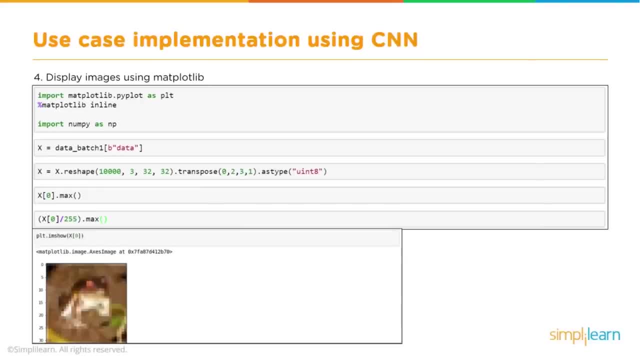 So for the next step, or step four as we're calling it, we want to display the image using matplot library. There's many ways to display the images. You could even well there's other ways to drill into it, but matplot library is really good for this. 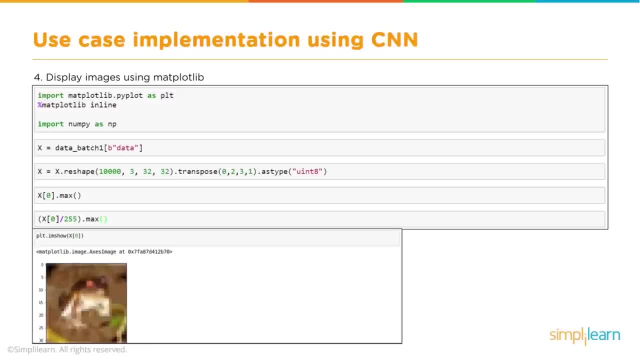 And we'll also look at our first reshape setup, or shaping the data, So you can have a little glimpse into what that means. So we're going to start by importing our matplot And, of course, since I am doing, Jupyter Notebook. 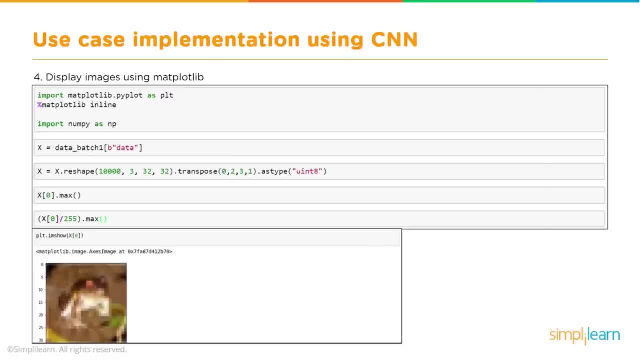 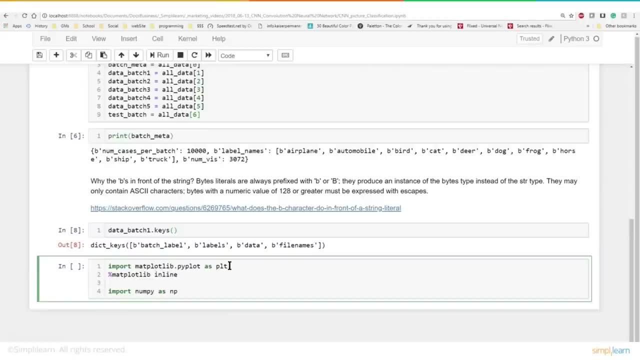 I need to do the matplot inline command, So it shows up on my page. So here we go. We're going to import matplot librarypyplot as plt. And if you remember matplot library, the pyplot is like a canvas that we paint stuff onto. 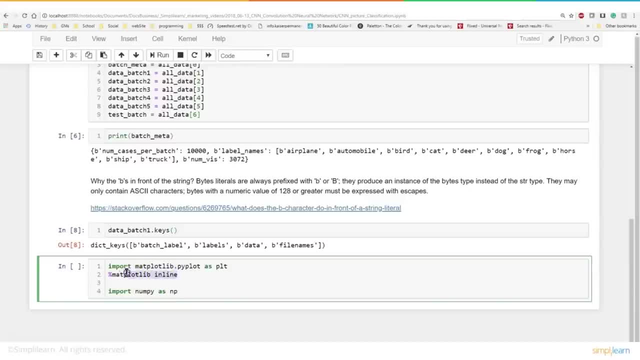 And there's my percentage sign matplot library inline, So it's going to show up in my notebook. And then, of course, we're going to import numpy as np for our numbers, Python array setup. And let's go ahead and set: x equals to. 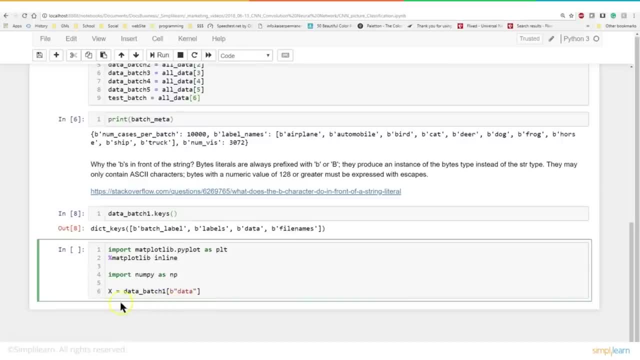 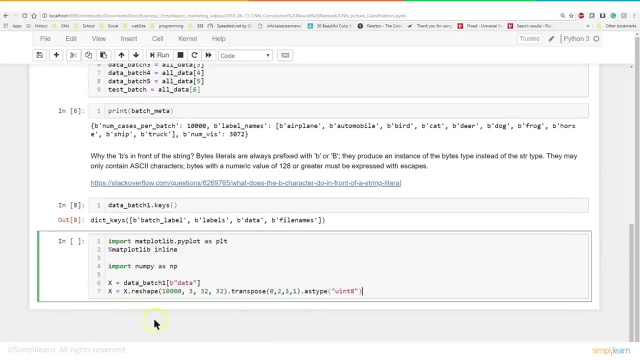 data, batch one. So this will pull in all the data going into the x value. And then, because this is just a long stream of binary data, we need to go a little bit of reshaping. So in here we have to go ahead and reshape the data. 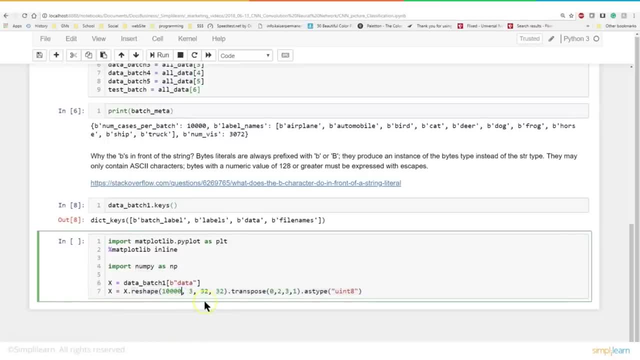 We have 10,000 images. Okay, that looks correct And this is kind of an interesting thing. It took me a little bit to. I had to go research this myself to figure out what's going on with this data And what it is. 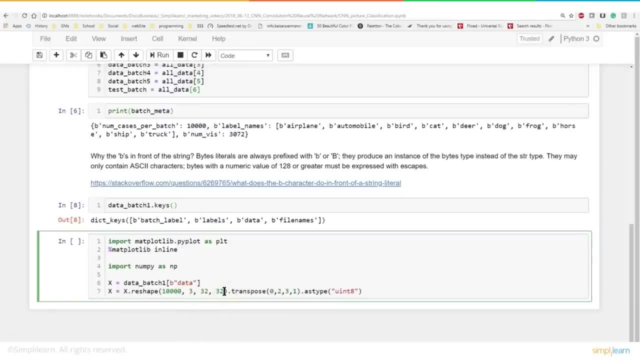 is. it's a 32 by 32 picture And let me do this, Let me go ahead and do a drawing pad on here. So we have 32 bits by 32 bits and it's in color. So there's three bits of color. 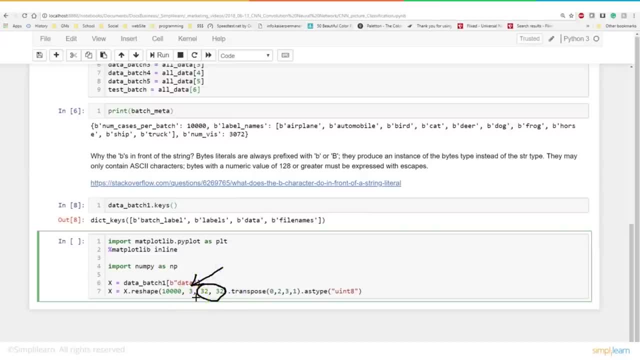 Now, I don't know why the data is particularly like this. It probably has to do with how they originally encoded it, But most pictures put the three afterward. So what we're doing here is we're going to take the shape, we're going to take the data, which is just a long stream of information. 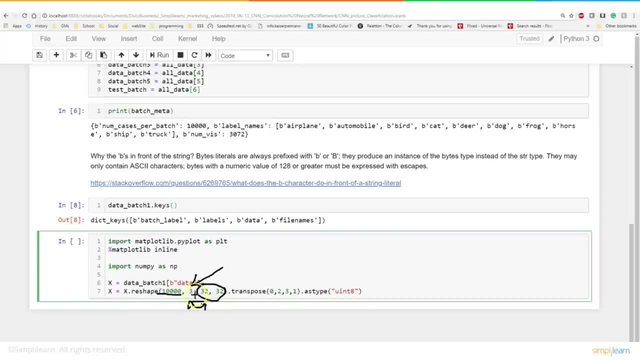 And we're going to break it up into 10,000 pieces, And those 10,000 pieces then are broken into three pieces each, And those three pieces then are 32 by 32.. You can look at this like an old fashioned projector, where they have the red screen. 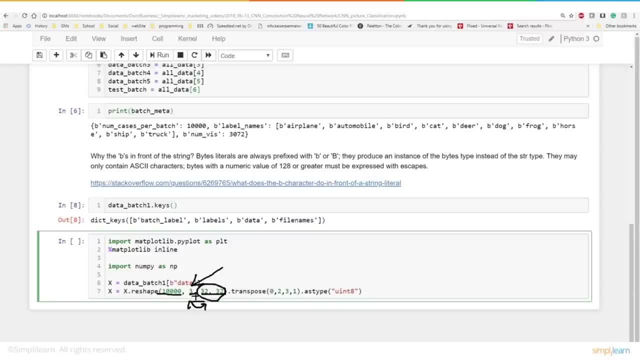 or the red projector, the blue projector and the green projector, and they add them all together And each one of those is a 32 by 32 bit. So that's probably how this was originally formatted. was in that kind of ideal? 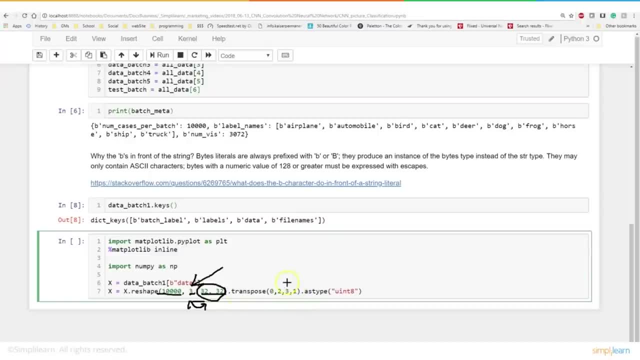 Things have changed So we're going to transpose it and we're going to take the three which was here and we're going to put it at the end. So the first part is reshaping the data from a single line, a bit data or whatever format it is, into 10,000 by three by 32 by 32.. 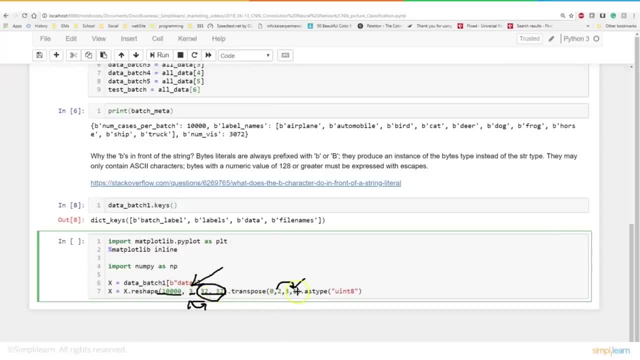 And then we're going to transpose the color factor to the last place, So it's the image, then the 32 by 32 in the middle. That's this part right here. And then, finally, we're going to take this, which is three bits of data, and put it at the end. 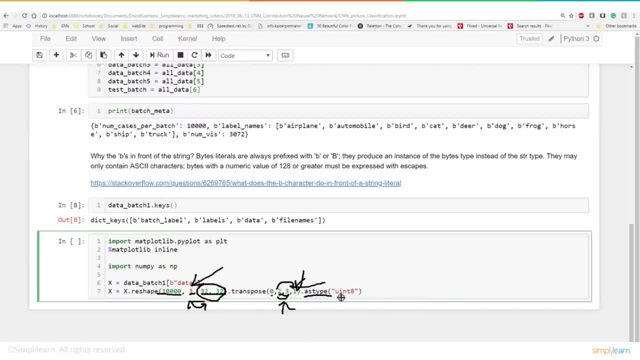 So it's more like we do the process images now And then as type. this is really important that we're going to use an integer eight. So I'm going to come in here and you'll see a lot of these. they'll try to do this with a float or a float 64.. 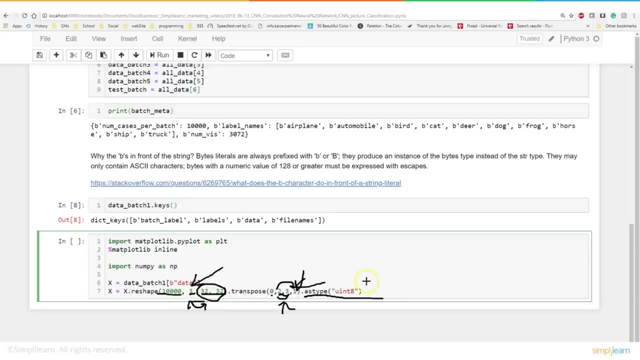 What you got to remember, though, is a float uses a lot of memory, So once you switch this into something that's not integer eight- which is goes up to 128, you are just going to the amount of RAM. let me just put that in here. 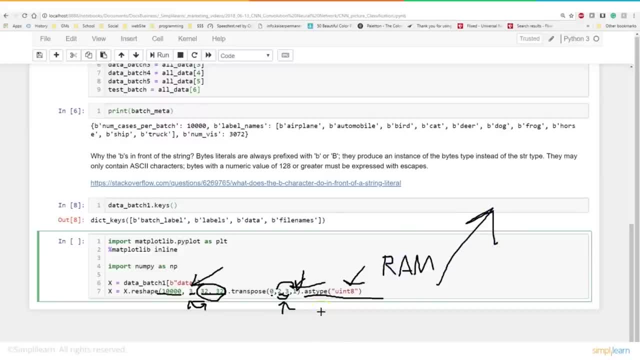 is going to go way up the amount of RAM that it loads, So you want to go ahead and use this. You can try the other ones and see what happens. if you have a lot of RAM on your computer For this exercise, this will work just fine. 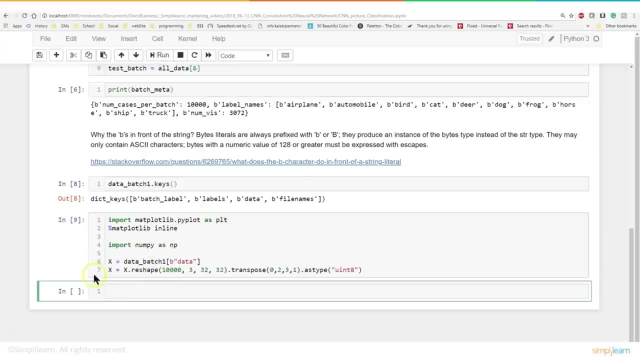 And let's go ahead and take that and run this. So now our X variable is all loaded and it has all the images in it from the batch one data batch one. And just to show we are talking about with the as type on there: 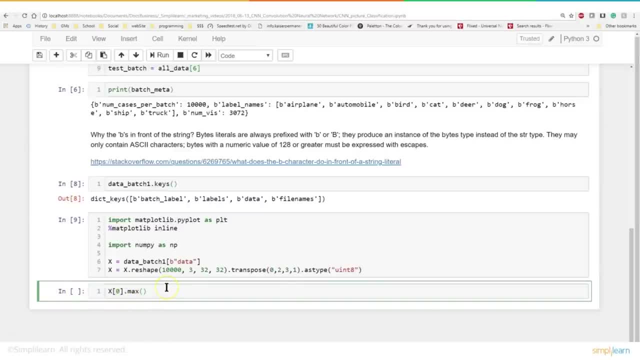 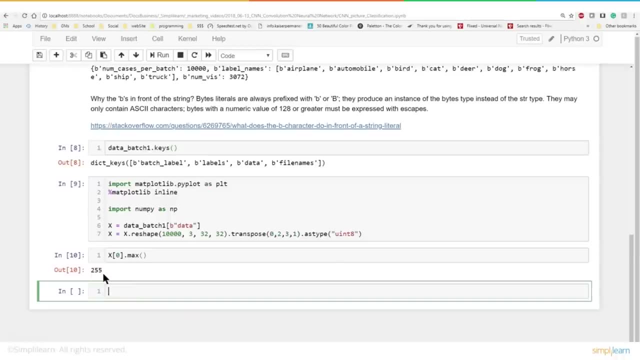 if we go ahead and take X zero and just look for its max value, let me go ahead and run that. You'll see it doesn't. oops, I said 128, it's 255.. You'll see, it doesn't go over 255,. 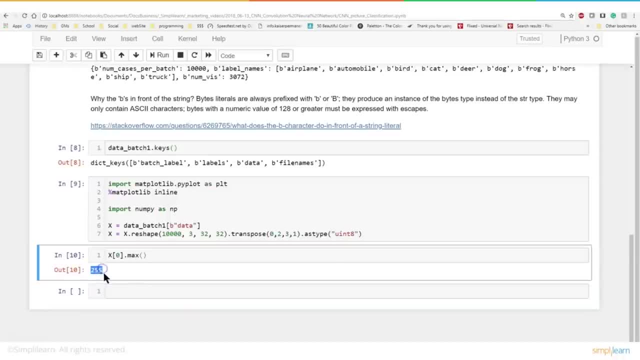 because it's basically an ASCII character is what we're. we're keeping that down to. we're keeping those values down. So they're only 255, 0 to 255, versus a float value which would bring this up exponentially in size. 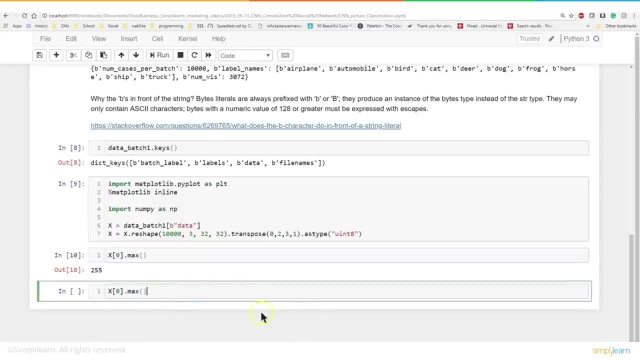 And since we're using the matplot library, we can do: oops, that's not what I wanted. Since we're using the matplot library, we can take our canvas and just do a pltim for image show. And let's just take a look at what X zero looks like. 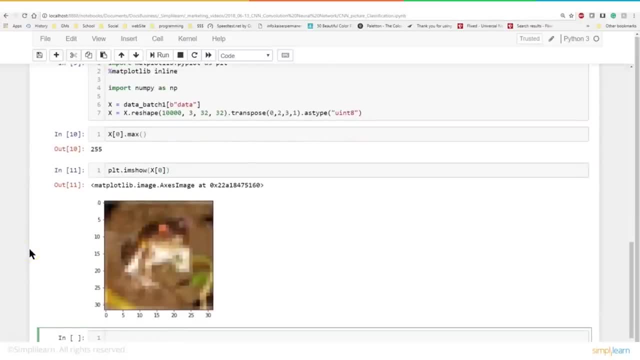 And it comes in. I'm not sure what that is, but you can see it's a very low grade image broken down to the minimal pixels on there, And if we did the same thing, oh, let's do. let's see what one looks like. 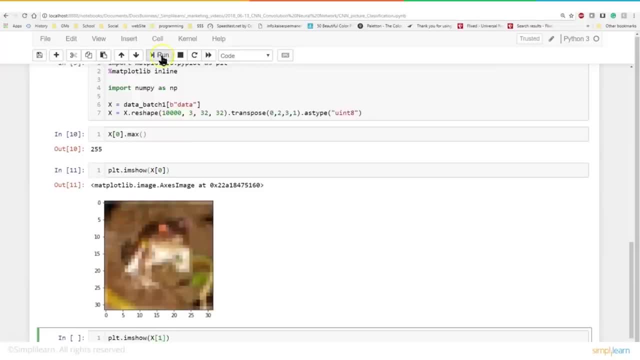 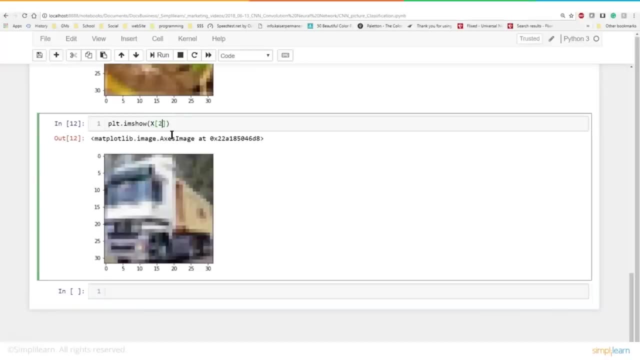 Hopefully it's a little easier to see. Run on there, not enter. Let's hit the run on that And we can see this is probably a semi truck. That's a good guess on there And I can just go back up here instead of typing the same line in over and over. 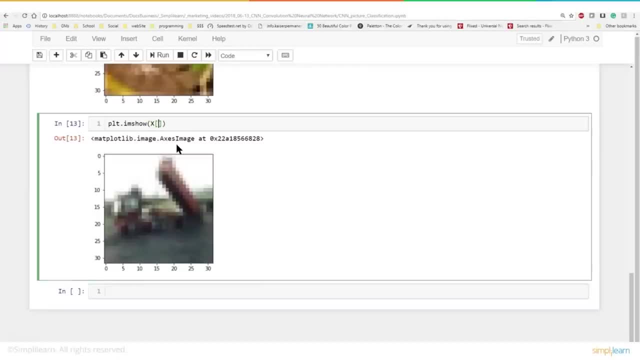 And we'll look at three. That looks like a dump truck unloading and so on. You can do any of the 10,000 images. We can just jump to 55. It looks like some kind of animal looking at us there. 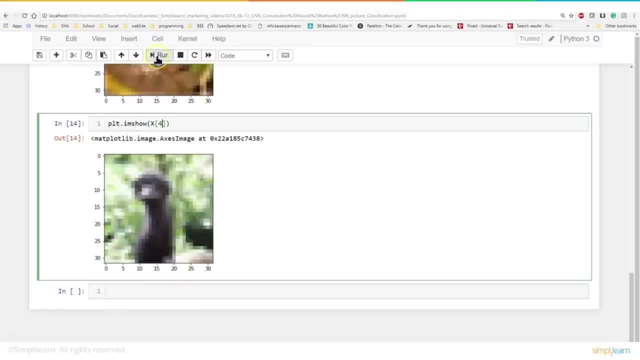 probably a dog, And just for fun, let's do just one more run on there And we can see a nice car for our image number four. So you can see we paced through all the different images. It's very easy to look at them. 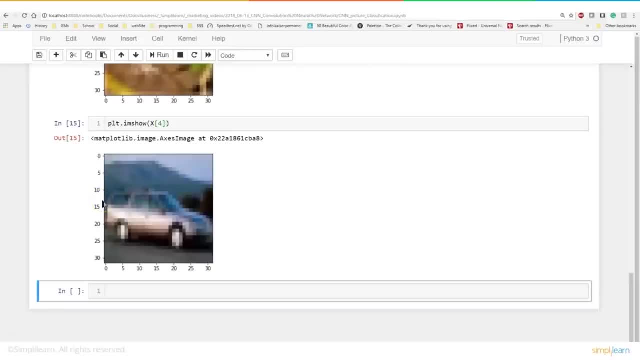 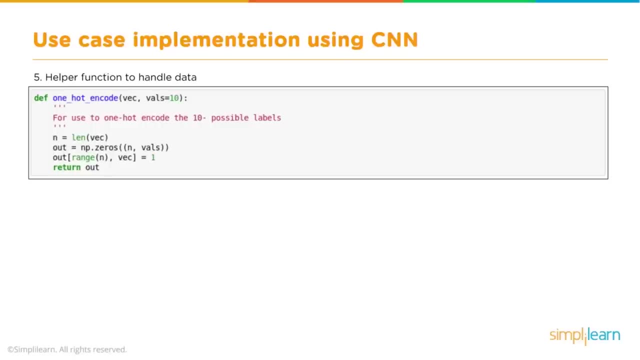 And they've been reshaped to fit our view and what the Matplot library uses for its format. So the next step is we're going to start creating some helper functions. We'll start by a one hot encoder to help us more processing the data. 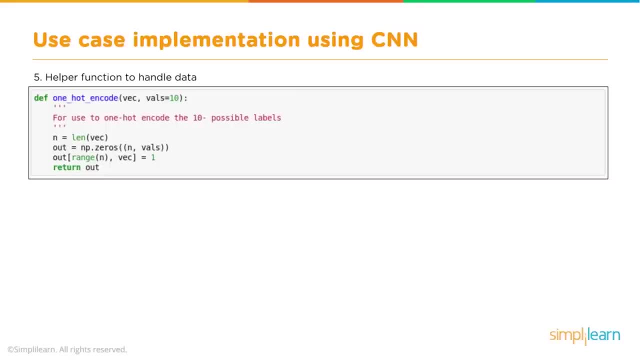 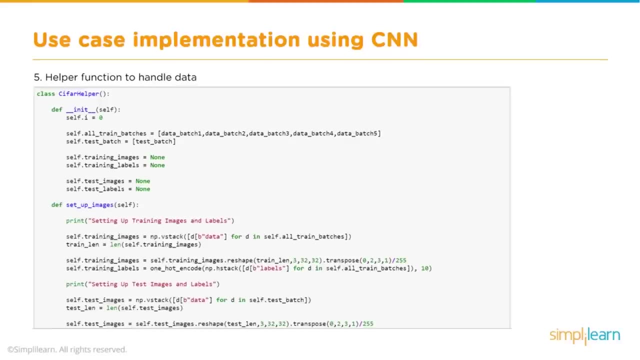 Remember that your labels, they can't just be words, They have to switch it And we use the one hot encoder to do that. And then we'll also create a class CIFAR helper. So it's going to have an init and a setup for the images. 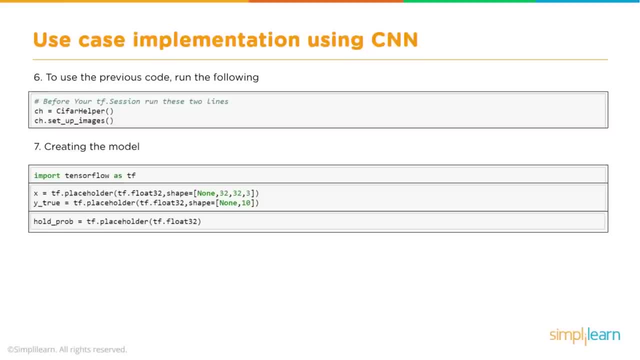 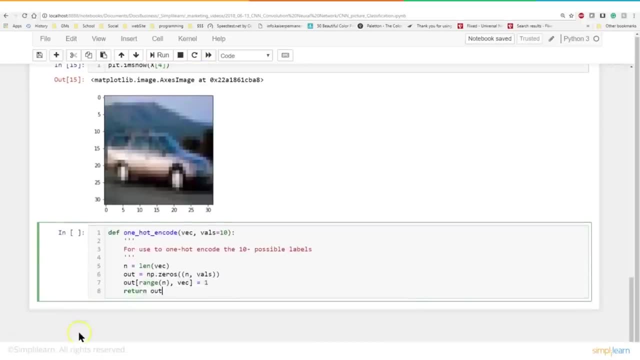 And then, finally, we'll go ahead and run that code So you can see what that looks like. And then we get into the fun part, where we're actually going to start creating our model, our actual neural network model. So let's start by creating our one hot encoder. 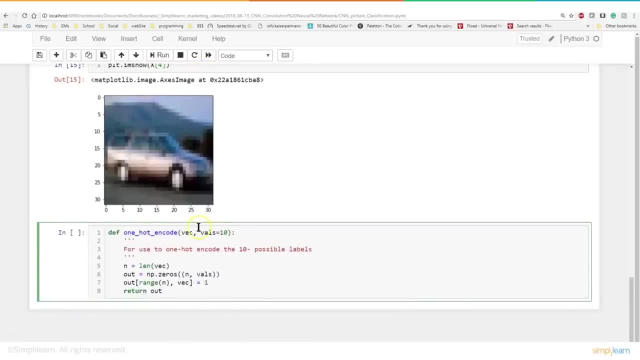 We're going to create our own here And it's going to return an out And we'll have our vector coming in and our values equal 10.. What this means is that we have the 10 values, the 10 possible labels. 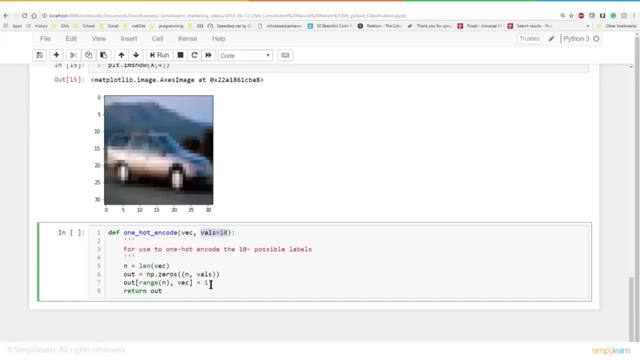 And remember we don't look at the labels as a number, because a car isn't one more than a horse. That'd be just kind of bizarre to have. horse equals zero, car equals one, plane equals two, cat equals three. So a cat plus a car equals what? 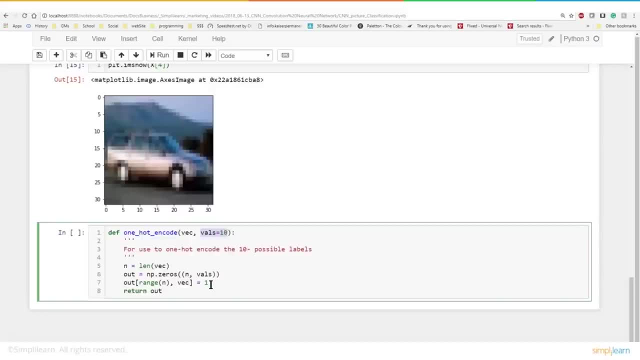 So instead we create a numpy array of zeros And there's going to be 10 values, So we have 10 different values in there. So you have zero or one. One means it's a cat, Zero means it's not a cat. 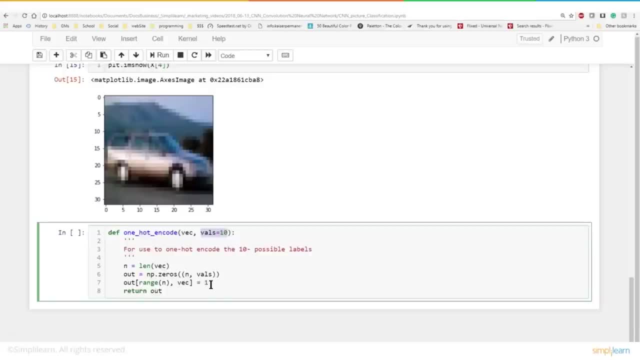 In the next line. it might be that one means it's a car, Zero means it's not a car. So instead of having one output with a value of zero to 10, you have 10 outputs with the values of zero to one. 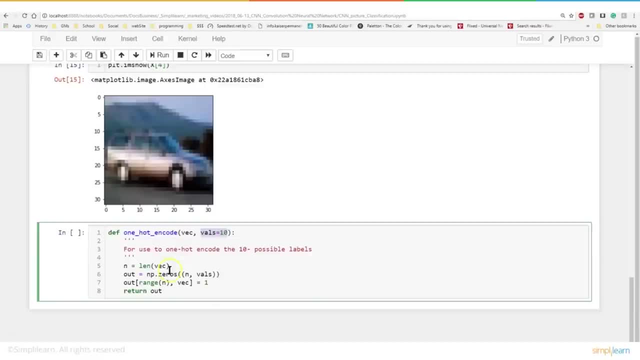 That's what the one hot encoder is doing here, And we're going to utilize this in code in just a minute. So let's go ahead and take a look at the next helpers. We have a few of these helper functions we're going to build. 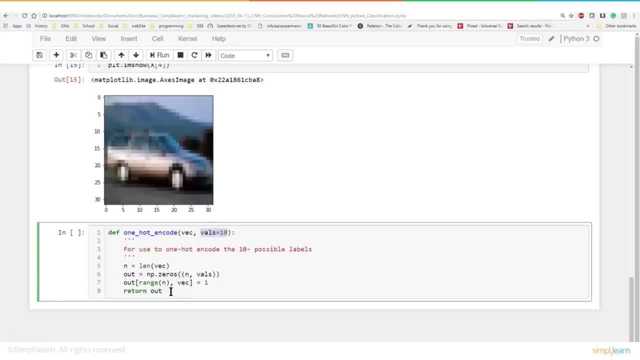 And when you're working with a very complex system, a very complicated Python project, dividing it up into separate definitions and classes is very important. Otherwise it just becomes really ungainly to work with. So let's go ahead and put in our next helper, which is a class. 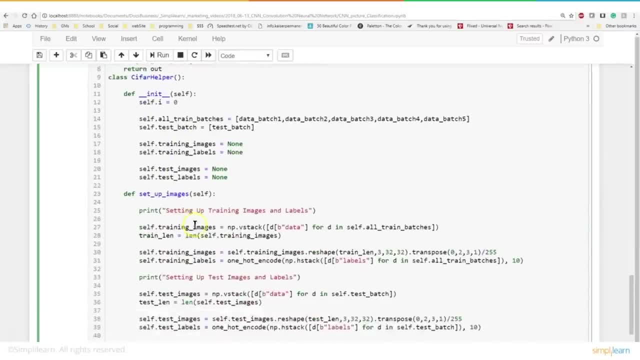 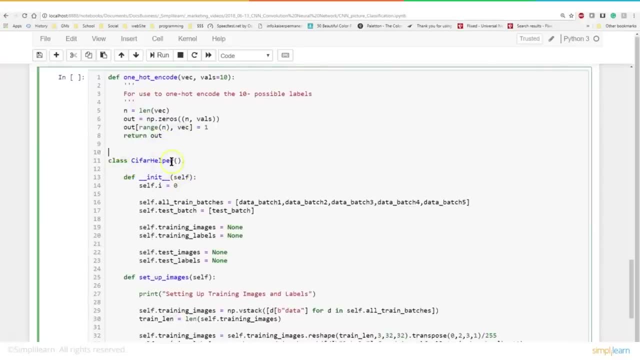 And there's a lot in this class, So we'll break it down here And let's just start to put a space right in there. There we go. Now this is a little bit more readable. Add a second space. So we're going to create our class, the Cypher Helper. 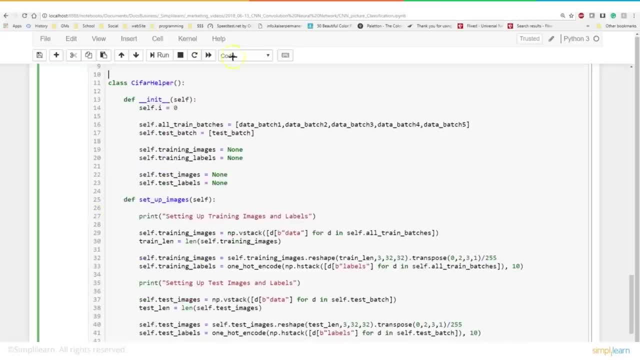 And we'll start by initializing it Now. there's a lot going on in here, So let's start with the init part. selfi equals 0.. That will come in in a little bit. We'll come back to that in the lower part. 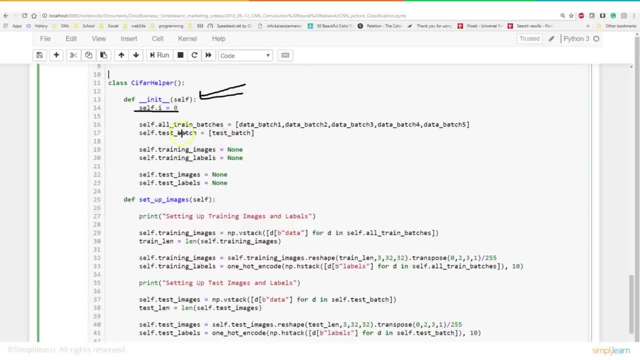 We want to initialize our training batches. So when we went through this, there was like a meta batch. We don't need the meta batch, But we do need the data batch 1,, 2,, 3,, 4, 5.. 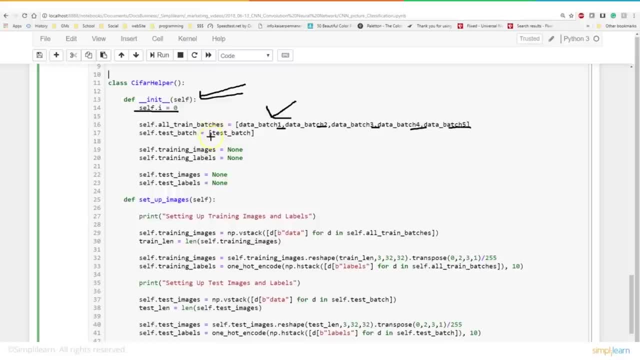 And we do not want the testing batch in here. This is just the self, all trained batches. So we're going to make an array of all those different images And then, of course, we're going to test batch out. so we have our selftestbatch. 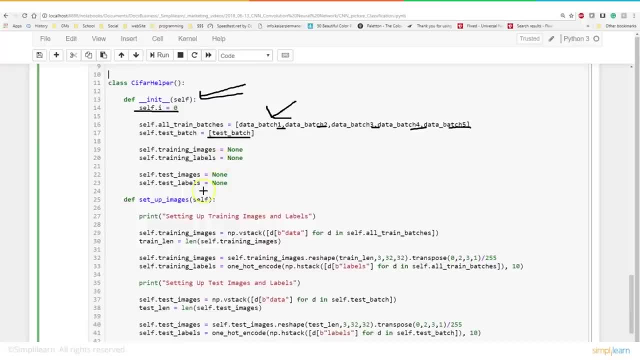 We're going to initialize the training images and the training labels And also the test images and the test labels. So this is just to initialize these variables in here. Then we create another definition down here And this is going to set up the images. 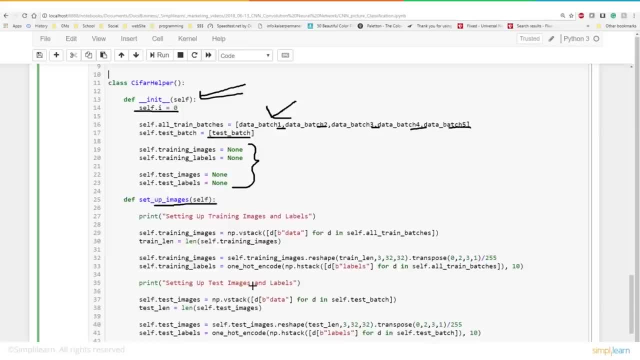 And let's just take a look and see what's going on in there. Now, we could have all just put this as part of the init part, since this is all just Helper stuff, But breaking it up again makes it easier to read. 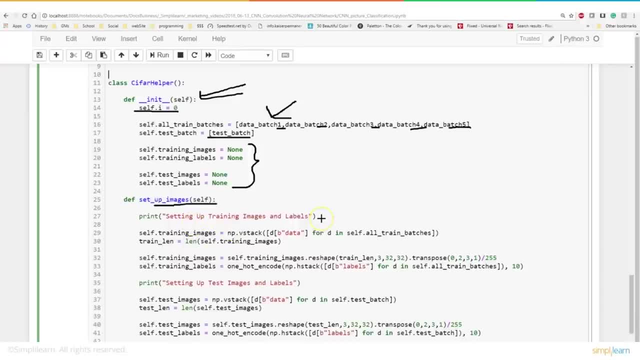 It also makes it easier, when we start executing the different pieces, to see what's going on. So that way we have a nice print statement to say: hey, we're now running this and this is what's going on in here. We're going to set up these self training images at this point. 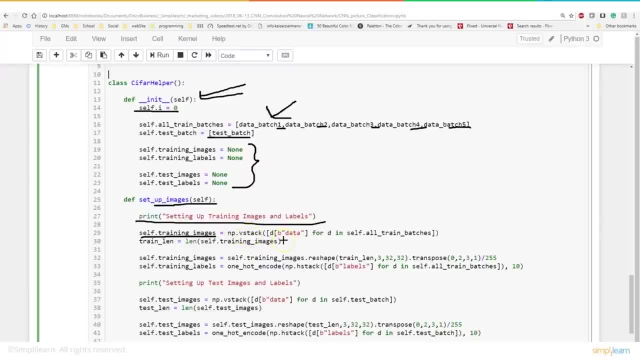 And that's going to go to a numpy array, vstack, And in there we're going to load up, in this case the data for D and self, all trained batches. Again, that points right up to here. So we're going to go through each one of these files, or each one of these data sets, because they're not a file anymore. 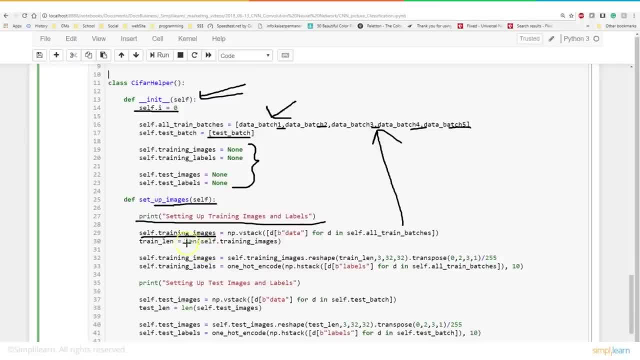 They're not a min Data batch. one points to the actual data And so our self training images is going to stack them all into a numpy array, And then it's always nice to get the training length And that's just a total number of self training images in there. 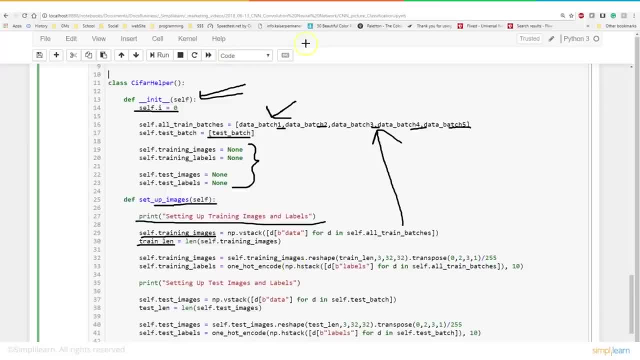 And then we're going to take the self training images And let me switch marker colors, because I am getting a little too much on the markers up here. Oops, there we go. Bring down our marker change so we can see it a little better. 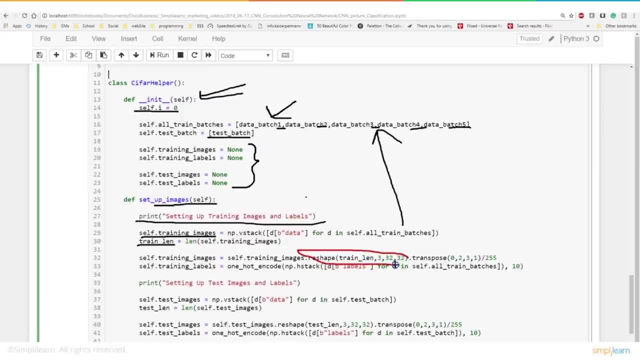 And at this point this should look familiar. Where did we see this? Well, when we wanted to look at this above and we wanted to look at the images in the Matplot library, we had to reshape it. So we're doing the same thing here. 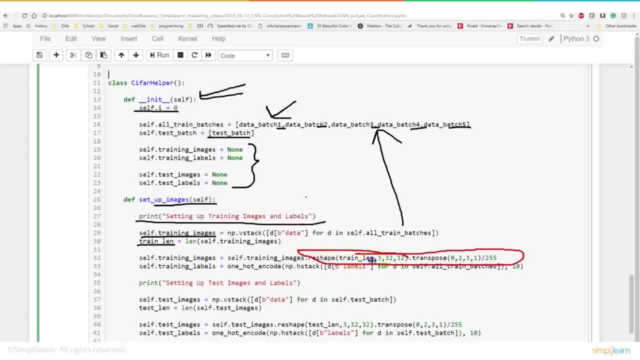 We're taking our self training images and, based on the training length, total number of images because we stacked them all together. So now it's just one large file of images We're going to take and look at it as our three video cameras that are each displaying 32 by 32.. 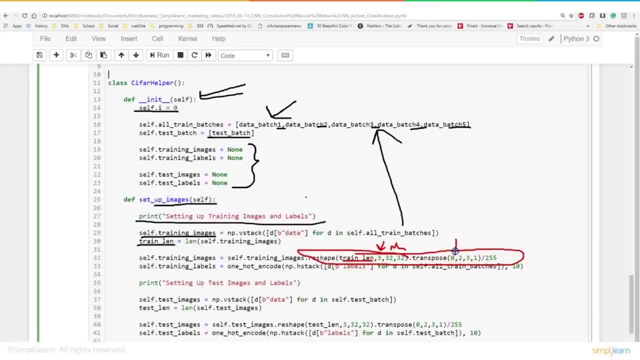 We're going to switch that around So that now we have Each of our images that stays the same place, and then we have our 32 by 32 and then by our three, our last, our three different values for the color. And of course we want to go ahead and they run this where you say: divide by 255.. 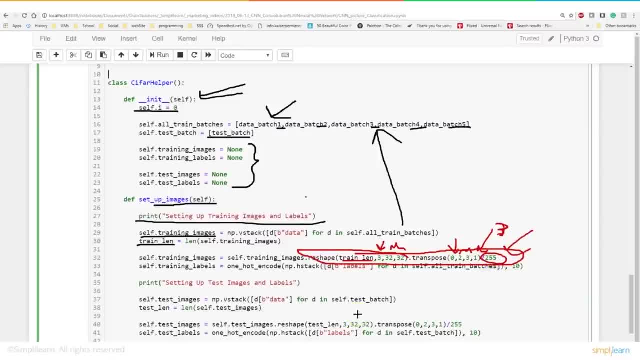 That was from earlier. It just brings all the data into zero to one. That's what this is doing. So we're turning this into a zero to one array, which is all the pictures, 32 by 32, by three, And then we're going to take the self training labels and we're going to pump those through our one hot encoder we just made and we're going to stack them together. 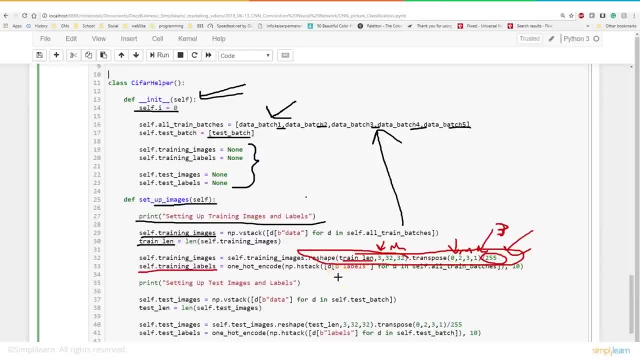 And again, we're converting this into an array that goes from: instead of having: horse equals one, dog equals two, and then horse plus dog would equal three, which would be cat. Now it's going to be, you know, an array of ten, where each one is zero to one. 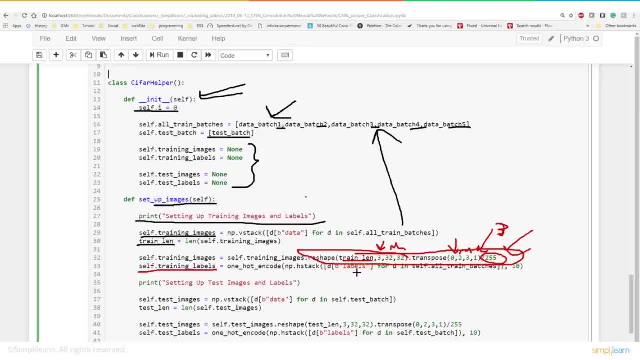 Then we want to go ahead and set up our test images and labels, And when we're doing this, You're going to see it's the same thing we just did with the rest of them. We just change colors right here. This is no different than what we were doing up here with our training set. 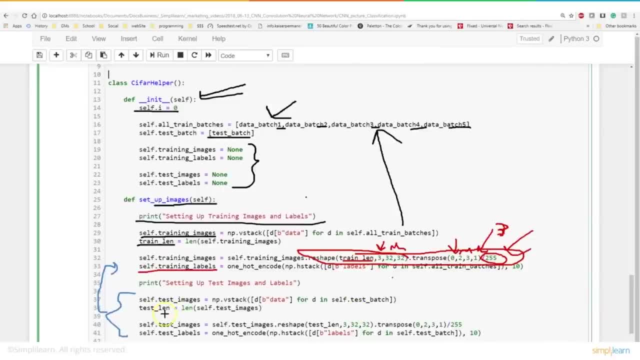 We're going to stack the different images. We're going to get the length of them So we know how many images are in there. You certainly could add them by hand, but it's nice to let the computer do it, especially if it ever changes on the other end and you're using other data. 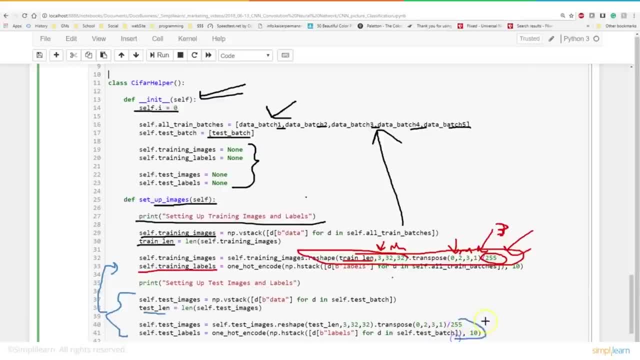 And again we reshape them and transpose them, And we also do the one hot encoder- Same thing we just did on our training images. So now our test images, Now our test images, are in the same format. So now we have a definition which sets up all our images in there. 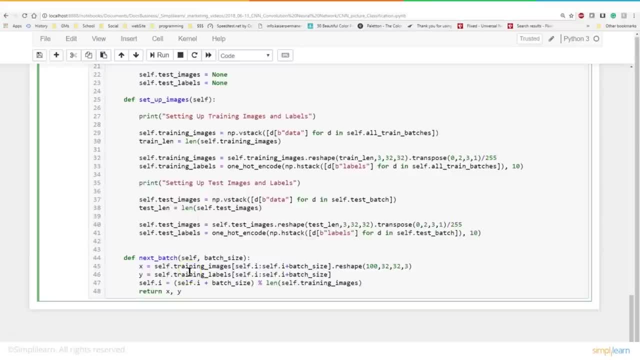 And then the next step is to go ahead and batch them, or next batch- And let's do another breakout here for batches, because this is really important to understand- Tends to throw me for a little loop when I'm working with TensorFlow or Keras or a lot of these. 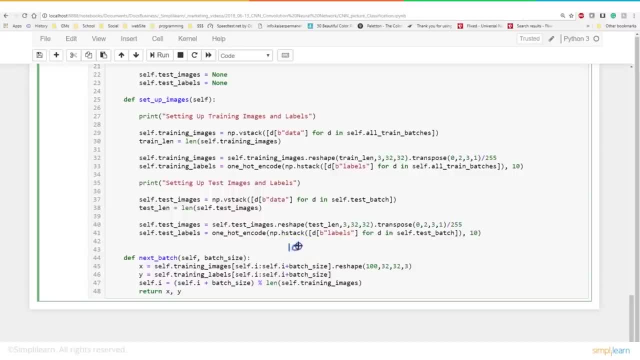 We have our data coming in. If you remember, we had like 10,000 photos. Let me just put 10,000 down here. We don't want to run all 10,000 at once, So we want to break this up into batch sizes. 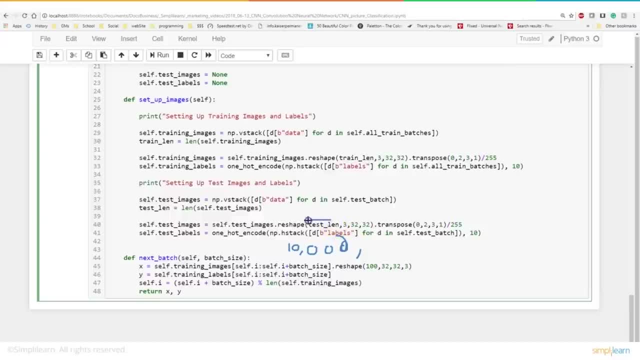 And you also remember that we had the number of photos. in this case, length of test or whatever number is in there. We also have 32 by 32 by 3.. So when we're looking at the batch size, we want to change this from 10,000 to a batch of. in this case, I think we're going to do batches of 100. 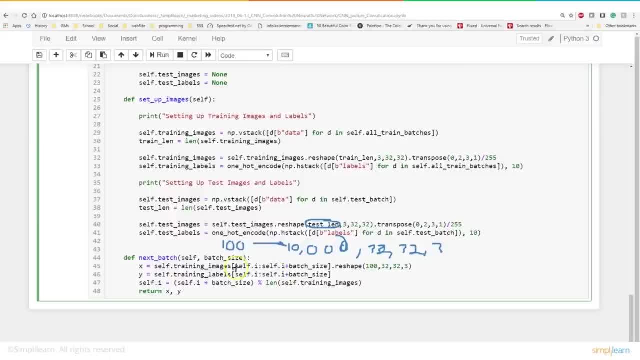 So we want to look at just 100, the first 100 of the photos, And, if you remember, we set selfi equal to 0.. So what we're looking at here is we're going to create X, We're going to get the next batch from the very initialized. 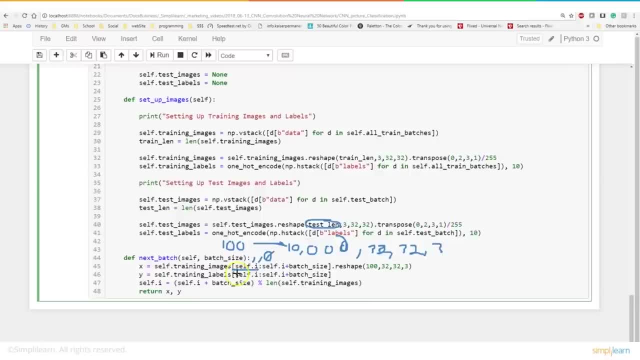 We've already initialized it for 0.. So we're going to look at X from 0 to batch size, which we set to 100. So just the first 100 images And then we're going to reshape that into- and this is important to let the data know- that we're looking at 100 by 32 by 32 by 3.. 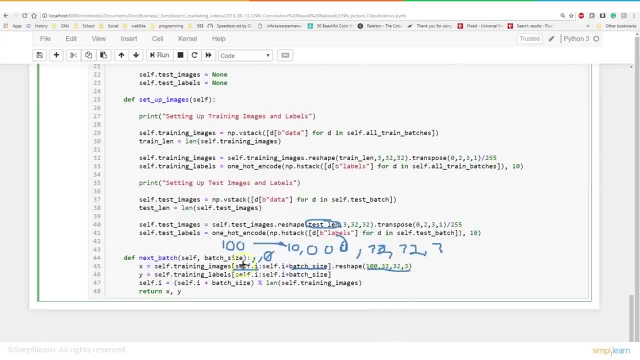 Now we've already formatted it to the 32 by 32.. This just sets everything up correctly, so that X has the data in there in the correct order and the correct shape, And then the Y, just like the X, is our labels. 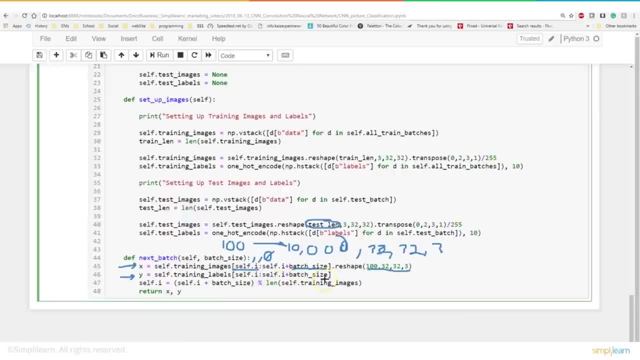 So our training labels. again, they go from 0 to batch size. In this case they do selfi plus batch size because the selfi is going to keep changing. And then finally we increment the selfi because we have 0.. 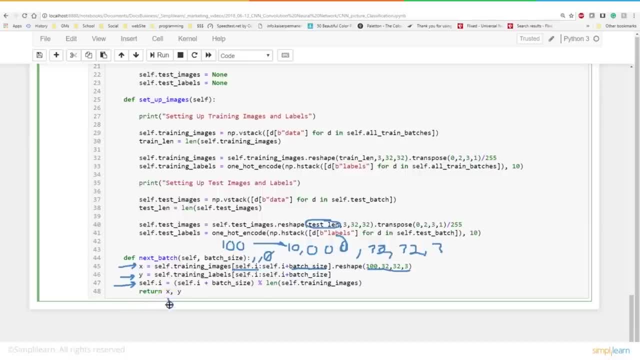 So the next time we call it, we're going to get the next batch size, And so basically, we have X and Y, X being the photo image, Y being the photograph data coming in And Y being the label, And that, of course, is labeled through one hot encoder. 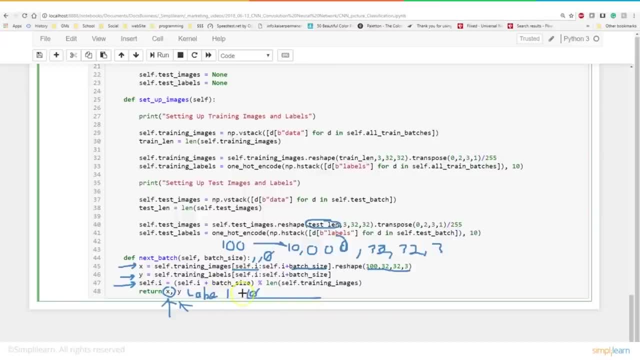 So, if you remember correctly, if it was, say, horse is equal to 0, it would be 1 for the 0 position, since this is the horse, And then everything else would be 0 in here. Let me just put lines through there. 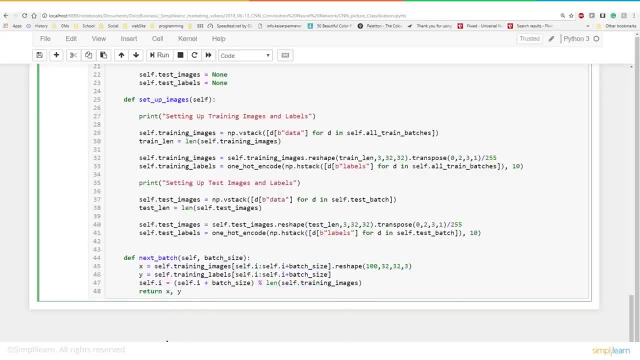 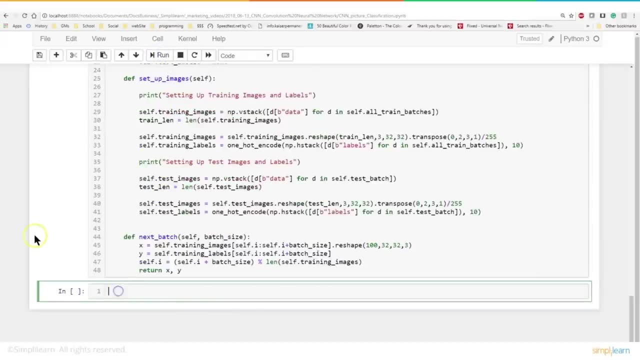 There we go. There's our array. Hard to see that array, So let's go ahead and take that And we're going to finish loading it, since this is our class. So, with all this, our setup over here, let's go ahead and load that up. 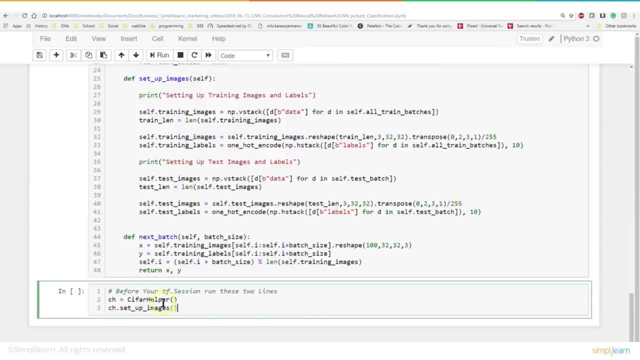 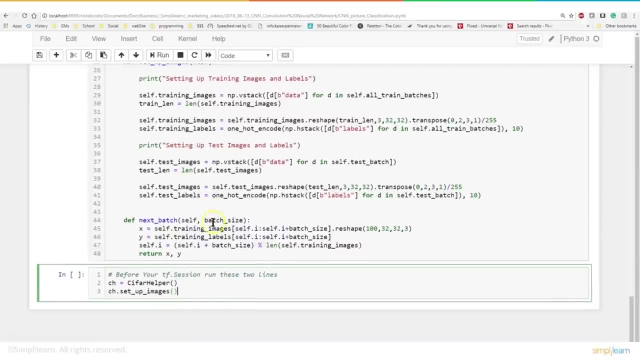 And so we're going to create a variable ch with the cfar helper in it, And then we're going to do chsetupimages. Now we could have just put all of the setup images under the init, But by breaking this up into two parts it makes it much more readable. 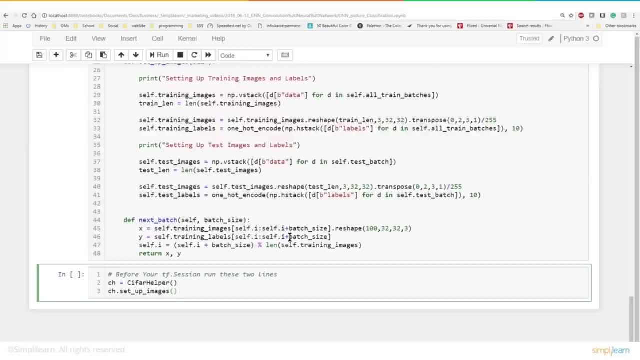 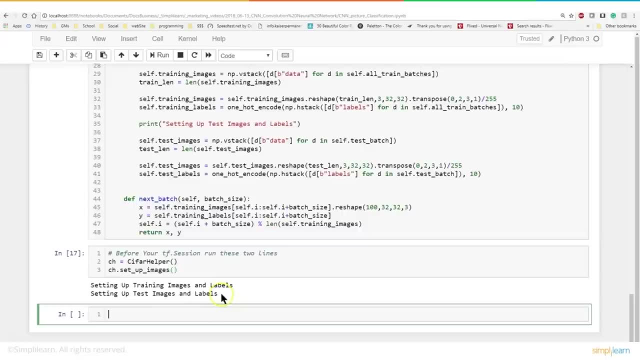 And also if you're doing other work, there's reasons to do that. as far as the setup, Let's go ahead and run that And you can see where it says setting up training images and labels, setting up test images. And that's one of the reasons we broke it up is so that if you're testing this out, 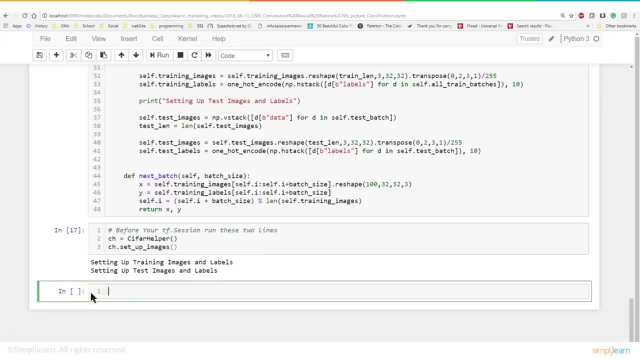 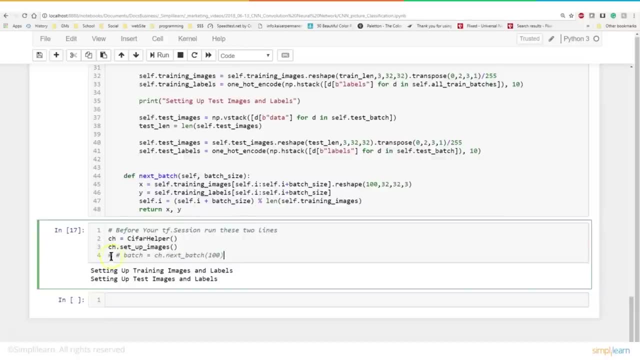 you can actually have print statements in there telling you what's going on, which is really nice. They did a good job with this setup. I like the way that it was broken up in the back. And then one quick note: you want to remember that batch to set up the next batch. 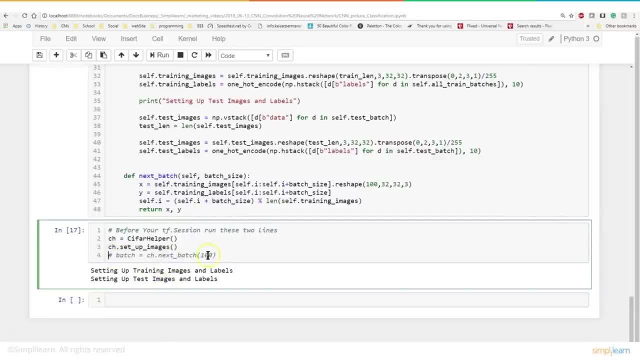 we have to run batch equals ch, next batch of 100, because we're going to use the 100 size. But we'll come back to that. We're going to use that. Just remember that. that's part of our code we're going to be using in a minute from the definition we just made. 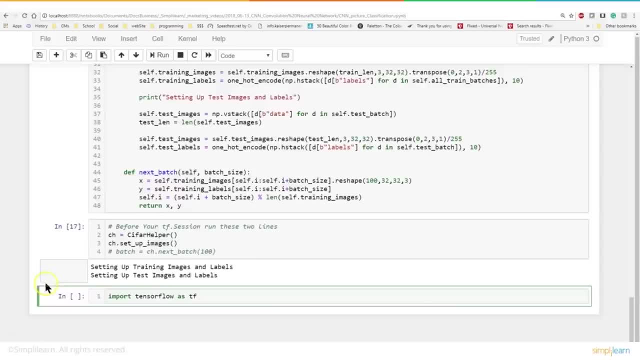 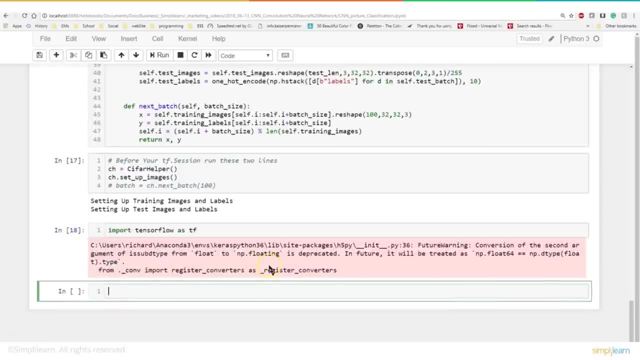 So now we're ready. We're ready to create our model. First thing we want to do is we want to import our tensorflow as tf. I'll just go ahead and run that so it's loaded up And you can see we've got a warning here. 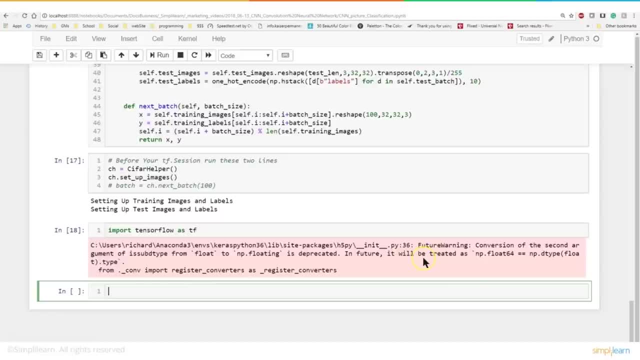 That's because they're making some changes. It's always growing And they're going to be depreciating one of the values from float64 to float type, or it's treated as an NP float64.. Nothing to really worry about because this doesn't even affect what we're working on. 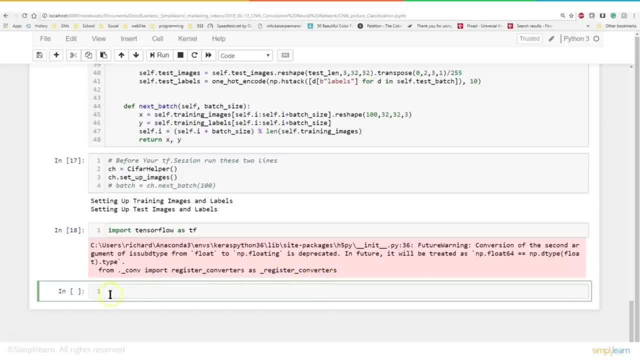 because we've set all of our stuff to a 255 value or 0 to 1.. And do keep in mind that 0 to 1, 0 to 1 value that we converted to 255 is still a float value. But it'll easily work with either the numpy float64 or the numpy dtype float. 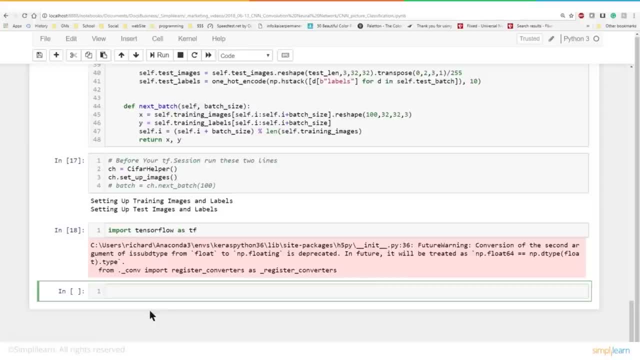 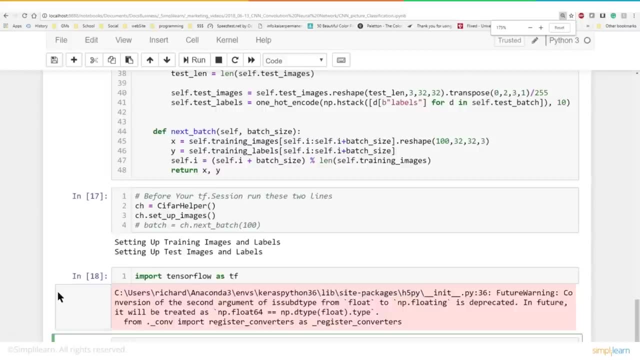 It doesn't matter which one it goes through. So the depreciation would not affect our code. as we have it And in our tensorflow we'll go ahead. Let me just increase the size in there just a moment so you can get a better view of what we're typing in. 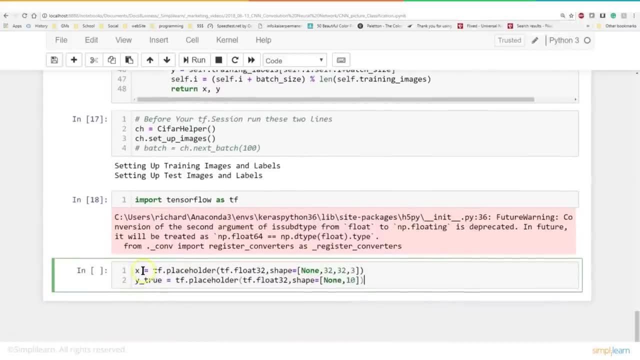 We're going to set a couple placeholders here, And so we have. we're going to set x equals tf, placeholder tf: float32.. We just talked about the float64 versus the numpy float. We're actually just going to keep this at float32.. 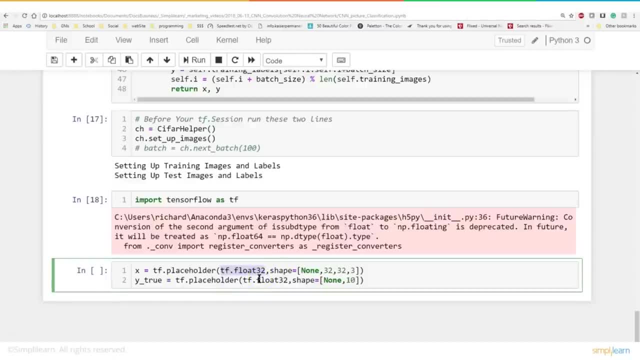 More than a significant number of decimals for what we're working with And since it's a placeholder, we're going to set the shape equal to and we've set it equal to none, because at this point we're just holding the place on there. 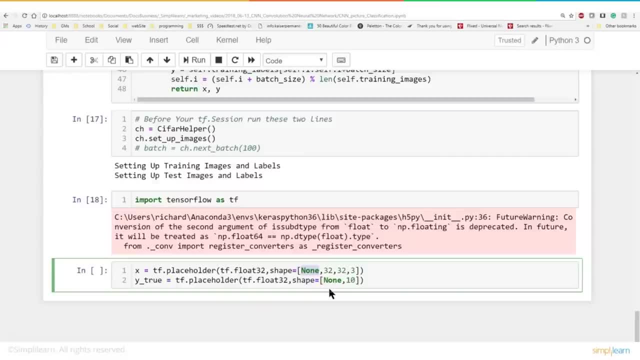 We'll be setting up as we run the batches. That's what that first value is, And then 32 by 32 by 3.. That's what we reshaped our data to fit in, And then we have our y, true, equal to 0.. 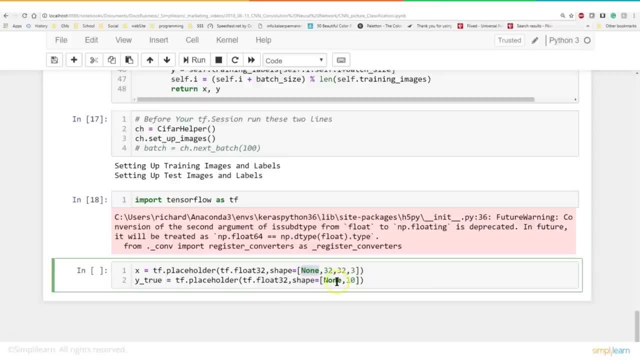 And then we have our tf float32.. And the shape equals none comma 10.. 10 is the 10 different labels we have, So it's an array of 10.. And then let's create one more placeholder. We'll call this hold prob or hold probability. 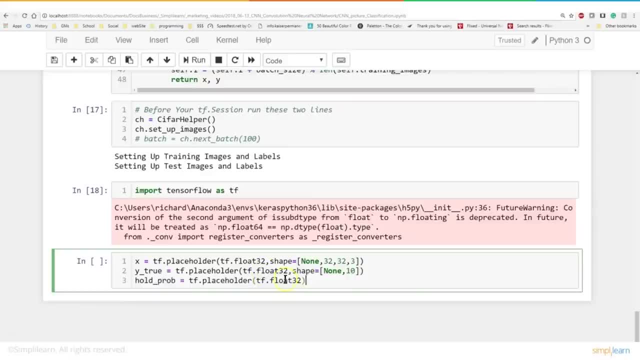 And we're going to use this. We don't have to have a shape or anything for this. This placeholder is for what we call dropout. If you remember from our theory, before we drop out so many nodes it's looking at or the different values going through. 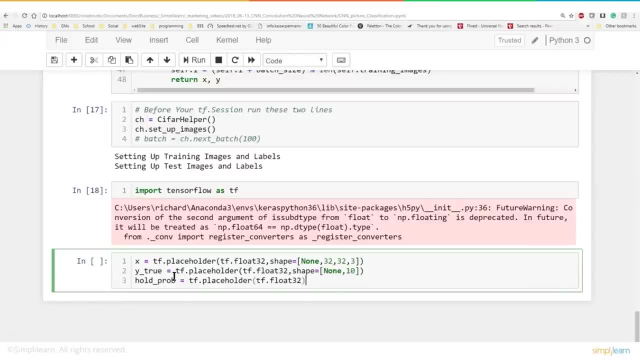 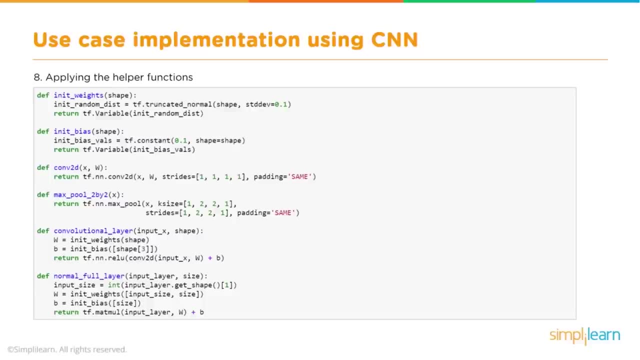 which helps decrease bias. So we need to go ahead and put a placeholder for that also, And we'll run this, so it's all loaded up in there. So we have our three different placeholders. And since we're in TensorFlow, when you use Keras it does some of this automatically. 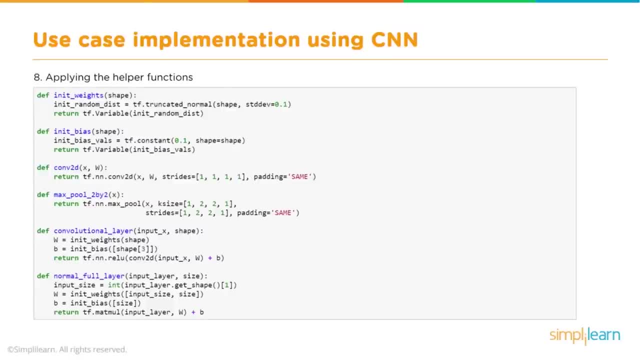 But we're in TensorFlow. direct Keras sits on TensorFlow. We're going to go ahead and create some more helper functions. We're going to create something to help us initialize the weights, initialize our bias, If you remember that each layer has to have a bias going in. 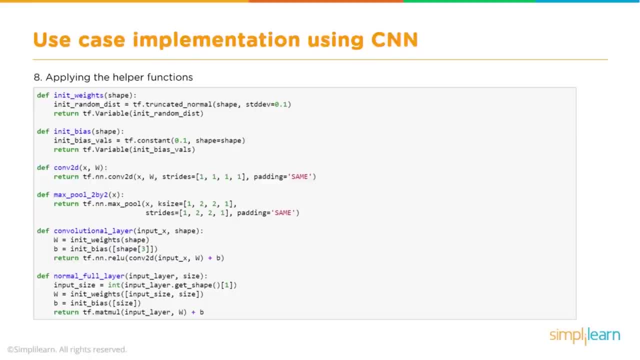 We're going to go ahead and work on our conversional 2D, our max pool, So we have our pooling layer, our convolutional layer and then our normal full layer. So we're going to go ahead and put those all into definitions. 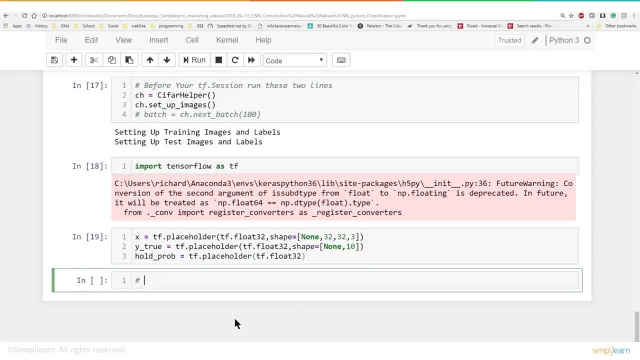 And let's see what that looks like in code. And you can also grab some of these helper functions from the MNIST, the NIST setup. We just put that in there if you're under the TensorFlow, So a lot of these are already in there. 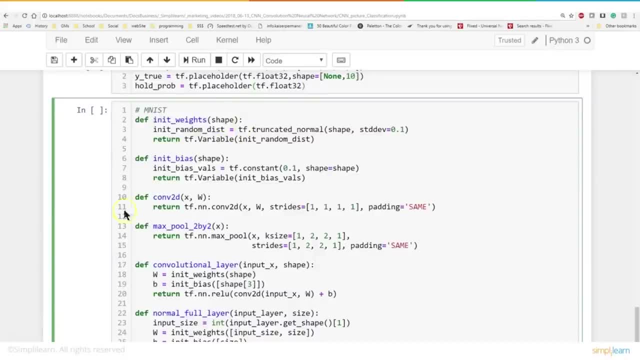 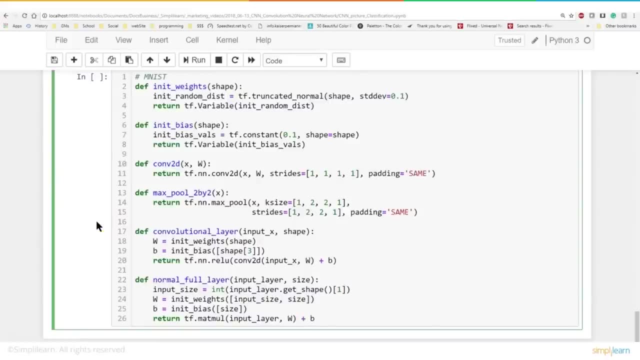 but we're going to go ahead and do our own And we're going to create our init weights, And one of the reasons we're doing this is so that you can actually start thinking about what's going on in the backend. So, even though there's ways to do this online, 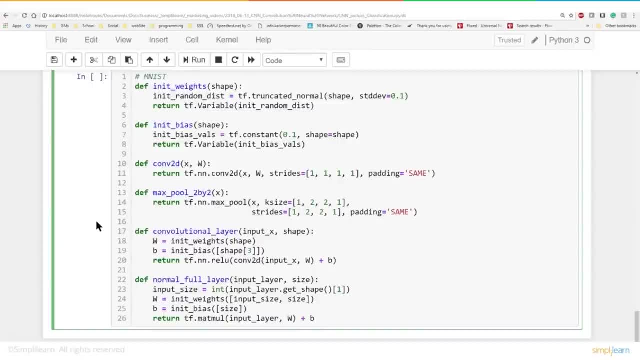 with an automation. sometimes these have to be tweaked and you have to put in your own setup in here. Now we're not going to be doing that, We're just going to recreate them for our code. And let's take a look at this. 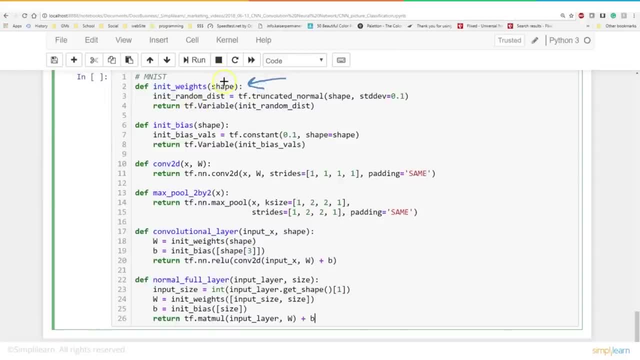 We have our weights, And so what comes in is going to be the shape And what comes out is going to be random numbers. So we're going to go ahead and just init some random numbers based on the shape, with a standard deviation of 0.1. 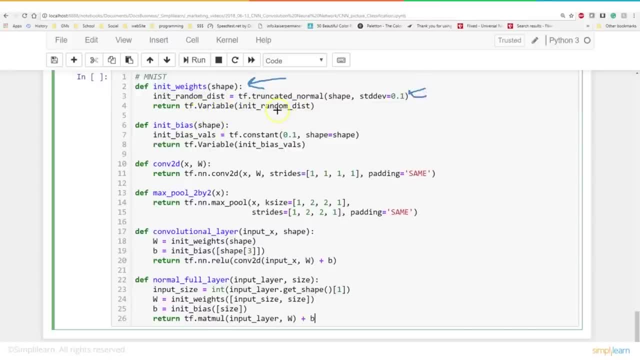 Kind of a fun way to do that. And then the tf variable, init random distribution. So we're just creating a random distribution on it. That's all that is for the weights. Now you might change that. You might have a higher standard deviation. 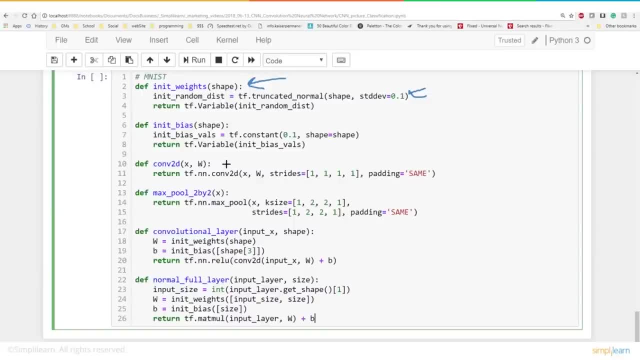 In some cases you actually load preset weights. That's pretty rare. Usually you're testing that against another model or something like that, and you want to see how those weights configure with each other. Now, remember we have our bias, So we need to go ahead and initialize the bias with a constant. 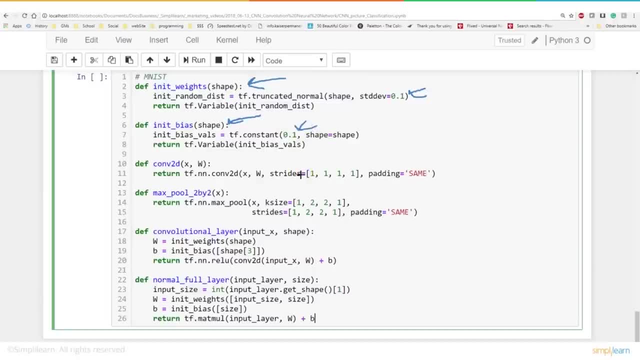 In this case, we're using 0.1.. A lot of times the bias is just put in as 1 and then you have your weights add on to that, But we're going to set this as 0.1.. So we're going to set this as 0.1.. 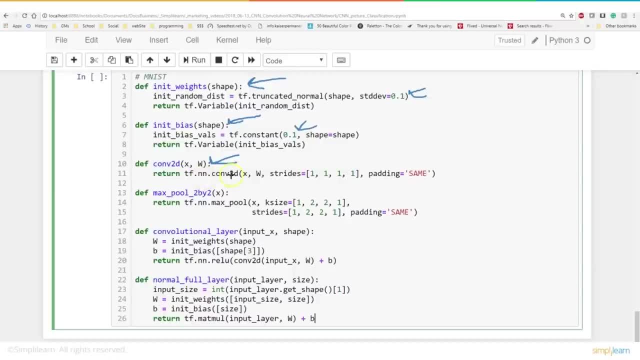 So we want to return a convolutional 2D, in this case a neural network. This would be a layer on here. What's going on with the 2D is? we're taking our data coming in. We're going to filter it. 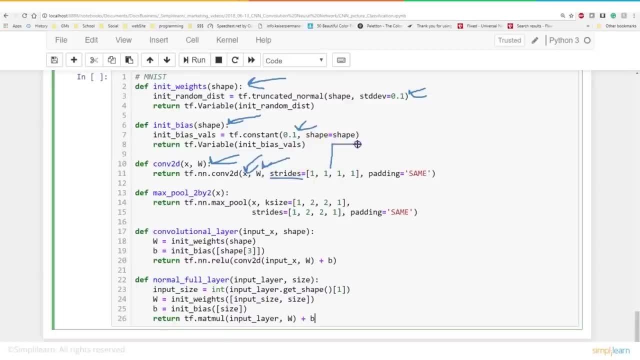 Strides. if you remember correctly, strides came from. here's our image, and then we only look at this picture here And then maybe we have a stride of 1.. So we look at this picture here, We continue to look at the different filters, going on there. 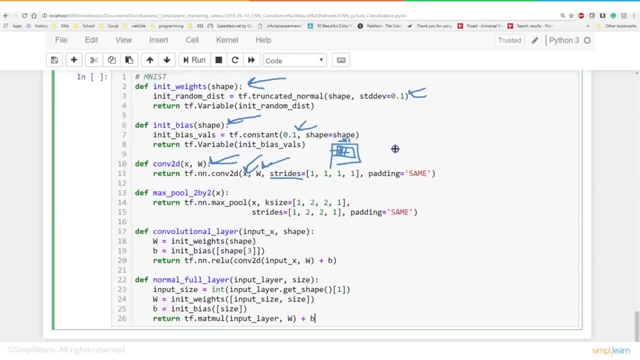 The other thing this does is that we have our data coming in as 32 by 32 by 3.. And we want to change this so that it's just: this is three dimensions and it's going to reformat this as just two dimensions. 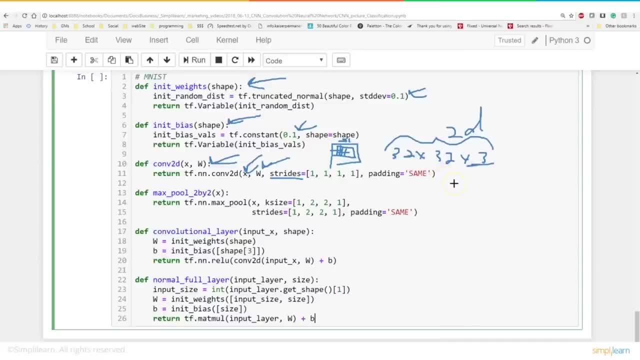 So it's going to take this number here and combine it with the 32 by 32.. So this is a very important layer here because it's reducing our data down using different means And it connects down. I'm just going to jump down one here. 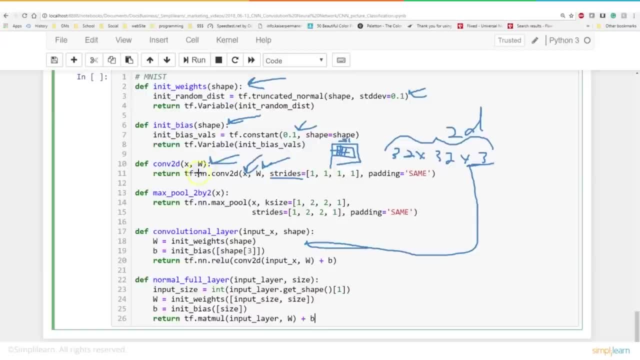 It goes with the convolutional layer. So you have your kind of your pre-formatting and the setup and then you have your actual convolution layer. that goes through on there And you can see here we have init weights by the shape: init bias, shape of three. 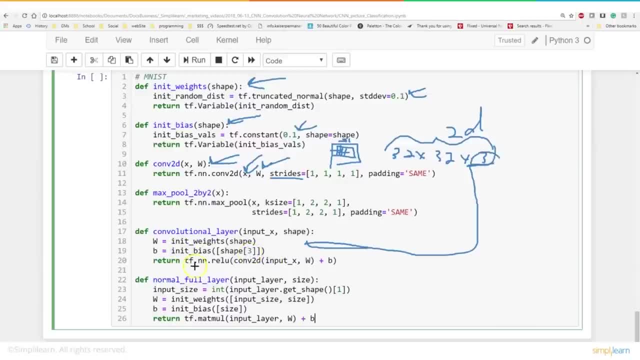 because we have the three different. here's our three again. And then we return the TFNN relu with the convention 2D. So this convolutional has this feeding into it right there. It's using that as part of it. 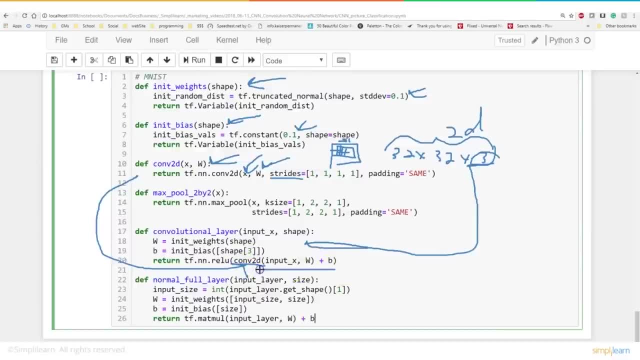 And of course the input is the xy plus b, the bias. So that's quite a mouthful, but these two are the keys here to creating the convolutional layers there: The convolutional 2D coming in and then the convolutional layer. 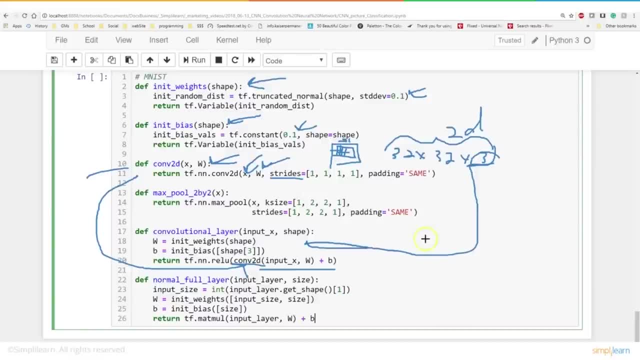 which then steps through and creates all those filters we saw. Then, of course, we have our pooling. So after each time we run it through the convectional layer, we want to pool the data, If you remember correctly, on the pool side. and let me just get rid of all my marks. 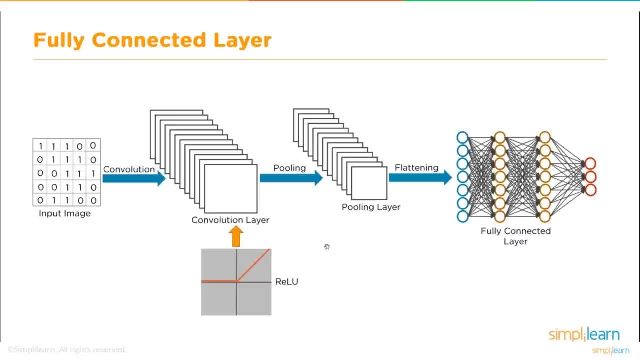 it's getting a little crazy there And in fact let's go ahead and jump back to that slide. Let's just take a look at that slide over here. So we have our image coming in and then we create our convolutional layer. 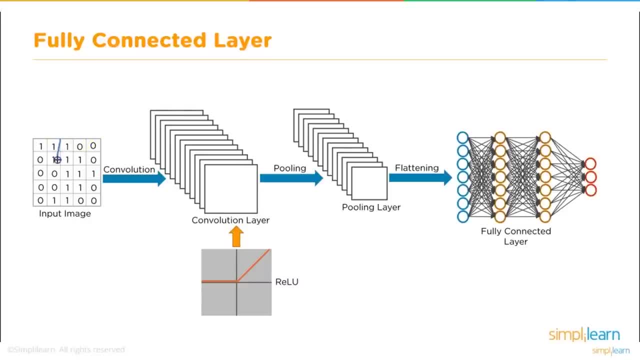 with all the filters. Remember, the filters go, you know the filters coming in here and it looks at these four boxes and then if it's a step, let's say step two- it then goes to these four boxes and then the next step. 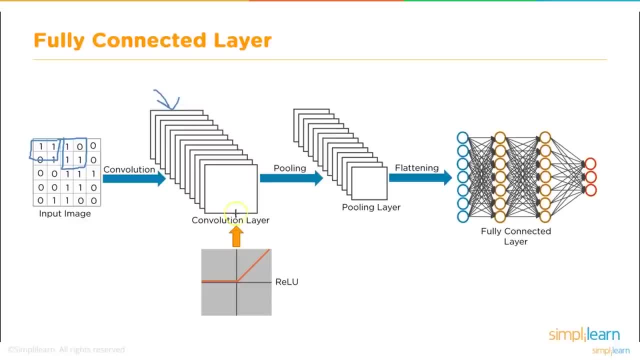 and so on. So we have our convolutional layer that we generate, or convolutional layers. They use the relu function. There's other functions out there For this, though the relu is the most, the one that works the best, at least so far. 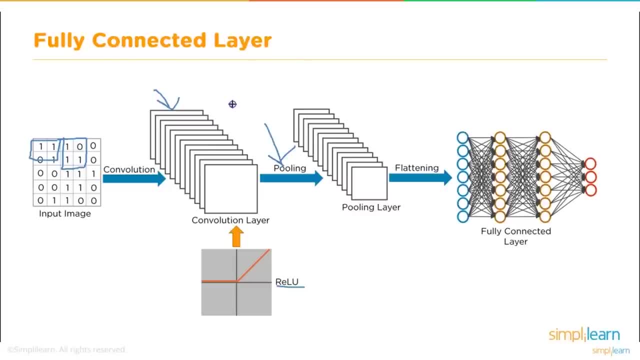 I'm sure that will change. Then we have our pooling. Now, if you remember correctly, the pooling was max. So if we had the filter coming in and they did the multiplication on there and we have a one and maybe a two here. 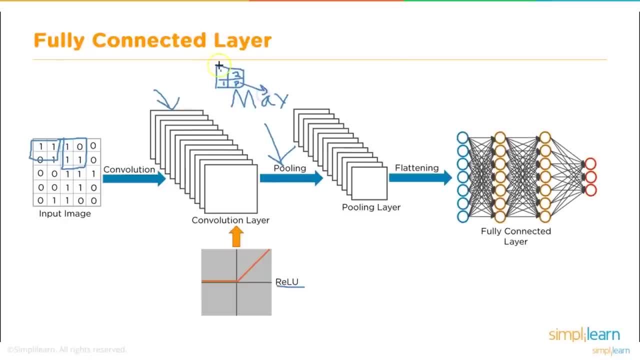 and another one here and a three here. three is the max, And so out of all of these you then create an array that would be three, and if the max is over here, two or whatever it is. That's what goes into the pooling. 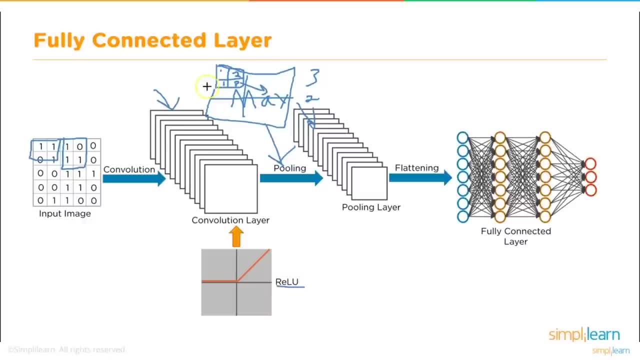 and what's going on in our pooling. So again, we're reducing that data down, We're reducing it down as small as we can and then, finally, we're going to flatten it out into a single array and that goes into our fully connected layer. 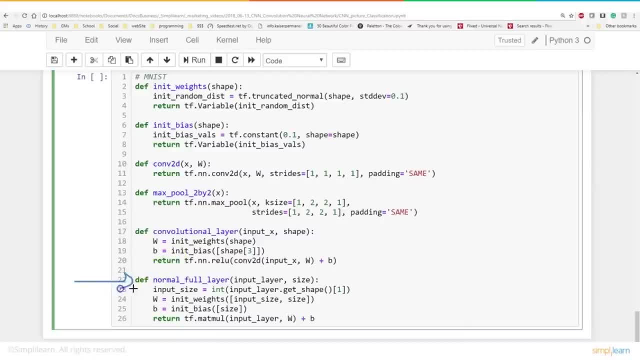 And you can see that here in the code Right here we're going to create our normal full layer. So at some point we're going to take from our pooling layer. this will go into some kind of flattening process and then that will be fed into the full. 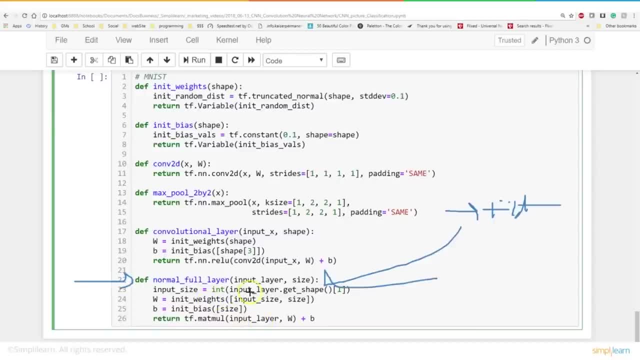 the different layers going in down here, And so we have our input size. You'll see our input layer get shape, which is just going to get the shape for whatever's coming in, And then input size- initial weights- is also based on the input layer coming in. 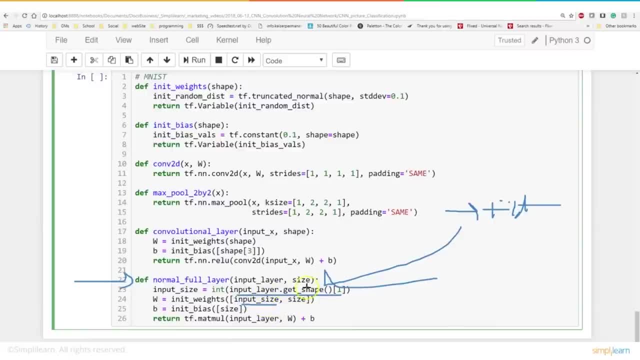 And the input size down here is based on the input layer shape. So we're just going to already use the shape and already have our size coming in. And of course you have to make sure you init the bias. Always put your bias on there. 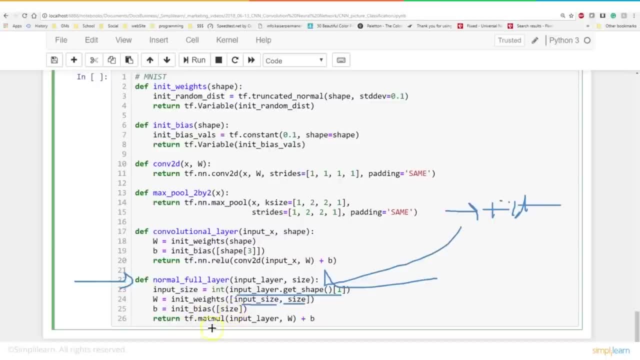 and we'll do that based on the size. So this will return tfmatmul input layer W plus B. This is just a normal full layer. That's what this means right down here. That's what we're going to return. So that was a lot of steps we went through. 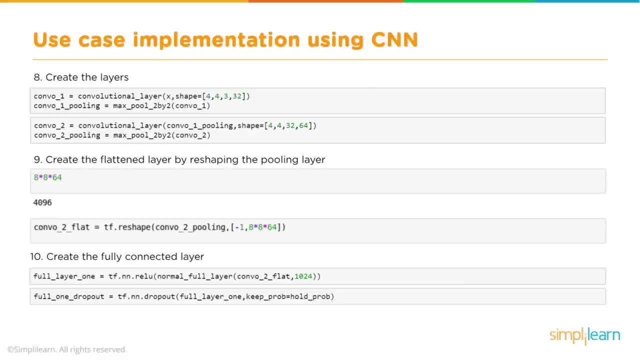 Let's go ahead and run that, So those are all loaded in there, And let's go ahead and create the layers. Let's see what that looks like. Now that we've done all the heavy lifting and everything, we get to do all the easy part. 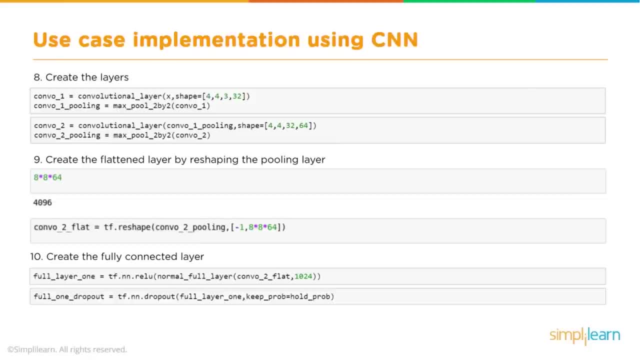 Let's go ahead and create our layers. We'll create a convolution layer one and two, two different convolutional layers, And then we'll take that and we'll flatten that out, create a reshape, pooling in there for our reshape, And then we'll have our full layer. 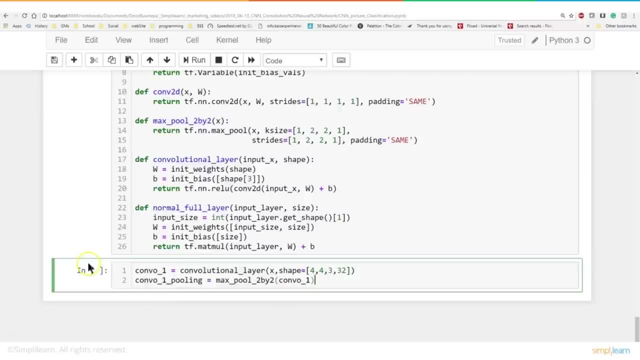 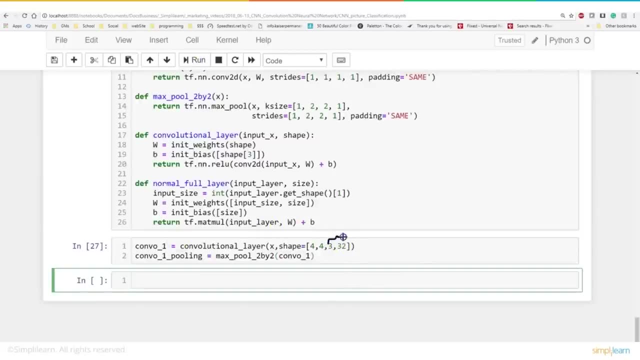 at the end. So let's start by creating our first convolutional layer. Then we come in here and let me just run that real quick And I want you to notice on here the three and the 32.. This is important because coming into this convolutional layer, 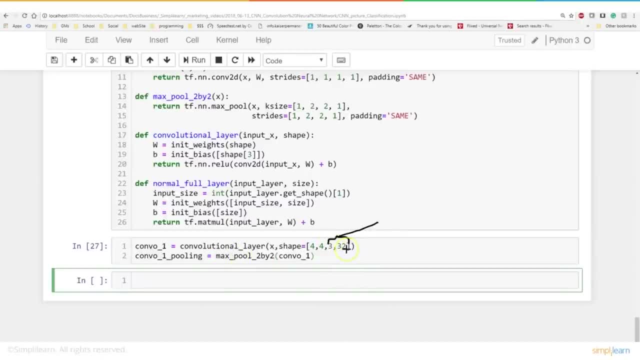 we have three different channels and 32 pixels each, So that has to be in there, The four and four you can play with. This is your filter size. So, if you remember, you have a filter and you have your image and the filter. 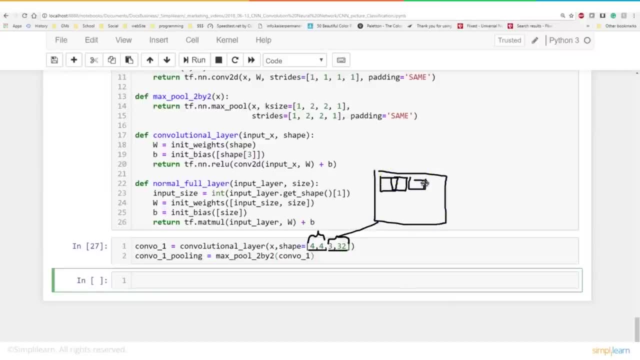 And the filter slowly steps over and filters out this image, depending on what your step is For this particular setup, four, four is just fine. That should work pretty good for what we're doing and for the size of the image. And then, of course, at the end. 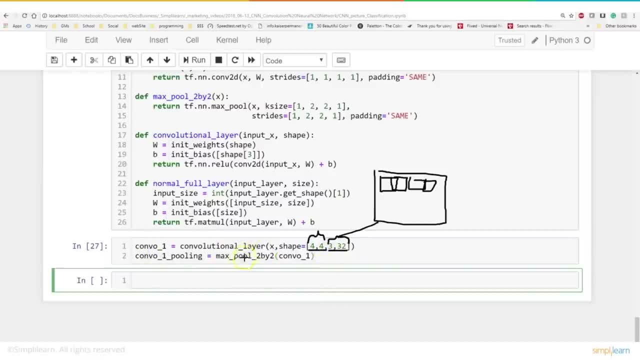 once you have your convolutional layer set up, you also need to pool it And you'll see that the pooling is automatically set up so that it would see the different shape based on what's coming in. So here we have max two by two. 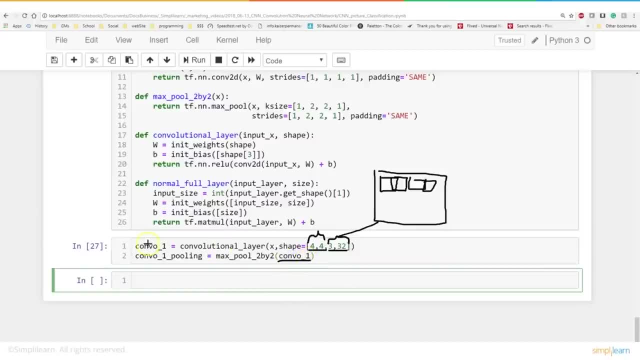 and we put in the convolutional one that we just created. the convolutional layer we just created goes right back into it And that right up here, as you can see, is the x It's coming in from here. So notice to look at the first model and set the data accordingly. 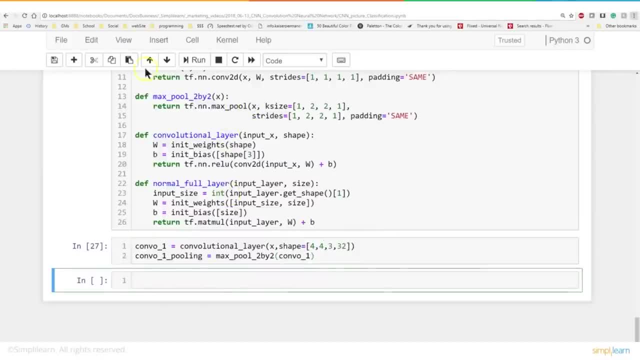 Set that up so it matches, And we went ahead and ran this already. I think I ran it. Let me go ahead and run it again. And if we're going to do one layer, let's go ahead and do a second layer down here. 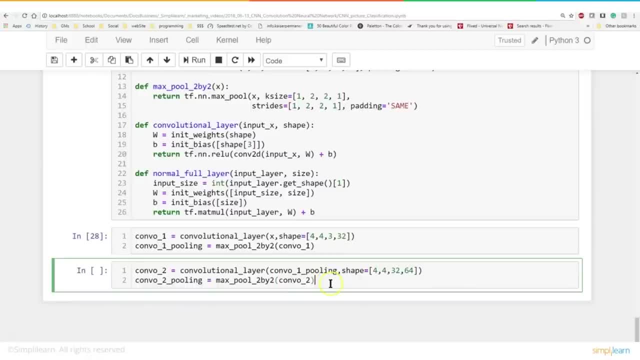 And we'll call it convo two. It's also a convolutional layer on this And you'll see that we're feeding convolutional one in the pooling. So it goes from convolutional one into convolutional one pooling, from convolutional one pooling into convolutional two. 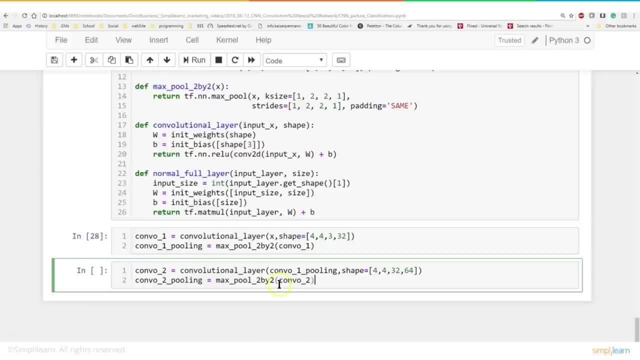 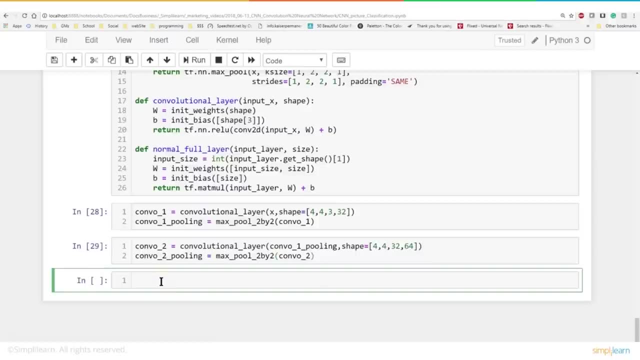 and then from convolutional two into convolutional two, pooling, And we'll go ahead and take this and run this, so these variables are all loaded into memory. And for our flattened layer, let's go ahead, and we'll do, since we have 64 coming out of here. 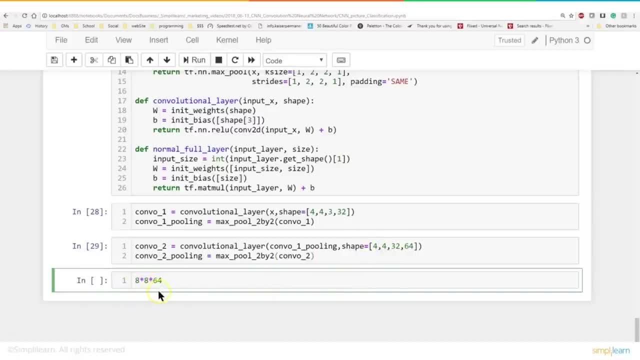 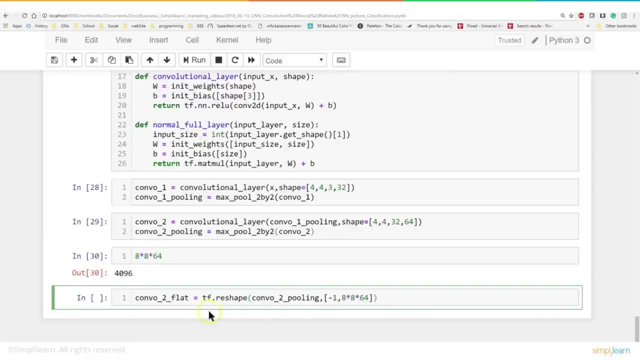 and we have four by four going in. let's do eight by eight by 64.. So let's do that. Let's do 4096.. This is going to be the flat layer. So that's how many bits are coming through on the flat layer. 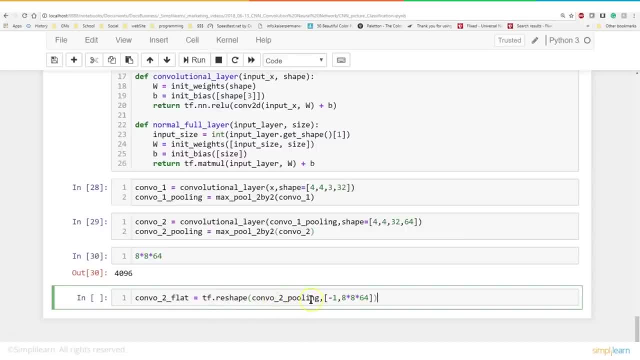 And we'll reshape this. So we'll reshape our convo two pooling and that will feed into here the convo two pooling, And then we're going to set it up as a single layer that's 4096 in size. That's what that means there. 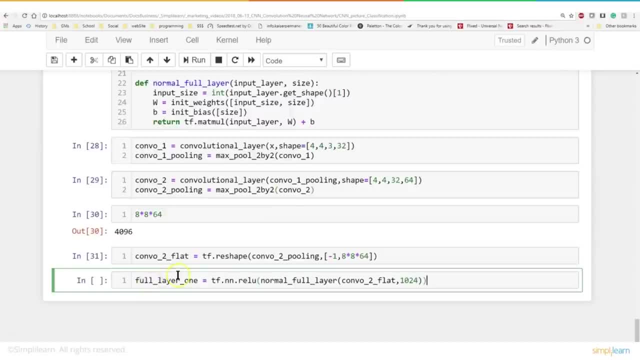 We'll go ahead and run this. So we've now created this variable, the convo, two flat, And then we have our first full layer. This is the final neural network where we have the flat layer going in And we're going to again use the ReLU. 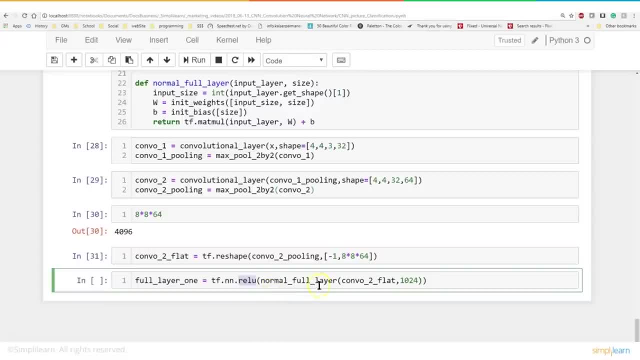 for our setup on there in a neural network for evaluation, And you'll notice that we're going to create our first full layer, Our normal full layer. that's our definition. So we created that. That's creating the normal full layer, And our input for the data comes right here from the 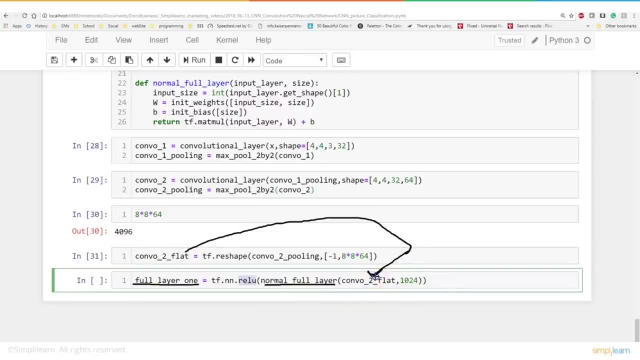 this goes right into it: the convo two flat. So this tells it how big the data is And we're going to have it come out. It's going to have 1024.. That's how big the layer is coming out. We'll go ahead and run this. 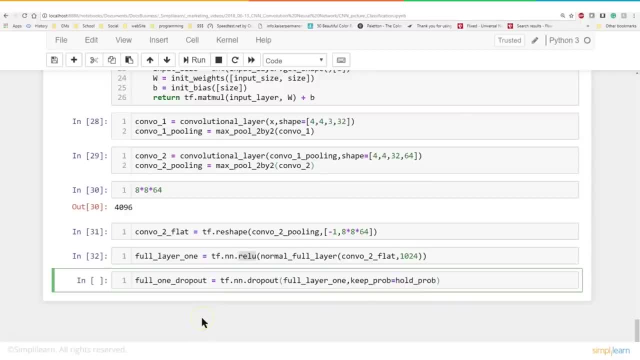 So now we have our full layer one And with the full layer one we want to also define the full one dropout to go with that. So our full layer one comes in. Keep probability equals, hold probability- Remember we created that earlier- And the full layer one is what's coming into it. 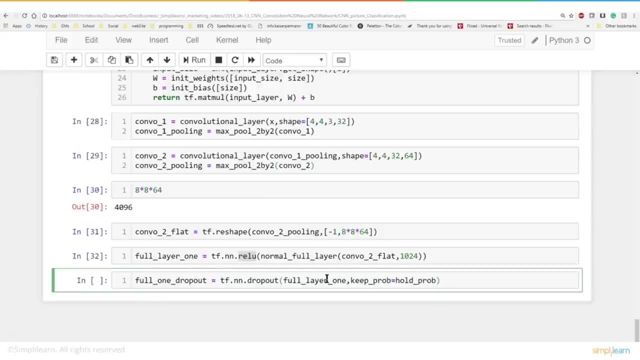 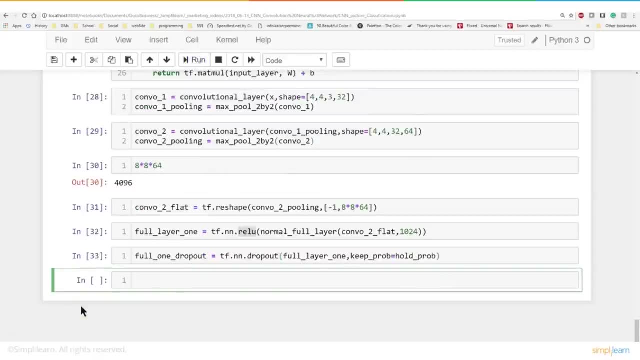 And this is going backwards and training the data. We're not training every weight, We're only training a percentage of them each time, which helps get rid of the bias. So let me go ahead and run that And finally, we'll go ahead and create a Y predict. 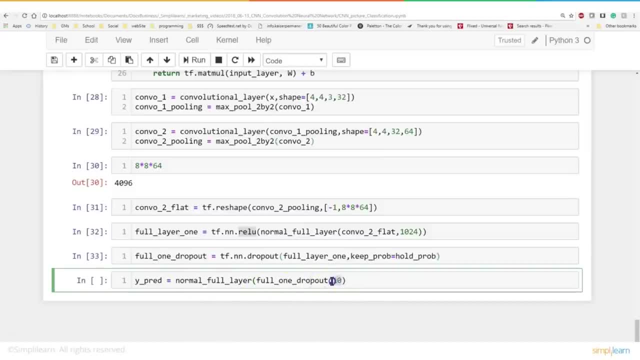 which is going to equal the normal full one dropout and 10, because we have 10 labels in there. Now in this neural network we could have added additional layers. That would be another option to play with. You can also play with instead of 1024,. 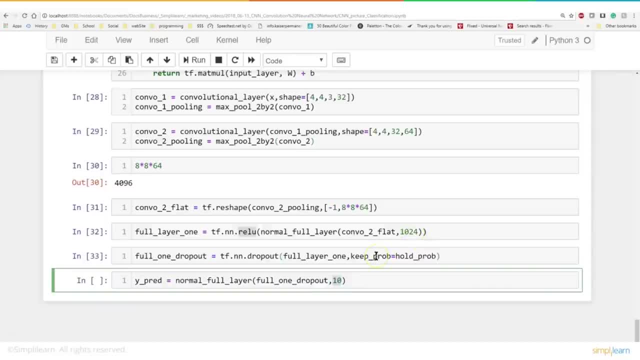 you can use other numbers for the way that sets up and what's coming out and going into the next one. We're only going to do just the one layer and the one layer dropout And you can see if we did another layer. it'd be really easy just to feed in the full one dropout. 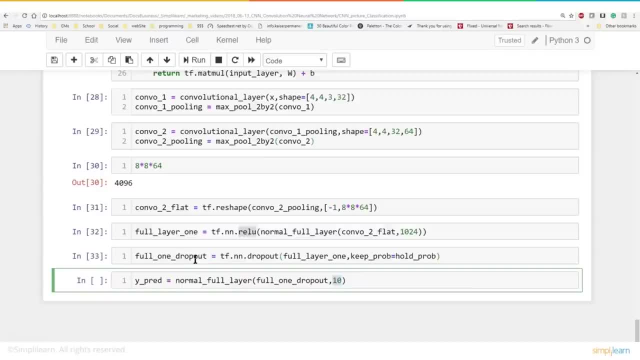 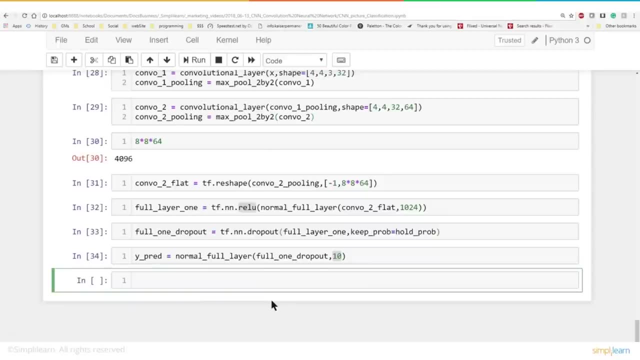 into full layer two And then full layer two dropout would have full layer two feed into it And then you'd switch that here for the Y prediction. For right now, this is great. This particular data set is tried and true and we know that this will work on it. 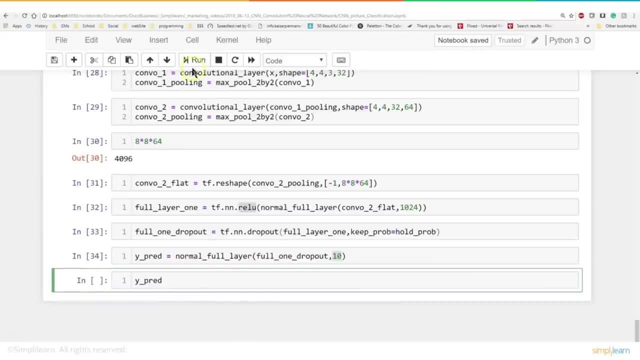 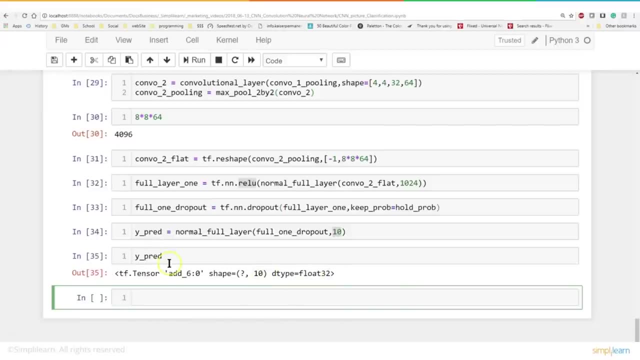 And if we just type in Y, predict, and we run that, we'll see that this is a tensor object shape. question mark 10, D, type 32.. A quick way to double check what we're working on. So now we've got all of our. 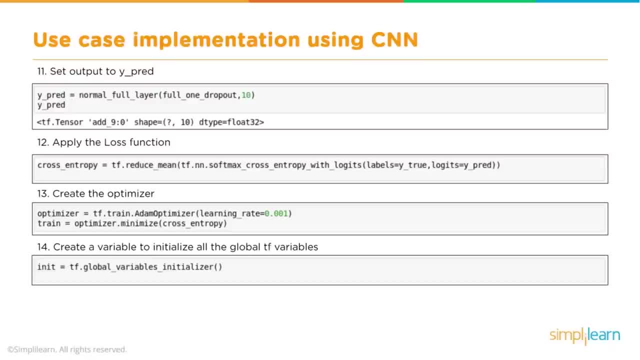 we've done a setup all the way into the Y predict, which we just did. We want to go ahead and apply the loss function and make sure that's set up in there, Create the optimizer and then train our optimizer and create a variable to initialize. 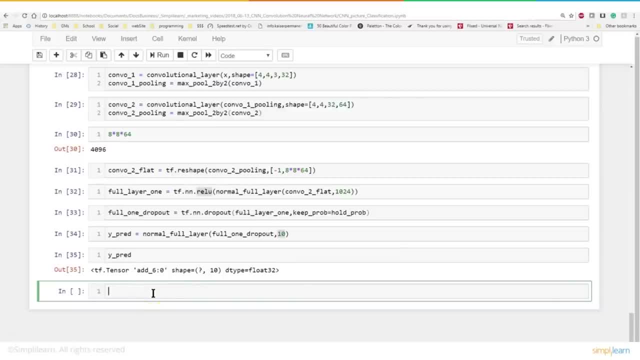 all the global TF variables. So before we dive in to the loss function, let me point out one quick thing, or just kind of a rehab over a couple things, And that is when we're playing with these setups. we pointed out up here that we can change the four, four. 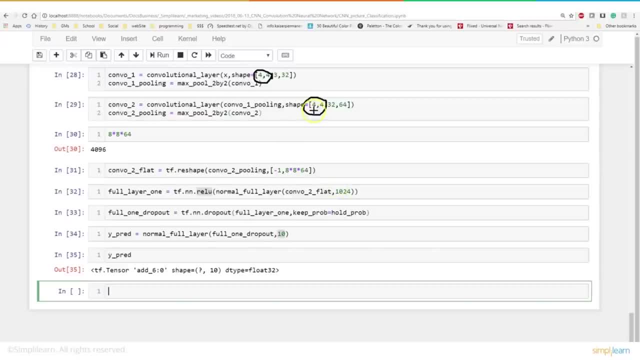 and use different numbers there, They change your outcome. So depending on what numbers you use here will have a huge impact on how well your model fits. And that's the same here with the 1024 also. This is also another number that if you continue to raise that number, 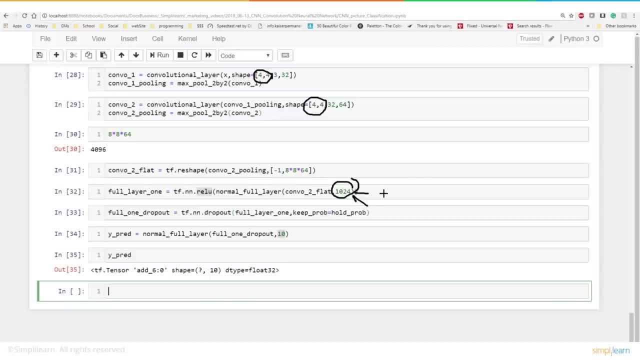 you'll get possibly a better fit. You might overfit And if you lower that number you'll use less resources And generally you want to use this in the exponential growth And exponential being two, four, eight, sixteen And in this case, 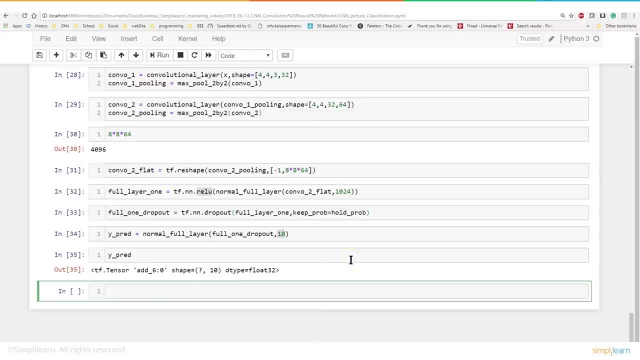 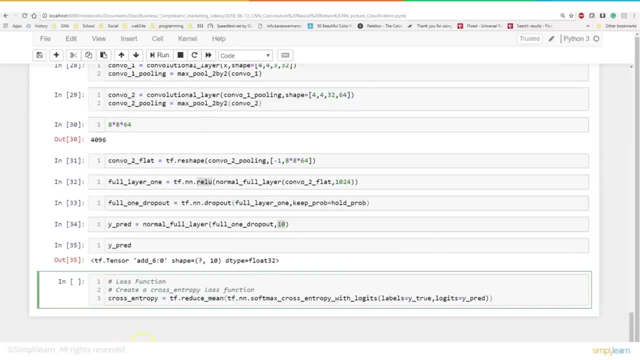 the next one down would be 512.. You can use any number there, but those would be the ideal numbers when you look at this data. So the next step in all this is we need to also create a way of tracking how good our model is. 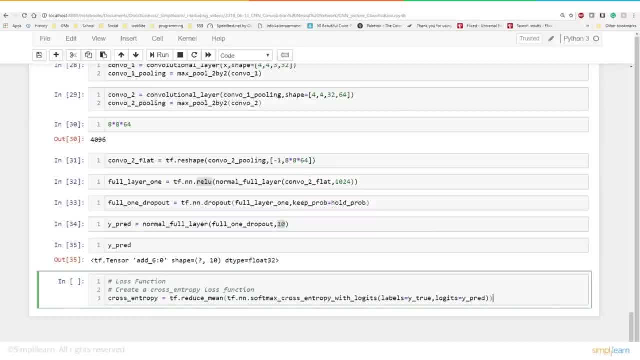 And we're going to call this a loss function, And so we're going to create a cross entropy loss function, And so, before we discuss exactly what that is, let's take a look and see what we're feeding it. We're going to feed it our labels. 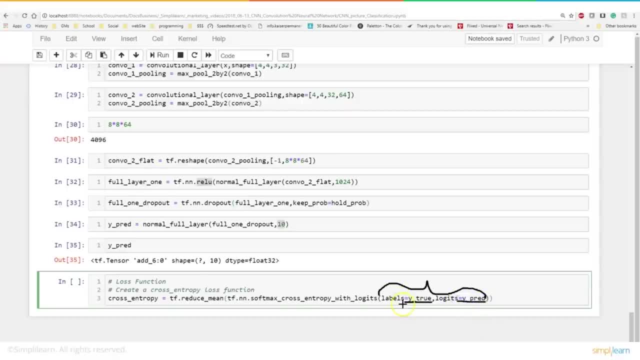 and we have our true labels and our prediction labels. So coming in here is where the two different variables we're sending in, or the two different probability distributions, is one that we know is true and what we think it's going to be. Now this function right here. 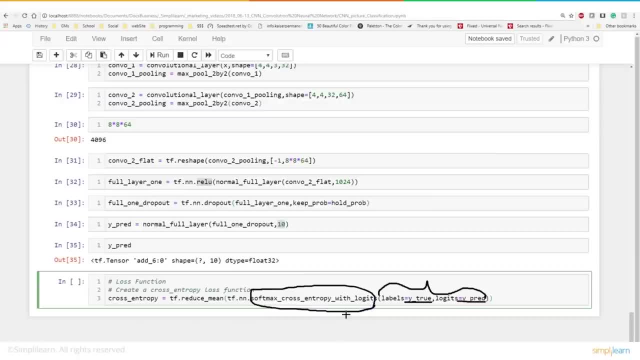 when they talk about cross entropy. in information theory, the cross entropy between two probability distributions over the same underlying set of events measures the average number of bits needed to identify an event drawn from the set. That's a mouthful, Really. we're just looking at. 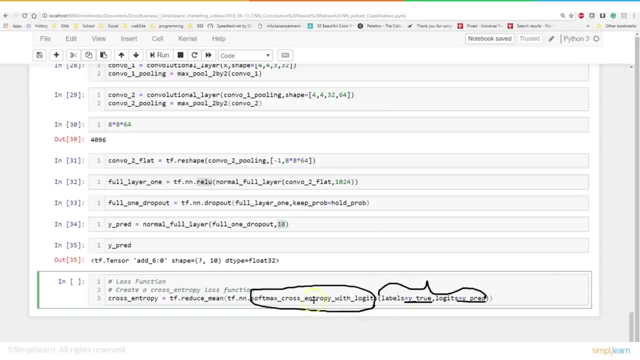 the amount of error in here, How many of these are correct and how many of these are incorrect. So how much of it matches? And we're going to look at that. we're just going to look at the average. That's what the mean. 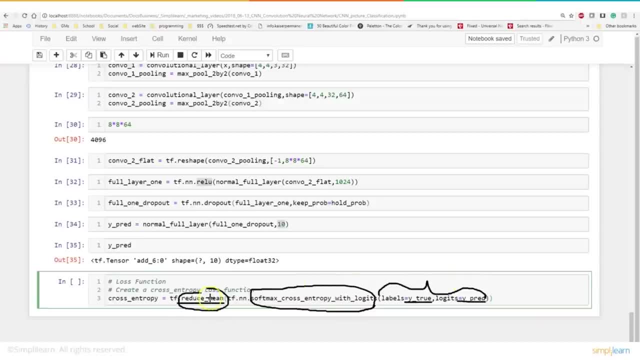 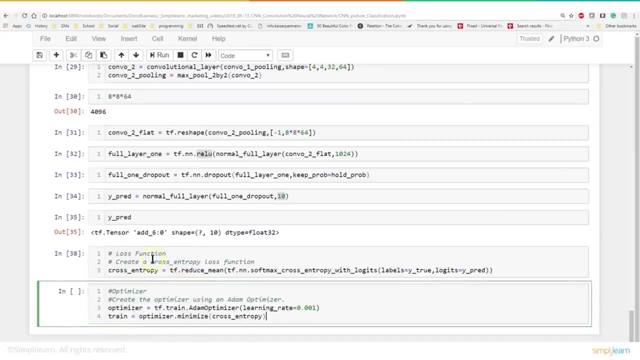 the reduced to the mean means here. So we're looking at the average error on this, And so the next step is we're going to take the error. We want to know our cross entropy or our loss function, how much loss we have. 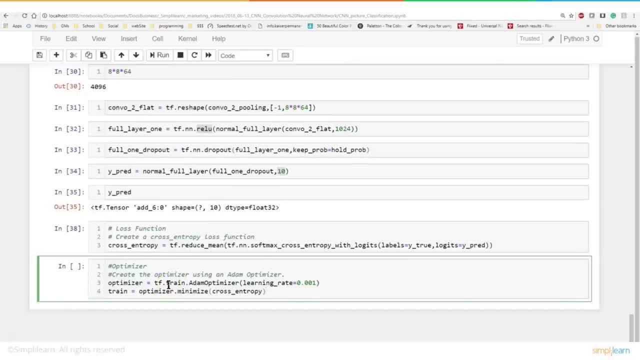 That's going to be part of how we train the model. So when you know what the loss is- and we're training it- you feed that back into the back propagation setup, And so we want to go ahead and optimize that. Here's our optimizer. 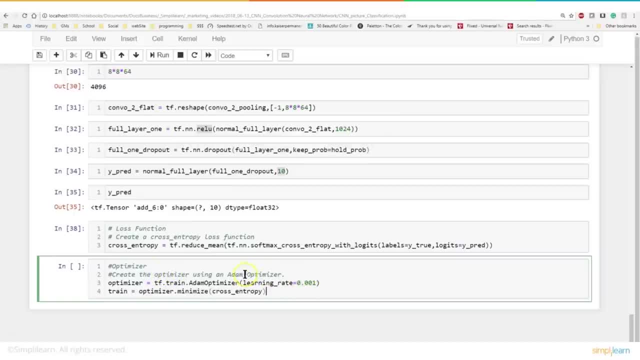 We're going to create the optimizer using an atom optimizer. Remember there's a lot of different ways of optimizing the data. Atom's the most popular used. So our optimizer is going to equal the tftrain atom optimizer. If you don't remember what the learning rate is, 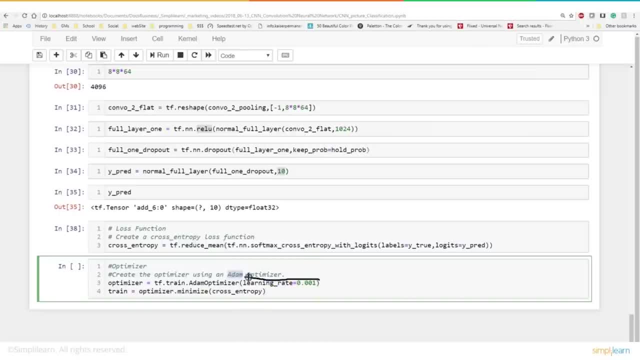 let me just pop this back into here. Here's our learning rate: When you have your weights, you have all your weights and your different nodes that are coming out. Here's our node: It has all its weights And then the error is being sent back through. 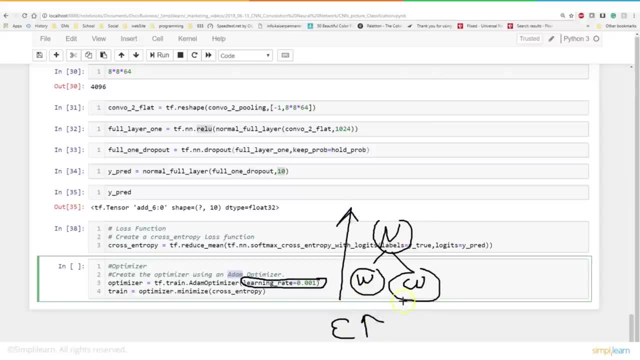 in reverse on our neural network. So we take this error and we adjust these weights based on the different formulas. In this case, the atom formula is what we're using. We don't want to just adjust them completely. We don't want to change this weight. 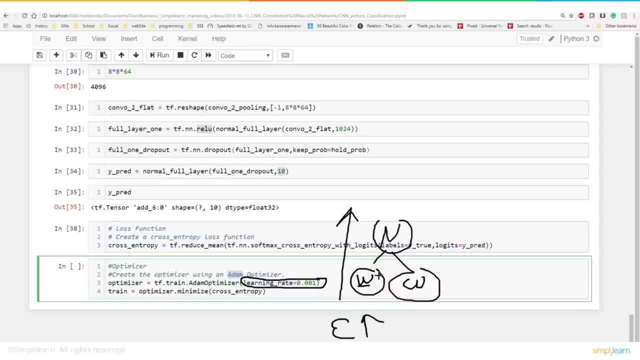 so it exactly fits the data coming through, Because if we made that kind of adjustment, it's going to be biased to whatever the last data we sent through is. Instead, we're going to multiply that by .001 and make a very small shift. 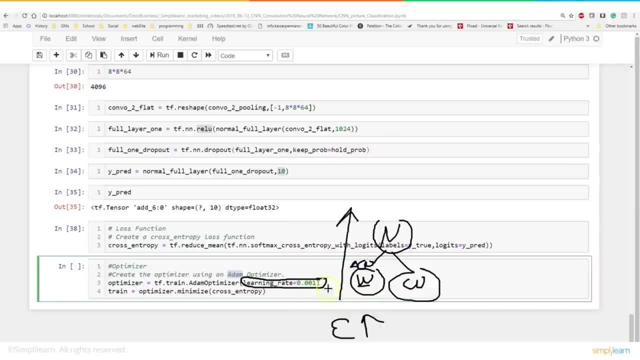 So our delta W is only .001 of the actual delta W of the full change. we're going to compute from the atom And then we want to go ahead and train it. So our training, or set up a training variable or function, And this is going to equal our optimizer. 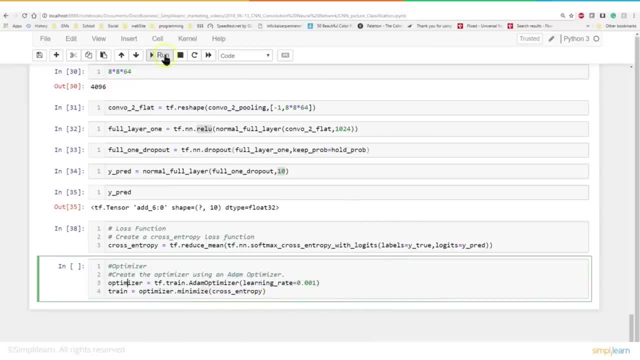 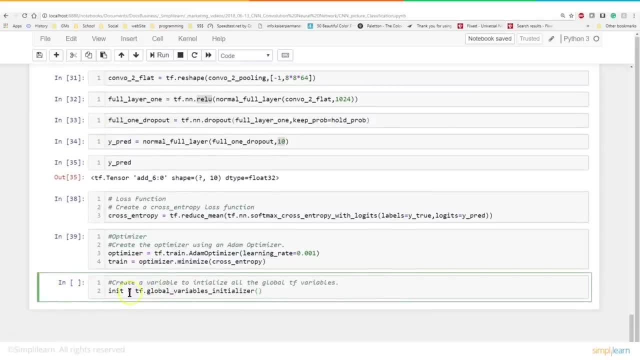 minimize cross entropy And we make sure we go ahead and run this So it's loaded in there And then we're almost ready to train our model. But before we do that, we need to create one more variable in here, And we're going to create a variable. 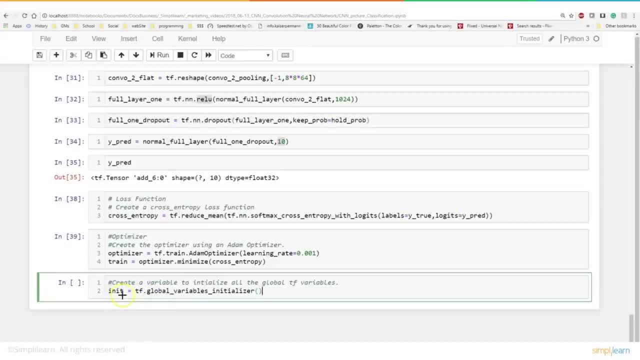 to initialize all the global TF variables And when we look at this, the TF global variable initializer- this is a TensorFlow object. It goes through there and it looks at all our different setup that we have going under our TensorFlow and then initializes those variables. 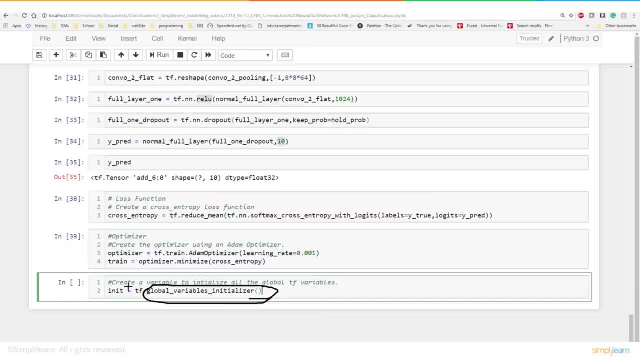 So it's kind of like a magic wand because it's all hidden in the back end of TensorFlow. All you need to know about this is that you have to have the initialization on there, which is an operation, And you have to run that once you have your setup going. 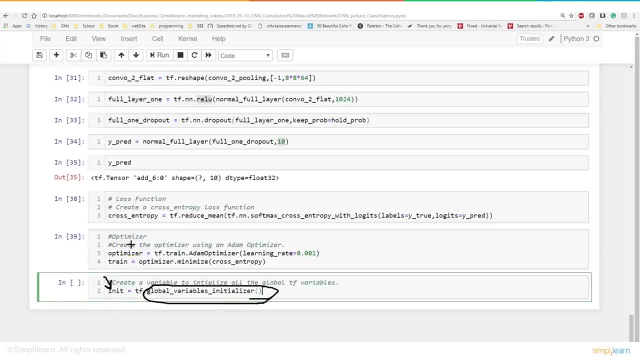 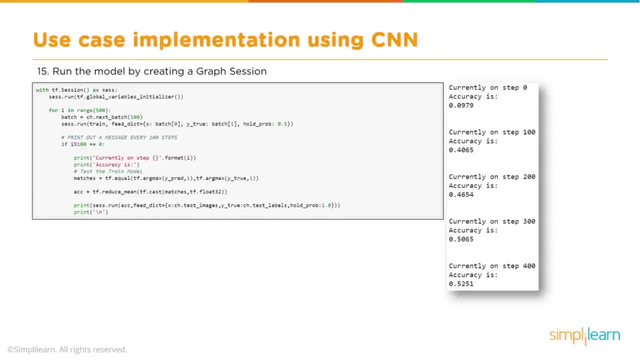 So we'll go ahead and run this piece of code, And then we're going to go ahead and train our data. So let me run this, So it's loaded up there, And so now we're going to go ahead and run the model by creating a graph session. 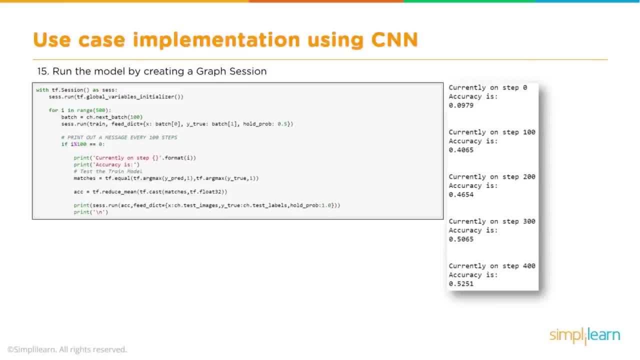 Graph session is a TensorFlow term, So you'll see that coming up. It's one of the things that throws me, because I always think of GraphX and Spark and graph as just general graphing, But they talk about a graph session, So we're going to go ahead and run the model. 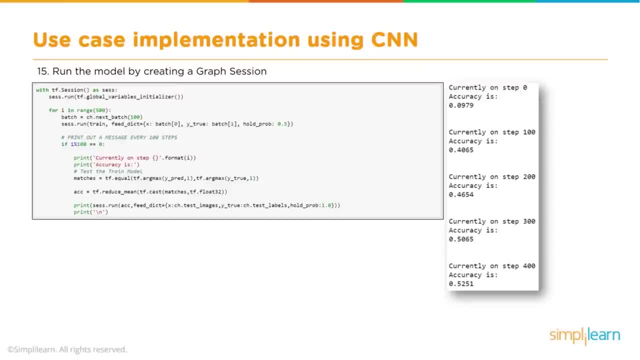 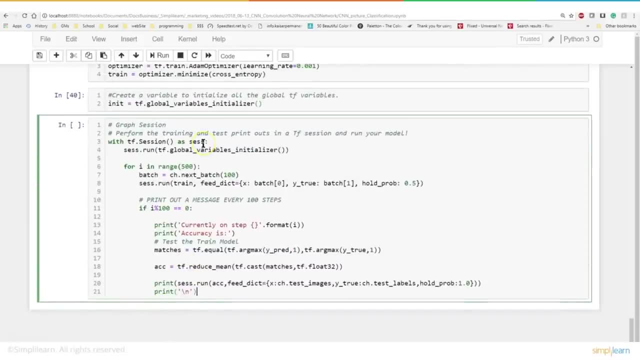 And let's go ahead and walk through this what's going on here, And let's paste this data in here. And here we go. So we're going to start off with a TF session as ses, So that's our actual TF session we've created. 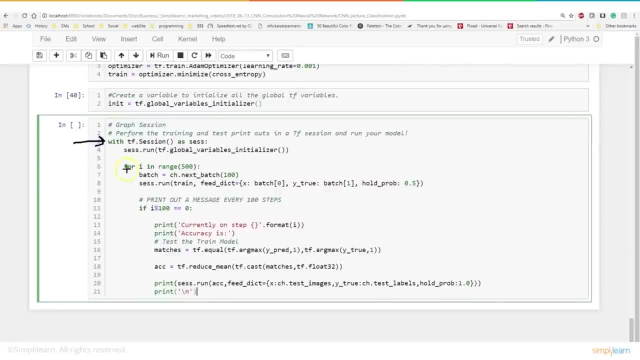 So we're right here with the TF session. Our session we're creating, we're going to run TF global variable initializer. So right off the bat we're initializing our variables here And then we have for i in range 500.. So what's going on here? 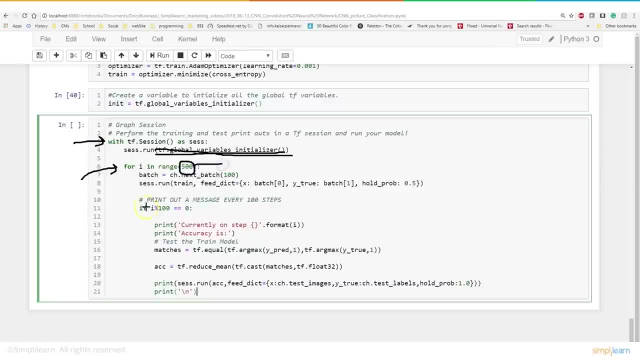 remember 500, we're going to pick the data up and we're going to batch it in at 500 points each. We've created our session run, So we're going to do with TF session as session right here. We've created our variable session. 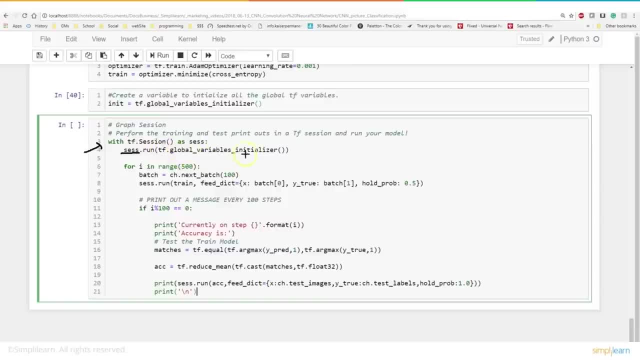 And then we're going to run and we're going to go ahead and initialize it. So we have our TF global variables initializer that we created. That initializes our session in here. The next thing we're going to do is we're going to go for i in range of 500. 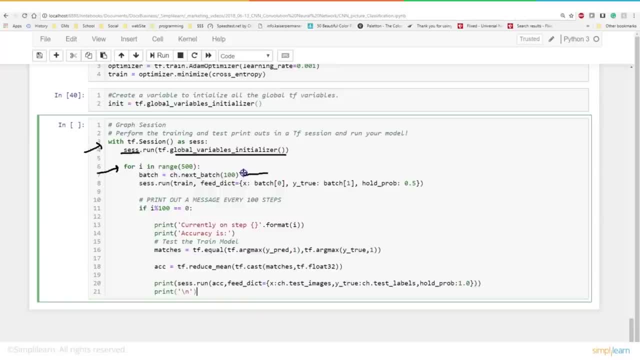 batch equals ch dot next batch. So, if you remember correctly, this is loading up 100 pictures at a time And this is going to loop through that 500 times. So we are literally doing what is that? 500 times 100 is 50,000.. 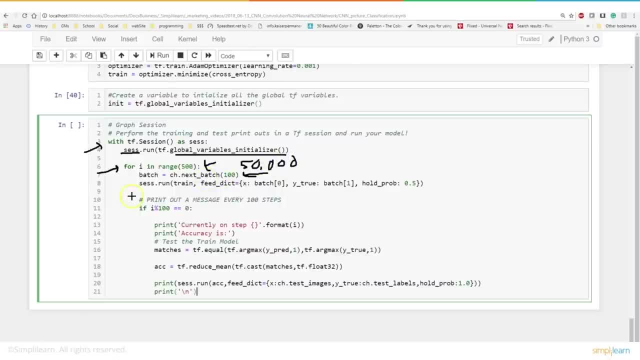 So that's 50,000 pictures we're going to process right there And the first process is: we're going to do a session run. We're going to take our train. We created our train variable or optimizer in there. We're going to feed it the dictionary. 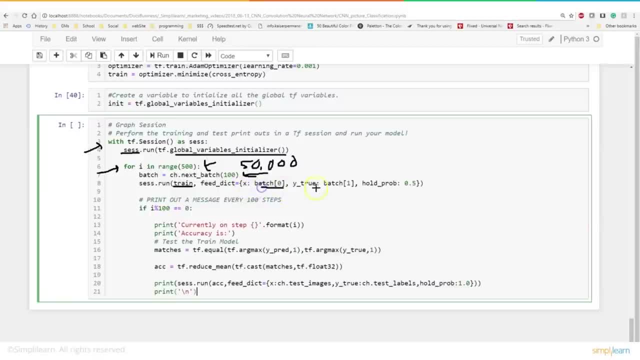 We had our feed dictionary that we created And we have x equals 0 coming in y, true batch one hold the probability 0.5.. And then, just so that we can keep track of what's going on, we're going to every 100 steps. 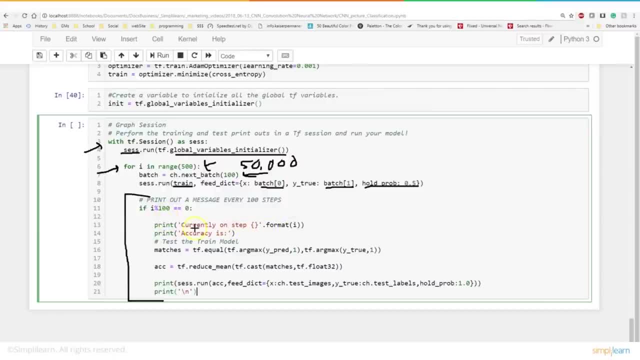 we're going to run a print. So currently on step format, accuracy is and we're going to look at matches: equals tf dot. equal tf argument y: prediction one: tf dot. arg max y, true comma one. So we're going to look at this. 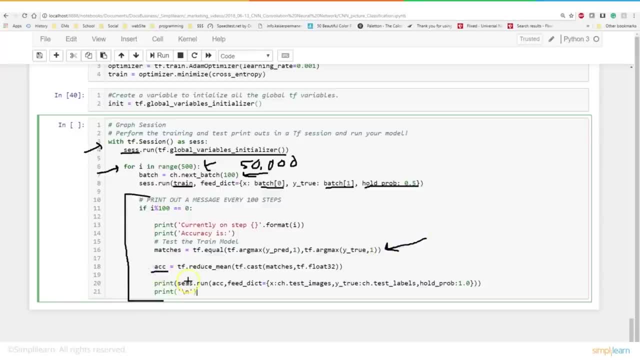 as how many matches it has. And here our ACC. all we're doing here is we're going to take the matches, how many matches they have. It creates, it generates a chart. We're going to convert that to float. That's what the tf cast does. 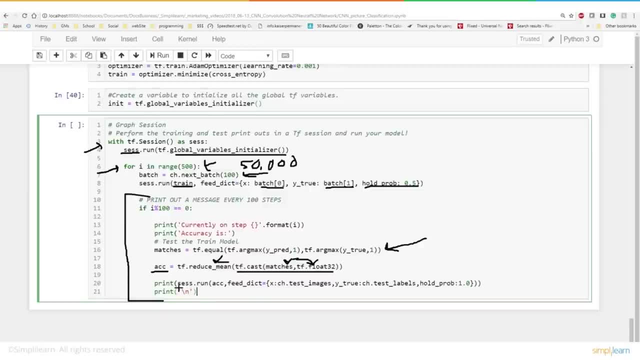 And then we just want to know the average. We just want to know the average of the accuracy, And then we'll go ahead and print that out. Print session run: accuracy feed dictionary. So it takes all this and it prints out our accuracy on there. 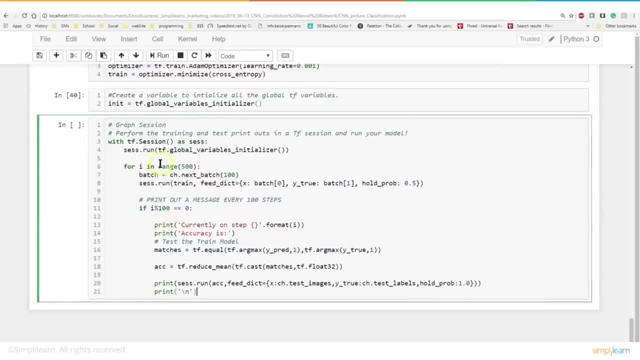 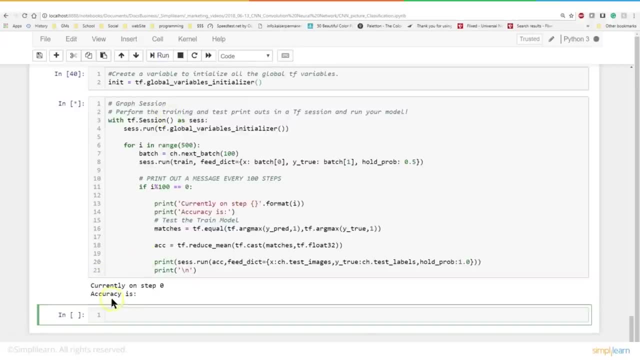 So let's go ahead and take this Screen's there, Let's go ahead and take this and let's run it, And this is going to take a little bit to run. So let's see what happens on my old laptop And we'll see here that we have our current. 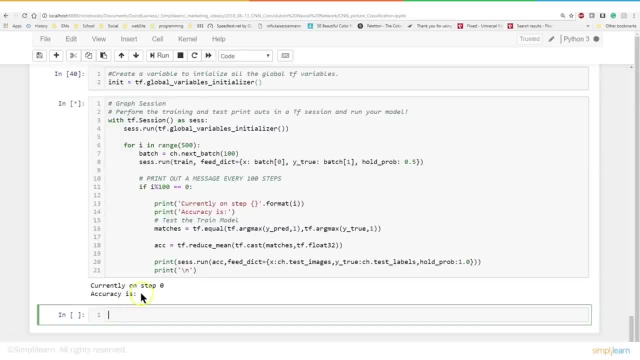 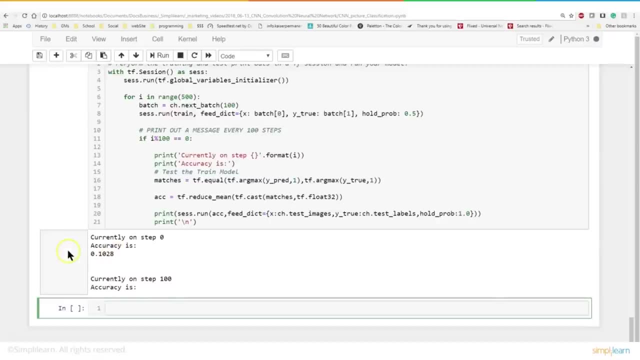 we're currently on step zero. It takes a little bit to get through the accuracy And this will take just a moment to run. We can see that on our step zero it has an accuracy of 0.1 or 0.1028.. 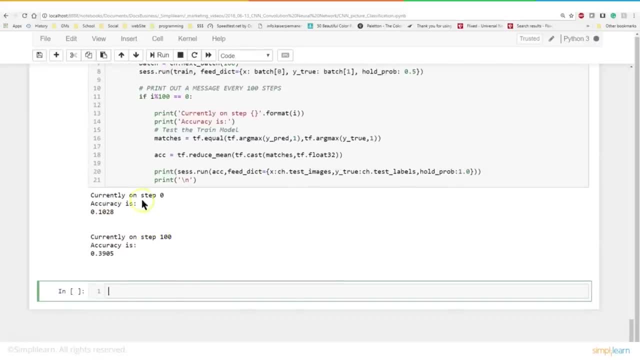 And as it's running, we'll go ahead. you don't need to watch it run all the way, but this accuracy is going to change a little bit up and down. So we've actually lost some accuracy during our step two, But we'll see how that comes out. 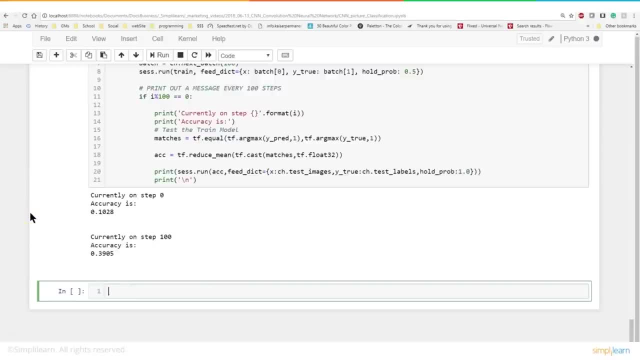 Let's come back after we run it all the way through and see how the different steps come out. I was actually reading that backwards. The way this works is: the closer we get to one, the more accuracy we have. So you can see here. 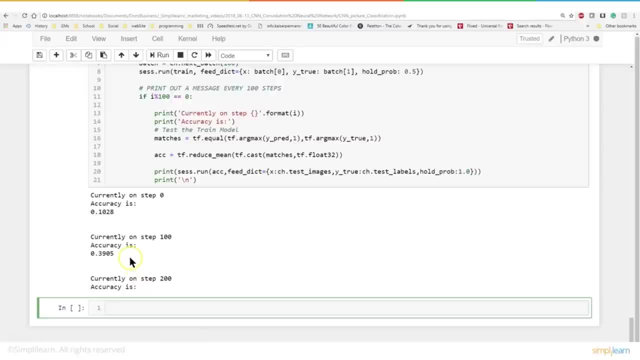 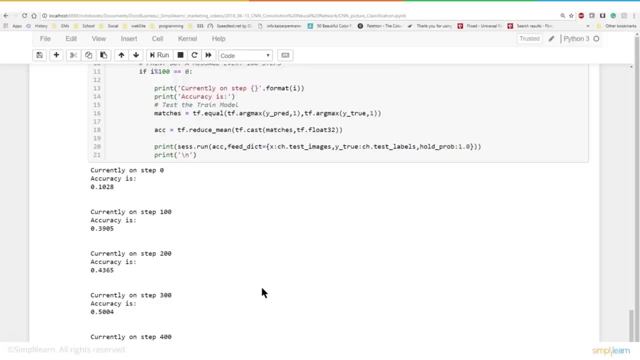 we've gone from a 0.1 to a 0.39.. And we'll go ahead and pause this and come back and see what happens when we're done with the full run. All right, Now that we've prepared the meal. 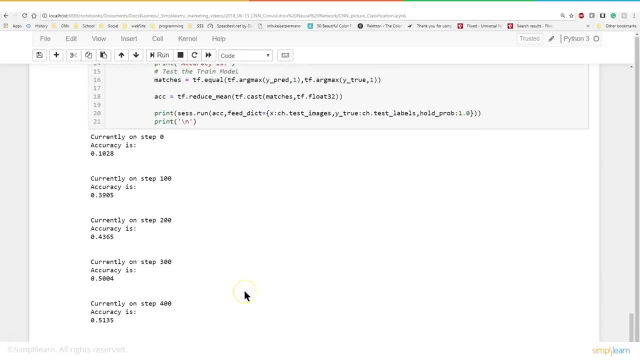 got it in the oven and pulled out my finished dish here. If you've ever watched any of the old cooking shows. let's discuss a little bit about this accuracy going on here, And how do you interpret that. We've done a couple things. 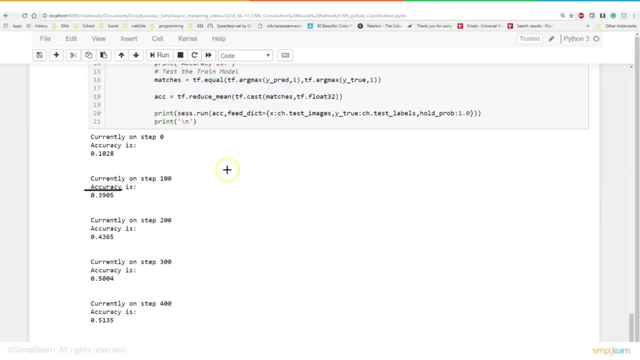 First, we've defined accuracy. The reason I got it backwards before is you have loss or accuracy, And with loss you'll get a graph that looks like this. It goes: oops, that's an S, by the way. There we go. 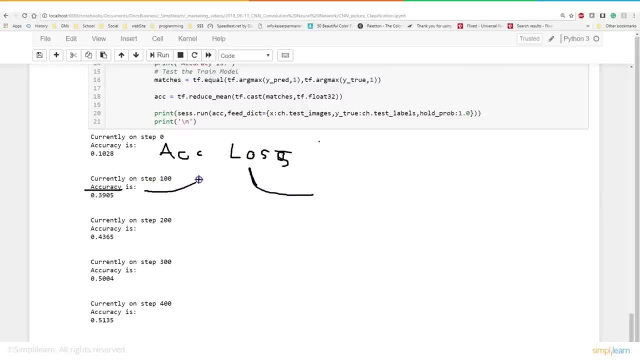 You get a graph that curves down like this, And with accuracy, you get a graph that curves up. This is how good it's doing. Now, in this case, one is supposed to be really good accuracy- That means it gets close to one. 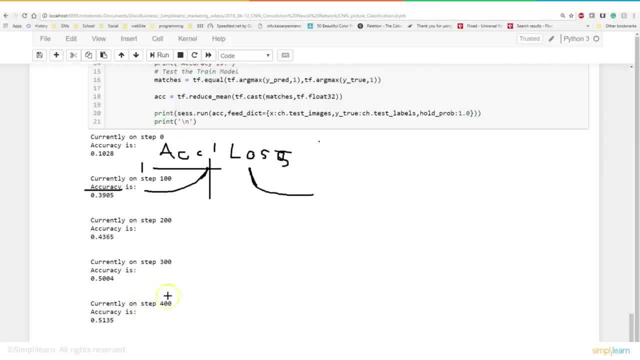 but it never crosses one. So if you have an accuracy of one, that is phenomenal- In fact, that's pretty much unheard of. And the same thing with loss: If you have a loss of zero, that's also unheard of. Zero is actually on this axis, right here. 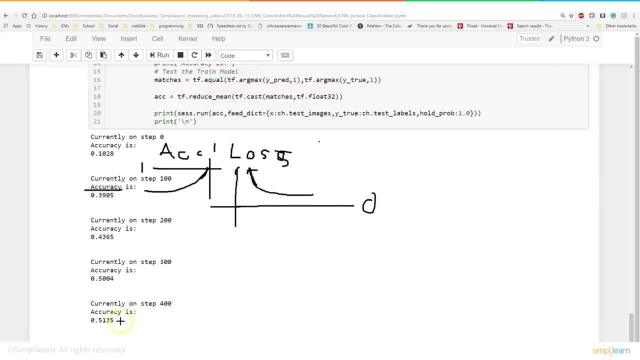 as we go in there. So how do we interpret that? Because if I was looking at this and I go, oh, 0.51,, that's 51%, You're doing 50-50.. No, this is not percentage. 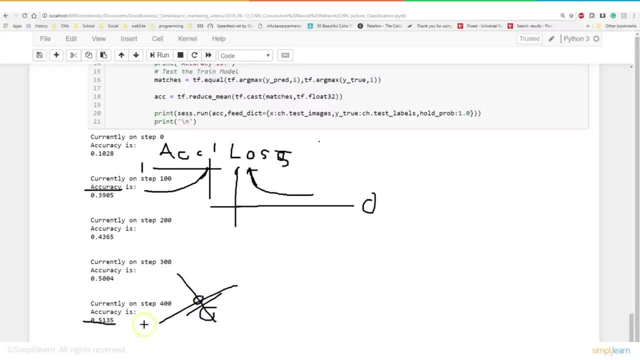 Let me just put that in here. It is not percentage, This is logarithmic. What that means is that 0.2 is twice as good as 0.1. And when we see 0.4, that's twice as good as 0.2.. 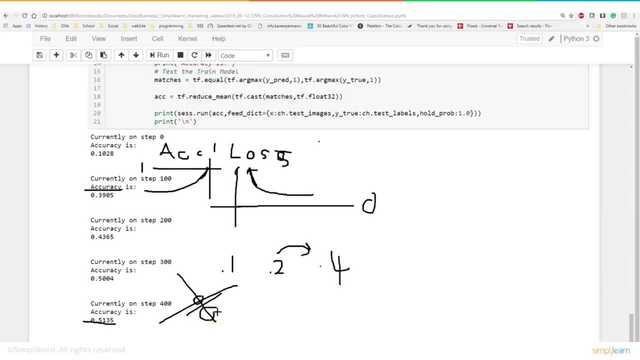 Real way to convert this into a percentage. You really can't say this is a direct percentage conversion. What you can do, though, is in your head: if we were to give this a percentage, we might look at this as 50%. 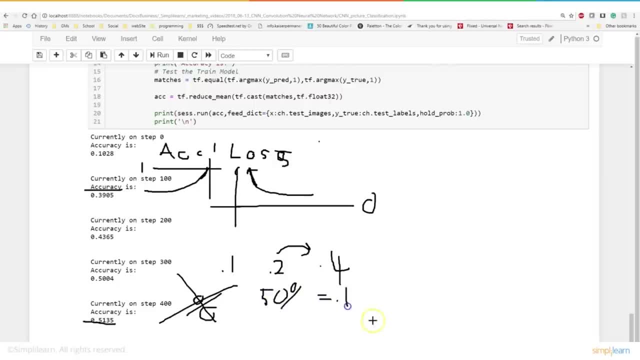 or just guessing- equals 0.1. And if 50% roughly equals 0.1, that's where we started up here at the top, Remember, at the top here here's our 0.1028.. The accuracy of 50%. 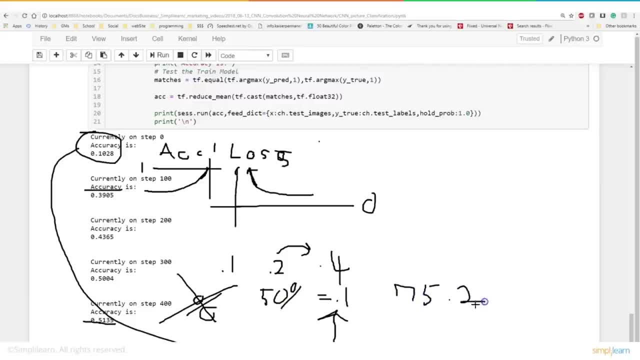 then 75% is about 0.2, and so on and so on. Don't quote those numbers, because that doesn't work that way. They say that if you have 0.95,, that's pretty much saying 100%, And if you have anywhere between 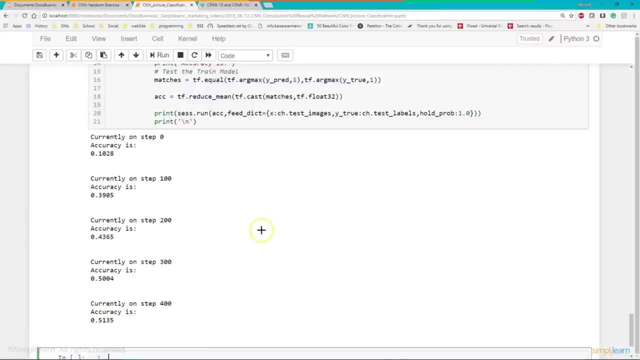 you'd have to go look this up. Let me go ahead and remove all my drawings there. So the magic number is 0.5.. We really want to be over a 0.5 in this whole thing And we have both 0.5004.. 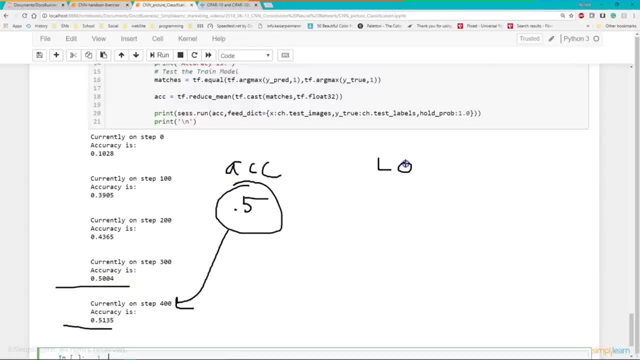 Remember, this is accuracy. If we were looking at loss then we'd be looking the other way. But 0.05, instead of how high it is, we want how low it is. But with accuracy, being over a 0.5 is pretty valid. 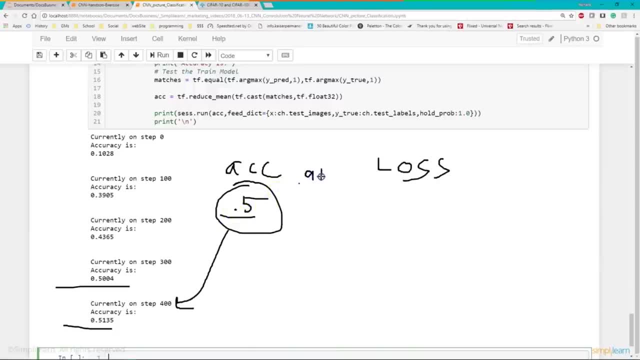 That means this is pretty solid, And if you get to a 0.95, then it's a direct correlation. That's what we're looking for here in these numbers And you can see we finished with this model at 0.5135,, so still good. 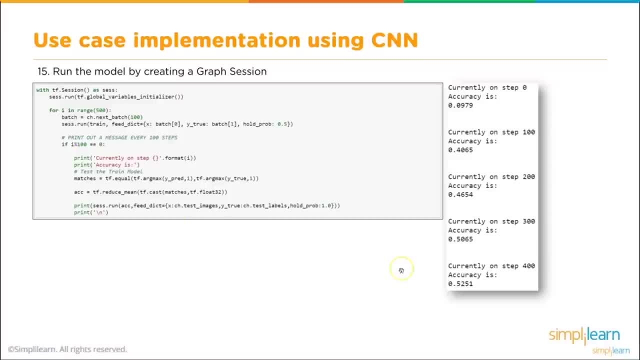 And if we look at when they ran this in the other end- remember there's a lot of randomness that goes into it- when we seed the weights, They got 0.5251, so a little better than ours, But that's fine. 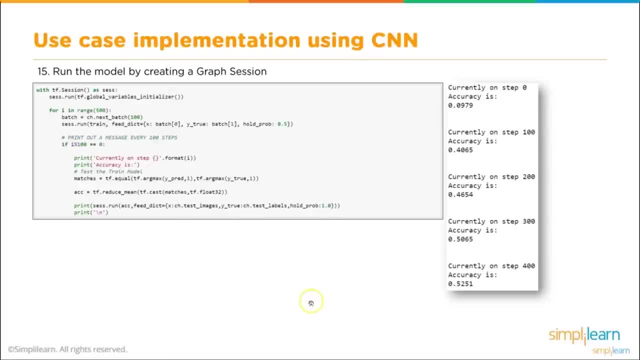 You'll find your own comes up a little bit better or worse, depending on just that randomness. And so we've gone through the whole model We've created, we've trained the model and we've also gone through on every 100th run. 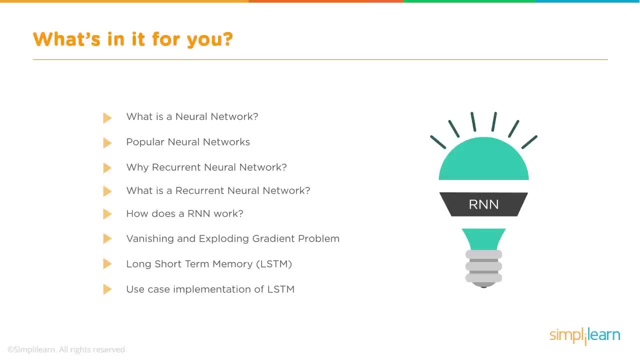 to test the model to see how accurate it is. We will start with, of course, the fundamentals. What is a neural network? In popular neural networks, it's important to know the framework we're in and what we're going to be looking at specifically. 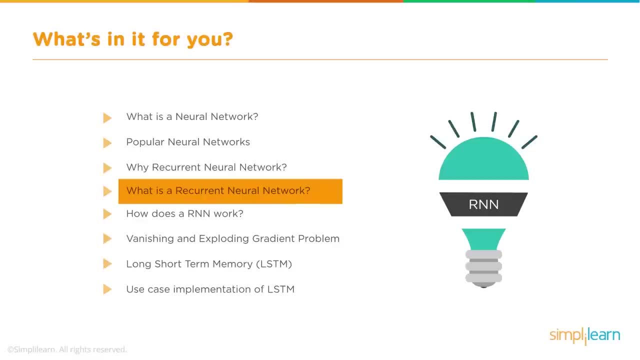 Then we'll touch on why a recurrent neural network, what is a recurrent neural network and how does an RNN work? One of the big things about RNNs is what they call the vanishing and exploding gradient problem, So we'll look at that. 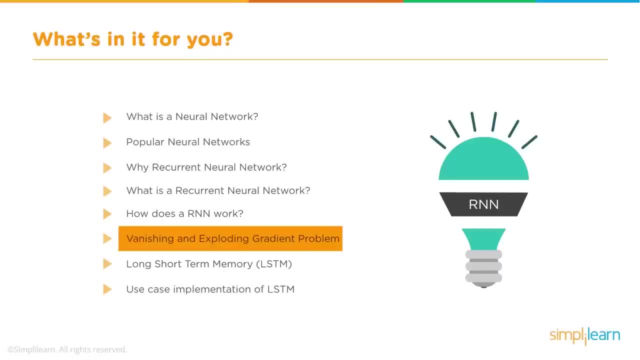 And then we're going to be using a use case study. It's going to be in Keras on TensorFlow. Keras is a Python module for doing neural networks in deep learning, And in there there's what they call long short-term memory- LSTM. 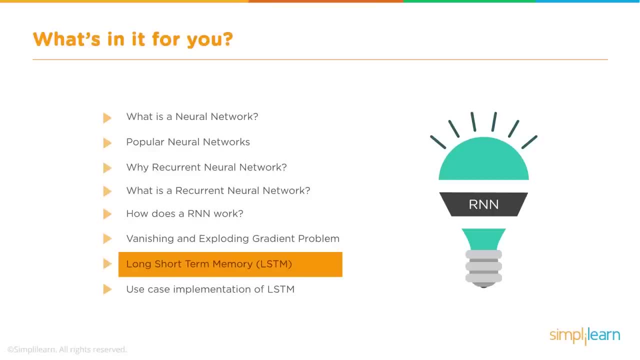 And then we'll use the use case to implement our LSTM on the Keras. So when you see that LSTM, that is basically the RNN network And we'll get into that. The use case is always my favorite part Before we dive into any of this. 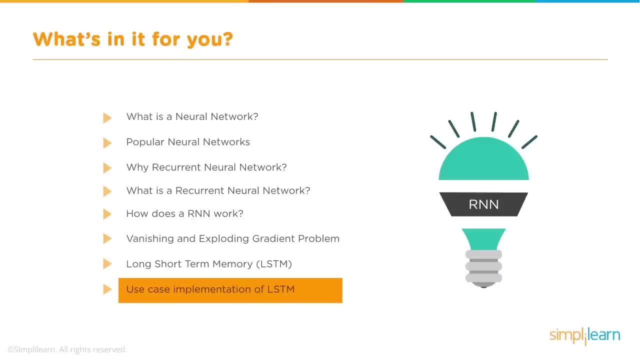 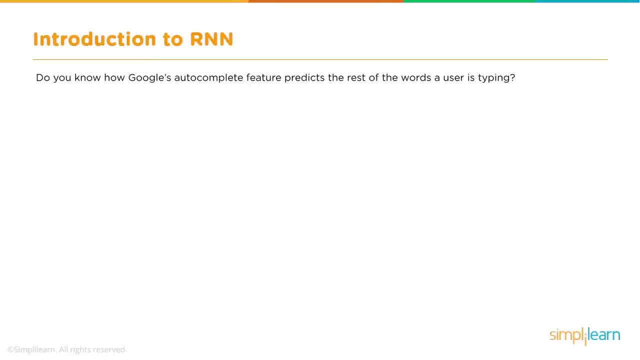 we're going to take a look at what is an RNN or an introduction to the RNN. Do you know how Google's autocomplete feature predicts the rest of the words a user is typing? I love that autocomplete feature as I'm typing away. 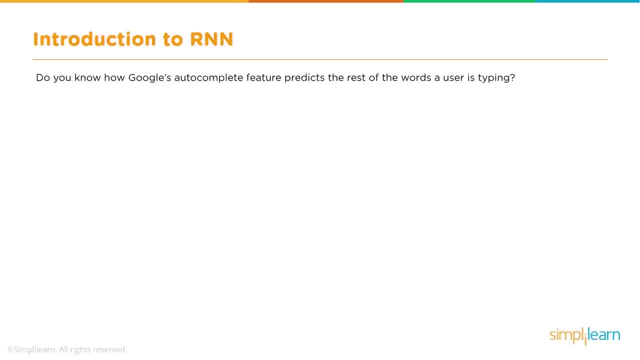 It saves me a lot of time. I can just kind of hit the enter key and it autofills everything and I don't have to type as much. Well, first is a collection of large volumes of most frequently occurring consecutive words. This is fed into a recurrent neural network. 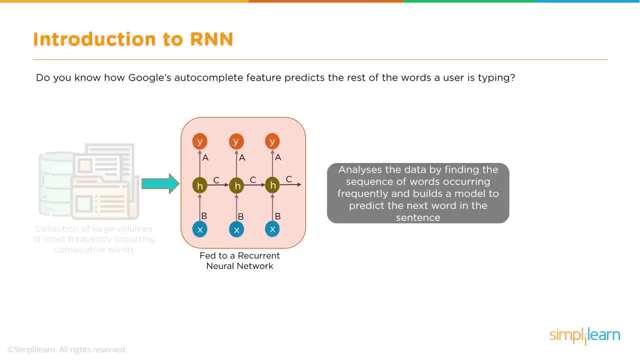 analysis the data by finding the sequence of words occurring frequently and builds a model to predict the next word in the sentence. And then Google: what is the best food to eat in Los? I'm guessing you're going to say Los, Mexico, No? 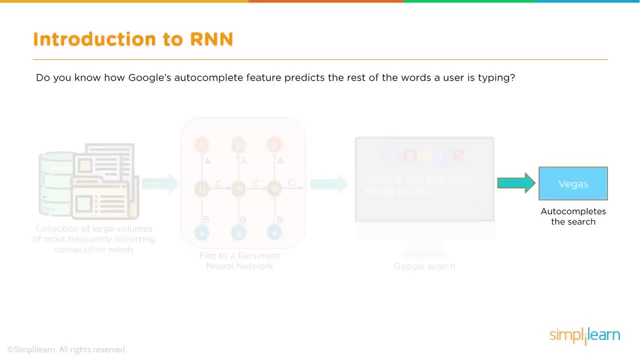 It's going to be Las Vegas. So the Google search will take a look at that and say, hey, the most common autocomplete is going to be Vegas in there, And usually it gives you three or four different choices. So it's a very powerful tool. 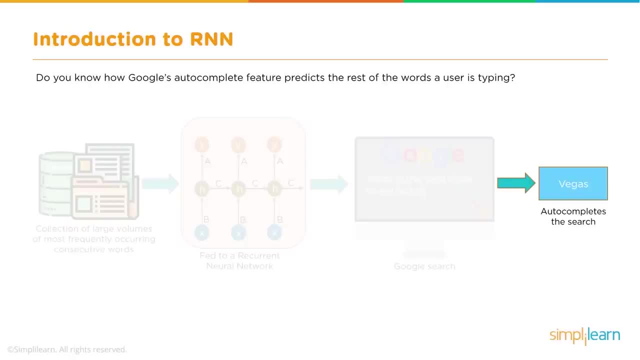 It saves us a lot of time, especially when we're doing a Google search or even in Microsoft words has a. Some people get very mad at it because it autofills with the wrong stuff, But you know you're typing away and it helps you autofill. 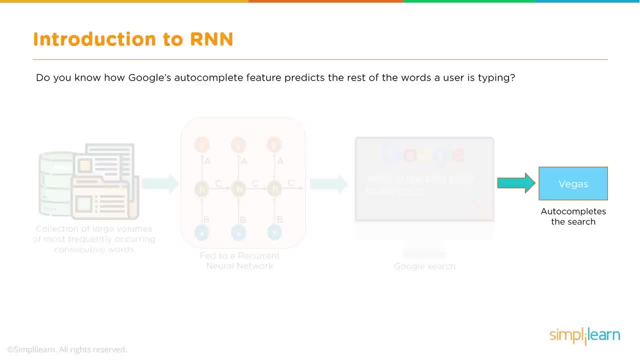 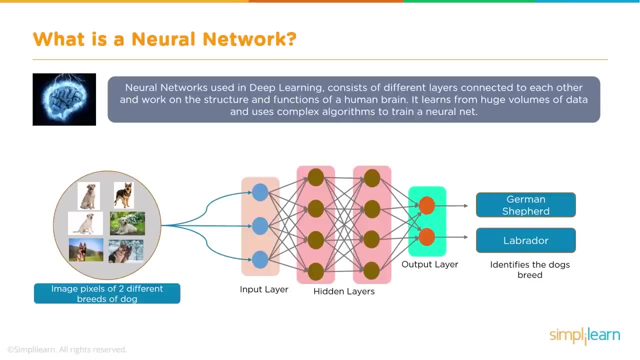 I have that in a lot of my different packages. It's just a standard feature that we're all used to now. So before we dive into the RNN and getting into the depths, let's go ahead and talk about what is a neural network. 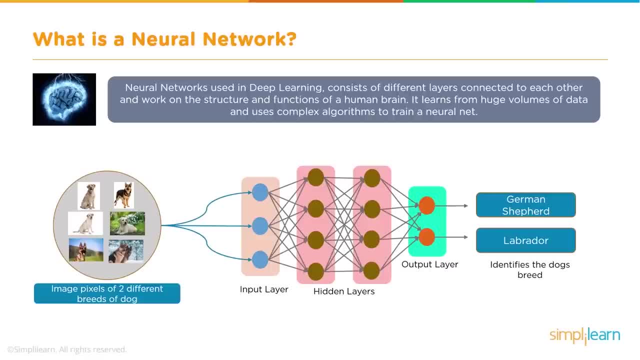 Neural networks used in deep learning consist of different layers connected to each other and work on the structure and functions of a human brain. You're going to see that thread- human in human brain and human thinking throughout deep learning, The only way we can evaluate an artificial intelligence or anything like that. 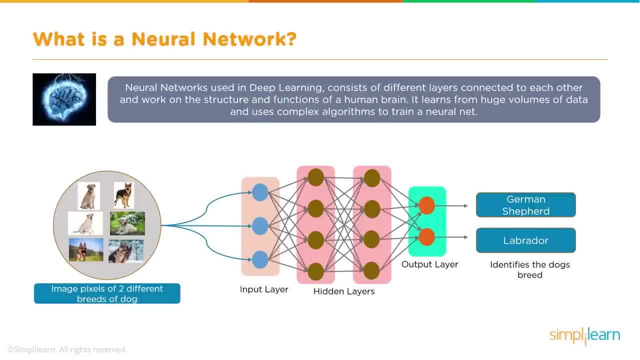 is to compare it to human function- Very important note on there- And it learns from huge volumes of data And it uses complex algorithms to train a neural net. So in here we have image pixels of two different breeds of dog. One looks like a nice floppy-eared lab. 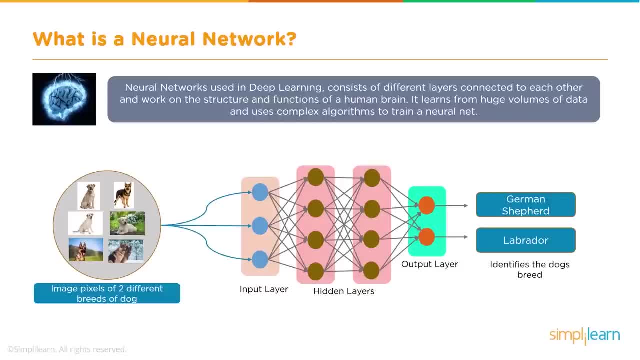 and one a German Shepherd. You know both wonderful breeds of animals. That image then goes into an input layer. That input layer might be formatted at some point because you have to let it know like different pictures are going to be different sizes and different color content. 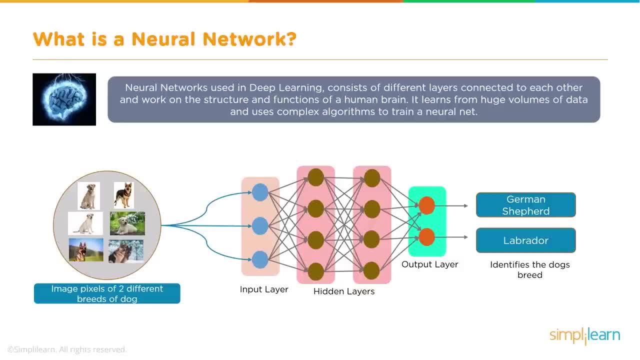 Then it'll feed into hidden layers. So each of those pixels or each point of data goes in and then splits into the hidden layer, which then goes into another hidden layer, which then goes to an output layer, RNN. there's some changes in there. 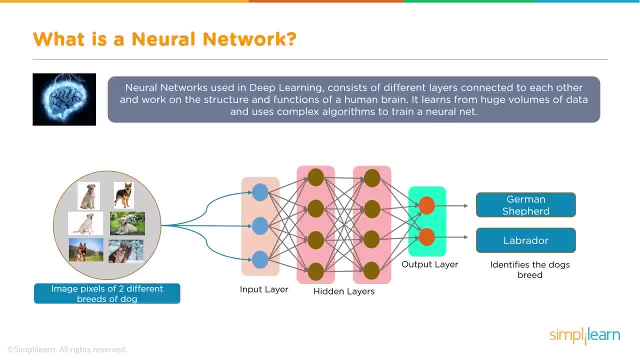 which we're going to get into. So it's not just a straightforward propagation of data, like we've covered in many other tutorials. And finally you have an output layer, and the output layer has two outputs. It has one that lights up if it's a German Shepherd. 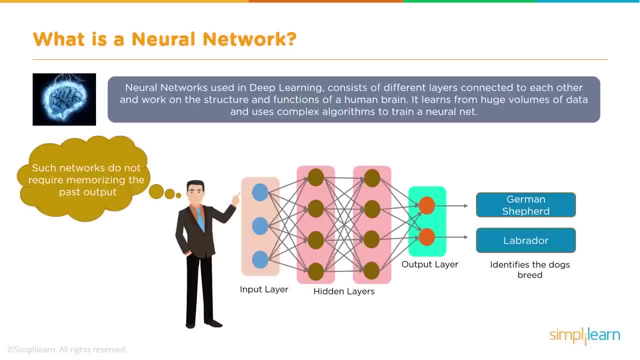 and another that lights up if it's a Labrador So it identifies the dog's breed. Set networks do not require memorizing the past output, So our forward propagation is just that: It goes forward and doesn't have to re-memorize stuff. 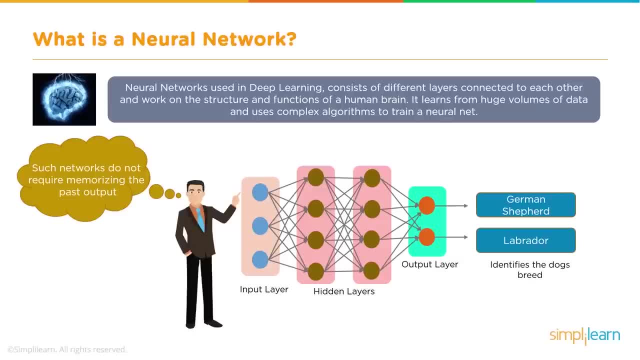 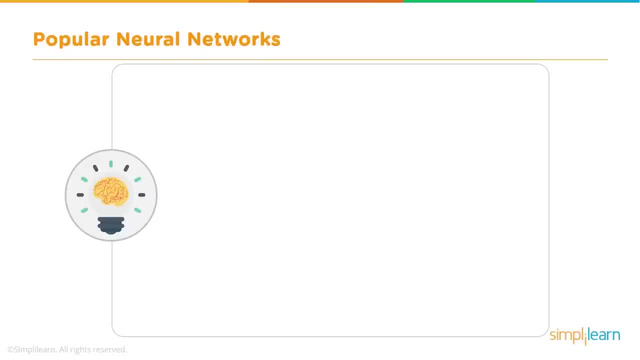 And you can see there that's not actually me in the picture, dressed up in my suit. I haven't worn a suit in years, So as we're looking at this, we're going to change it up a little bit. Before we cover that, let's talk about popular neural networks. 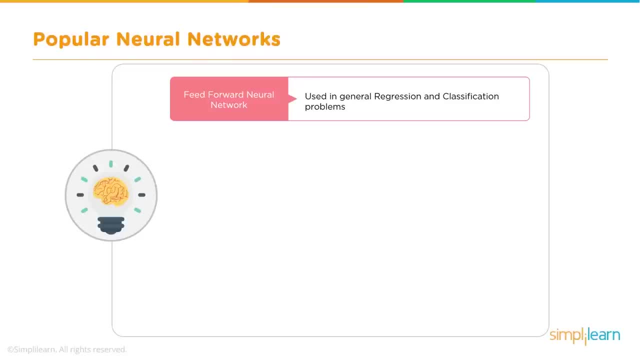 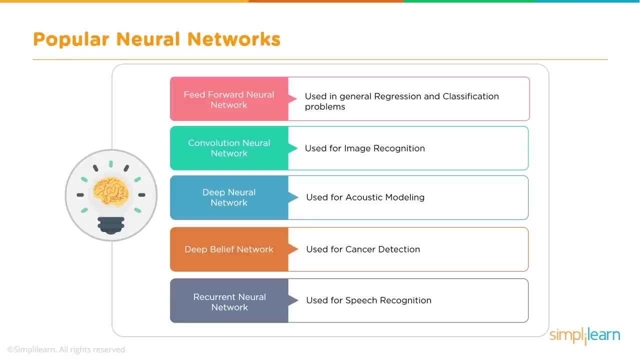 First, there's the feed forward neural network, used in general regression and classification problems, And we have the convolution neural network, used for image recognition, Deep neural network used for acoustic modeling, Deep belief network used for cancer detection, And recurrent neural network used for speech recognition. 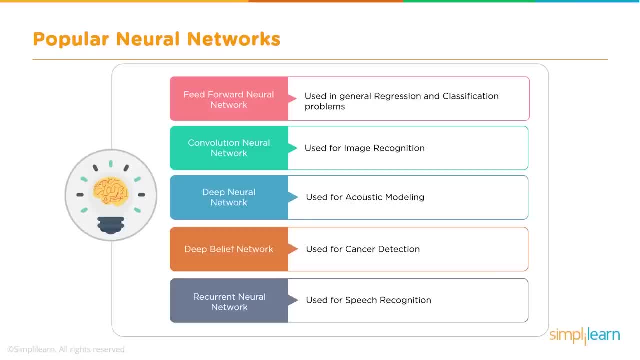 Now taking a lot of these and mixed them around a little bit. so just because it's used for one thing doesn't mean it can't be used for other modeling. But generally this is where the field is and this is how those models are generally being used right now. 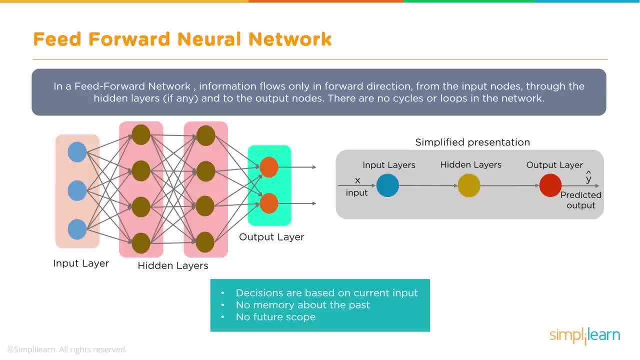 So we talk about a feed forward neural network. In a feed forward neural network, information flows only in the forward direction from the input nodes through the hidden layers, if any, and to the output nodes. There are no cycles or loops in the network, And so you can see here: 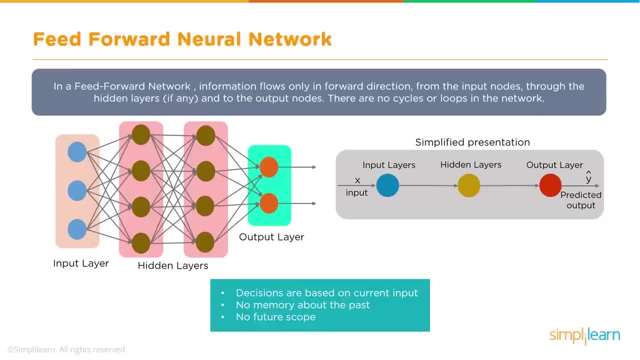 we have our input layer and I was talking about how it just goes straight forward into the hidden layers, so each one of those connects and then connects to the next hidden layer and connects to the output layer And of course we have a nice simplified version where it has a predicted output. 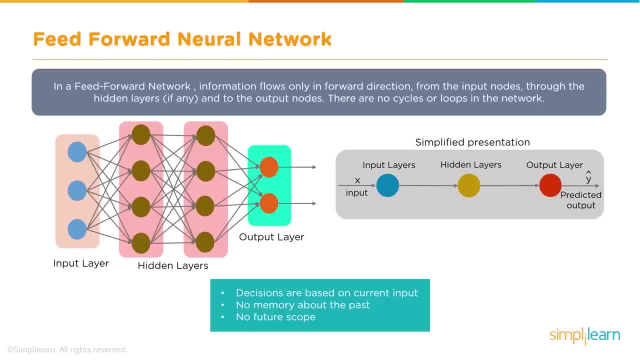 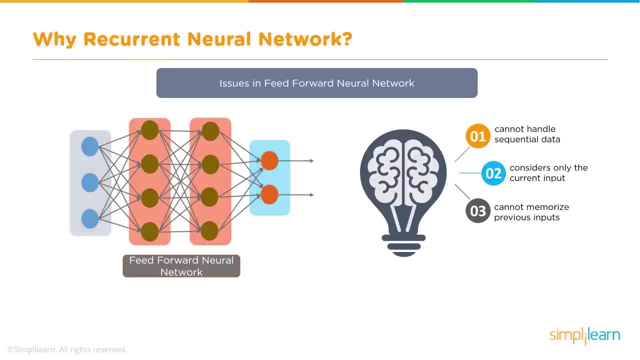 and they refer to the input as X a lot of times, and the output as Y. Decisions are based on current input, no memory about the past, no future scope. Why? recurrent neural network Issues in feed forward neural network, So one of the biggest issues. 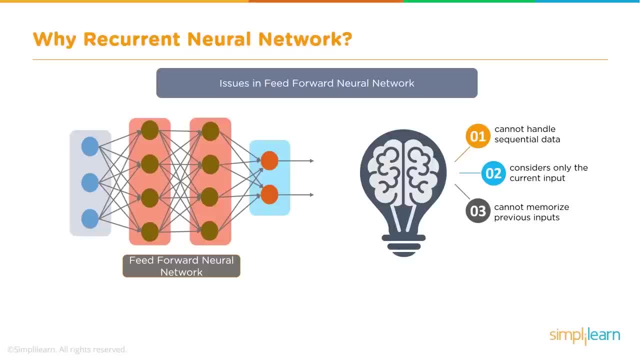 is because it doesn't have a scope of memory or time. a feed forward neural network doesn't know how to handle sequential data. It only considers only the current input. So if you have a series of things, and because three points back affects what's happening now, 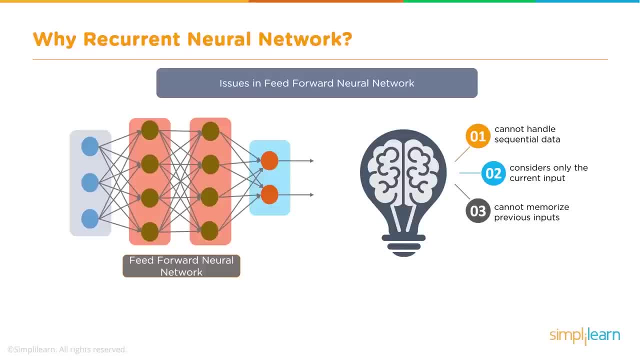 and what's your output affects what's happening. that's very important. so whatever I put as an output is going to affect the next one. A feed forward doesn't look at any of that. it just looks at this is what's coming in and it cannot memorize. 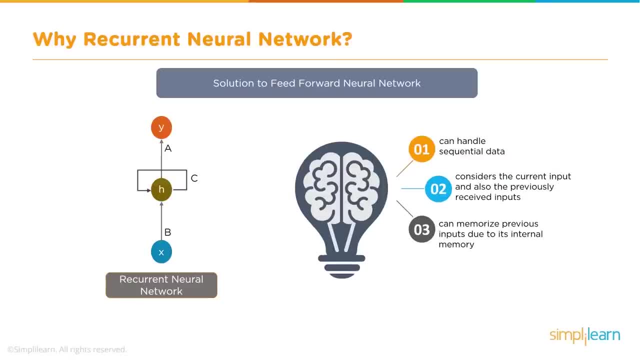 previous inputs, so it doesn't have that list of inputs coming in. Solution to feed forward neural network. You'll see here where it says recurrent neural network and we have our X on the bottom going to H, going to Y. that's your feed forward. 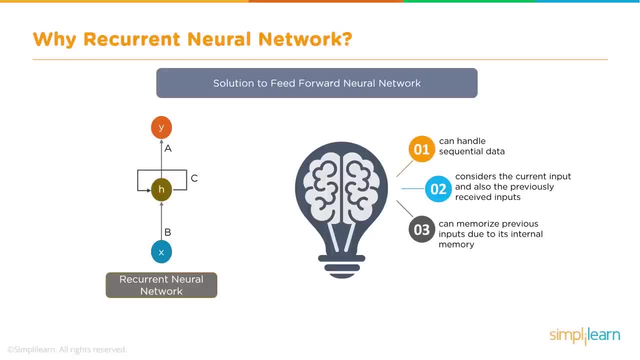 But right in the middle it has a value C. so there's a whole other process that's memorizing what's going on in the hidden layers, and the hidden layers, as they produce data, feed in to the next one, So your hidden layer might have an output. 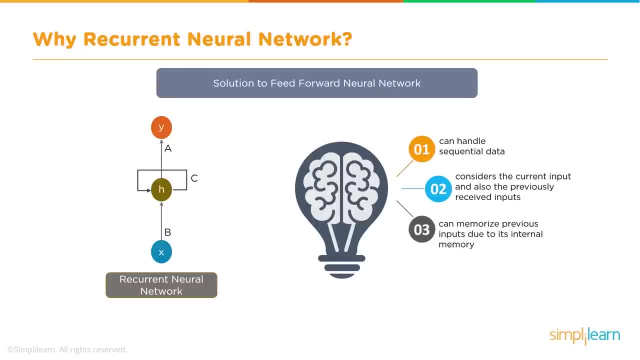 that goes off to Y, but that output goes back into the next prediction coming in. What this does is: this allows it to handle sequential data. It considers the current input and also the previously received inputs And, if we're going to look at general drawings, 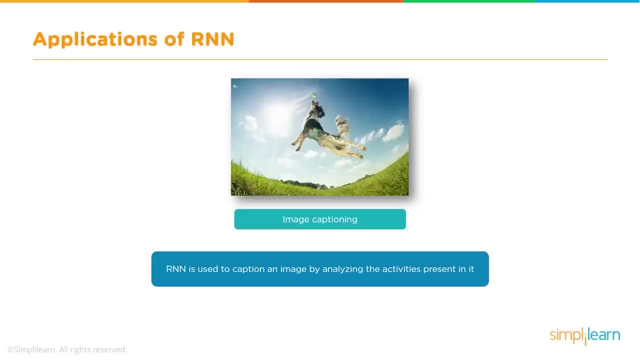 and solutions. we should also look at applications of the RNN Image captioning. RNN is used to caption an image by analyzing the activities present in it: A dog catching a dog or catching a ball in midair. That's very tough. 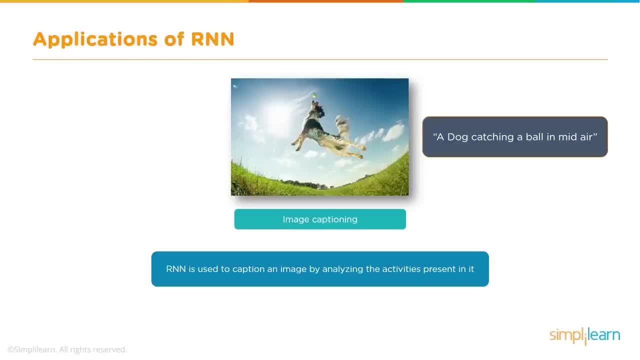 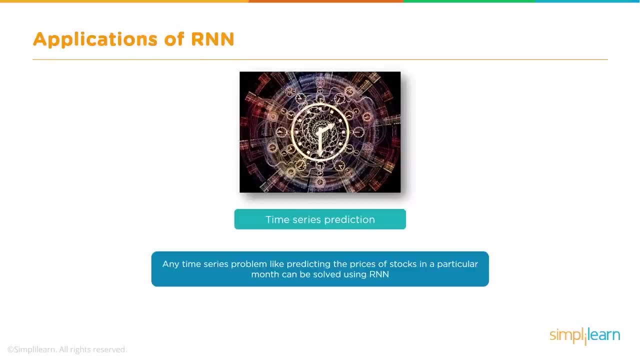 I mean, you know we have a lot of stuff that analyzes images of a dog and the image of a ball, but it's able to add one more feature in there that's actually catching the ball in midair. Time series prediction. Any time series problem? 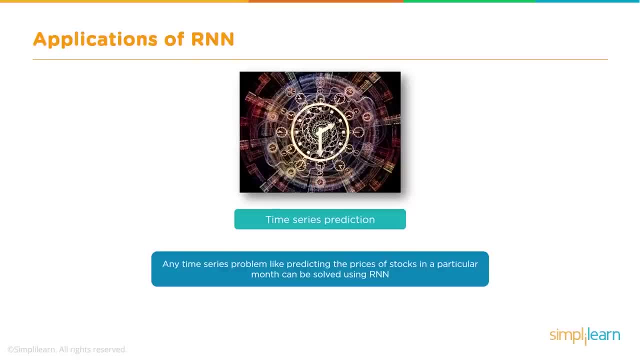 like predicting the prices of stocks in a particular month can be solved using RNN, And we'll dive into that in our use case and actually take a look at some stock. One of the things you should know about analyzing stock today is that if you're analyzing the whole stock the stock market at the New York Stock Exchange in the US produces somewhere in the neighborhood. if you count all the individual trades and fluctuations by the second, it's like three terabytes a day of data. So we're only going to look at one stock. 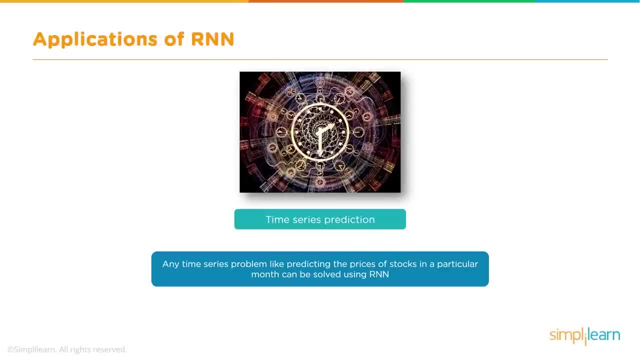 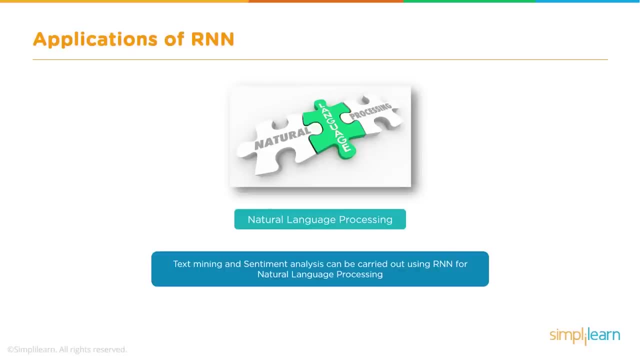 Just analyzing one stock is really tricky In here. we'll give you a little jump on that. so that's exciting, but don't expect to get rich off of it immediately. Another application of the RNN is natural language processing, Text mining and sentiment analysis. 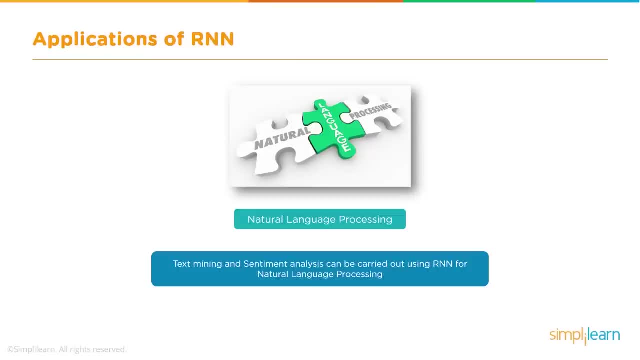 can be carried out by the RNN for natural language processing, And you can see right here the term natural language processing, when you stream those three words together, is very different than if I said processing language naturally. So the time series is very important when we're analyzing. 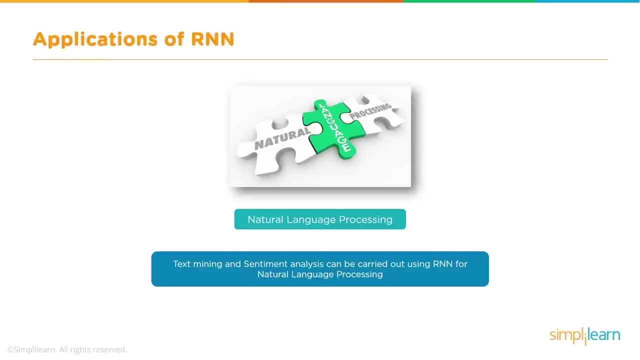 sentiments. It can change the whole value of a sentence just by switching the words around, or if you're just counting the words, you may get one sentiment where, if you actually look at the order they're in, you get a completely different sentiment. When it rains: 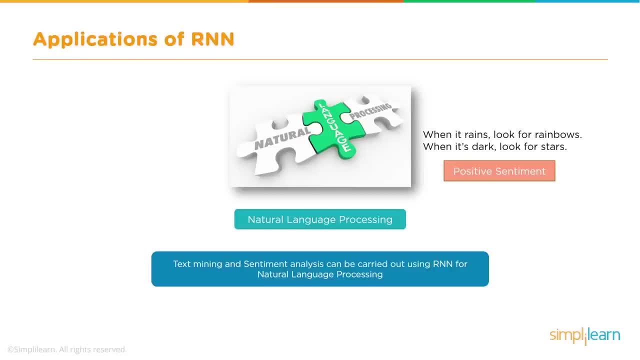 look for rainbows. Most of these are positive sentiments and they're based upon the order of which the sentence is going in Machine translation. given an input in one language, RNN can be used to translate the input into different languages. as output, I myself. 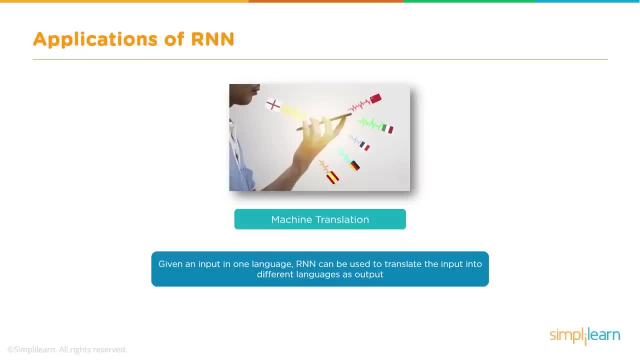 am very linguistically challenged, but if you study languages- and you're good with languages- you know right away that if you're speaking English you would say big cat and if you're speaking Spanish you would say cat big. So that translation is really important. there's all kinds. 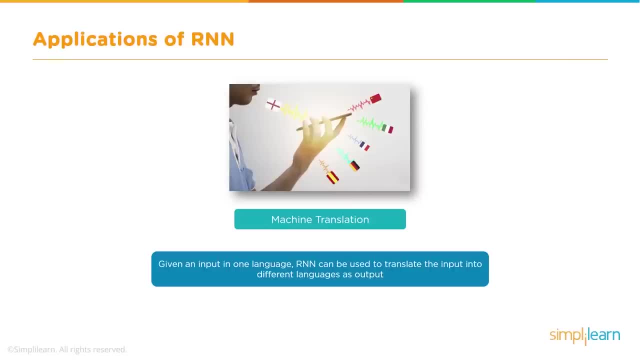 of parts of speech that are important to know by the order of the words. Here this person is speaking in English and getting translated, and you can see here a person is speaking in English in this little diagram. I guess that's denoted by the flags. I have a flag. 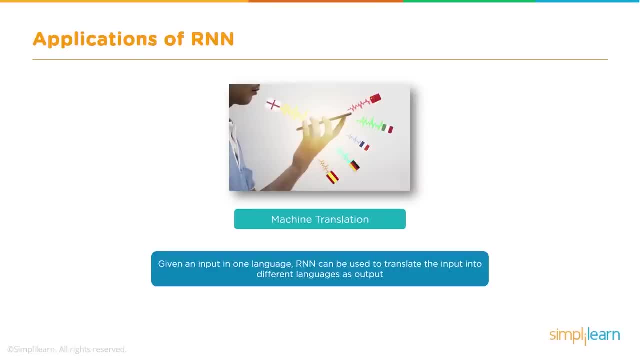 I own it? no, but they're speaking in English and it's getting translated into Chinese, Italian, French, German and Spanish languages. Some of the tools coming out are just so cool, so somebody like myself- I can now travel into worlds I would never think of, because I can have. 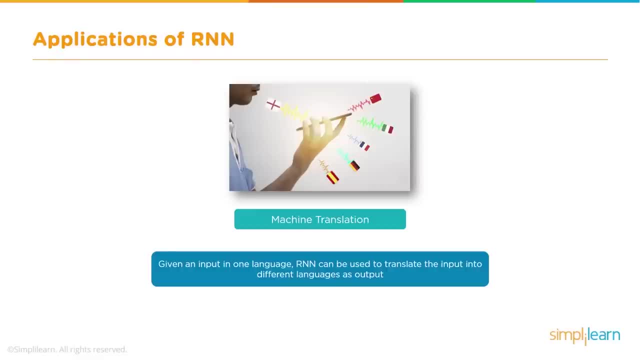 something translate my English back and forth readily and I'm not stuck with a communication gap. So let's dive into what is a recurrent neural network. Recurrent neural network works on the principle of saving the output of a layer and feeding this back to the input. 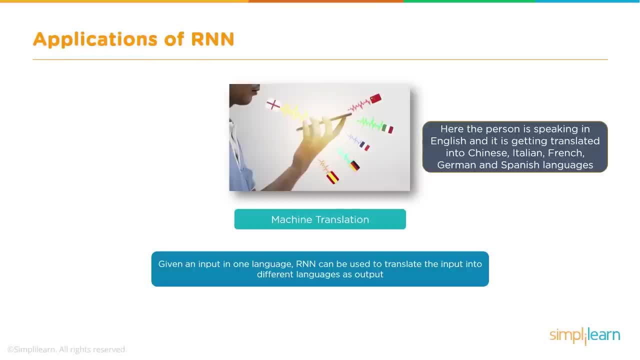 in order to predict the output of the layer Sounds a little confusing. when we start breaking it down it'll make more sense and usually we have a propagation forward neural network with the input layers, the hidden layers and the hidden layers and the hidden layers into Y. 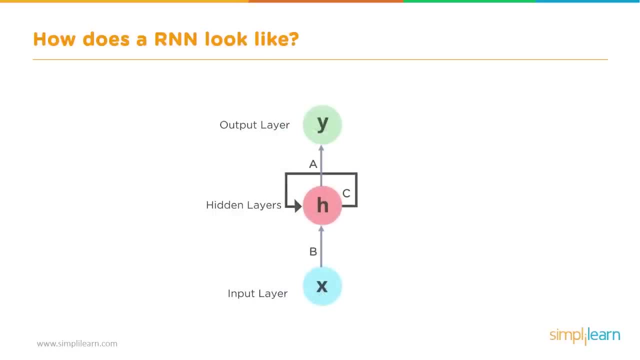 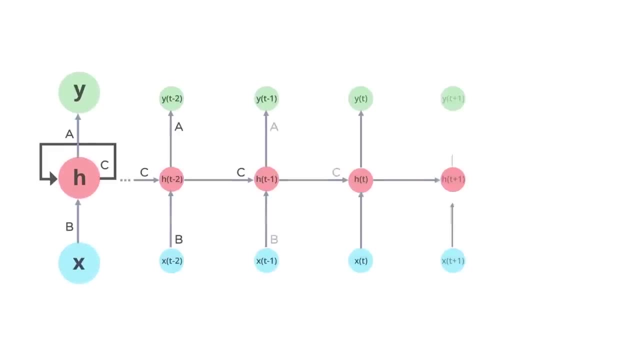 and they usually draw it very simplified: X to H with C as a loop, A to Y, where A, B and C are the perimeters. A lot of times you'll see this kind of drawing in here, digging closer and closer into the H and how it works. 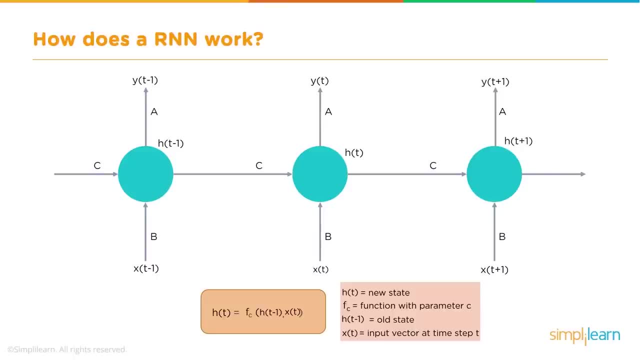 Going from left to right, you'll see that the C goes in and then the X goes in. so the X is going upward bound and C is going, is going out, and C is also going out. That's where it gets a little confusing. So here we have. 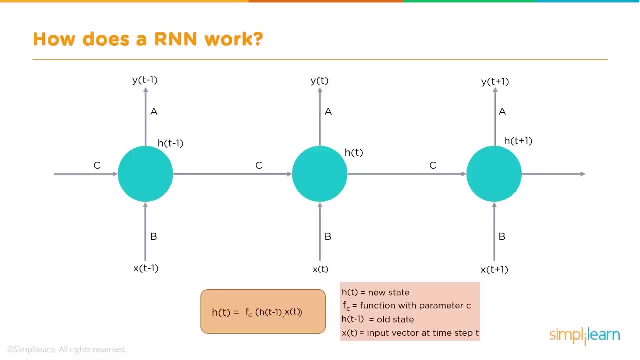 X in, C in, and then we have Y out and C out, And C is based on HT minus one. So our value is based on. the Y and the H value are connected to each other. They're not necessarily the same value, because H can be its own thing And usually we draw this or we represent it as a function H of. 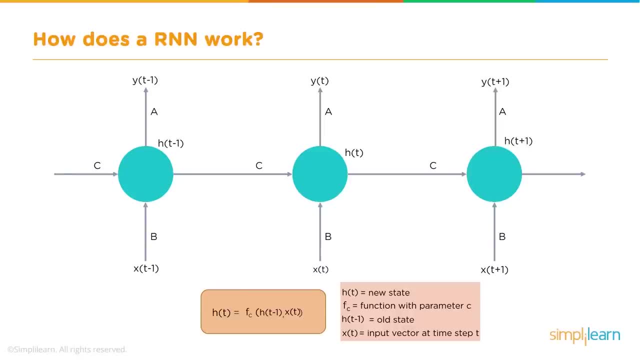 T equals a function of C, where H of T minus one, that's the last H output and X of T going in, So it's the last output of H combined with the new input of X, where HT is the new state, FC is a. 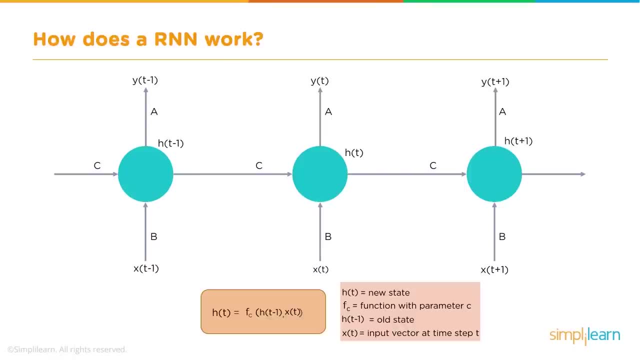 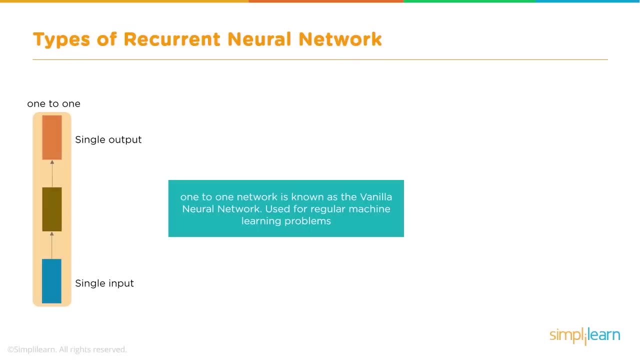 function with the parameter C. That's a common way of denoting it. HT minus one is the old state coming out, And then X of T is an input vector at time of step T. Well, we need to cover types of recurrent neural networks, And so the first one. 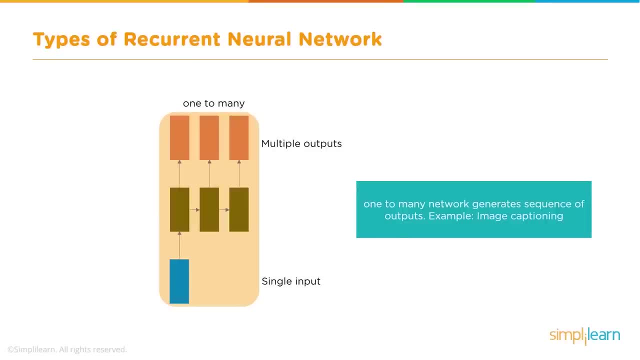 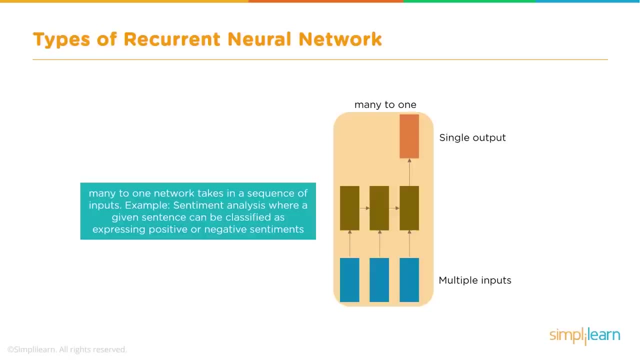 is the recurrent neural networks, And so the first one is the recurrent neural networks is the most common one, which is a one-to-one single output. One-to-one neural network is usually known as a vanilla neural network, used for regular machine learning problems. Why? Because 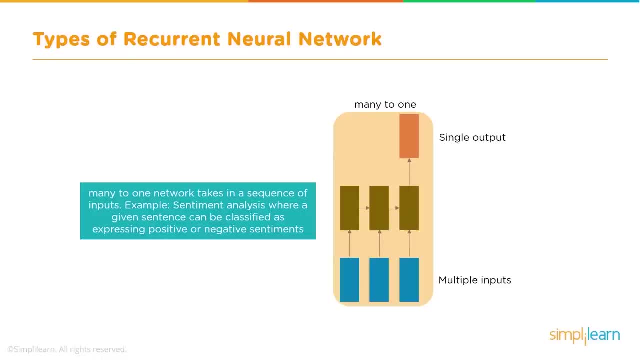 vanilla is usually considered kind of just a real basic flavor. But because it's very basic, a lot of times they'll call it the vanilla neural network, which is not the common term but it is kind of a slang term. People will know what you're talking about usually if you say that. 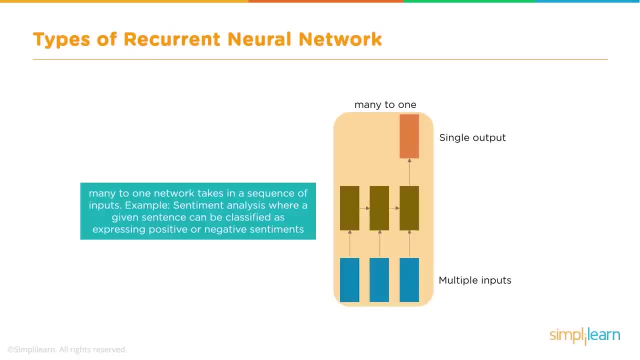 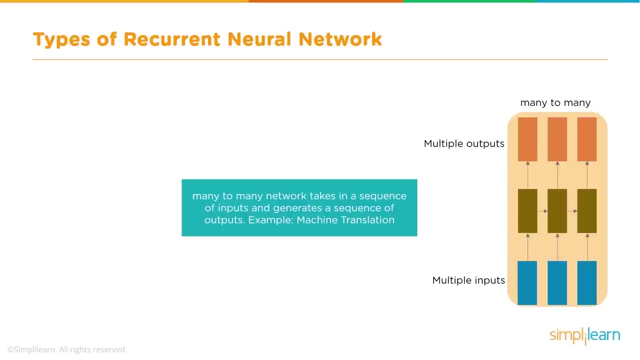 Then we run one-to-many, So you have a single input and you might have multiple outputs- in this case, image captioning, as we looked at earlier, where we have not just looking at it as a dog, but a dog catching a ball in the air- And then you have many-to-one network takes in a sequence of 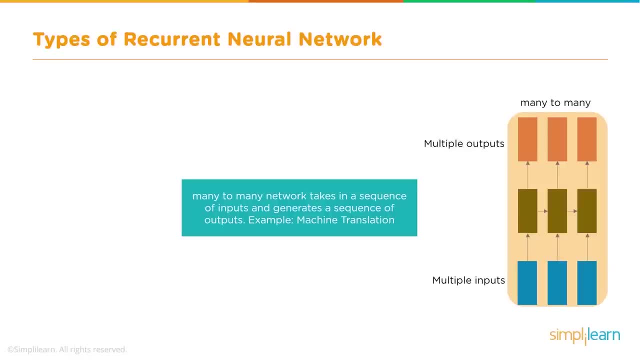 inputs. Examples: sentiment analysis, where a given sentence can be classified as expressing positive or negative sentiments, And we looked at that as we were discussing: if it rains, look for a rainbow, So positive sentiment where rain might be a negative sentiment. 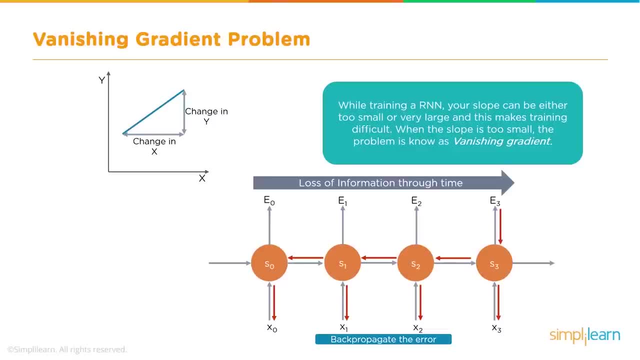 if you're just adding up the words in there, And then, of course, if you're going to do a one-to-one, many-to-one, one-to-many, there's many-to-many networks- takes in a sequence of inputs and generates a sequence of outputs. Example: machine translation. 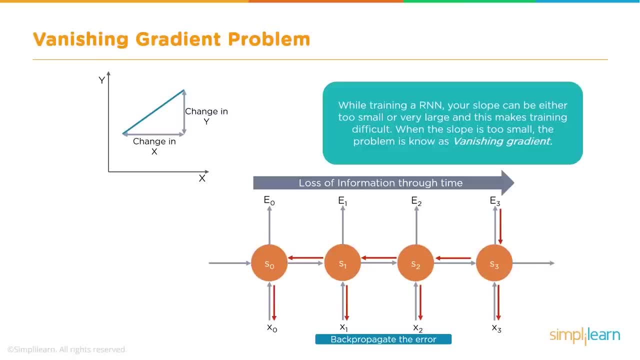 So we have a lengthy sentence coming in in English and then going out in all the different languages. You know just a wonderful tool, Very complicated set of computations. You know, if you're a translator, you realize just how difficult it is to translate into different languages. 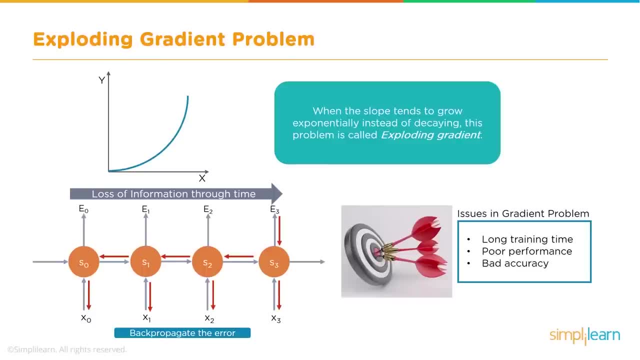 One of the biggest things you need to understand when we're working with this neural network is what's called the vanishing gradient. Well, training an RNN, your slope can be either too small or very large, And this makes training difficult. When the slope is too small, the problem is known as vanishing gradient, And you'll see. 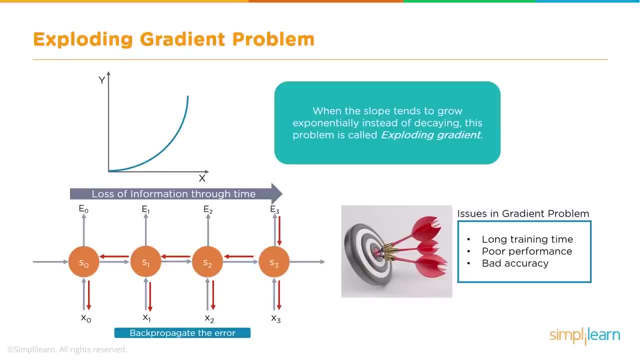 here they have a nice image: loss of information through time. So if you're pushing not enough information forward, that information is lost, And then when you go to train it you start losing the third word in the sentence or something like that, or it doesn't quite follow the full logic. 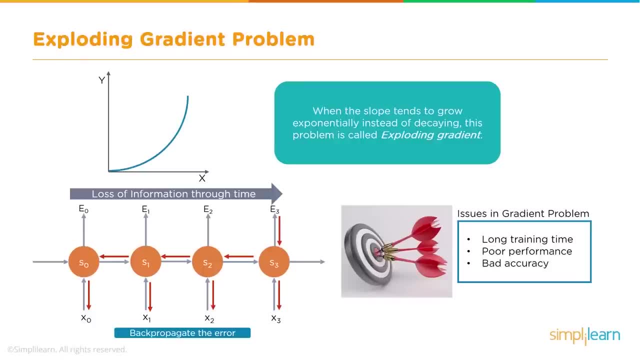 of what you're working on. Exploding gradient problem. Oh, this is one that runs into everybody. When you're working with this particular neural network, when the slope tends to grow exponentially instead of decaying, this problem is called exploding gradient. Issues in gradient problem: long training time, poor. 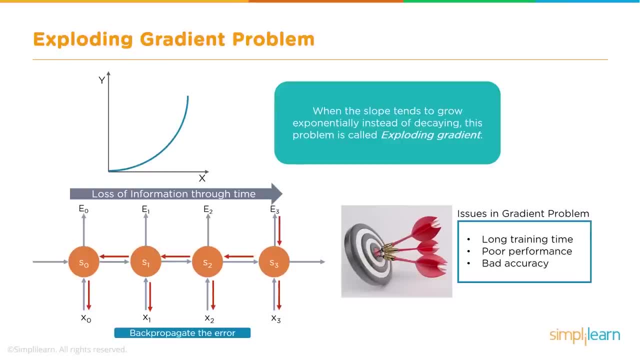 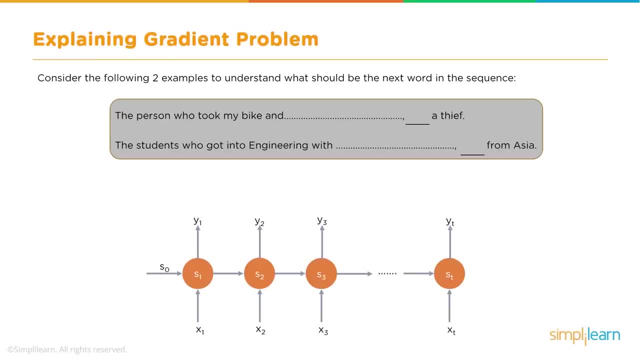 performance, bad accuracy. And I'll add one more in there: Your computer. if you're on a lower end computer testing out a model, will lock up and give you the memory error: Exploding gradient problem. Consider the following two examples to understand what should be the next step in your 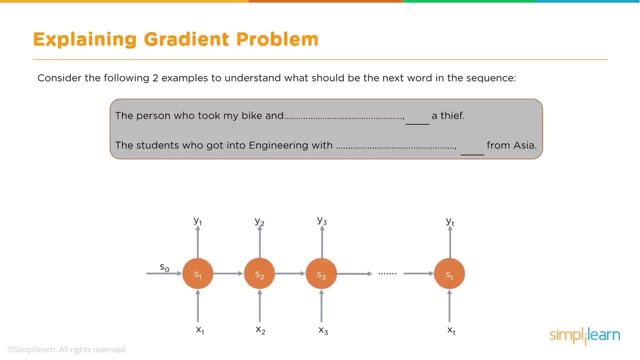 social engineering study. if your data can develop better, You can look up near zero matching cases of the results. лом 89 00 01 01 01 01 01 09 10. 11 0 01 20 01 20. 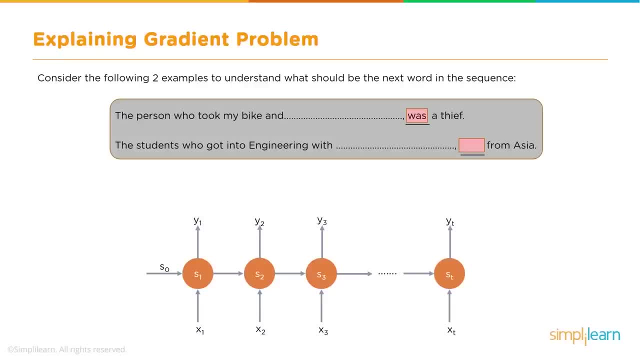 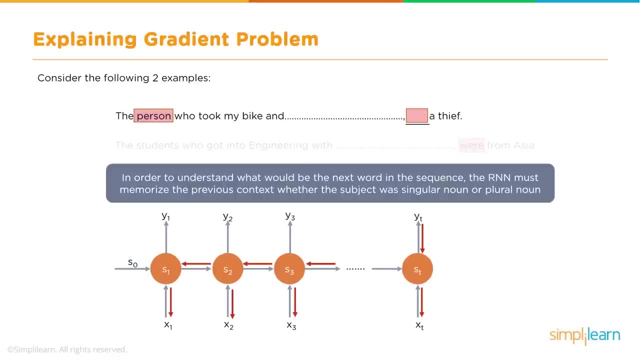 01 22 01 23 024 025 026. person who took the bike- so we'll go back to the person who took the bike- was blank a thief. In order to understand what would be the next word in the sequence, the RNN must memorize the previous context, whether the subject was: 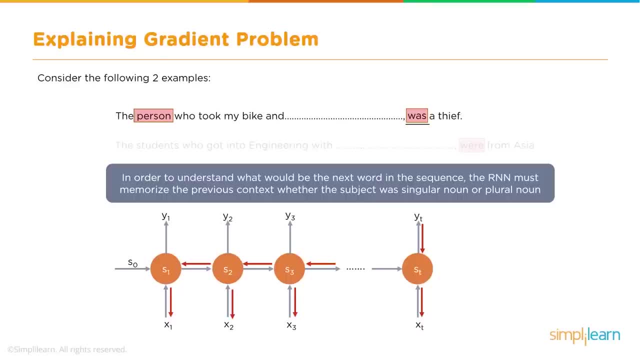 singular noun or a plural noun. So was a thief is singular. The student who got into engineering. well, in order to understand what would be the next word in the sequence, the RNN must memorize the previous context, whether the subject was singular noun or a plural noun. And so you can see here the students who got 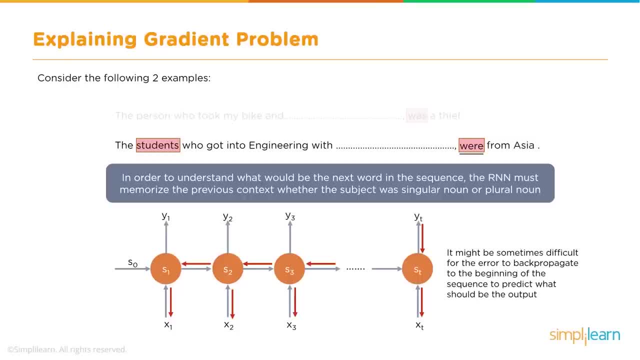 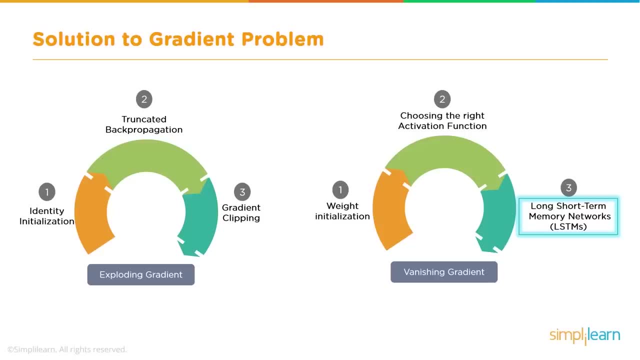 into engineering with blank were from Asia. It might be sometimes difficult for the error to back, propagate to the beginning of the sequence, to predict what should be the output. So when you run into the gradient problem, we need a solution, The solution to the gradient problem. First we're going to look at 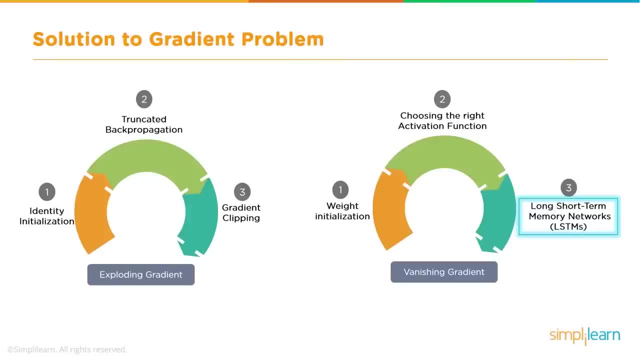 exploding gradient where we have three different solutions, depending on what's going on. One is identity initialization. So the first thing we want to do is see if we can find a way to minimize the identities coming in instead of having it identify everything. just the important information we're looking at. 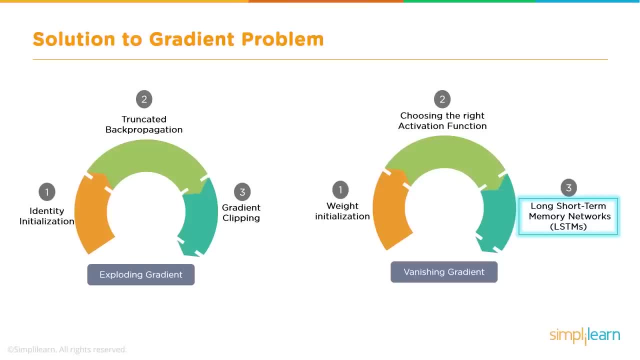 Next is to truncate the back propagation. So instead of having whatever information it's sending to the next series, we can truncate what it's sending. We can lower that particular set of layers, make those smaller. And finally, is a gradient clipping, So when we're training it, we can clip what that gradient looks like. 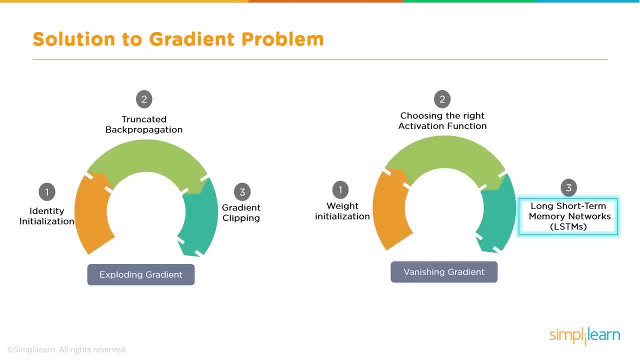 and narrow the training model that we're using. When you have a vanishing gradient- the option problem- we can take a look at weight initialization: Very similar to the identity, but we're going to add more weights in there so it can identify different aspects of what's coming in better, Choosing the right. 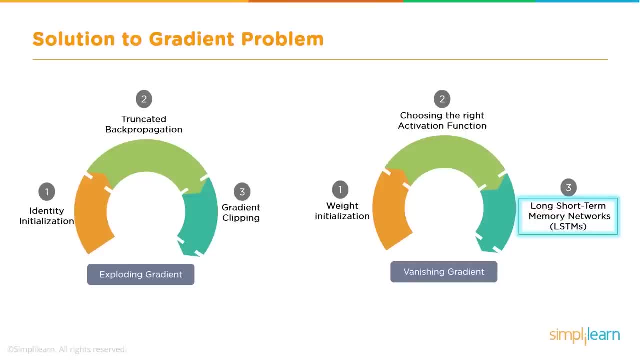 activation function. That's huge. So we might be activating based on one thing and we need to limit that. We haven't talked too much about activation functions, so we'll look at that just minimally. There's a lot of choices out there And then 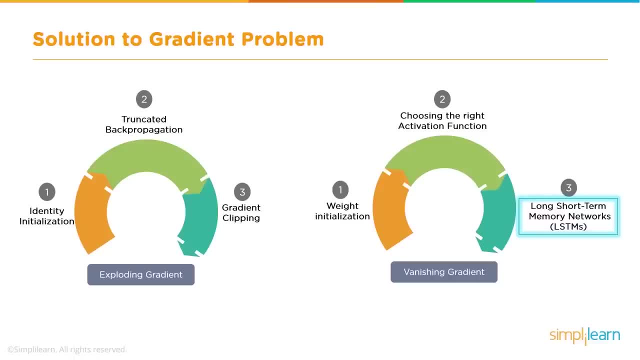 finally, there's long short-term memory networks, the LSTMS. We can make adjustments to that. So just like we can clip the gradient as it comes out, we can also expand on that. We can increase the memory network, the size of it, so it handles more information. And one of the most common 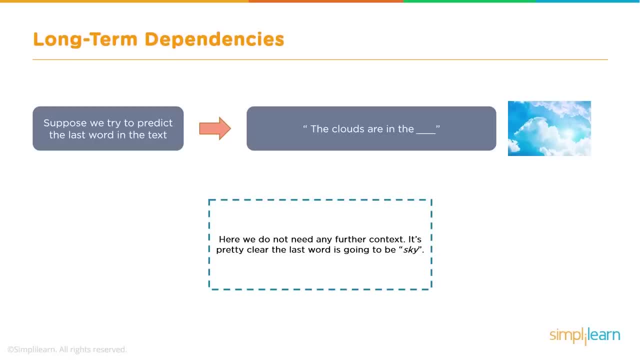 problems in today's setup is what they call long-term dependencies. Suppose we try to predict the last word of the text. The clouds are in the- and you probably said- sky Here. we do not need any further context. It's pretty clear that the last 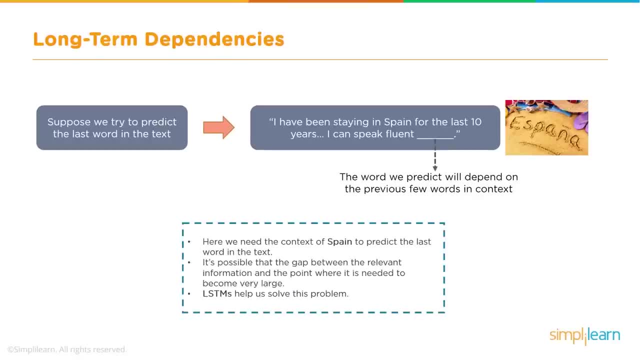 word is going to be sky, Suppose we try to predict the last word in the text. I have been staying in Spain for the last 10 years. I can speak fluent. Maybe you said Portuguese or French. No, you probably said Spanish. The word we predict will depend on the previous few words in. 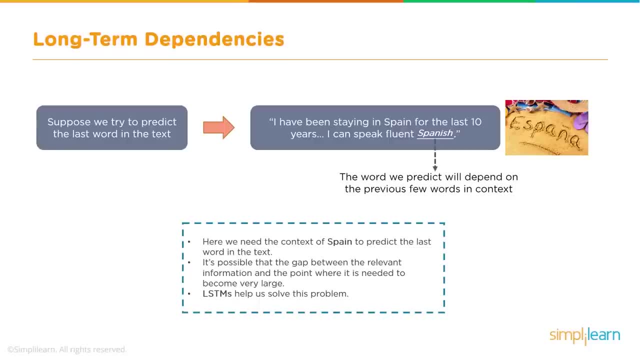 context. Here we need the context of Spain to predict the last word in the text. It's possible that the gap between the relevant information and the point where it is needed to become very large LSTMs help us solve this problem. So the 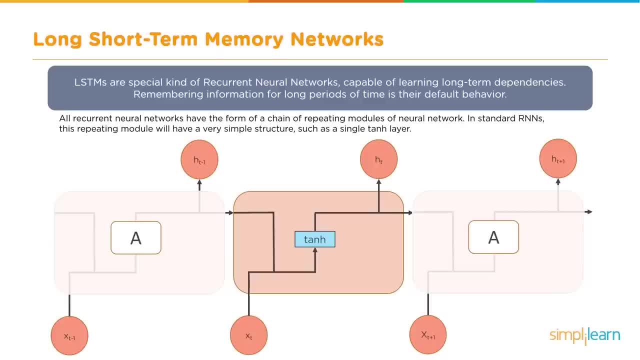 LSTMS are a special kind of recurrent neural network capable of learning long-term dependencies. Remembering information for long periods of time is their default behavior. All recurrent neural networks have the form of a chain of repeating modules of neural network connections. In standard RNNs, this repeating module will have a very simple structure, such as a single. 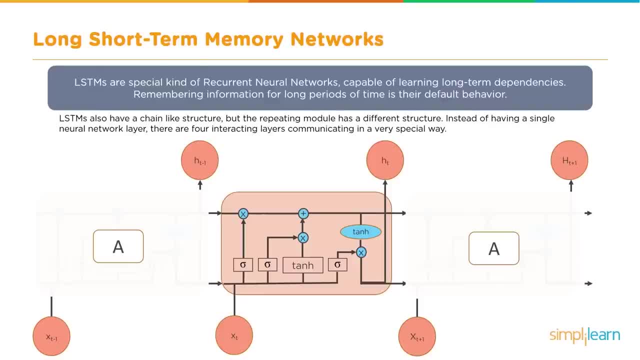 tangent H layer. LSTMSs also have a chain-like structure, but the repeating module has a different structure. Instead of having a single neural network layer, there are four interacting layers communicating in a very special way. LSTMSs are a special kind of recurrent neural network capable of learning long-term dependencies. Remembering information for long periods of time is their default behavior. 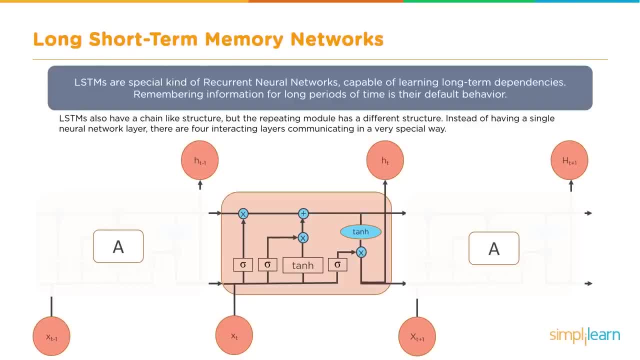 LSTMSs also have a chain-like structure, but the repeating module has a different structure. Instead of having a single neural network layer, there are four interacting layers communicating in a very special way. As you can see, the deeper we dig into this, the more complicated the graphs get In here. I want you to note that you have X at T minus one coming in. You have a. very complex structure and you have an extra layer in there to be able to connect with. However, we're going to use some things from this structure that I've already described. The thing that you have to remember is that these structures are separate. If we use a chain like structure, we're going to have two forms of the same chain. 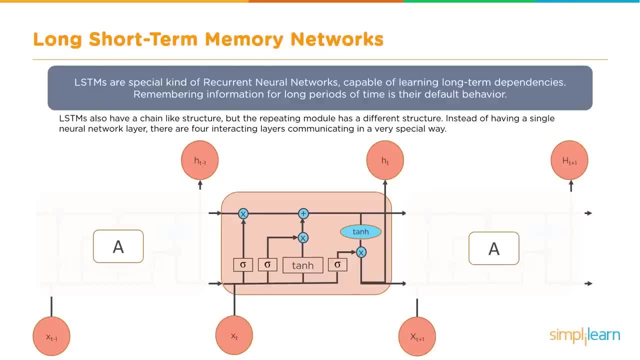 graphs kit In here. I want you to note that you have x of t minus 1 coming in, you have x of t coming in and you have x of t plus 1, and you have h of t minus 1, and h of t coming in and h of t. 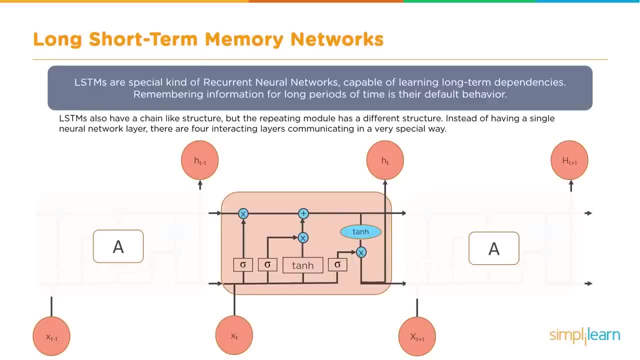 plus 1 going out, and of course on the other side is the output a. In the middle we have our tangent h, but it occurs in two different places, So not only when we're computing. the x of t plus 1 are. 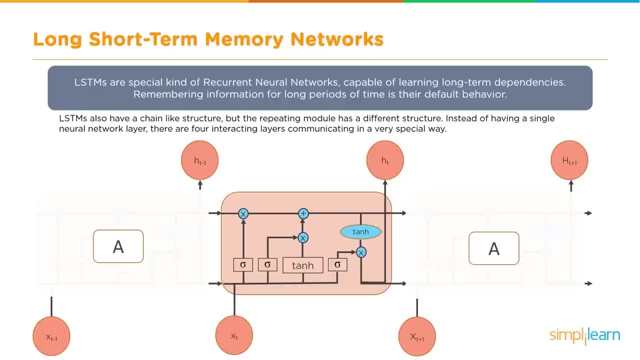 we getting the tangent h from x of t, but we're also getting that value coming in from the x of t minus 1.. So the short of it is: as you look at these layers, not only does the propagate through the first layer goes into the second layer, back into itself, but it's also going into the third. 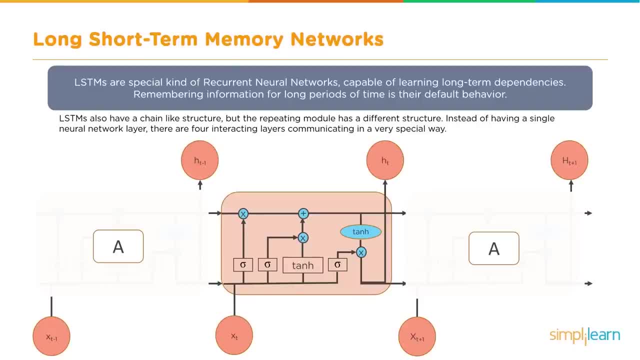 layer. So now we're kind of stacking those up and this can get very complicated. as you grow that in size, It also grows in memory too and in the amount of resources it takes. But it's a very powerful tool to help us address. 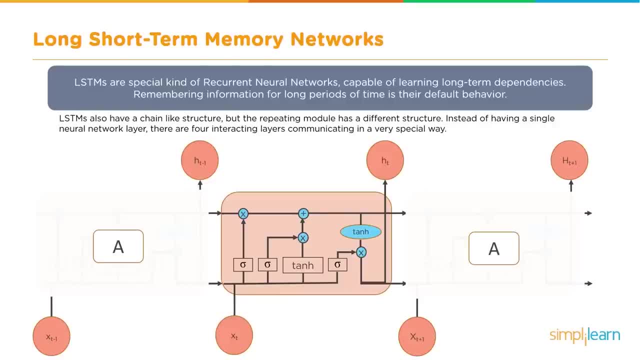 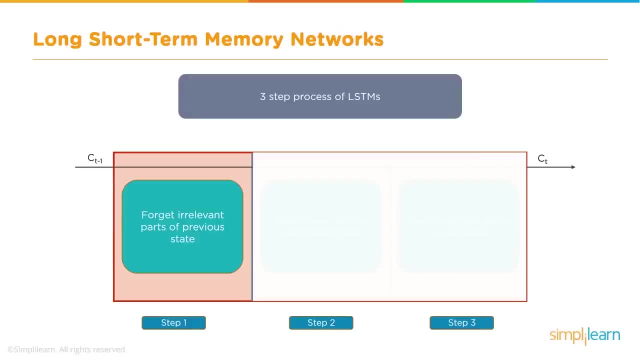 the problem of complicated, long sequential information coming in, like we were just looking at in the sentence And when we're looking at our long short term memory network. there's three steps of processing in the LSTMS that we look at. The first one is: we want to forget irrelevant. 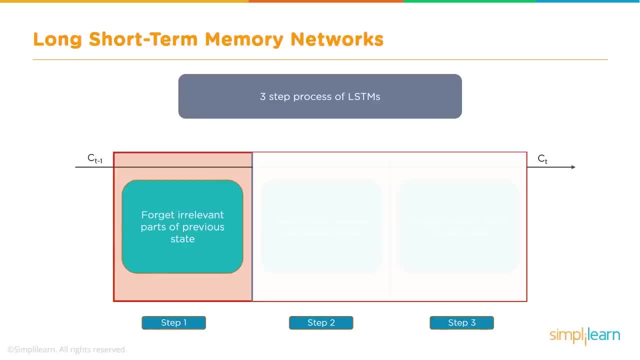 parts of the previous state. You know, a lot of times, like you know, is as in a, unless we're trying to look at whether it's a plural noun or not, they don't really play a huge part in the. 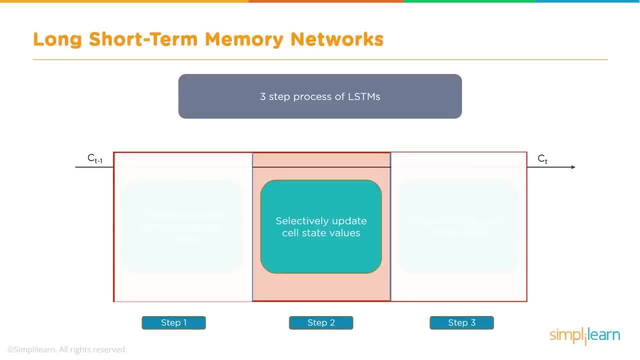 language, so we want to get rid of them. Then selectively update. selectively update the cell state values, So we only want to update the cell state values that reflect what we're working on. And finally, we want to only output certain parts of the cell state. 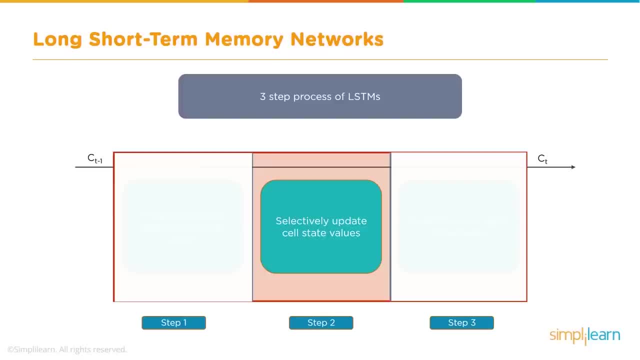 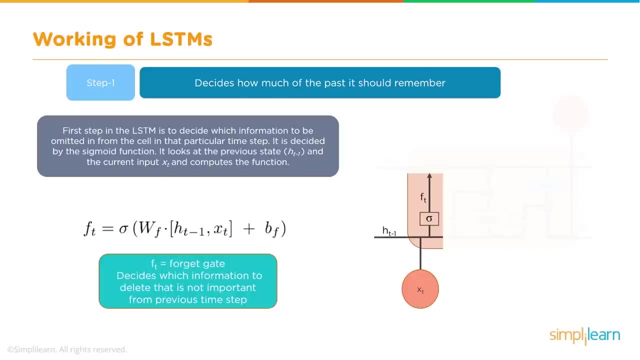 So, whatever is coming out, we want to limit what's going out too. So let's dig a little deeper into this. Let's just see what this really looks like. So step one decides how much of the past it should remember. First step in the LSTM is to decide which information to 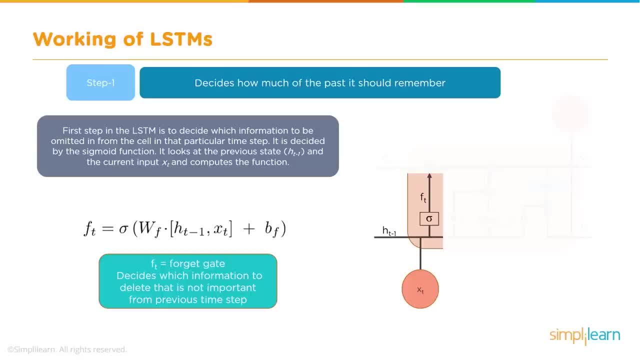 be omitted in from the cell in that particular time step. It is decided by the sigmoid function. It looks at the previous state, h at t minus 1, and the current input, x at t, and computes the function. So you can see over here we have a function of t equals the sigmoid function of the. 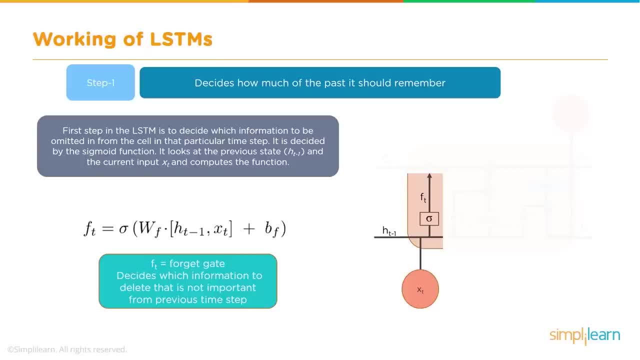 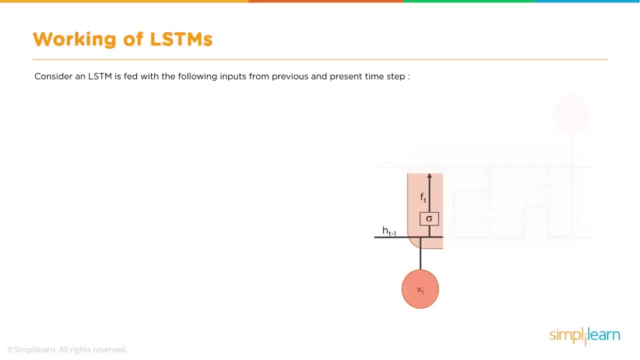 weight of f, the h at t minus 1 and then x at t plus. of course you have a bias in there with any of our neural networks, so we have a bias function. So f of t equals forget gate decides which information to delete. that is not important. from the previous time step, Considering an. 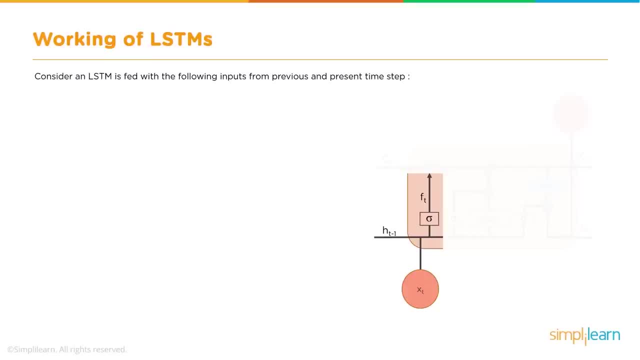 STM is fed with the following inputs from the previous and present time. step: Alice is good in physics. John, on the other hand, is good in chemistry. So previous output: John plays football. well, He told me yesterday over the phone that he had served as a captain of his college football. 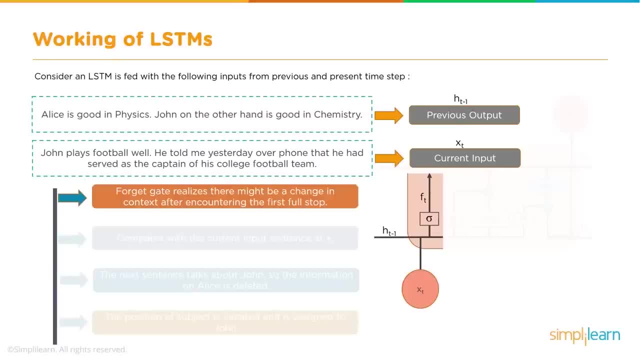 team. That's our current input. So, as we look at this, the first step is the forget gate realizes there might be a change in context after encountering the first full stop. Compares with the current input sentence of x at t. So we're looking at the. 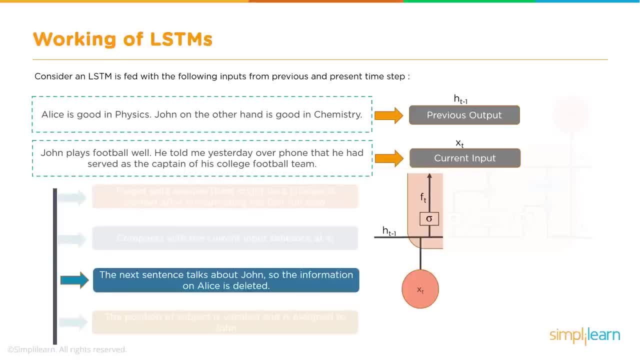 full stop and then compares it with the input of the new sentence. The next sentence talks about John, so the information on Alice is deleted. Okay, that's important to know. So we have this input coming in and if we're going to continue on with John, then that's going to be the primary. 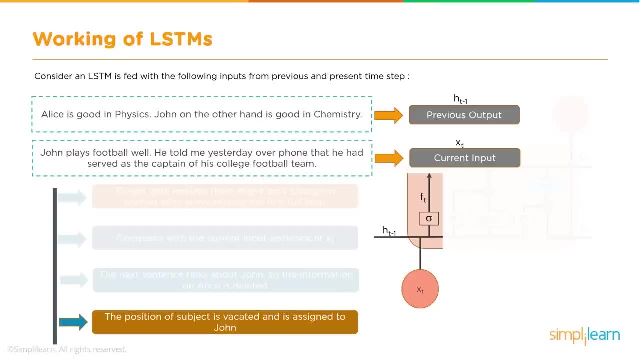 information we're looking at, The position of the subject is vacated and is assigned to John, And so in this one we've seen that we've weeded out a whole bunch of information and we're only passing information on John, since that's now the new topic. So step two is then to decide how much. 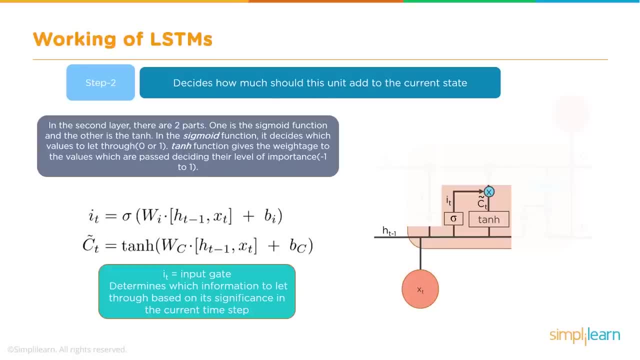 this unit add to the current state. In the second layer there are two parts. One is the sigmoid function and the other is the tangent h. In the sigmoid function it decides which values to let through, zero or one. Tangent h function gives the weightage to the values which are passed. 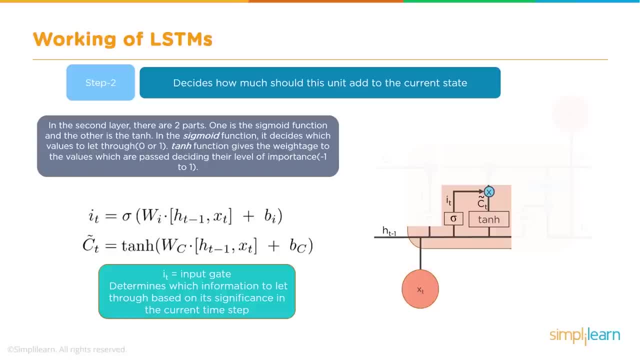 deciding their level of importance. minus one to one, And you can see the two formulators that come up. the i of t equals the sigmoid of the weight of i, a to t minus one x of t plus the bias of i, And tangent of h of the weight of c, of h of t minus one x of t plus the bias of c. So our i of t equals. 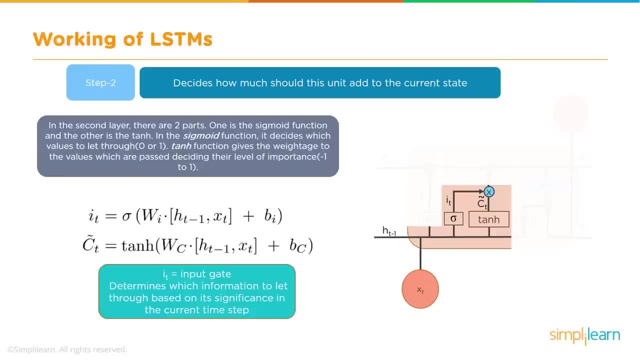 the input gate determines which information to let through, based on its significance in the current time step. If this seems a little complicated, don't worry, because a lot of the programming is already done when we get to the case study. Understanding, though, that this is part of the 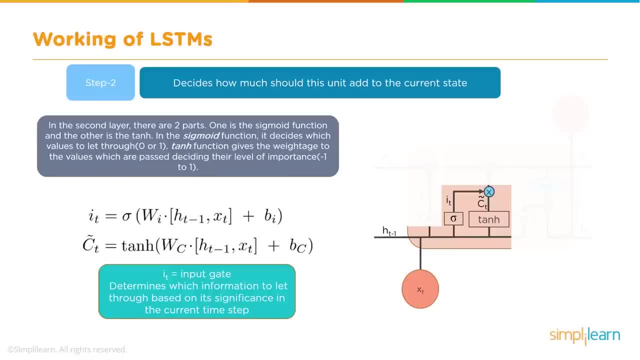 program is important when you're trying to figure out these, what to set your settings at. You should also note when you're looking at this. it should have some semblance to your forward propagation neural network, Where we have a value assigned to a weight plus a bias- Very important steps than any of the 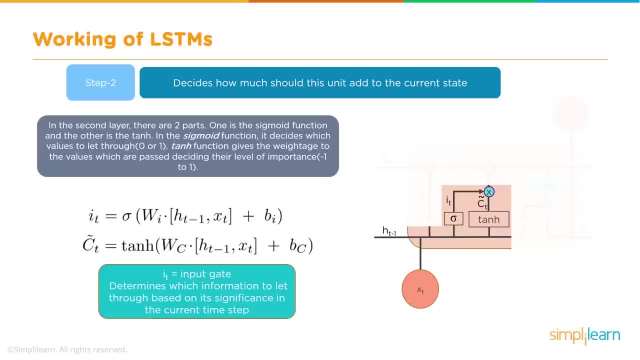 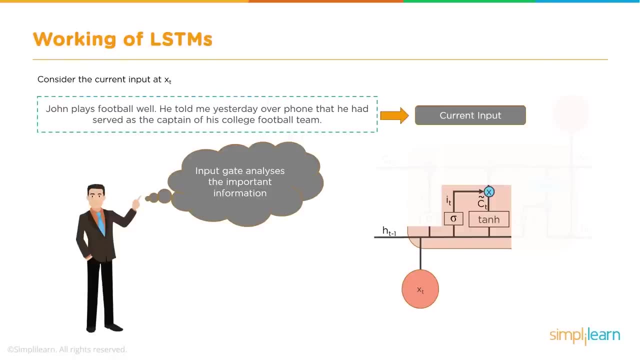 neural network layers, Whether we're propagating into them the information from one to the next or we're just doing a straightforward neural network propagation. Let's take a quick look at this, what it looks like from the human standpoint. as I step out of my suit again. Consider the current input. 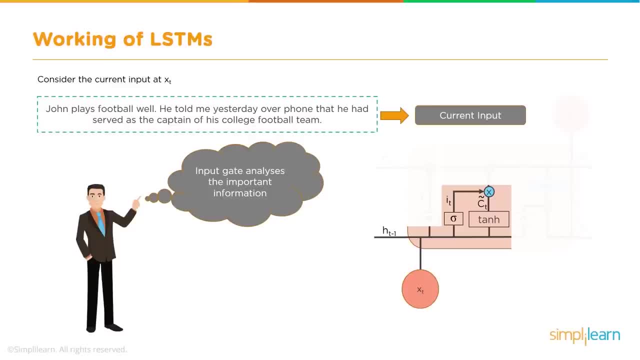 at x of t. John plays football. well, He told me yesterday over the phone that he had served as a captain of his college football team. He said that he was a captain of his college football team. That's our input. Input gate analysis, the important information: John plays football and he was a. 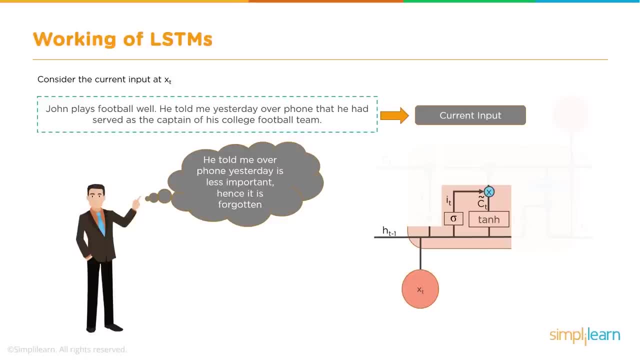 captain of his college team is important, He told me over the phone yesterday- is less important, Hence it is forgotten. This process of adding some new information can be done via the input gate. Now, this example is as a human form- and we'll look at training this stuff in just a minute- But as a 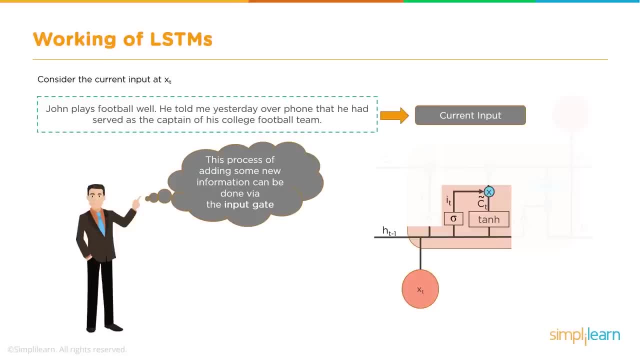 human being. if I wanted to get this information from a conversation- Maybe it's a google voice listening in on you or something like that- How do we weed out the information that he was talking to me on the phone yesterday? Well, I don't want to memorize that he talked to me on the phone yesterday, Or maybe that is important, But in this, 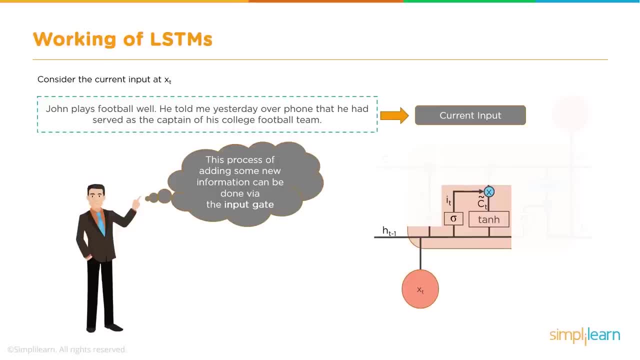 case it's not. I want to know that he was the captain of the football team. I want to know that he served. I want to know that John plays football and he was a captain of the college football team. Those are the two things that I want to take away as a human being- Again, we measure a lot of this. 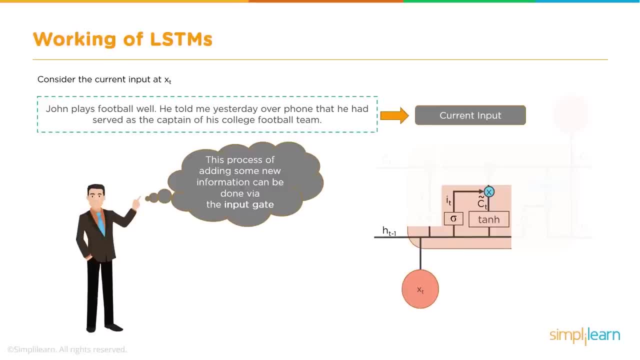 from the human viewpoint and that's also how we try to train them So we can understand these neural networks. Finally, we get to step three: Decides what part of the brain is the most important part of the human viewpoint. Finally, we get to step three: Decides what part of the brain is the most important part of the human viewpoint. 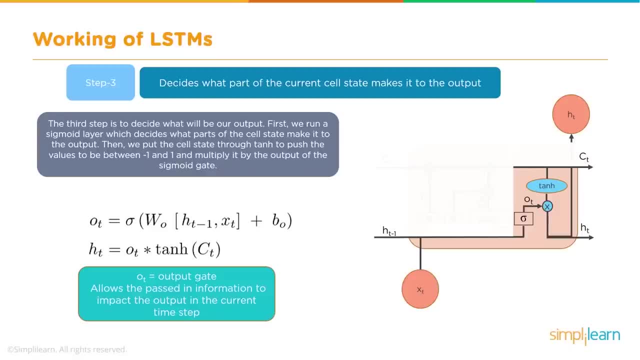 Finally we get to step three, Decides what part of the brain is the most important part of the human viewpoint. The third step is to decide what will be our output. First we run a sigmoid layer which decides what parts of the cell state make it to the output. Then we put the cell state through. 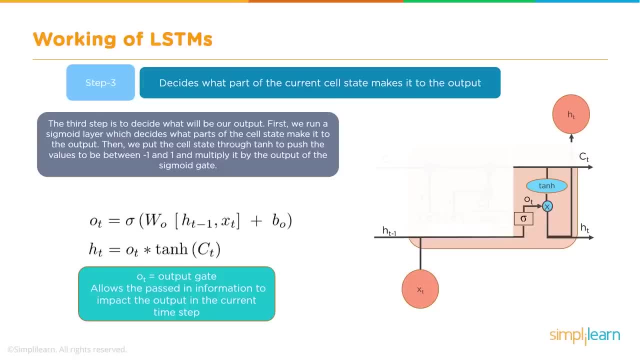 the tangent h to push the values to be between minus one and one and multiply it by the output of the sigmoid gate. So when we talk about the output of t, we set that equal to the sigmoid of the weight of zero, of the h of t minus one and back one step in time by the. 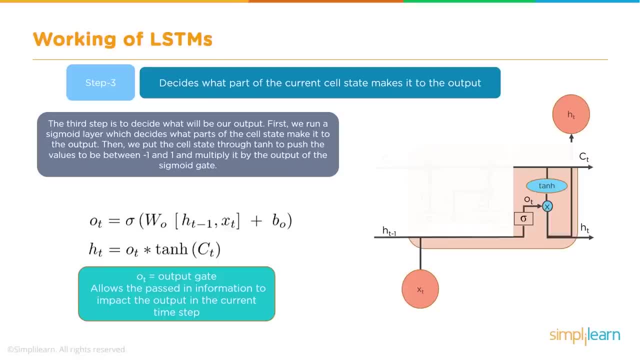 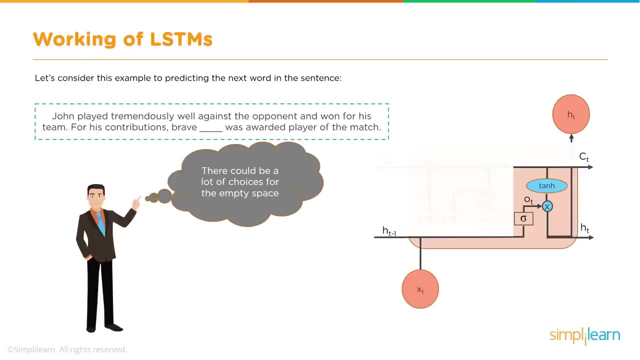 x of t plus, of course, the bias. the h of t equals the out of t times the tangent of the tangent h of c of t. So our o of t equals the output gate allows the passed in information to impact the output in the current time step. Let's consider the example to predicting the next word in the sentence. 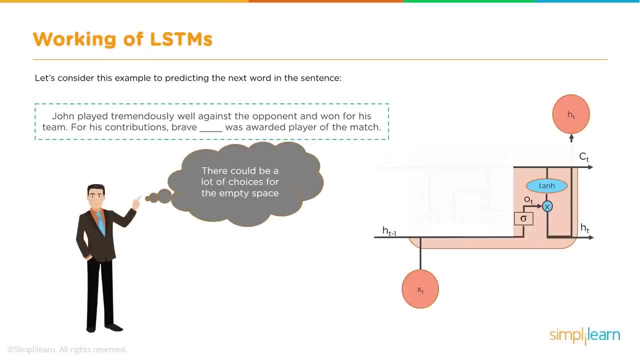 John played tremendously well against the opponent and won for his team. For his contributions, brave blank was awarded player of the match. There could be a lot of choices for the empty space. Current input: brave is an adjective. Adjectives describe a noun. John could be the best output. 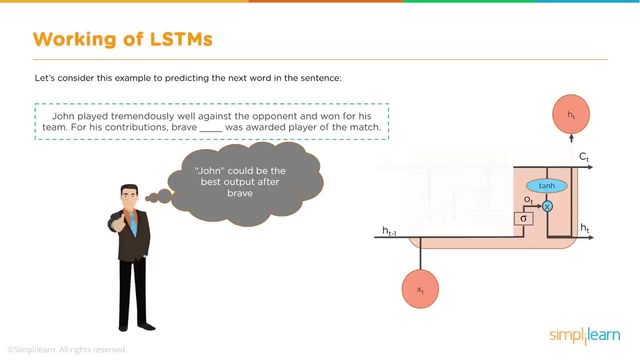 after brave Thumbs up for John, awarded player of the match. and if you were to pull just the nouns out of the sentence team doesn't look right because that's not really the subject. we're talking about Contributions. you know, brave contributions or brave team, brave player, brave match, So you look. 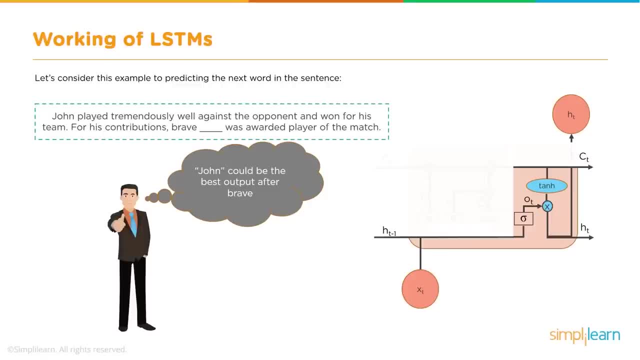 at this and you can start to train this, these, this neural network. so it starts looking at it and goes, oh no, John, is what we're talking about. So, if you look at this and you can start to train this, this neural network, so it starts looking at it and goes: oh no, John, is what we're talking about. 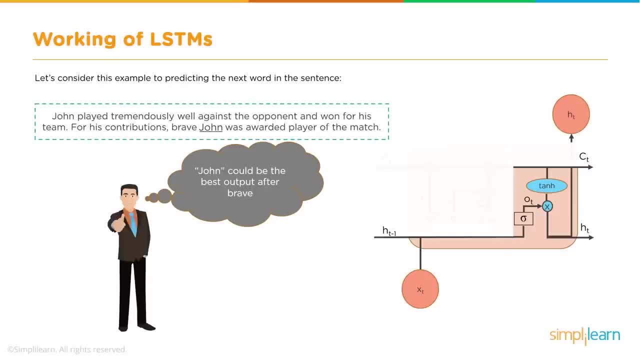 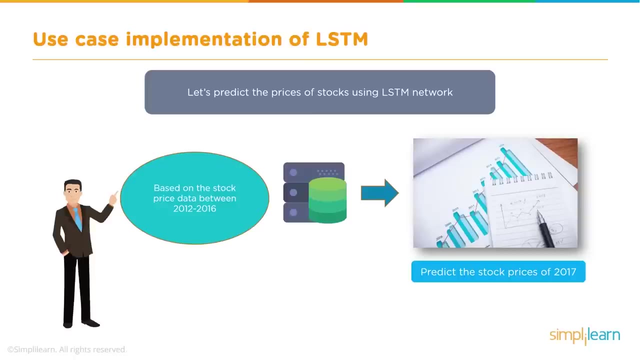 So brave is an adjective, John's going to be the best output and we give John a big thumbs up. And then, of course, we jump into my favorite part, the case study. Use case implementation of LSTM. Let's predict the prices of stocks using the LSTM network based on the stock price data between 2012. 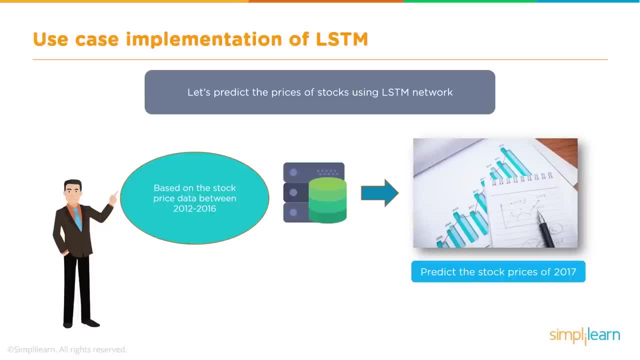 2016.. We're going to try to predict the stock prices of 2017, and this will be a narrow set of data. We're not going to do the whole stock market either. We're going to try to predict the stock prices of 2017, and this will be a narrow set of data. we're not going to do the whole stock market either. 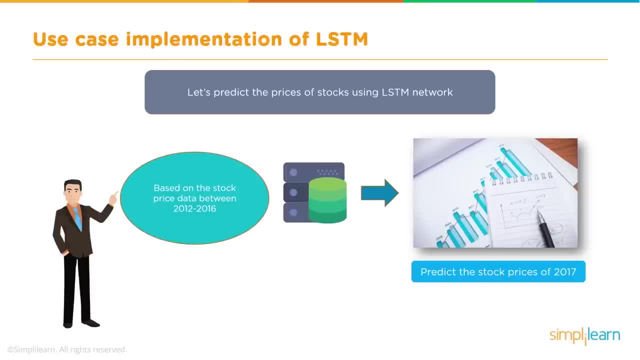 turns out that the new york stock exchange generates roughly three terabytes of data per day. that's all the different trades up and down of all the different stocks going on, and each individual one second to second or nanosecond to nanosecond. but we're going to. 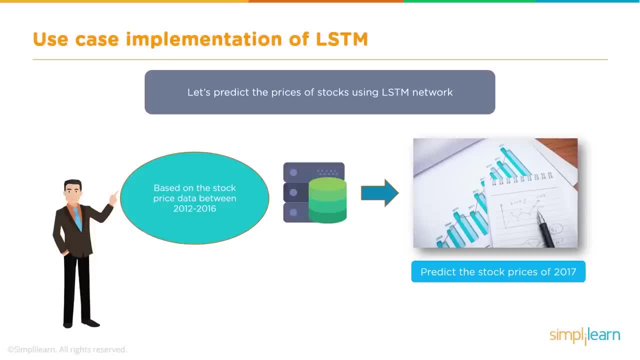 limit that to just some very basic, fundamental information. so don't think you're going to get rich off this today, but at least you can give an odd. you can give a step forward in how to start processing something like stock prices- a very valid use for machine learning in today's 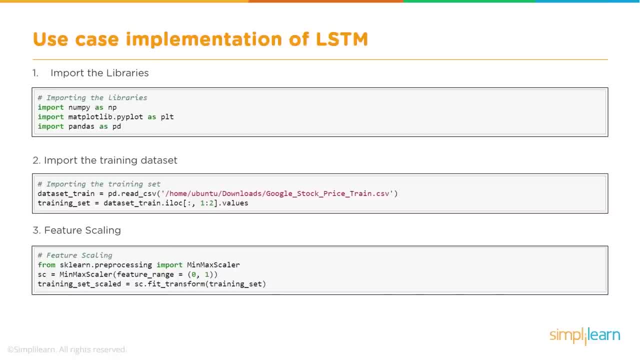 markets. use case: implementation of lstm. let's dive in. we're going to import our libraries. we're going to import the training set and get the scaling going now. if you watch any of our other tutorials, a lot of these pieces should start to look very familiar, because it's very similar. 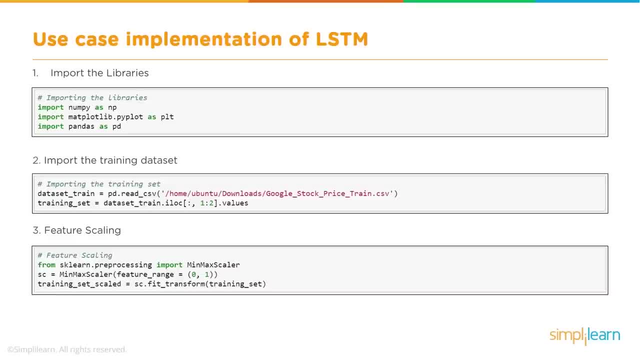 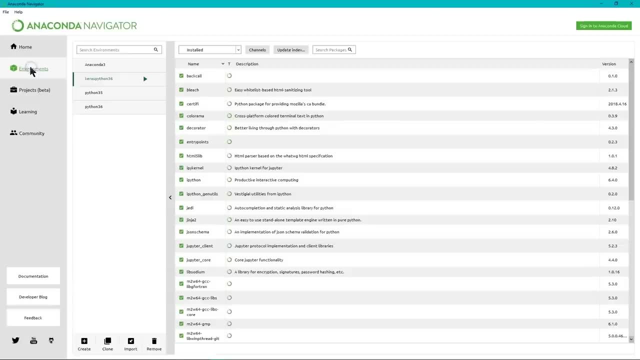 setup. but let's take a look at that. and just a reminder, we're going to be using anaconda, the jupiter notebook. so here i have my anaconda navigator when we go under environments. i've actually set up a cross. python 3- 6. i'm in python 3- 6 and, uh, nice thing about anaconda, especially the. 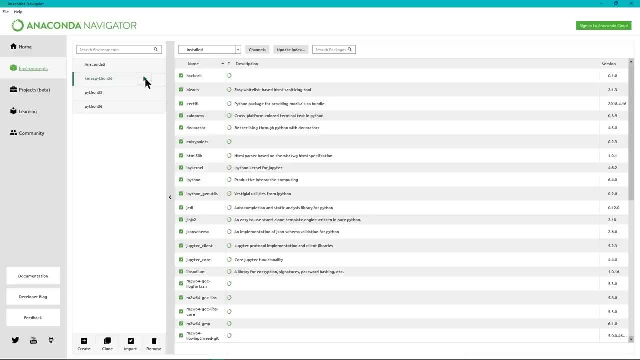 newer version. remember a year ago messing with anaconda- different versions of python in different environments. anaconda now has a nice interface and i have this installed both on a ubuntu linux machine and on windows so it works fine on there. you can go in here and open a terminal window. 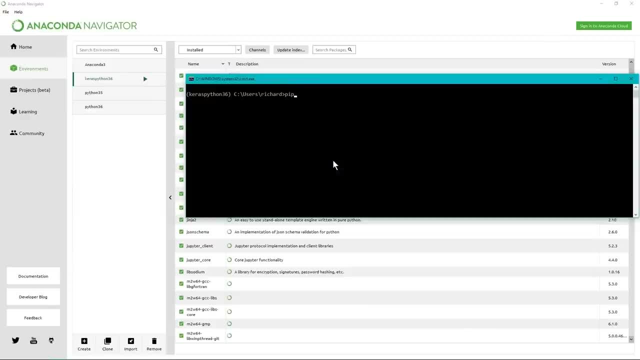 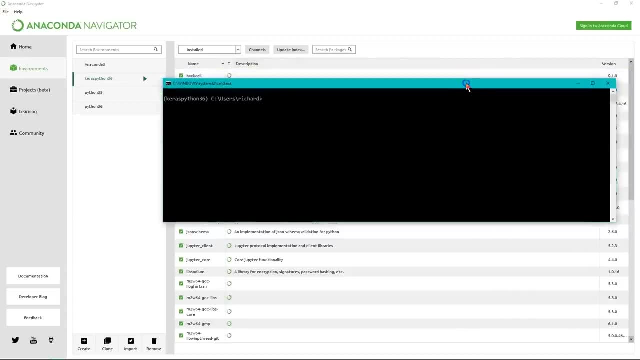 and then in here, once you're in the terminal window. this is where you're going to start installing, using pip to install your different modules and everything. now we've already pre-installed them, so we don't need to do that in here, but if you don't have them installed in your particular environment, you'll need to do that. 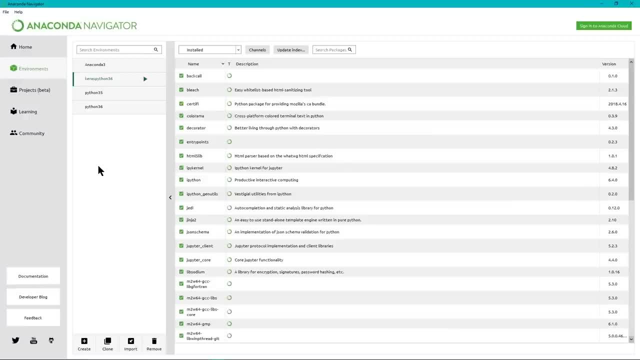 and of course you don't need to use the anaconda or the jupiter, you can use whatever favorite python ide you like. i'm just a big fan of this because it keeps all my stuff separate. you can see, on this machine i have specifically installed one for karas, since we're going to be working with karas. 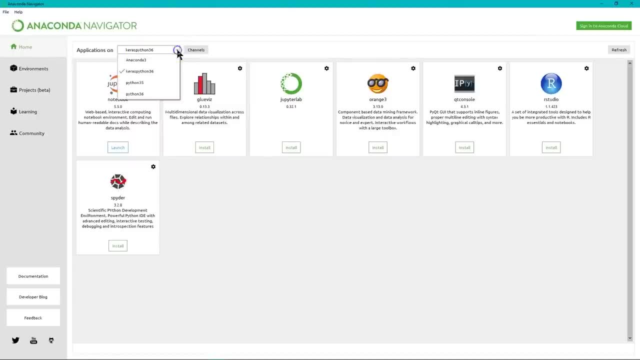 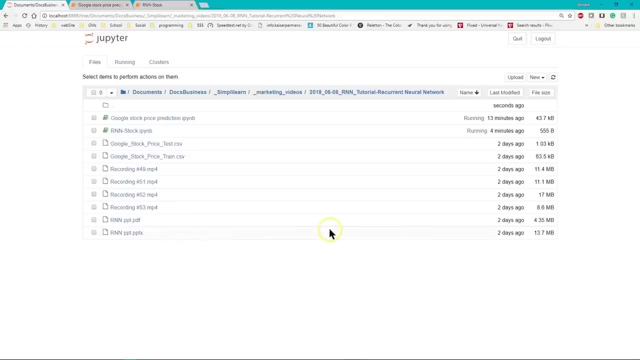 under tensorflow, we go back to home. i've gone up here to application and that's the environment i've got here, and then we'll click on the launch. jupiter notebook: now i've already in my jupiter notebook um have set up a lot of stuff so that we're ready to go kind of like martha stewart's. 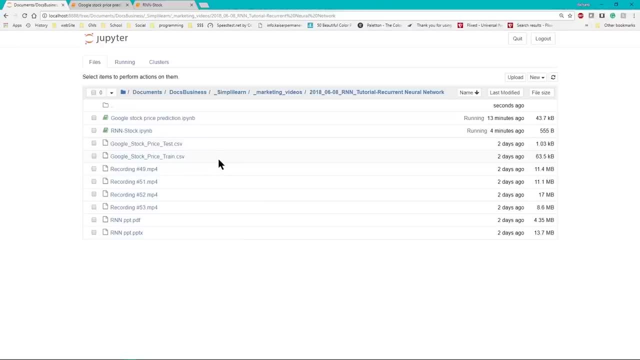 in the old cooking shows. we want to make sure we have all our tools for you so you're not waiting for them to load. and if we go up here to where it says new, you can see where you can create a new python3. that's what we did here underneath the setup, so it already has all the modules. 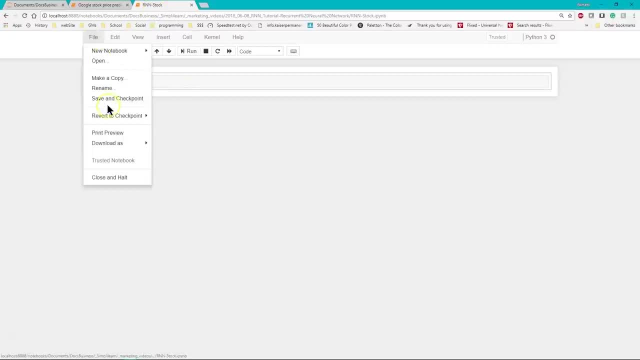 installed on it and i'm actually renamed this. if you go under file, you can rename it. we've i'm rnn stock and let's just take a look and start diving into the code. let's get into the exciting part now. we've looked at the tool and, of course, you might be using a different tool, which is fine. 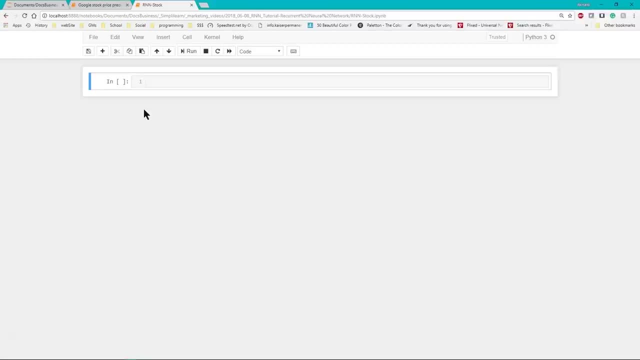 let's start putting that code in there and seeing what those imports and uploading everything looks like. now, first half is kind of boring when we hit the run button because we're going to be importing numpy as np. that's, uh, the number python, which is your numpy array, and the matplot library. 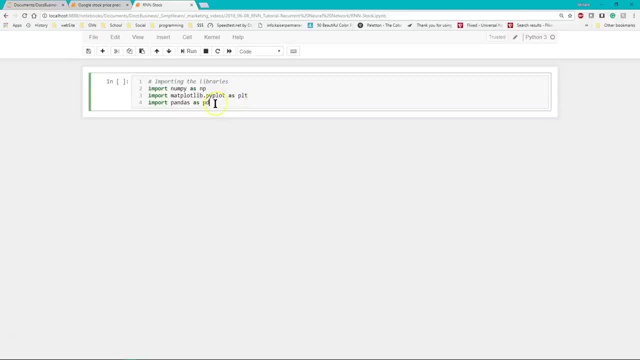 because we're going to do some plotting at the end and our pandas for our data set, our pandas is pd and when i hit run it really doesn't do anything except for load those modules. just a quick note. let me just do a quick draw here. oops, shift alt. there we go. you'll notice when we're doing this. 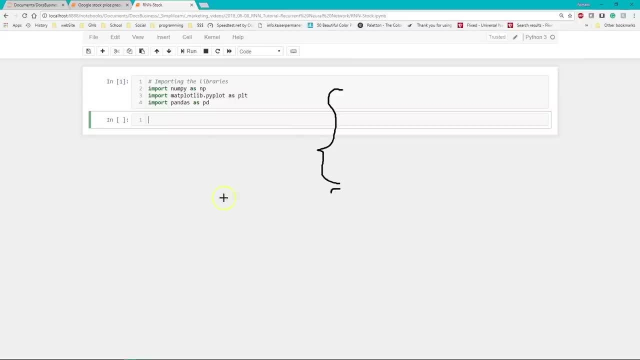 setup. if i was to divide this up, oops, i'm going to. actually, let's overlap these. here we go. this first part that we're going to do is our data prep- a lot of prepping involved, in fact, depending on what your system- and since we're using karas, i put 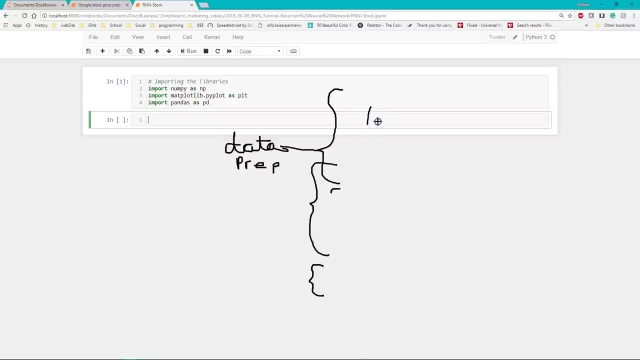 an overlap here, but you'll find that almost, maybe even half of the code we do is all about the data prep, and the reason i overlapped this with karas- let me just put that down because that's what we're working in- is because karas has like their own preset stuff, so it's already pre-built in. 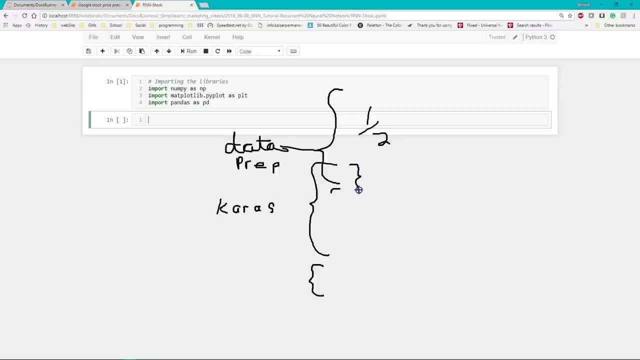 which is really nice. so there's a couple steps, a lot of times, that are in the karas setup. we'll take a look at that to see what comes up in our code as we go through and look at stock. and the last part is to evaluate and if you're working with 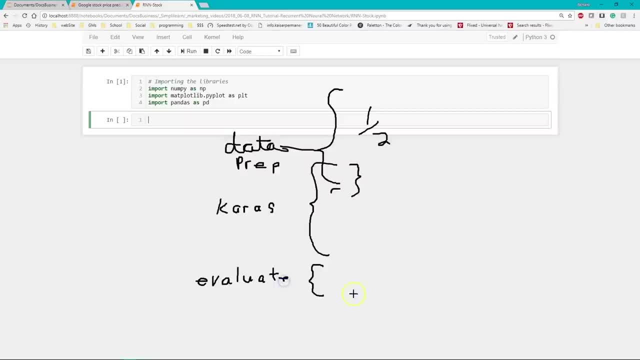 shareholders or classroom, whatever it is you're working with. the evaluate is the next biggest piece, so the actual code here crossed is a little bit more, but when you're working with some of the other packages you might have like three lines. that might be it. all your stuff is. 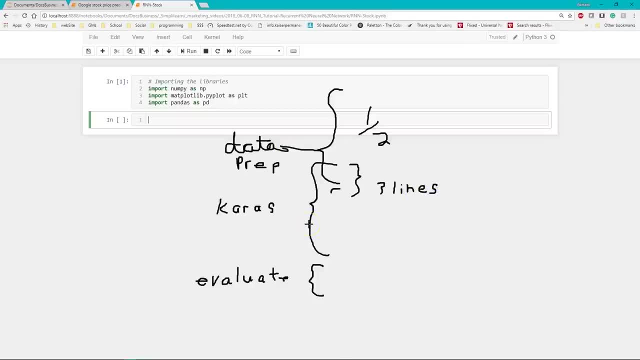 in your pre-processing and your data, since karas has is is cutting edge- and you load the individual. you'll see that there's a few more lines here and cross is a little bit more robust, and then you spend a lot of times, like i said, with the evaluate. you want to have something. you 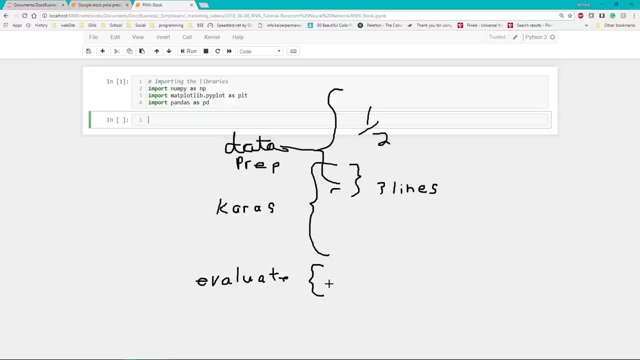 present to everybody else and say, hey, this is what i did, this is what it looks like. so let's go through those steps. this is like a kind of just general overview and let's just take a look and see what the next set of code looks like. and in here we have a data set train and it's going to 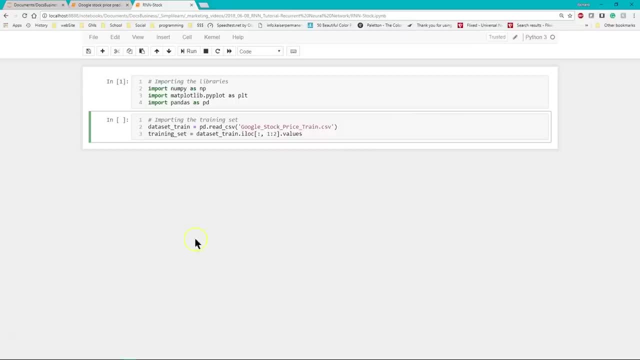 be read using the pd or pandas dot read csv and it's a google stock price train dot csv. and so we have training set equals data set, train dot i location and we've kind of sorted out part of that. so what's going on here? let's just take a look at, let's look at the actual file and see. 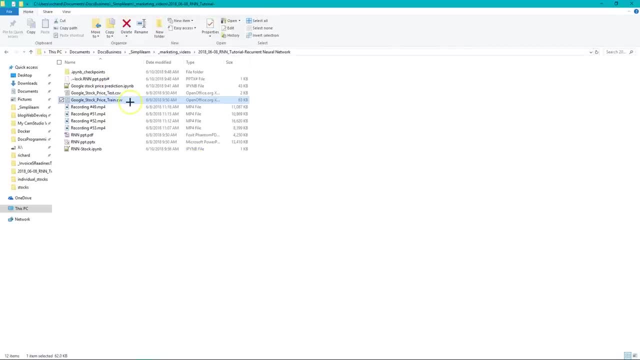 what's going on there now if we look at this, ignore all the extra files on this. i already have a train and a test set where it's sorted out. this is important to notice because a lot of times we do that as part of the pre-processing of the data, we take 20 of the data out so we can test it and 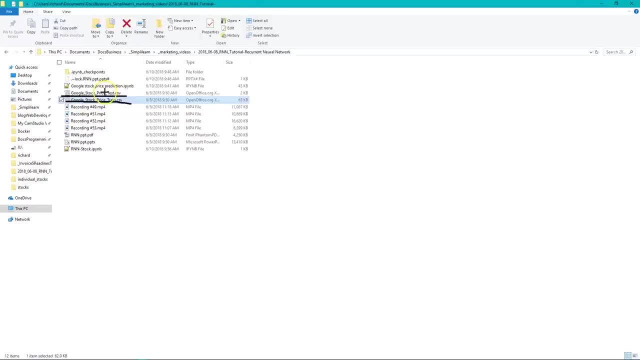 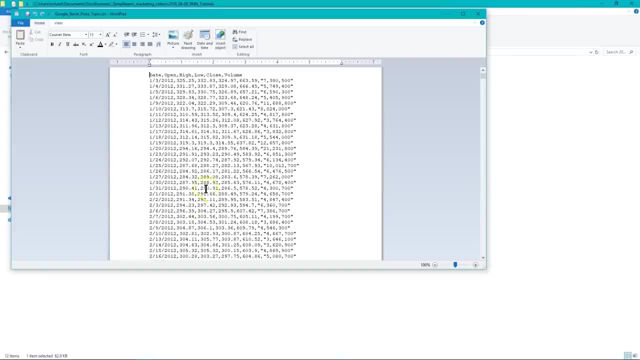 then we train the rest of it. that's what we use to create our neural network. that way we can find out how good it is. but let's go ahead and just take a look and see what that looks like as far as the file itself- and i went ahead and just opened this up in a basic word pad and text- 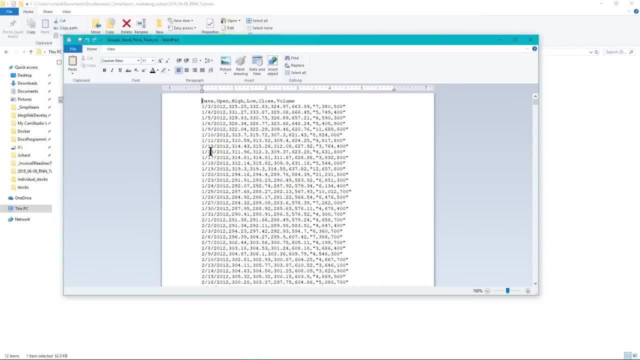 editor, just so we can take a look at it. certainly, you can open up an excel or any other kind of spreadsheet and we note that this is a comma separated variables. we have a date: open, high, low, close volume. this is the standard stuff that we import into our stock and we're the 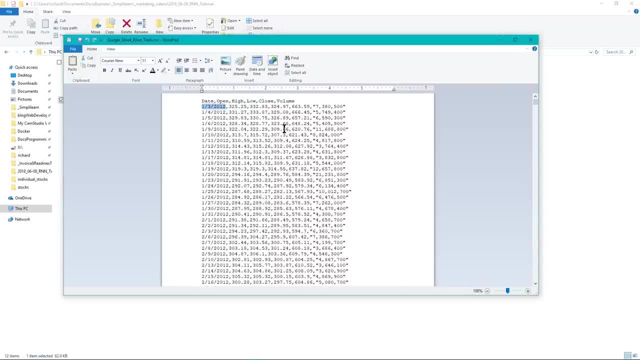 most basic set of information you can look at in stock. it's all free to download. in this case, we downloaded it from google. that's why we call it the google stock price and it specifically is google. this is the google stock values from. as you can see here, we started off at 1 3 2012.. 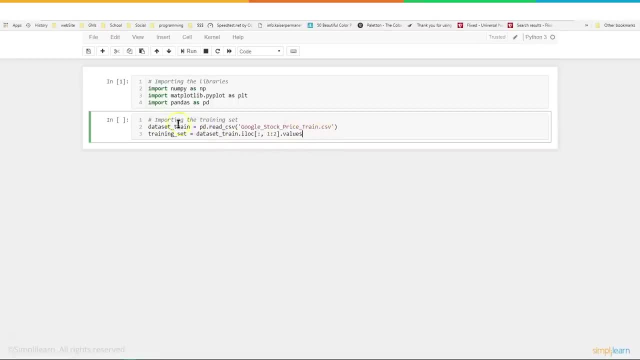 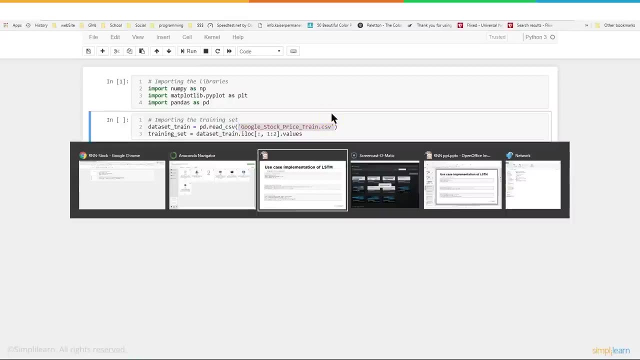 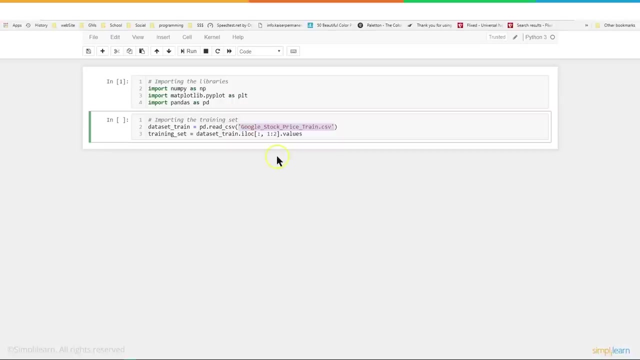 so when we look at this first setup up here, we have a data set: train equals pd, underscore csv and if you noticed on the original frame, let me just go back there- they had it set to home. ubuntu downloads google stock price train. i went ahead and changed that because 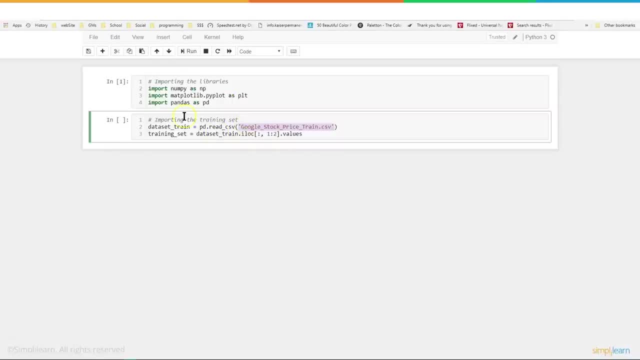 we're in the same file where i'm running the code, so i've saved this particular python code and i don't need to go through any special paths or have the full path on there. and then, of course, we want to take out certain values in here and you're going to notice that we're using 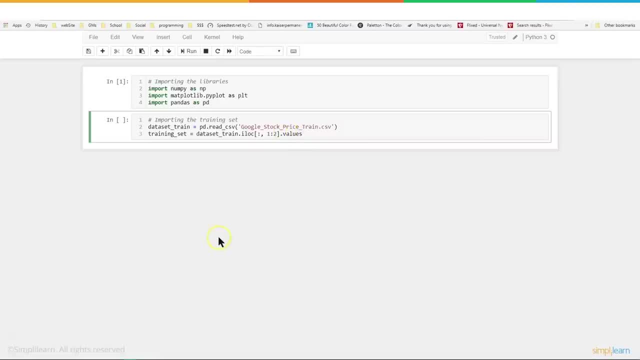 our data set and we're now in pandas, so pandas, basically, it looks like a spreadsheet and in this case, we're going to do i location, which is going to get specific locations. the first value is going to show us that we're pulling all the rows in the data. 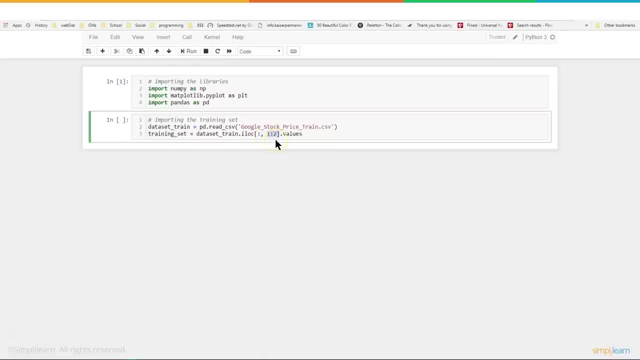 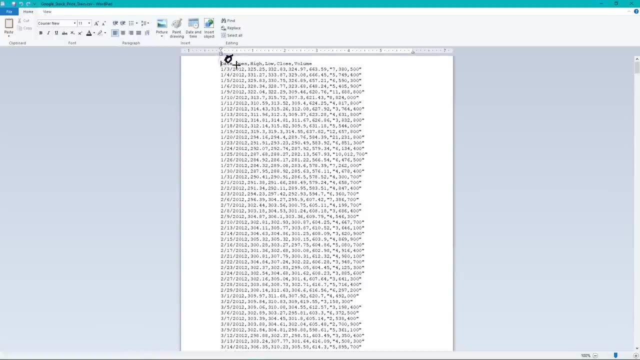 and the second one is we're only going to look at columns one and two and if you remember, here from our data, as we switch back on over columns, we always start with zero, which is the date, and we're going to be looking at open and high, which would be one and two. we'll just label that. 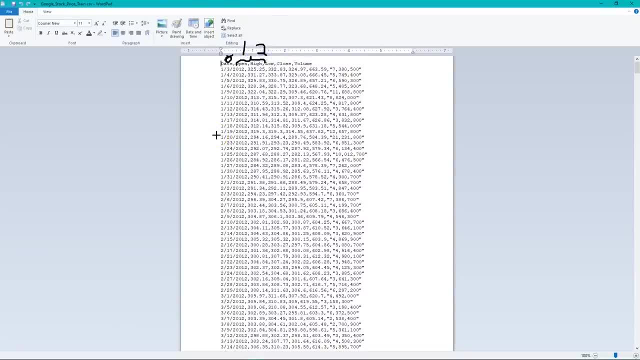 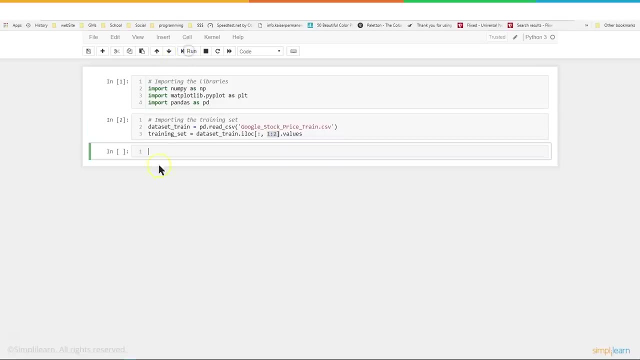 right there. so you can see now when you go back and do this. you certainly can extrapolate and do this on all the columns, but for the example let's just limit a little bit here so that we can focus on just some key aspects of stock, and then we'll go up here and run the code. and again i said the. 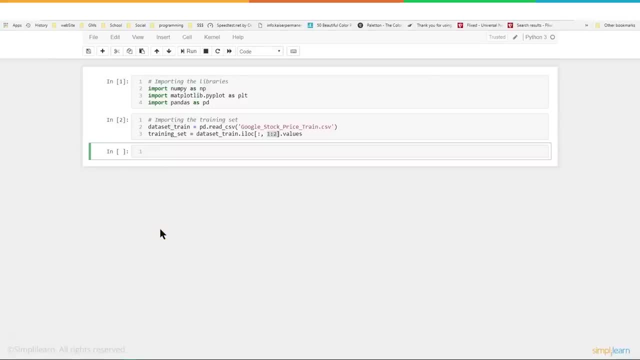 first half is very boring. whenever we hit the run button, it doesn't do anything because we're still just loading the data and setting it up. now that we've loaded our data, we want to go ahead and scale it. we want to do what they call feature scaling, and in here we're going to pull it up. 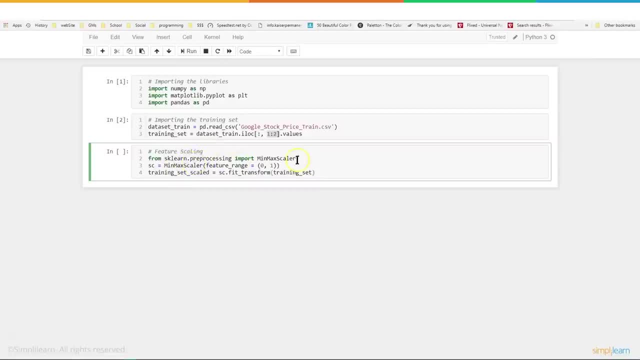 from the sk learn or the sk kit pre-processing import min max scaler. and when you look at this you got to remember that biases in our data. we want to get rid of that. so if you have something that's like a really high value, let's just draw a quick graph. and i have something here like the: 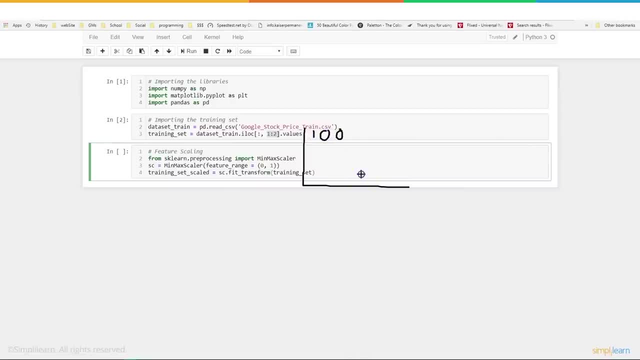 maybe the stock has a value. one stock has a value of a hundred and another stock has a value of five. um, you start to get a bias between different stocks and so when we do this, we go ahead and say, okay, a hundred is going to be the max and five is going to be the min, and then everything. 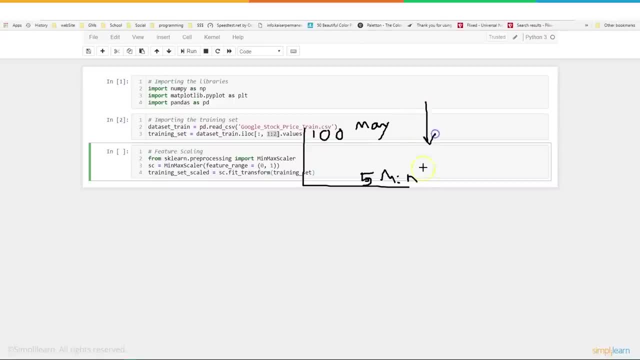 else goes, and then we change this, so we just squish it down- i like the word squish. so it's between one and zero. so 100 equals one, or one equals a hundred and zero equals five, and you can just multiply. it's usually just a simple multiplication. we're using uh multiplication. 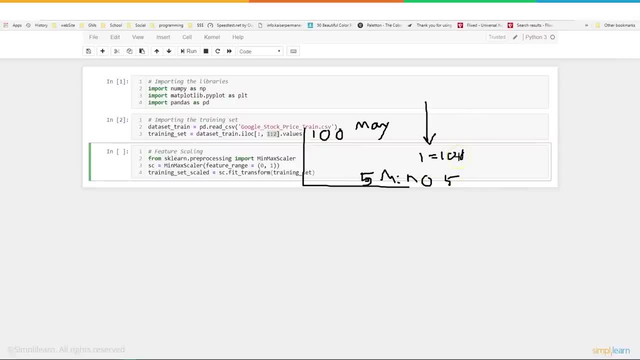 so it's going to be minus five, and then 100 divided, or 95 divided by one, so, or whatever value is is divided by 95.. and, uh, once we've actually created our scale, we've telling us going to be from zero to one. we want to take our training set and we're going to create a training. 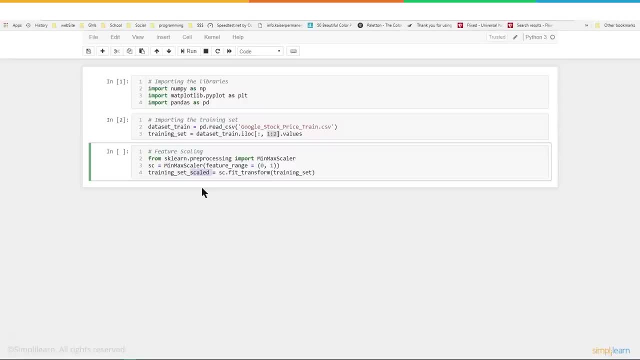 set scaled and we're going to use our scaler sc and we're going to fit. we're going to fit and transform the training set so we can now use the sc, this, this particular object. we'll use it later because, remember, we have to also scale that when we go to test our model and see how it works. and 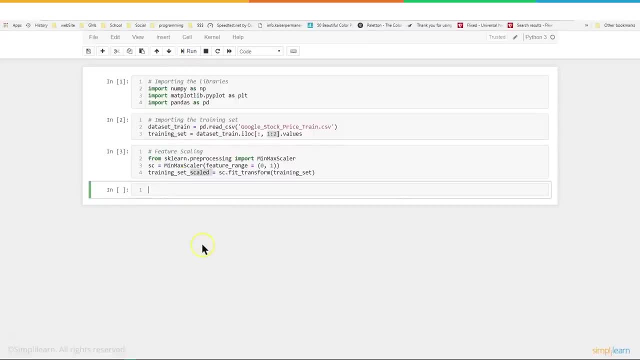 we'll go ahead and click on the run again. it's not going to have any output yet because we're just setting up all the variables. okay, so we paste the data in here and we're going to create the data structure with the 60 time steps and output. first note: we're running 60 time steps and that is. 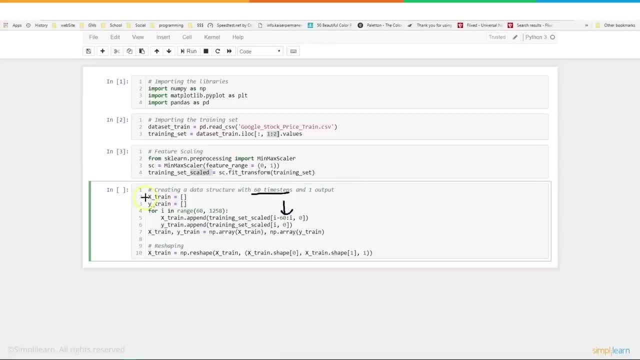 where this value here also comes in. so the first thing we do is we create our x train and y train and we set them to an empty python array- very important to remember what kind of array we're in, what we're working with- and then we're going to come in here, we're going to go for i in range. 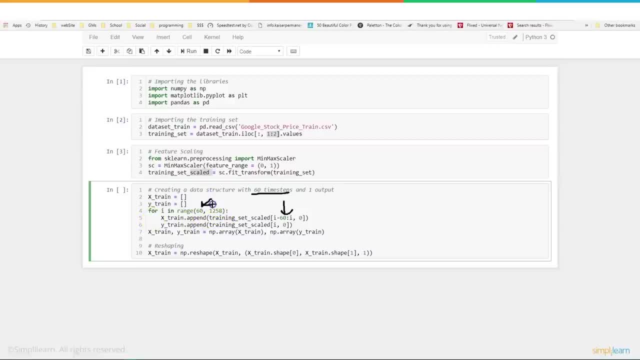 60 to 1258, there's our 60- 60 time steps, and the reason we want to do this is, as we're adding the data in, there's nothing below the 60. so if we're going to use 60 time steps, we have to start at. 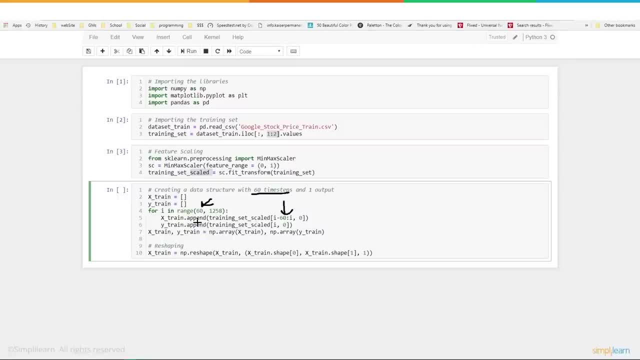 point 60 because it includes everything underneath of it. otherwise you'll get a pointer error. and then we're going to take our x train and we're going to append training set scaled. this is a scaled value between 0 and 1, and then, as i, is equal to 60. 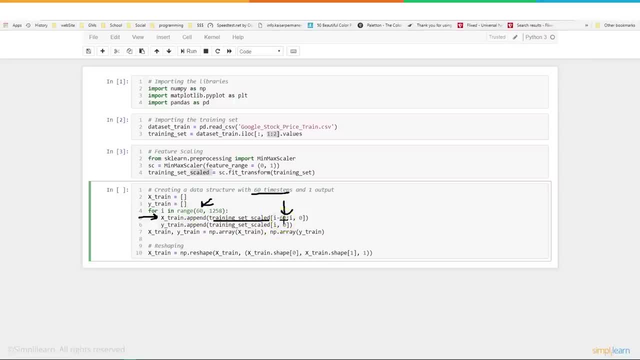 this value is going to be 60 minus 60 is 0.. so this actually is 0 to i. so it's going to be 0 to 60, 1 to 61- let me just circle this part right here: 1 to 61, 2 to 62 and so on and so on. and if 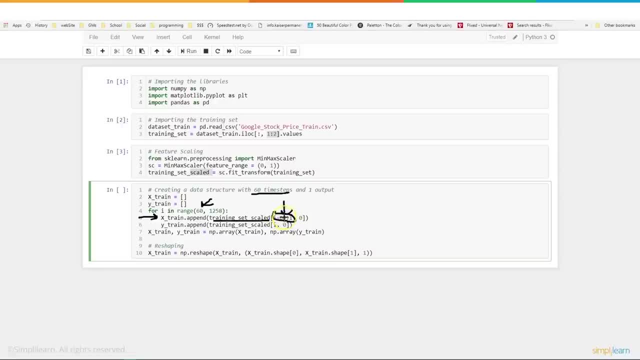 you remember i said 0 to 60. that's incorrect because it does not count. remember it starts at 0.. so this is a count of 60.. so it's actually 59.. important to remember that as we're looking at this and then the second part of this that we're looking at. so, if you remember correctly, here we go. 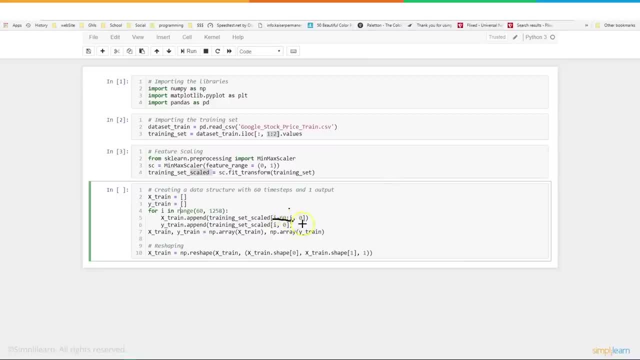 we go from 0 to 59 of i, and then we have a comma, a zero, right here, and so finally, we're just going to look at the open value. now i know we did put it in there for one to two, um, if you remember correctly. it doesn't count the second one, so it's just the open value we're looking at, just open. 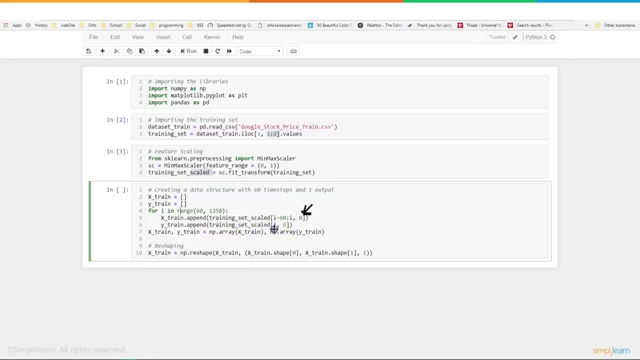 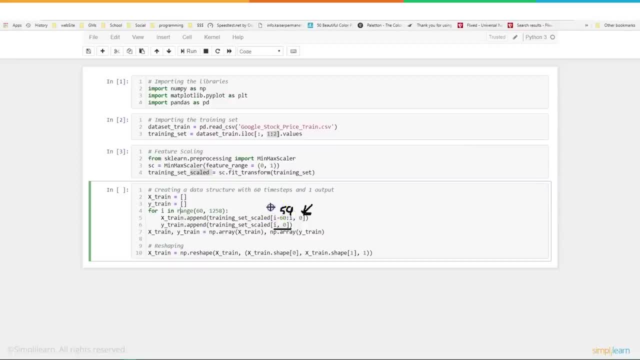 correctly, this is 0 to 59, so there's 60 values in it. uh, so when we do, i down here, this is number 60.. so we're going to do this is, we're creating an array and we have 0 to 59 and over here. 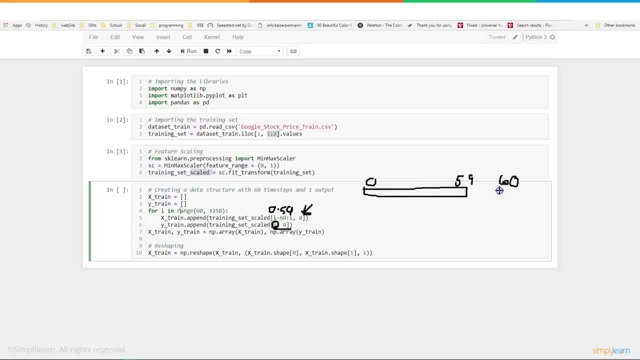 we have number 60, which is going into the y train. it's being appended on there and then this just goes all the way up. so this is down. here is a 0 to 59- and we'll call it 60, since that's the value over here- and it goes all the way up to 12- 58.. that's where this value here. 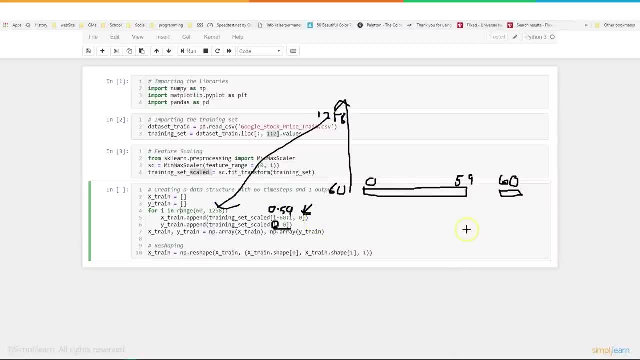 comes in. that's the length of the data we're loading. so we've loaded two arrays. we've loaded one array that has uh, which is filled with arrays from zero to 59, and we loaded one array, which is just the value and what we're looking at. you want to think about this as a time sequence? 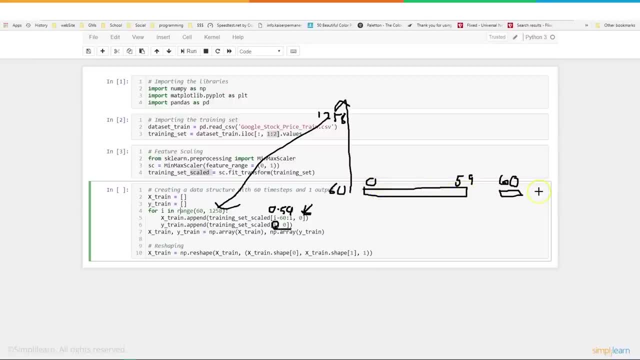 here's my open, open, open, open, open, open. what's the next one in the series? so we're looking at the google stock and each time it opens we want to know what the next one? 0 through 59, what's 60.. 1 through 60, what's 61, 2 through 62, what's 62, and so on and so on going up and then, once we've 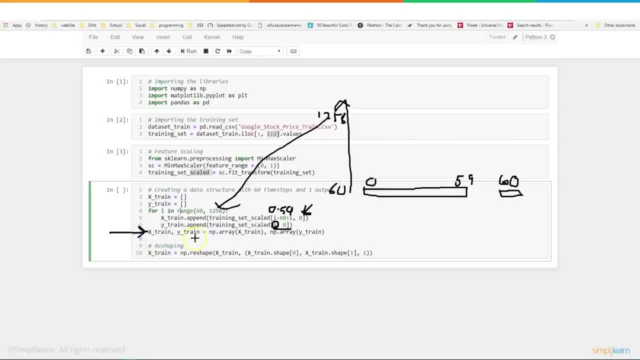 loaded those in our for loop. we go ahead and take x train and y train: equals np, dot array, x train, dot np array y train. we're just converting this back into a numpy array. that way we can use all the cool tools that we get with numpy array, including reshaping. 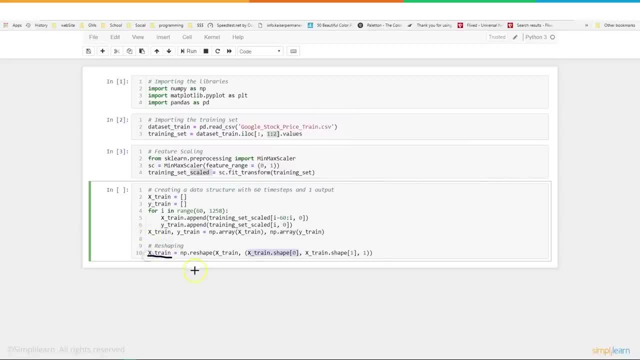 so if we take a look and see what's going on here, we're going to take our x train, we're going to reshape it. wow, what the heck does reshape mean? uh, that means we have an array, if you remember correctly, so many numbers by 60.. that's how wide it is, and so we're when. 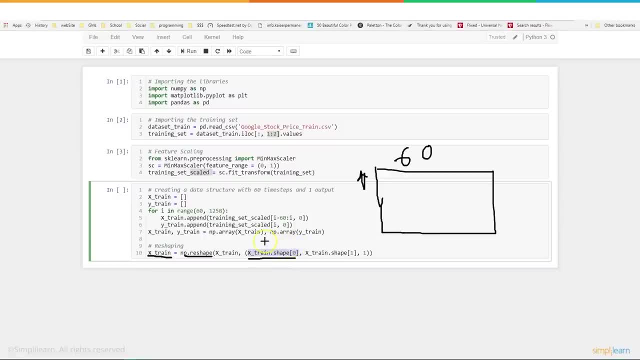 you, when you do x train dot shape, that gets one of the shapes and you get um x train dot shape of 1 and 2.. one gets the other shape and we're just making sure the data is formatted correctly, and so you use this to pull the fact that it's 60 by. in this case, where's that value? 60 by 1199, 1258 minus 60. 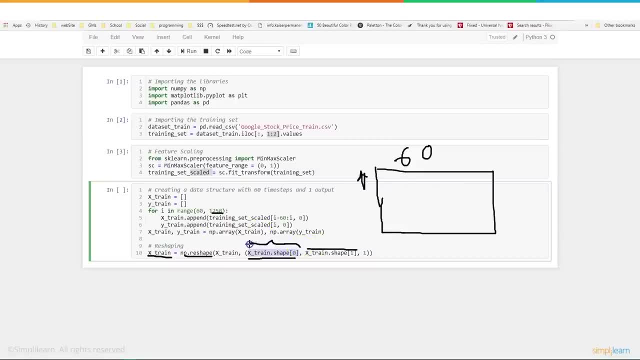 1199, and we're making sure that that is shaped correctly, so the data is grouped into 1199 by 60 different arrays, and then the one on the end just means at the end, because this, when you're dealing with shapes and numpy, they look at this as layers, and so the end layer needs to be one. 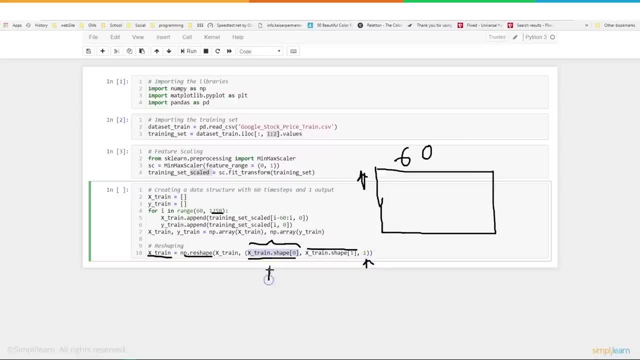 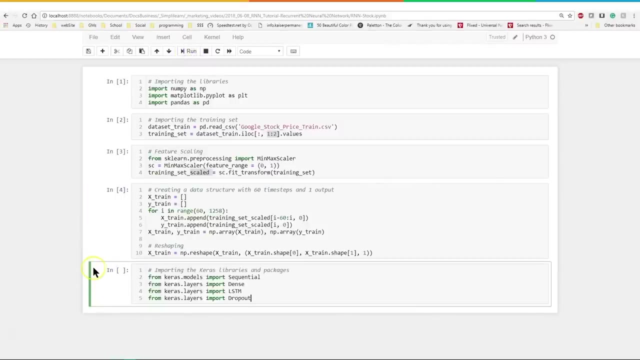 value. that's like the leaf of a tree, where this is the branch and then it branches out some more and then you get the leaf in P dot reshape comes from and using the existing shapes to form it, we'll go ahead and run this piece of code again- there's no real output- and then we'll import our 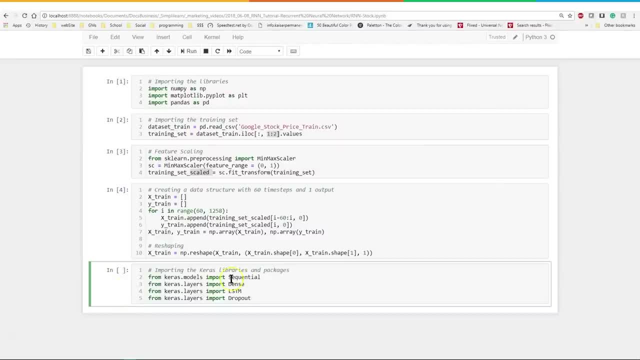 different cross modules that we need. so from cross models, we're going to import the sequential model from cross models. we're going to import the sequential model from cross models. we're going to model dealing with sequential data. we have our dense layers. we have actually three layers. we're 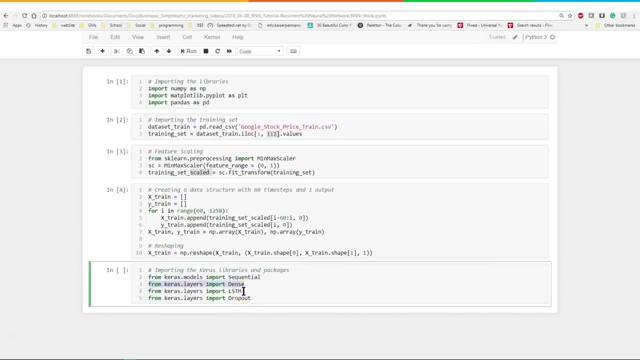 going to bring in our dense, our lstm- which is what we're focusing on- and our dropout, and we'll discuss these three layers more in just a moment. but you do need the with the lstm, you do need the dropout and then the final layer will be the dense. but let's go ahead and run this and that'll bring. 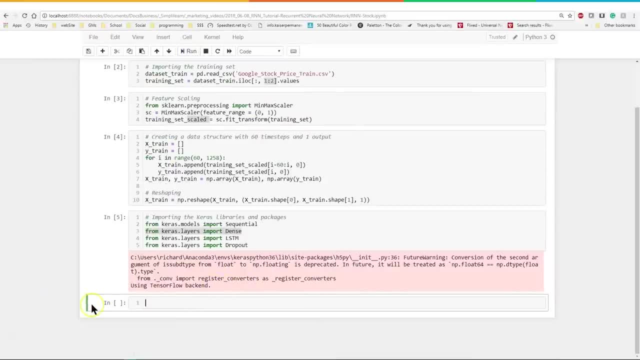 port our modules and you'll see we get an error on here. and if you read it closer, it's not actually an error, it's a warning. what does this warning mean? these things come up all the time when you're working with such cutting edge. modules are completely being updated all the time. we're 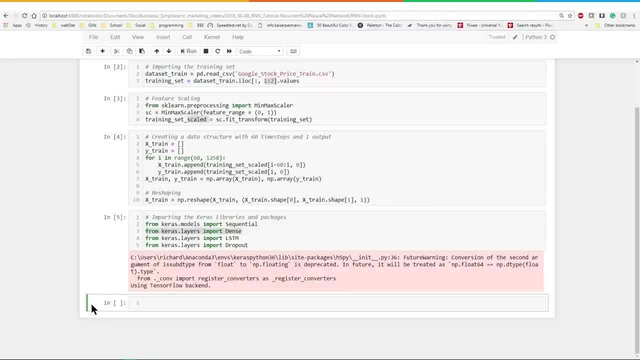 not going to worry too much about the warning. all it's saying is that the h5py module, which is part of karas, is going to be updated at some point, and if you're running new stuff on karas and you start updating your karas system, you better make sure that your h5py is updated too. 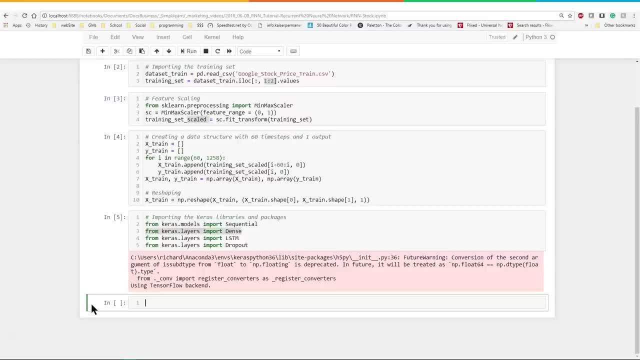 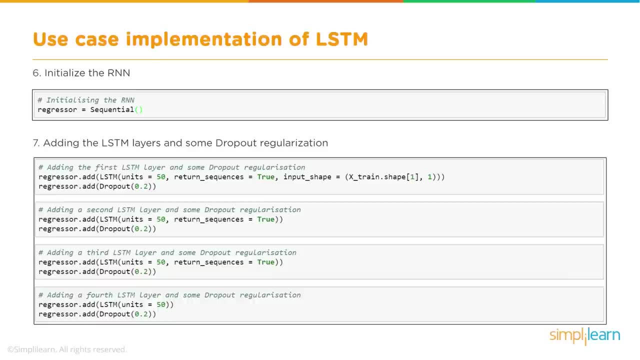 otherwise you're going to have an error later on and you can actually just run an update on the h5py now if you wanted to. not a big deal, we're not going to worry about that today, and i said we were going to jump in and start looking at what those layers mean. i meant that 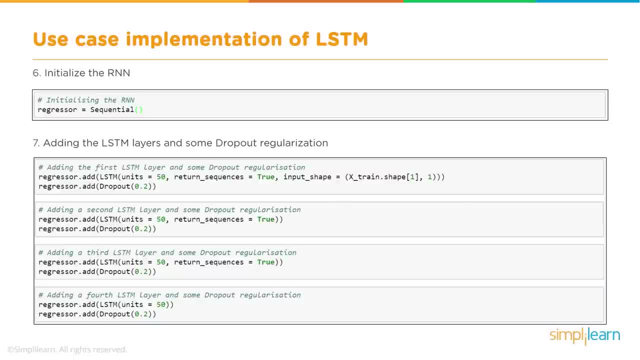 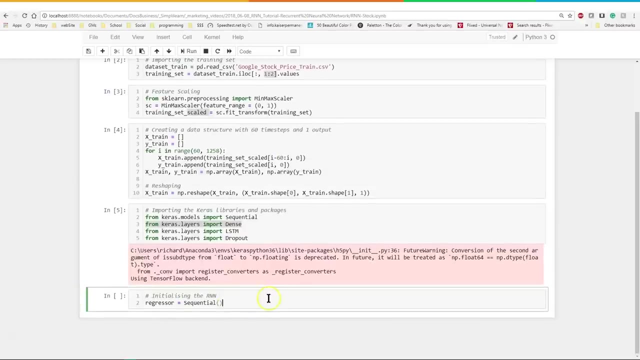 and we're going to start off with initializing the rnn and then we'll start adding those layers in and you'll see that we have the lstm and then the dropout lstm, then dropout, lstm, then dropout. what the heck is that doing? so let's explore that. we'll start by initializing the rnn- regressor. 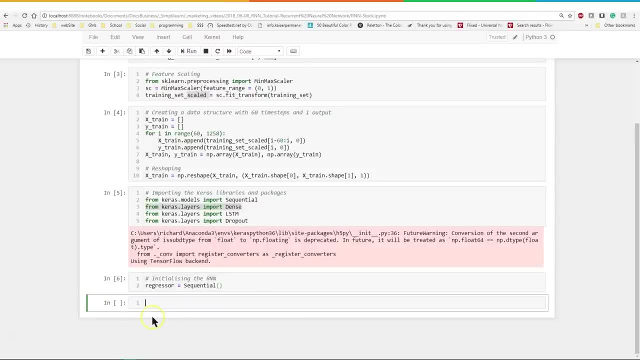 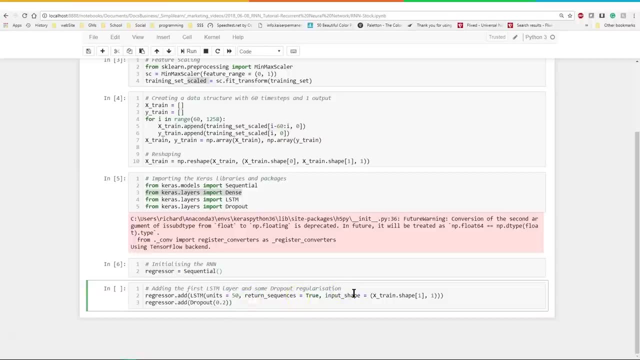 equals sequential, because we're using the sequential model and we'll run that and load that up and then we're going to start adding our lstm and then we're going to start adding our lstm layer and some dropout regularization and right there should be the q dropout regularization. 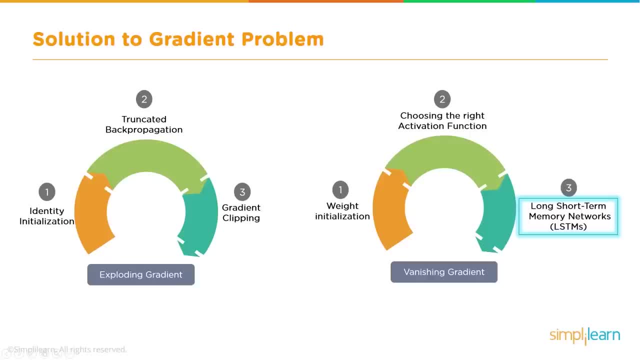 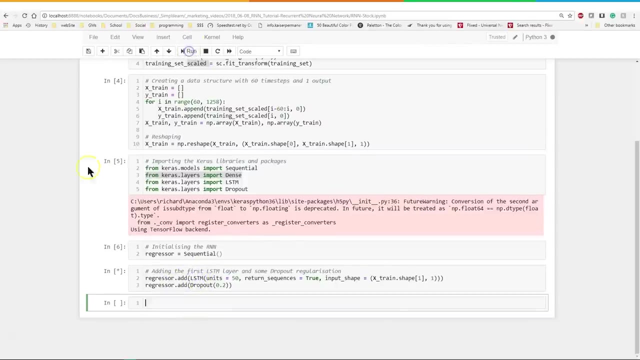 and if we go back here and remember our exploding gradient, well, that's what we're talking about. the dropout drops out unnecessary data, so we're not just shifting huge amounts of data through the network, so, and so we go in here. let's just go ahead and add this in. i'll go ahead and run this. 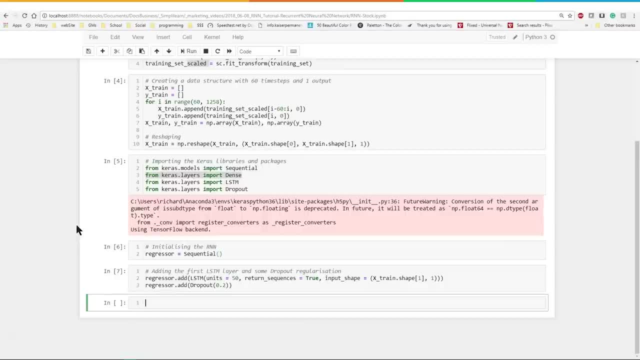 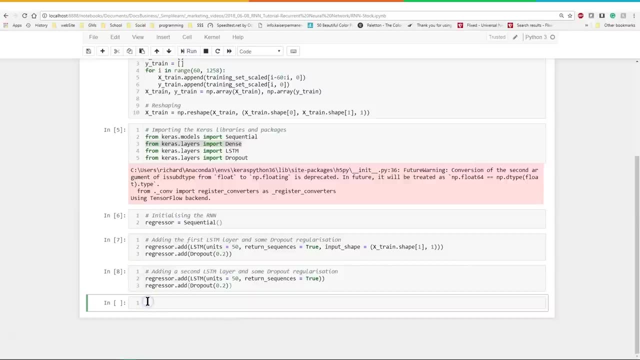 and we had three of them. so let me go ahead and put all three of them in and then we can go back over them. here's the second one, and let's put one more in. let's put that in, and we'll go ahead and put two more in. i meant to. i said one more in, but 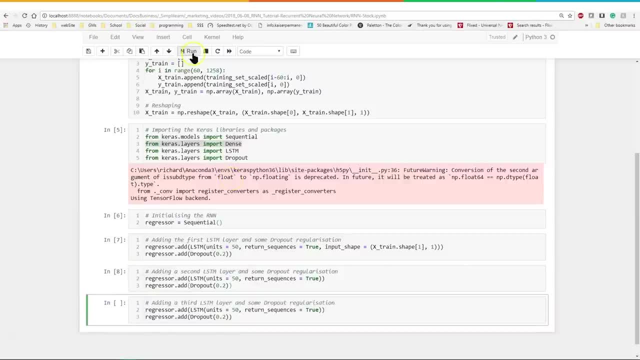 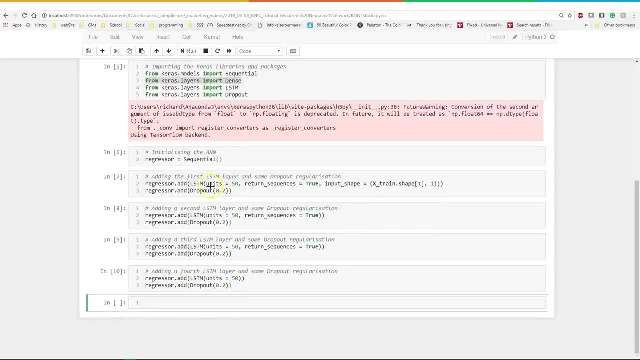 it's actually two more in, and then let's add one more after that and, as you can see, each time i run these they don't actually have an output. so let's take a closer look and see what's going on here. so we're going to add our first lstm layer in here. we're going to have units 50. the units is the. 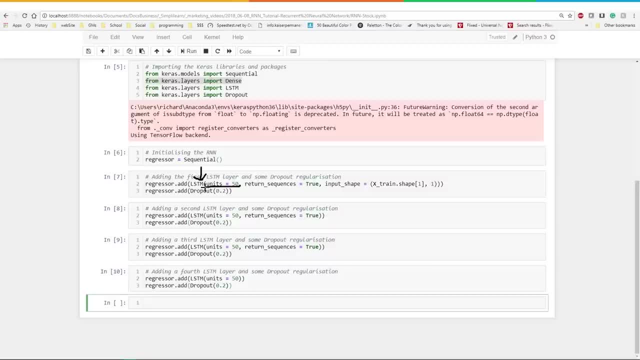 positive integer and it's the dimensionality of the output space. this is what's going out into the next layer, so we might have 60 coming in, but we have 50 going out. we have a return sequence because it is a sequence data, so we want to keep that true. and then you 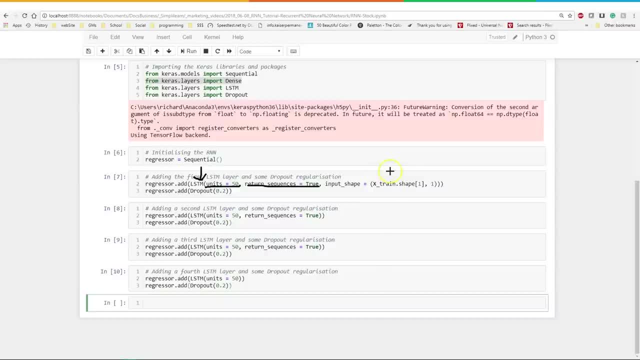 have to tell it what shape it's in. well, we already know the shape by just going in here and looking at x train shape. so input shape equals the x train shape of one comma one. makes it real easy. you don't have to remember all the numbers that put in 60 or whatever else is in there, you just let it. 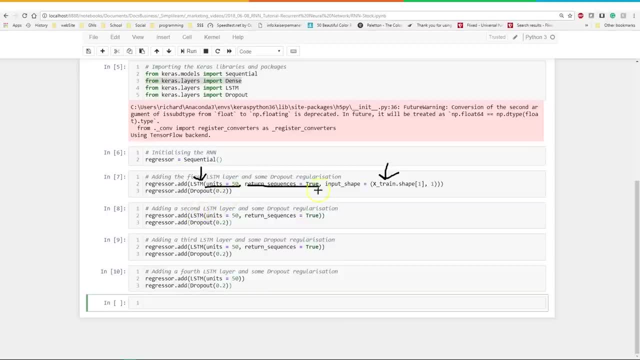 tell the regressor what model to use, and so we follow our stm with a dropout layer. now, understanding the dropout layer, it's kind of exciting, because one of the things that we're going to do is we're going to see how much of a change it's going to make, but at the same time, it's going to take a 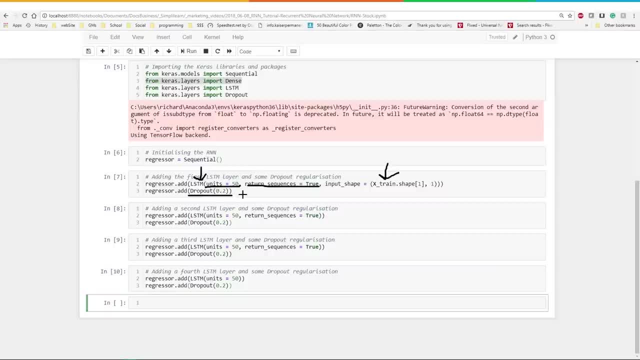 little bit of time, because actually the difference between an average and low-end state of state ofinya is that you could have a different state of integrand and a different set of parameters to make it a little bit more complex. and now we're going to see how. 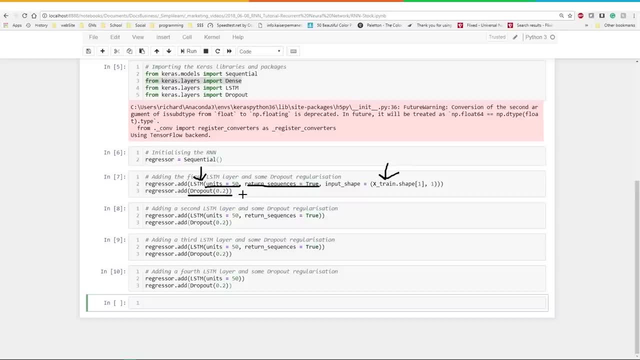 to put it on the sample, so that way we know what the difference is between the two. we're going to have a more constant learning cycle, and so we're going to look at it one by one. we're going to have 10 kind of switch modes and we're going to see how that works in a few minutes. we're going. 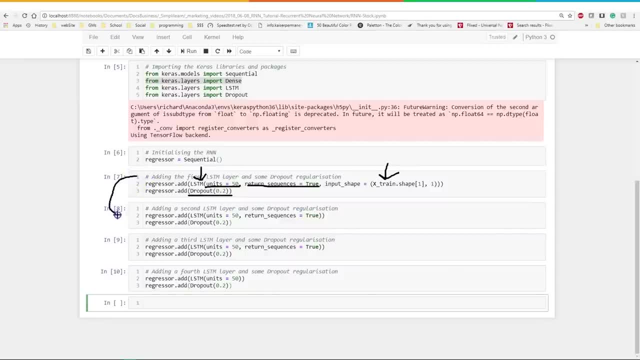 to see how the difference is going to be in terms of what data is going to be coming in, as well as in the, and finally, they see a big difference as we go from the first to the second and third and fourth. the first thing is we don't have to input the shape, because the shapes already the output units. 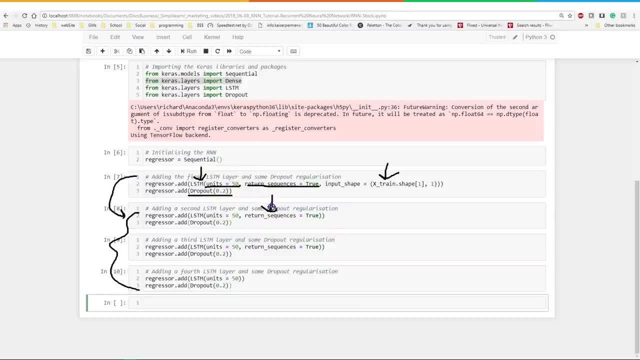 is 50 here. this out of the next step automatically knows this layer is putting out 50 and because it's the next layer, it automatically sets that and says: oh, 50 is coming out from our last layer. it's coming out, you know, goes into the regressor and of course we have our dropout and that's what's. 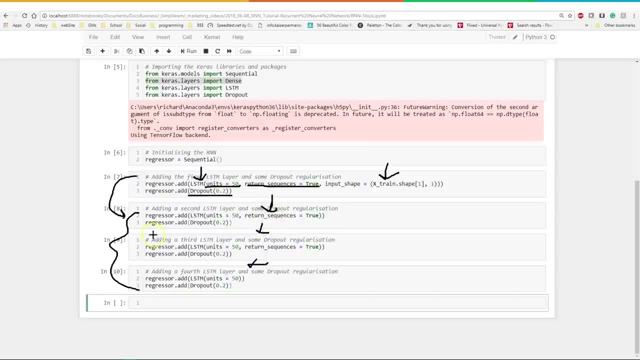 coming into this one and so on and so on, and so the next three layers. we don't have to let it know what the shape is. it automatically understands that and we're going to keep the units the same. we're still going to do 50 units. it's still a sequence coming through 50 units and a sequence. 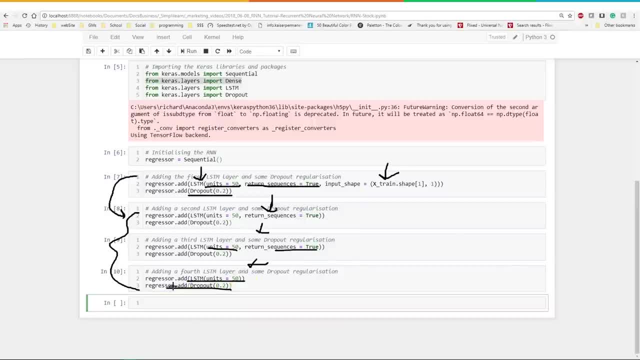 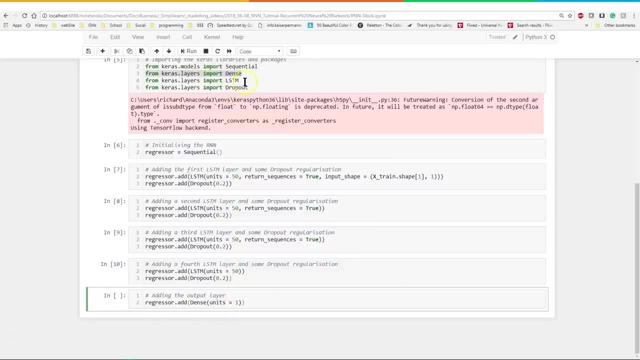 now the next piece of code is what brings it all together. let's go ahead and take a look at that and we come in here, we put the output layer, the dense layer and if you remember, up here we had the three layers, we had lstm, dropout and dense. dense just says we're going to bring. 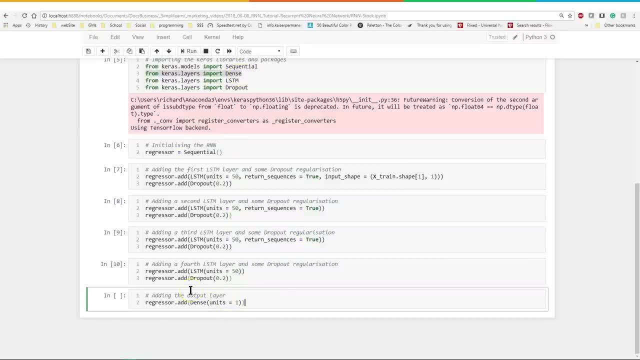 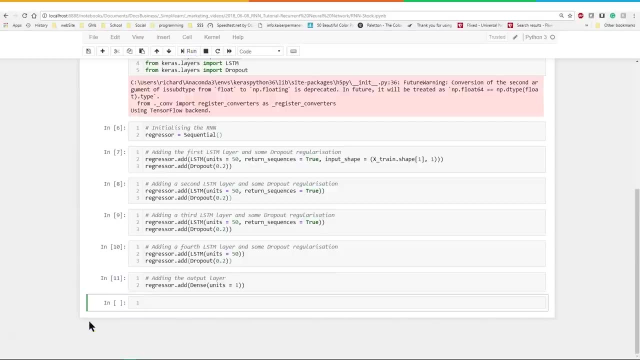 this all down into one output, instead of putting out a sequence. we just know. I want to know the answer at this point and let's go ahead and run that. and so in here you notice, all we're doing is setting things up one step at a time. so far, we've brought in our way up here. we brought in 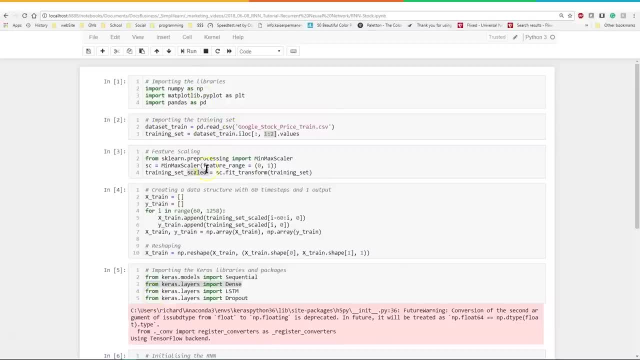 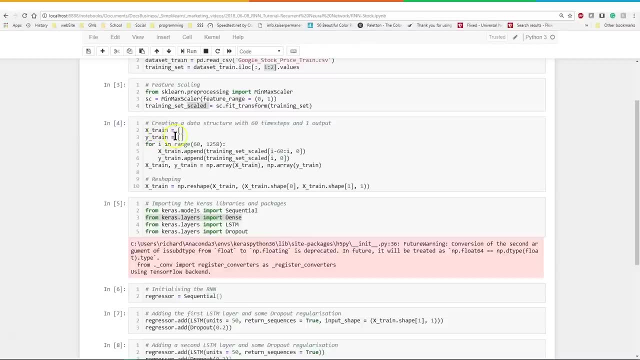 our data we bought in our different modules, we formatted the data for training it, we set it up. you know we have our white X train and our Y train. we have our source of data and the answers where we know so far that we're going to put in there. we've reshaped that. 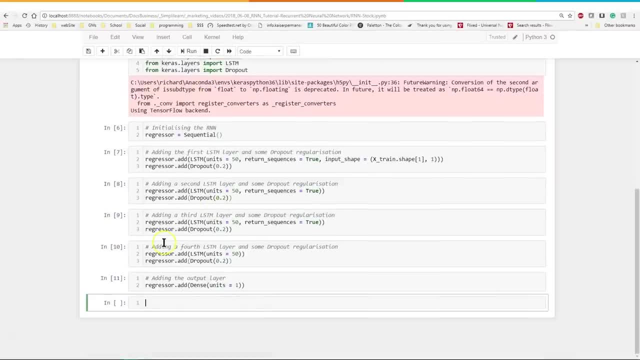 we've come in and built our cross, we've imported our different layers and we have in here. if you look, we have what five total layers now cross is a little different than a lot of other systems. there's a lot of other systems put this all in one line and do it automatic, but they don't give. 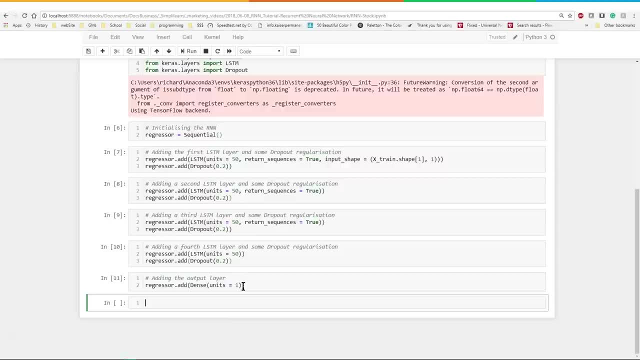 you the options of how those layers interface and they don't give you the options of how the data comes in. cross is cutting edge for this reason. so, even though it's a lot of extra steps and building the model, this has a huge impact on the output and what we can do with this. these 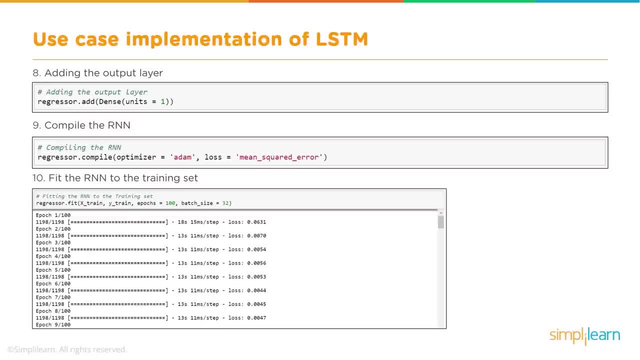 new models from karas. so we brought in our dense. we have our full model put together, our regressor, so we need to go ahead and compile it and then we're going to go ahead and fit the data. we're going to compile the pieces so they all come together and then we're going to run our training. 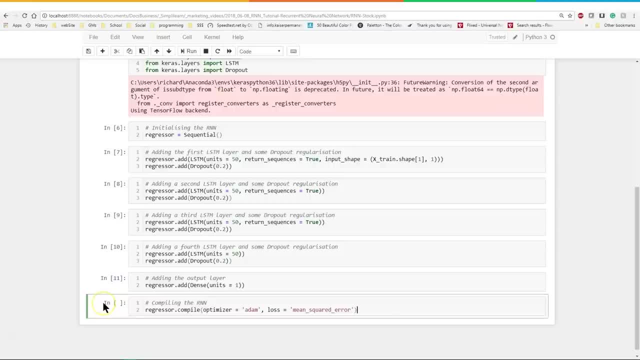 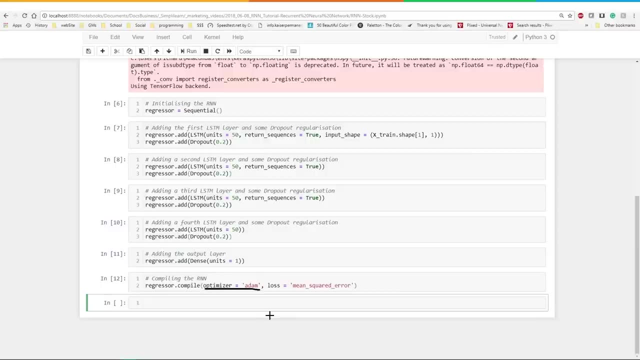 data on there and actually recreate our regressor. so it's ready to be used. so let's go ahead and compile that and I can go ahead and run that. and if you've been looking at any of our other tutorials on neural networks, you'll see we're going to use the optimizer Adam. Adam is optimized. 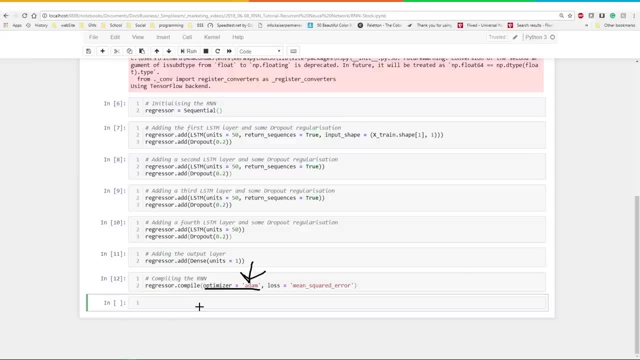 for big data. there's a couple other optimizers out there beyond the scope of this tutorial, but certainly Adam will work pretty good for this. and loss equals mean squared value, so when we're training it, this is what we want to base the loss on. how bad is our error? we're going to use the. 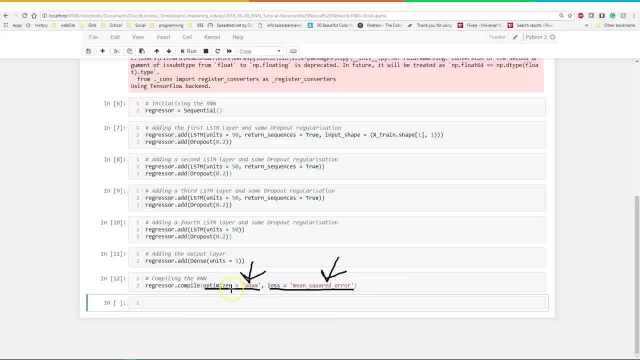 mean squared value for our error and the atom optimizer for its differential equations. you don't have to know the math behind them, but certainly it helps to know what they're doing and where they fit into the bigger models, and then, finally, we're going to do our fit fitting. 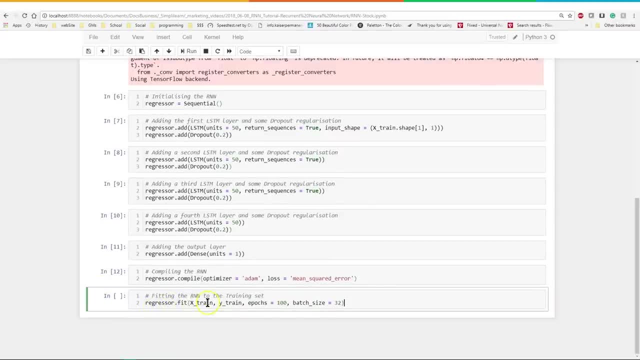 the RNN to the training set. we have the regressor dot, fit, X train, Y train, epics and batch size. so we know where this is. this is our data coming in for the X train, our Y train is the answer we're looking for of our data, our sequential input. 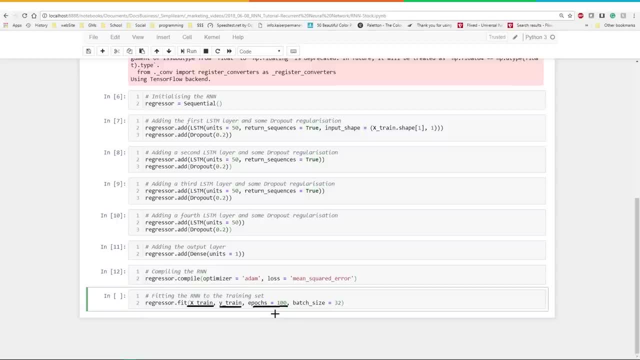 epics is how many times we're going to go over the whole data set. we created a whole data set of X train, so this is each, each of those rows, which includes a time sequence of 60 and batch size. another one of those things where cross really shines is if you were pulling this a from. 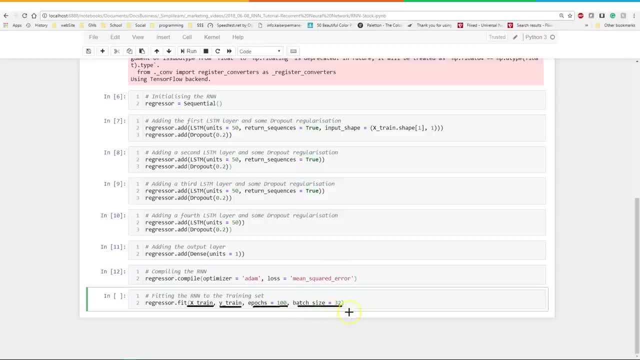 file. instead of trying to load it all into RAM, it can now pick smaller batches up and load those indirectly. we're not worried about pulling them off a file today because this isn't big enough to cause the computer too much of a problem to run, not too straining on the resources, but as we run. 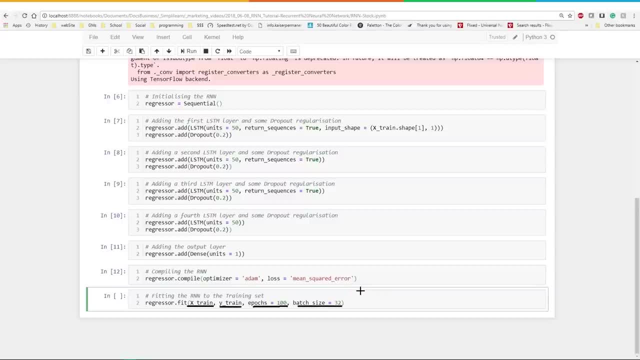 this. you can imagine what happened if I was doing a lot more than just one column in one set of stock, in this case, Google stock. imagine if I was doing this across all the stocks and I had, instead of just the open, I had open, close, a high, low, and you can actually 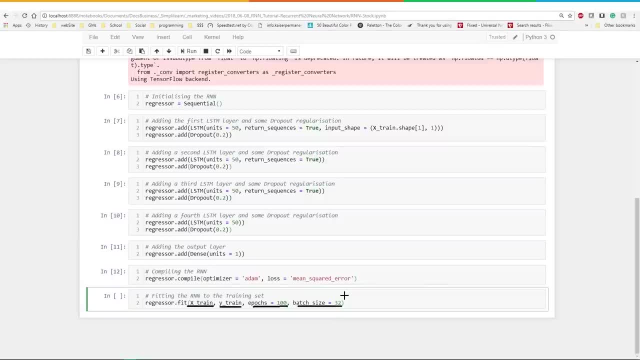 find yourself with about 13 different variables times 60. this is a time sequence. suddenly you find yourself with a gig of memory you're loading into your RAM, which will just completely you know if it's just, if you're not on multiple computers or cluster, you can start running into resource. 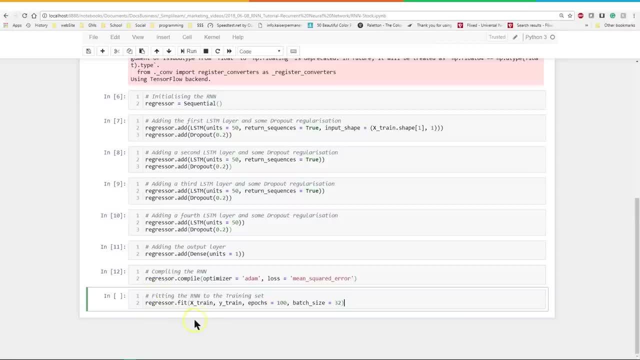 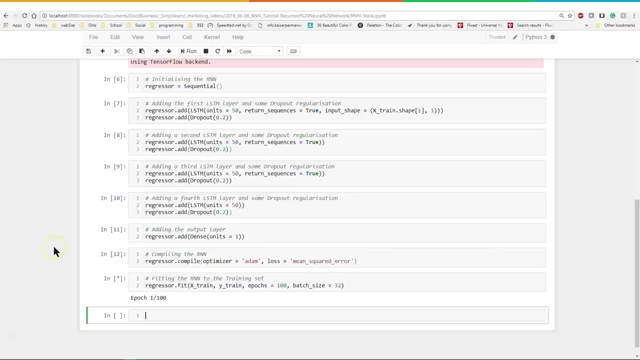 problems, but for this we don't have to worry about that. so let's go ahead and run this- and this will actually take a little bit on my computer, it's an older laptop- and give a second to kick in there. there we go. alright, so we have epic. so this is going to tell me it's running the first run. 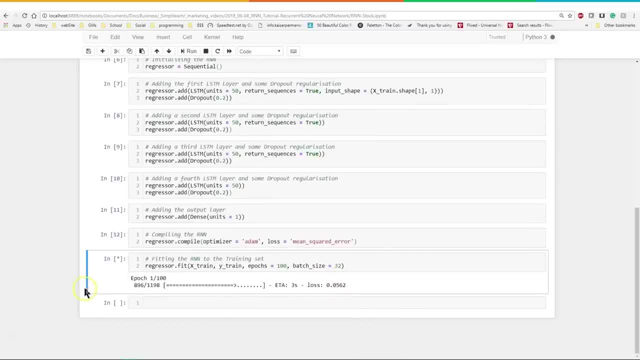 data and, as it's going through, it's batching them in 32 pieces, so 32 lines each time, and there's 1198. I think I said 1199 earlier, but it's 1198. I was off by one- and each one of these is 13 seconds, so you. 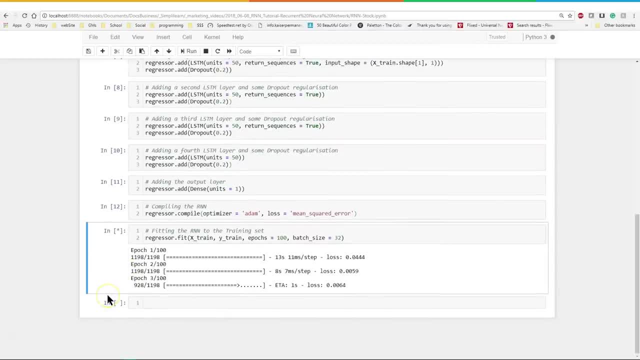 can imagine. this is roughly 20 to 30 minutes run time on this computer. like I said, it's an older laptop running at 0.9 gigahertz on a dual processor, and that's fine. what we'll do is: I'll go ahead and 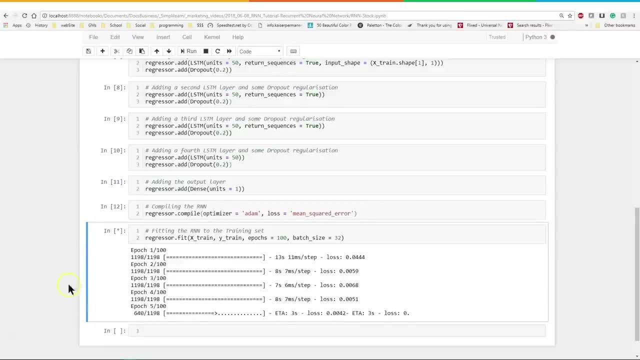 stop, go get a drink of coffee and come back and let's see what happens at the end and where this takes us. and, like you can see, it's running a little bit faster than what it used to do and, like any good cooking show, I've kind of gotten my latte. I also had some other stuff running in. 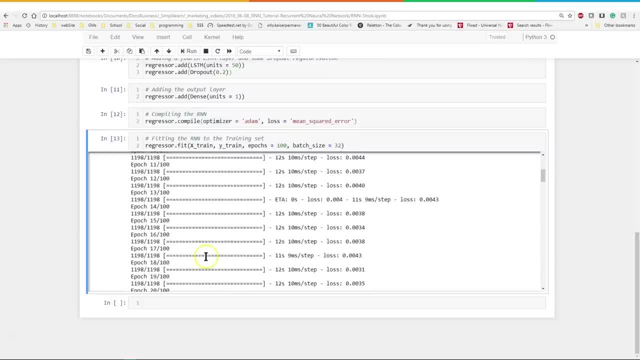 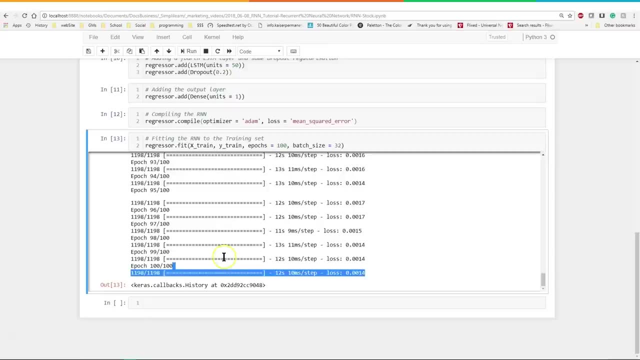 the background. so you'll see these numbers jumped up to like 19 seconds, 15 seconds which you can scroll through and you can see we've run it through 100 steps or 100 epics. so the question is, what does all this mean? one of the first things you'll notice is that our loss can is over. here it kind. 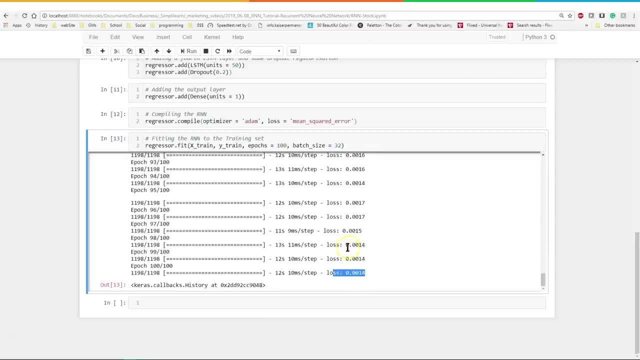 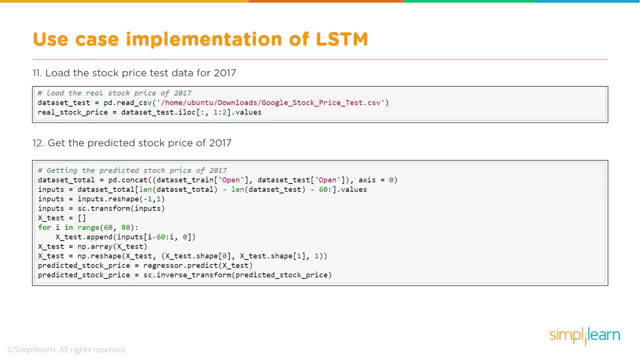 of stopped at 0.0014, but you can see it kind of goes down until we hit about 0.014 three times in a row. so we guessed our epic pretty close, since our loss has remained the same on there. so to find out what we're looking at, we're going to go ahead and load up our test data, the test data that we 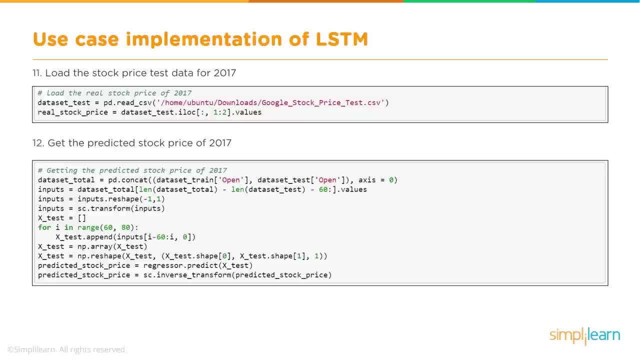 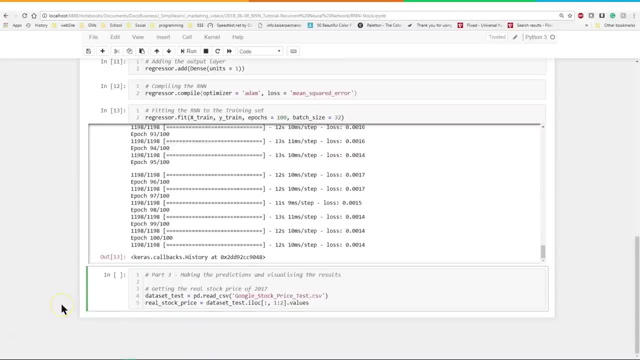 didn't process yet, and a real stock price data set test i location. this is the same thing we did when we prepped the data in the first place. so let's go ahead and go through this code and we can see. we've labeled it. part three: making the predictions and visualizing the results. so the 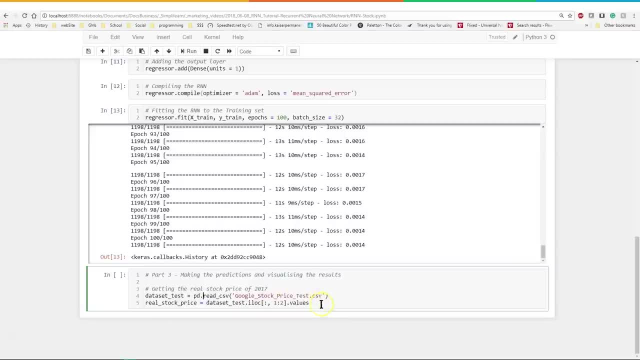 first thing we need to do is go ahead and read the data in from our test csv- and you see I've changed the path on it for my computer- and then we'll call it the real stock price, and again we're doing just the one column here and the values from i location, so it's all the rows. 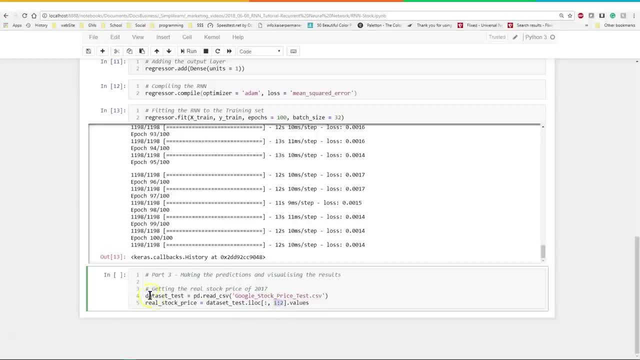 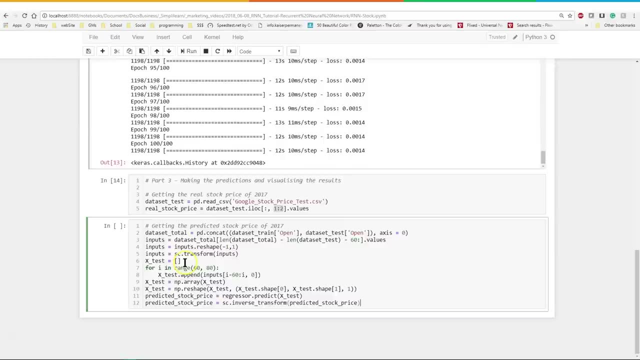 and just the values from these, that one location, that's the open stock open. let's go ahead and run that so that's loaded in there, and then let's go ahead and create. we have our inputs, we're going to create inputs here, and this should all look familiar. this is the same thing we did before. 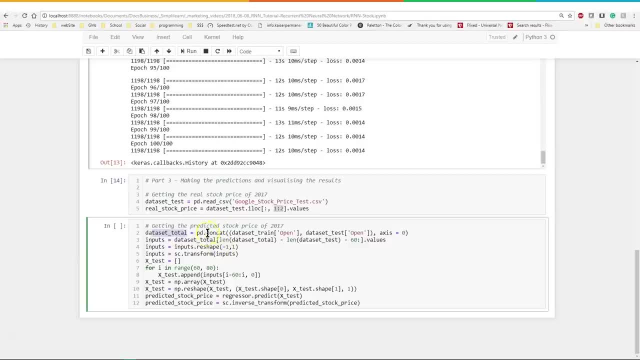 we're going to take our data set total, we're going to do a little pandas can cap from the data state and we're going to set it to the number that we need to set and ultimately that point is our index. so it's just a little more minimal, but here's just like anłe algorithm that, like I said, 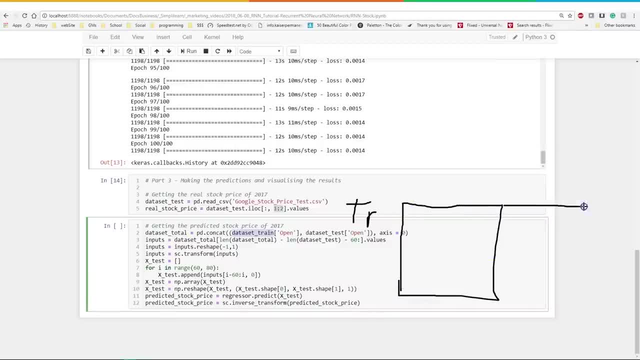 Premier's matrix set. we're going to mombo pneumonia set right here, set here and we'll go ahead and create the model. and then it's going to open the text tool. this will get lock up and let us go ahead and close it with our left-hand side. that a regular glue type computer. I can even return. 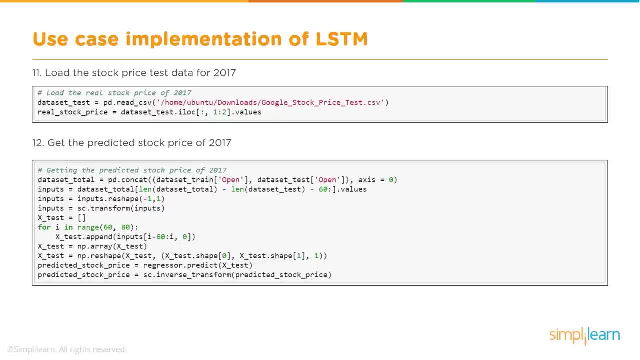 in our code where we can use: give us that a string to input: win each value in here, built into the SAMRends the test data that we didn't process yet and a real stock price data set test I location. this is the same thing. we did it when we prepped the data in the first. 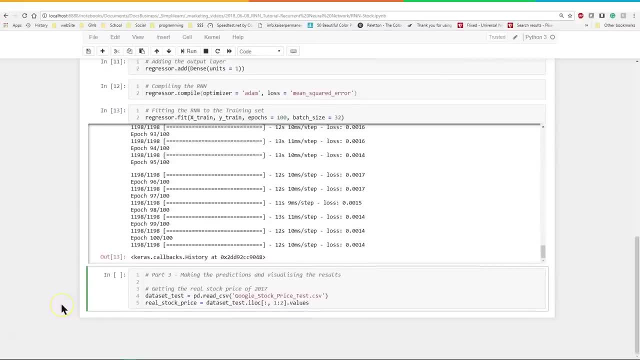 place. so let's go ahead and go through this code and we can see we've labeled it part three, making the predictions and visualizing the results. so the first thing we need to do is go ahead and read the data in from our test CSV, you see. 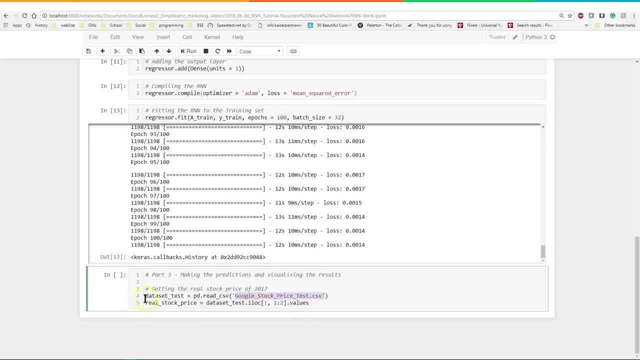 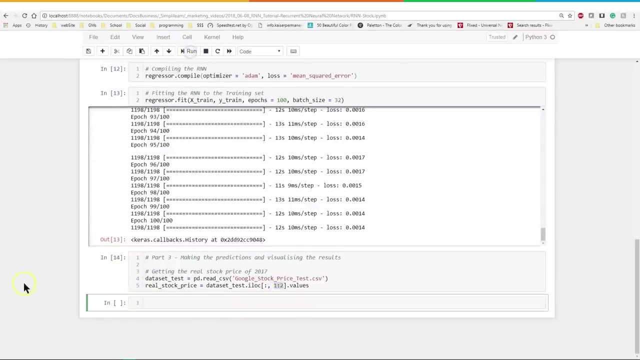 I've changed the path on it for my computer and then we'll call it the real stock price and again we're doing just the one column here and the values from my location. so it's all the rows and just the values from these, that one location. that's the open stock open. let's go ahead and run that, so that's. 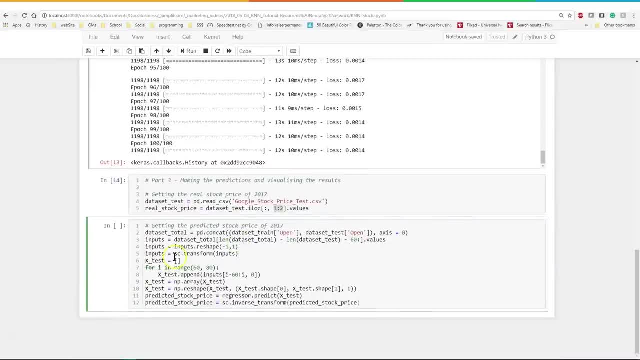 loaded in there and then let's go ahead and create. we have our inputs, we're gonna create inputs here and this should all look familiar because this is the same thing we did before. we're gonna take our data set total. we're gonna do a little pandas can cap from the data set train. now, remember the end of the. 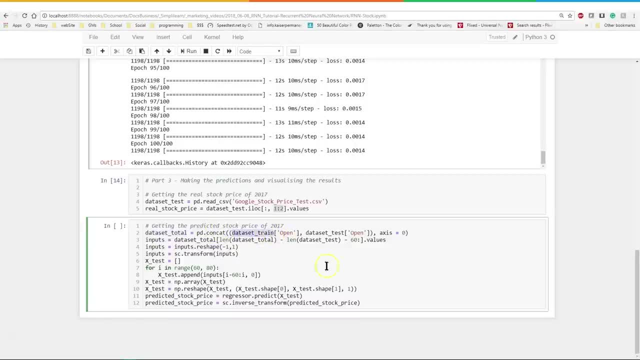 data set. train is part of the data going in and let's just visualize that just a little bit. here's our train data. let me just put TR for train and it went up to this value here, but each one of these values generated a bunch of columns. it was 60 across and this value here equals this one and this value here. 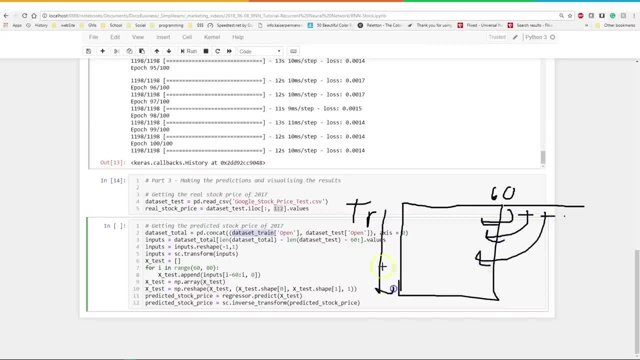 equals this one, and this value here equals this one, and so we need these top 60 to go into our new data, because that's part of the next data, or it's actually the top 59. so that's what this first setup is over. here is we're going in, we're doing the real stock price and 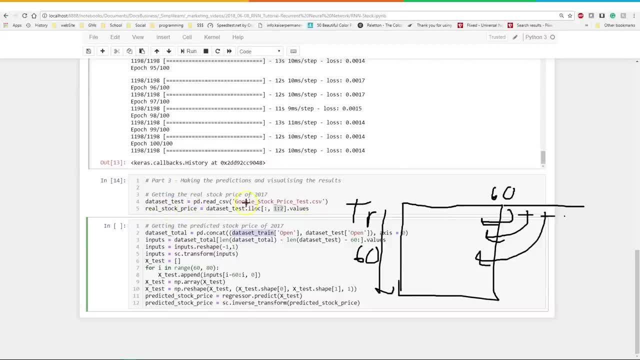 we're gonna just take the data set test and we're gonna load that in and then the real stock price is our data test test location. so we're just looking at that first column, the open price, and then our data set total. we're gonna take pandas and we're gonna concat and we're gonna take our data set train for the 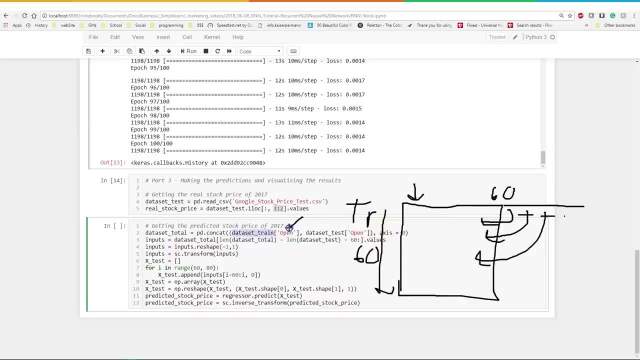 open and our data set test open, and this is one way you can reference these columns. we've referenced them a couple different ways. we've referenced them up here with the one two, but we know it's labeled as a pandas set is open, so pandas is great that way. lots of versatility there. and 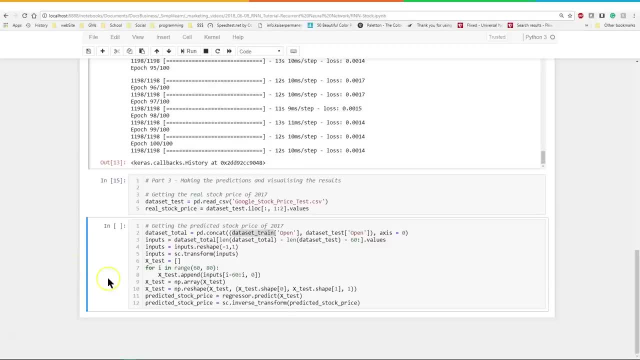 we'll go ahead and go back up here and run this. there we go and you'll notice this is the same as what we did before. we have our open data set. we've pended our two different or concatenated our two data sets together. we have our. 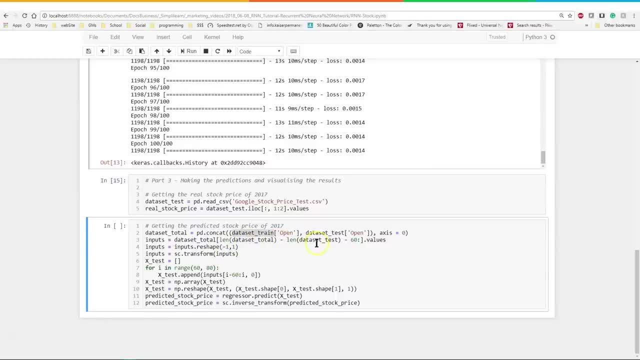 inputs equals data set total length. data set total minus length. the data set minus test minus 60 values. so we're gonna run this over all of them and you'll see why this works, because normally when you're running your test set versus your training set, you run them completely separately. 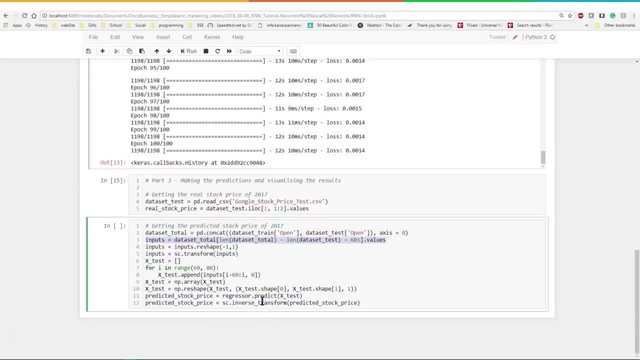 but when we graph this, you'll see that we're just gonna be. we'll be looking at the part that we didn't train it with to see how well it graphs, and we have our inputs, equals inputs, dot, reshapes or reshaping, like we did before. we're 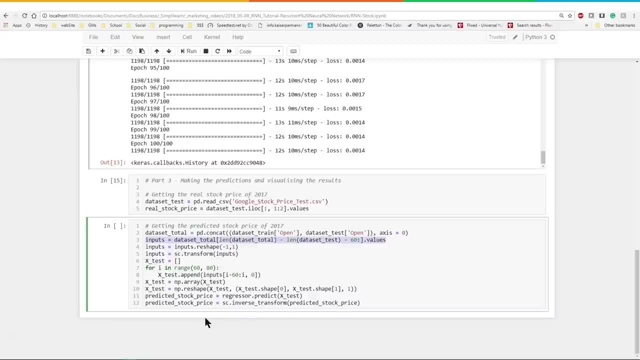 transforming our inputs. so if you remember from the transform between zero and one. and finally, I want to go ahead and take our X test and we're gonna create that X test and for I, in range 60 to 80. so here's our X test and we're 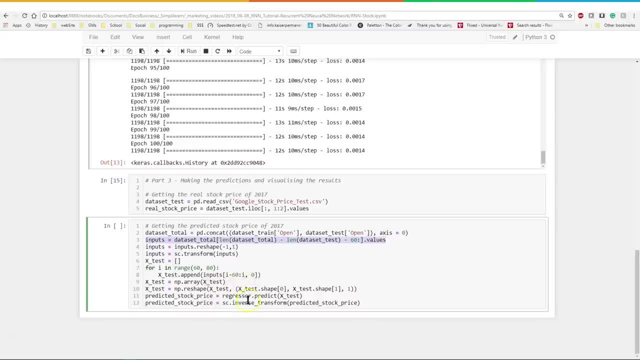 appending our inputs I to 60, which remember is 0 to 59, and I comma 0 on the other side. so it's just the first column which is our open column, and once again we take our X test, we convert it to a numpy array. we do the same. 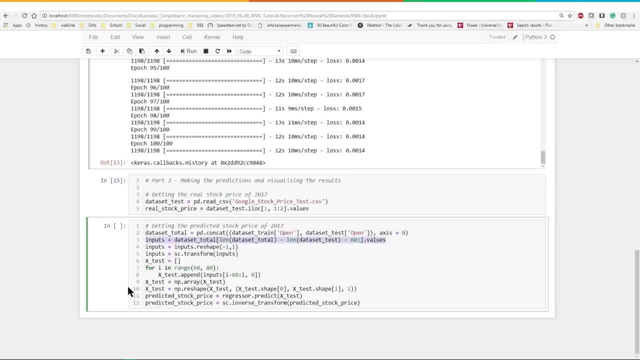 reshape we did before, and then we get down to the final two lines and here we have something new right here on these last two lines, let me just highlight those or mark them: predicted stock price equals regressor dot predicts X test. so we're predicting all the stock, including both the training and the testing model. 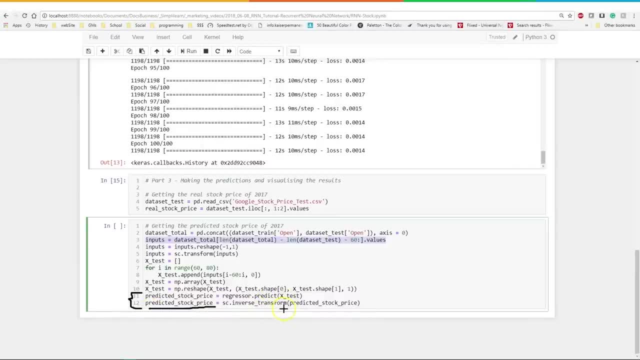 here and then we want to take this prediction and we want to inverse the transform. so, remember, we put them between 0 and 1. well, that's not going to mean very much to me to look at a float number between 0 & 1. I want the dollar. 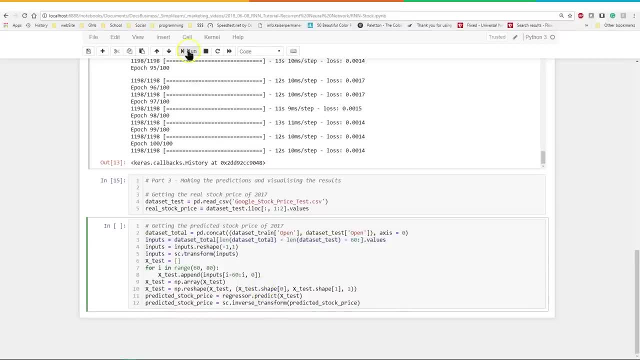 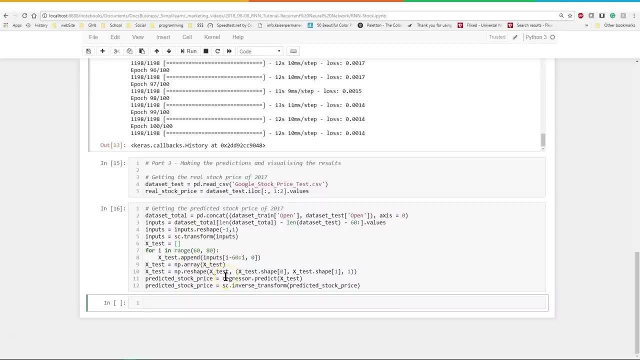 amounts. I want to know what the cash value is and we'll go ahead and run this and you'll see it runs much quicker than the training. that's what's so wonderful about these neural networks: once you put them together, takes just a second to run the same neural network that took us what a half hour to train head and plot. 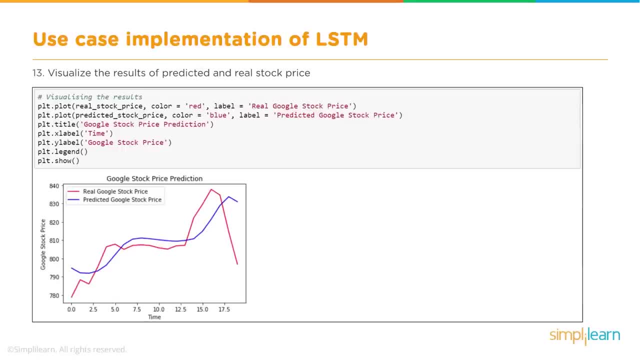 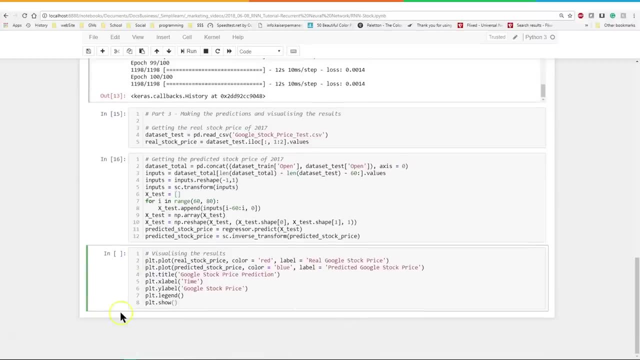 the data. we're gonna plot what we think it's gonna be and we're gonna plot it against the real data, what the Google stock actually did. so let's go ahead and add in code and let's pull this code up so we have our PLT. that's our hope. if 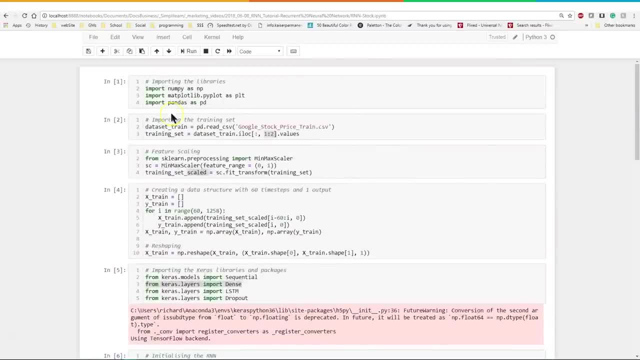 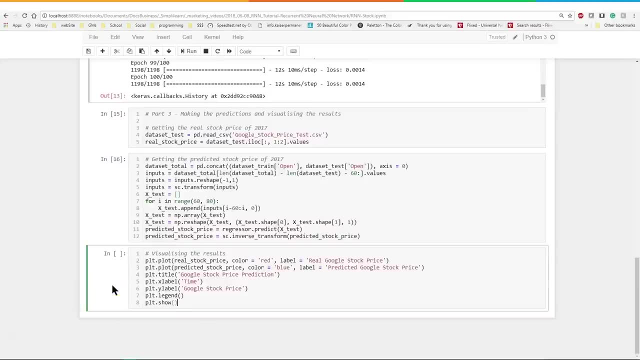 you remember from the very beginning- let me just go back up to the top- we have our matplotlibpyplot as PLT. that's where that comes in and we come down here. we're gonna plot- let me get my drawing thing out again. we're gonna go ahead and PLT is basically kind of like an object. it's one of the things that. 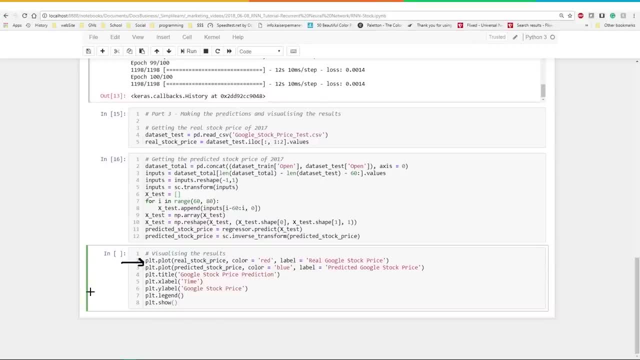 always threw me when I'm doing graphs in Python, because I always think you have to create an object and then it loads that class in there. well, in this case, PLT is like a canvas: you're putting stuff on. so if you've done HTML 5, you'll 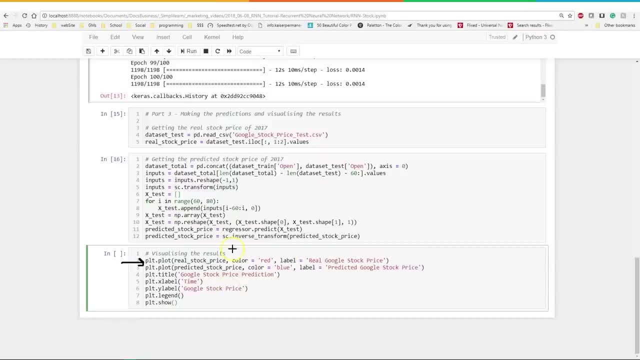 have the canvas object. this is the canvas. so we're gonna plot the real stock price- that's what it actually is- and we're gonna give that color red, so it's gonna be a bright red. we're gonna label it real Google stock price and then we're gonna do our predicted stock. we're gonna do it in blue and it's gonna 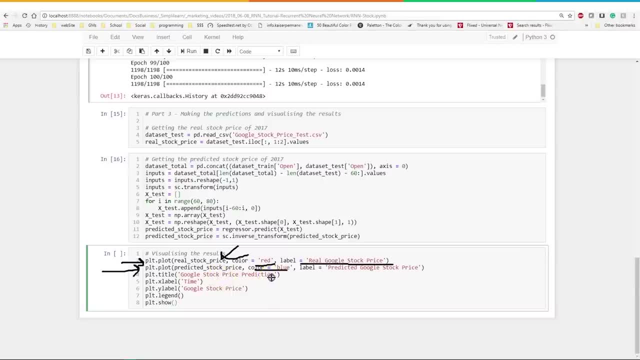 be labeled, predicted, and we'll give it a title. it's always nice to give a title to your graph, especially if you're gonna present this to somebody you know, to the office. and the X label is gonna be time, because it's a time series and we 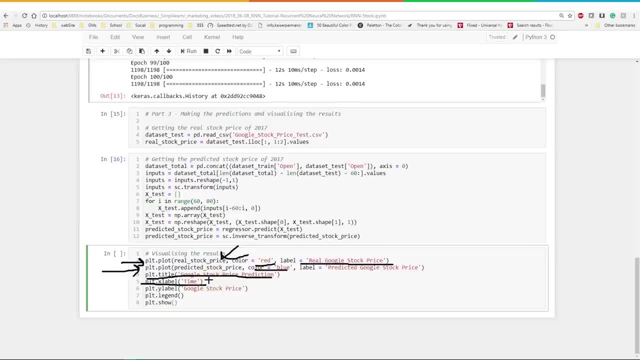 didn't actually put the actual date and times on here, but that's fine, we just know they're incremented by time. and then, of course, the Y label is the actual stock price. PLT dot legend tells us to build the legend on here so that the color red and real Google stock price show up on there. and then the plot shows. 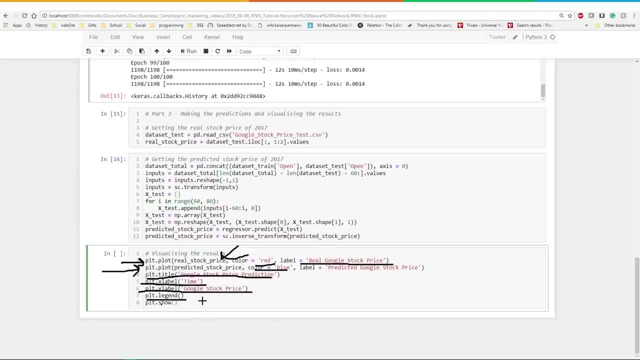 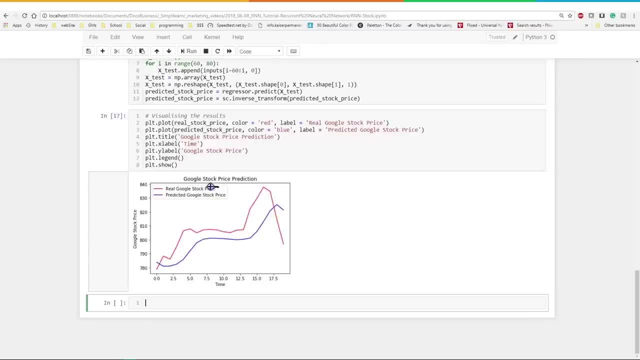 us that actual graph. so let's go ahead and run this and see what that looks like, and you can see, here we have a nice graph and let's talk just a little bit about that before we wrap it up. here's our legend. I was telling you about that's. 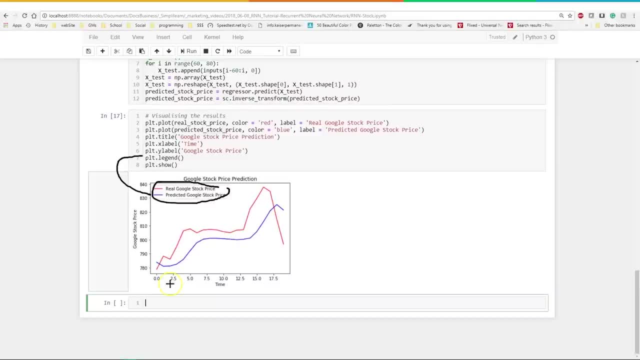 why we have the legend to show the prices. we have our title and everything, and you'll notice, on the bottom we have a time sequence. we didn't put the actual time in here. now we could have. we could have gone ahead and plotted the X, since we know what the dates are, and plotted this to dates, but we also know that it's. 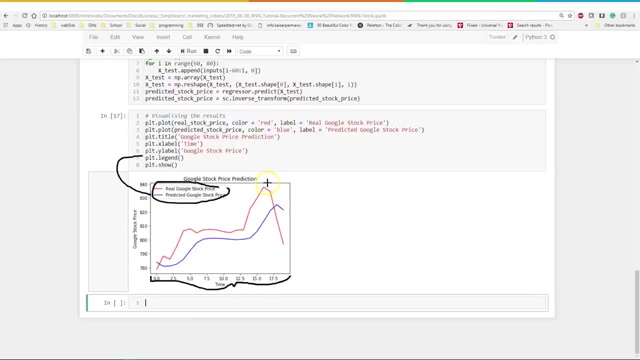 only the last piece of data that we're looking at. so last piece of data which, in somewhere, probably around here on the graph, I think it's like about 20 of the data, probably less than that- we have the Google price and the Google price has this little up.